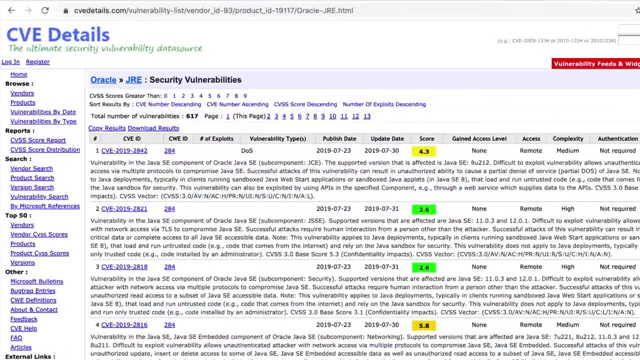 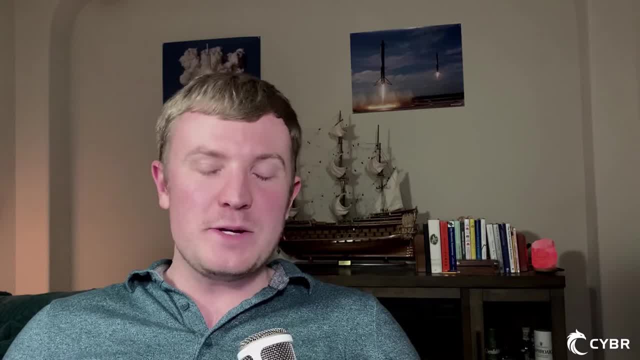 say that they don't have issues of their own, which we'll explore further in the course, but you get the idea. So I embarked on a journey to figure out how my application was compromised so quickly and easily and how I was able to get it to work. And that's when I found out that I had to go back to. 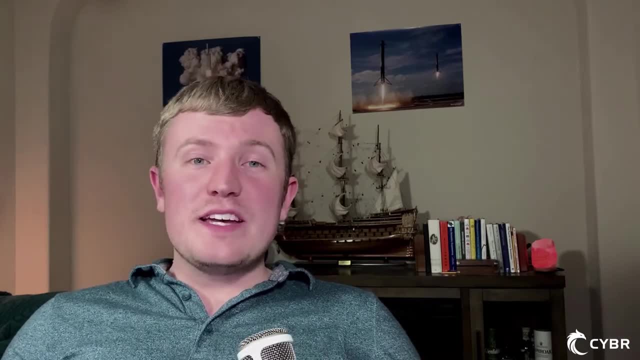 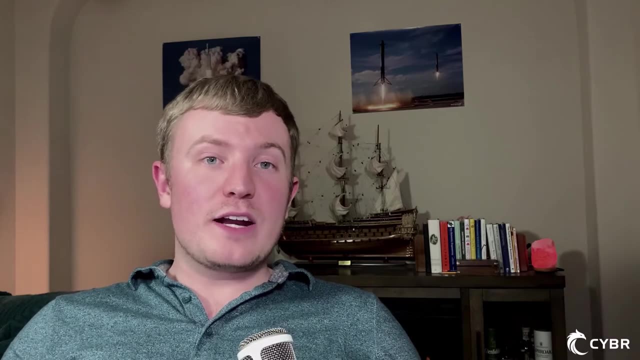 the internet. And after a few years of figuring it out, here I am today. Now this course is going to be more conceptual and higher level, since it is an introductory level course, but in the future we will release courses that go deeper, dive into application. 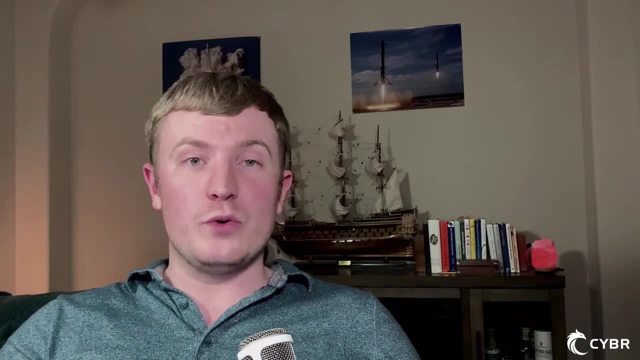 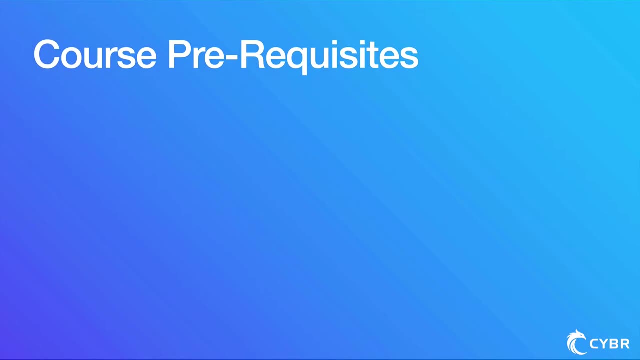 security. That way you can get your hands dirty learning with real world examples. Now, with that, we also assume a few things and consider the following to be prerequisites For one: we assume that you have at least a couple of years of programming experience. 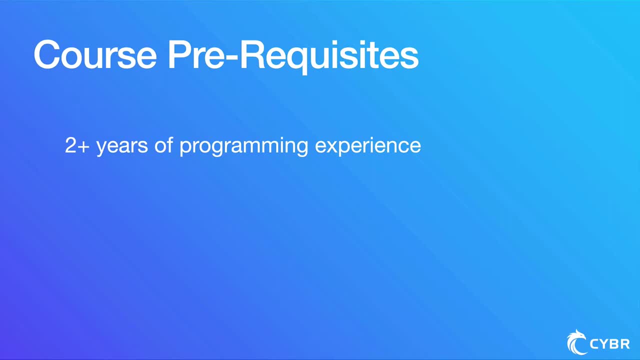 The language doesn't really matter, at least in regards to this course, but if you don't have any programming experience, this is probably not a course that you want to start with. We also assume that you're familiar with typical software development models- software engineering. 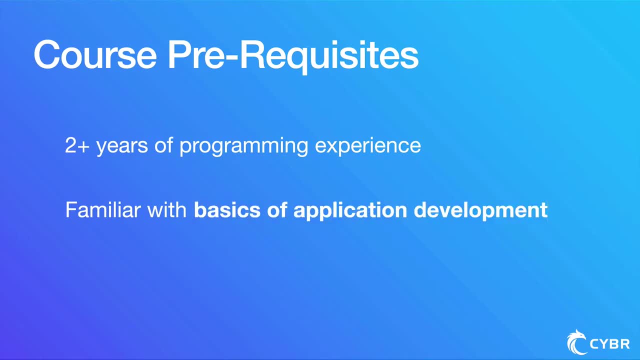 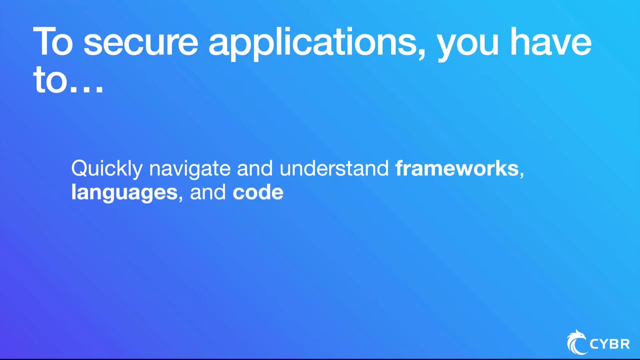 in general and just the basics of application development, because in order to secure applications, you have to be able to quickly navigate and understand frameworks, languages and code that you may not be familiar with, and you also need to have some familiarity with the 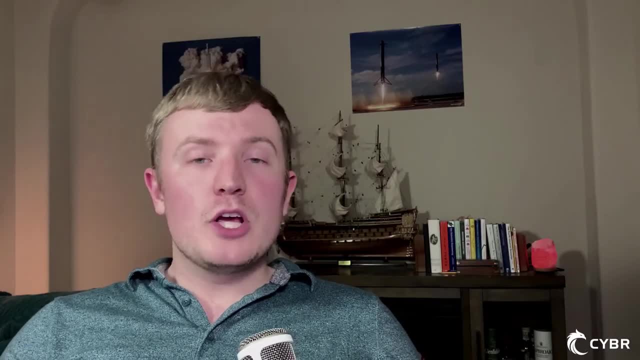 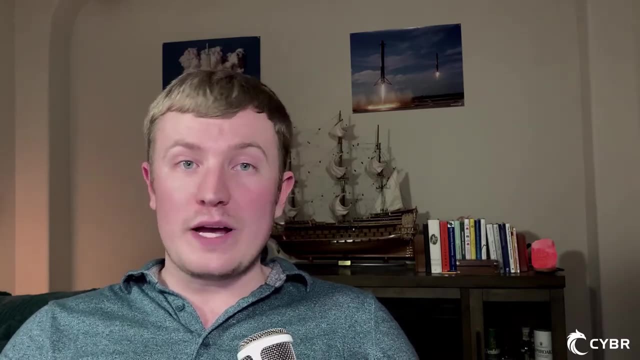 platform the code is running on. So if you're focusing on web development, you should know some basic Linux, or if you're focusing on mobile applications, you should have some application security and development. then you should know iOS or Android or maybe both. 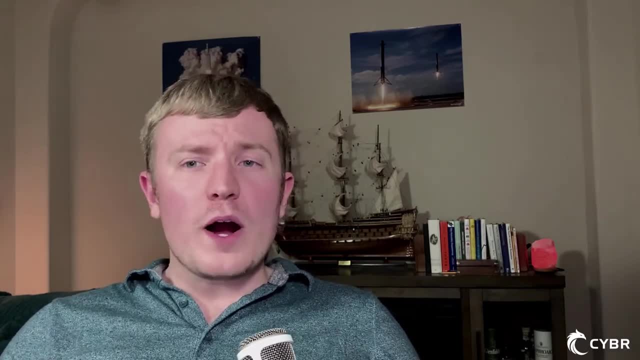 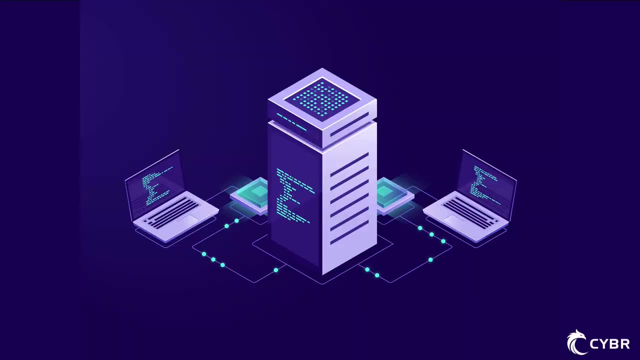 and so on. Now we'll talk more about application security, job requirements in the next lesson, but at the end of the day, you will be spending the bulk of your time analyzing source code, manipulating requests between your application and backend services and trying to find holes. 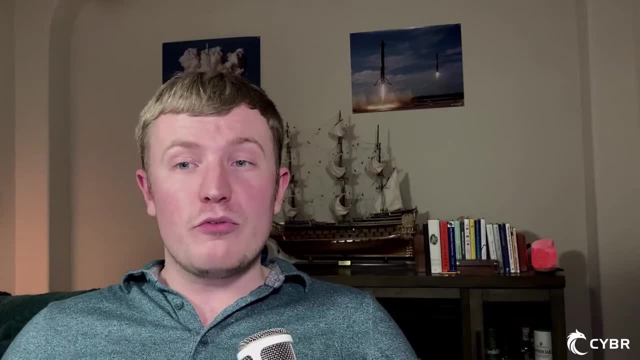 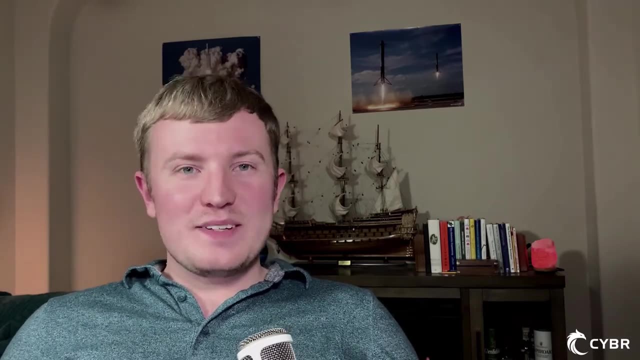 in the application security, And if you've never touched a line of code before, you simply won't be able to do this. So I'd recommend that you pause here and enroll in programming courses that pique your interest. But if you're still watching, I'm excited to get started. 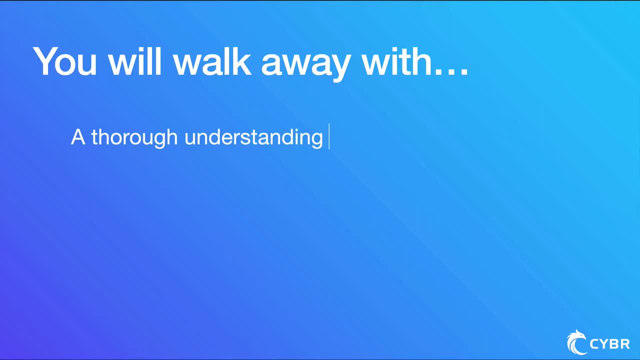 By the end of this course, you will walk away with a thorough understanding of application security concepts and how they relate to web, mobile and cloud applications, so that you can then dive deeper into those respective areas, depending on your interests and or job requirements. 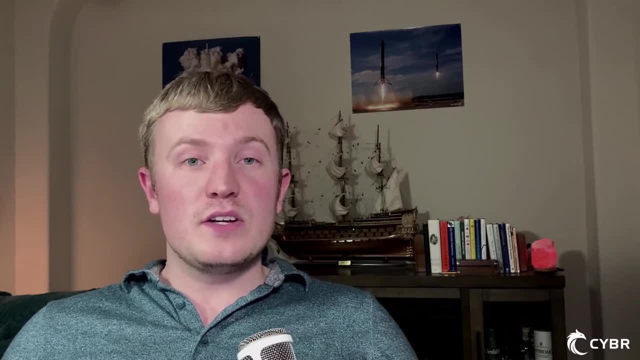 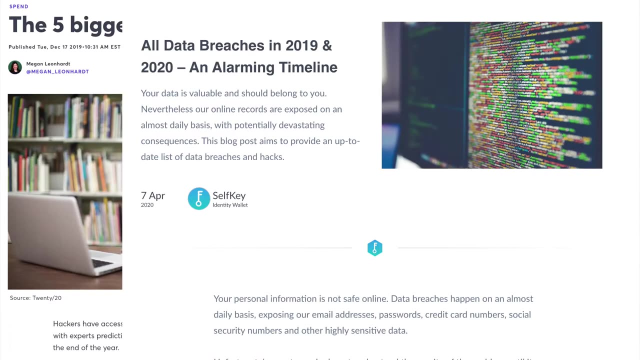 And now let's mark this lesson as complete and let's move on to the next lesson, where we explore application security jobs. We've become so accustomed to seeing reports like this and this and this, which all happened in the last couple of years, And we're talking about very public. 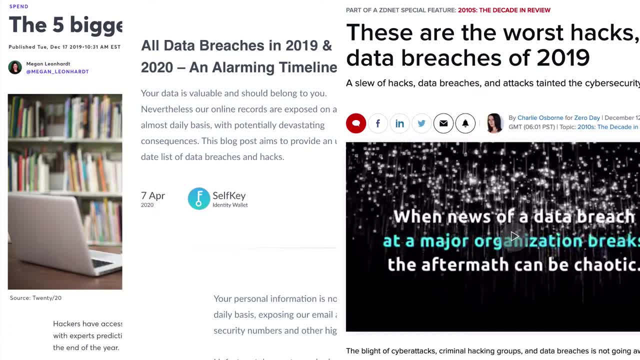 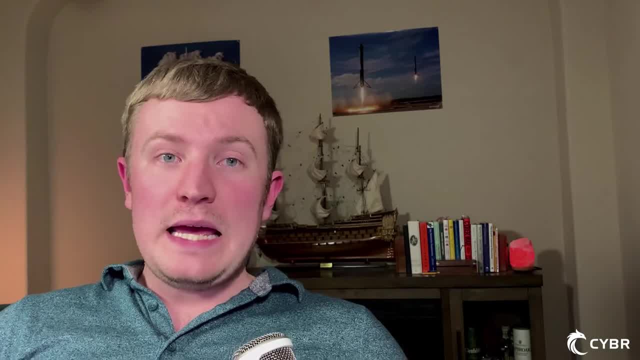 hacks on organizations that have massive budgets compared to small businesses, And while all these hacks could have been avoided, the fact of the matter is that this is complicated business. In fact, it's so complicated that organizations hire individuals to take care of securing their 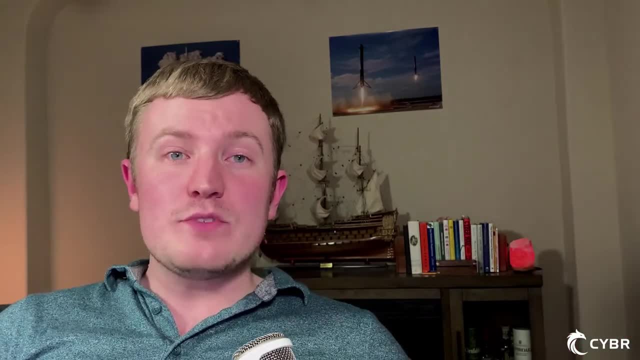 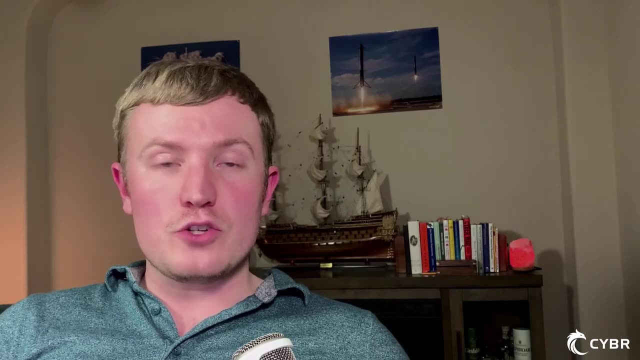 applications, Or sometimes they even hire entire teams or even entire departments to take care of this stuff. Now, if you're here, you're probably interested in learning more about application security, or you're interested in getting a job in application security, or maybe you already work. 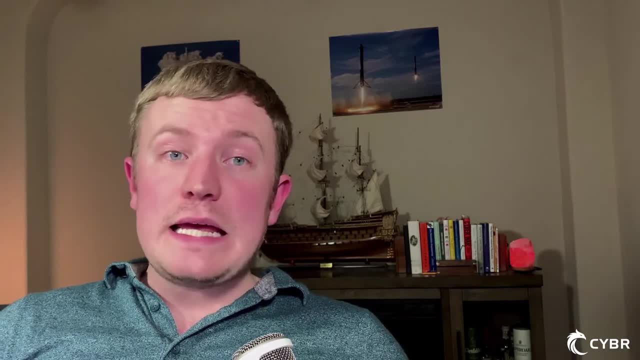 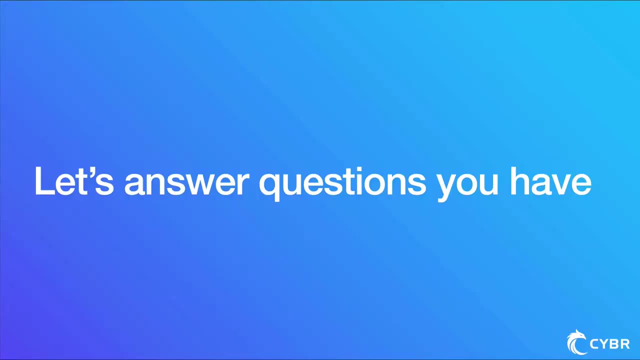 in the field and you're just looking to formalize your training. This lesson is geared more towards the people who are looking to enter this field, and this is their starting point. So this lesson aims to answer questions that you most likely have, such as: what kinds of jobs can I get with? 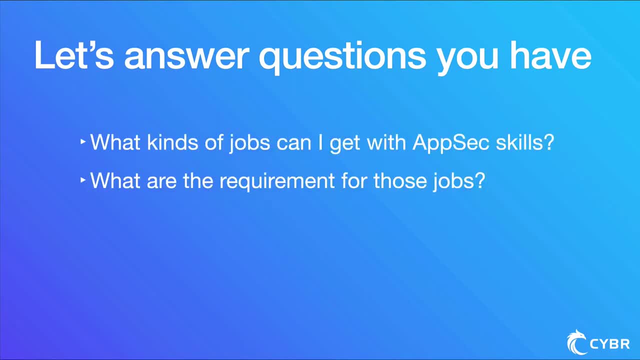 application security skills. What are the requirements for those jobs? What kinds of salaries can I expect, Etc? Now let's start with the first question, since it will help us answer all the others. Let's start with what kinds of jobs can I get with application security skills? 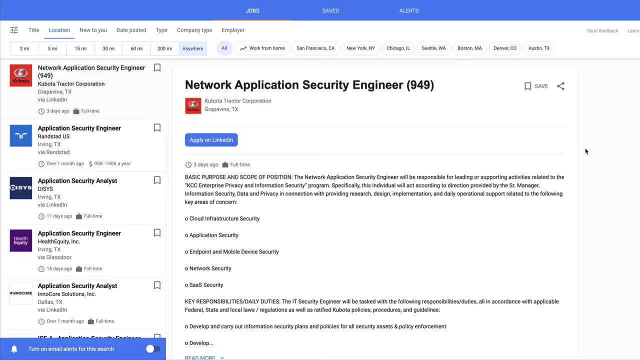 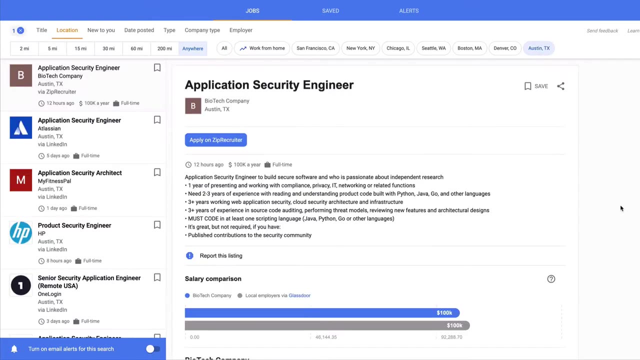 There are a number of different search engines that you can use to find jobs online, but in this case we're just using the basic Google job search. From here you can select a location or any other filter that you want, And in my case I'll just select Austin, Texas, And, as you can see, there, 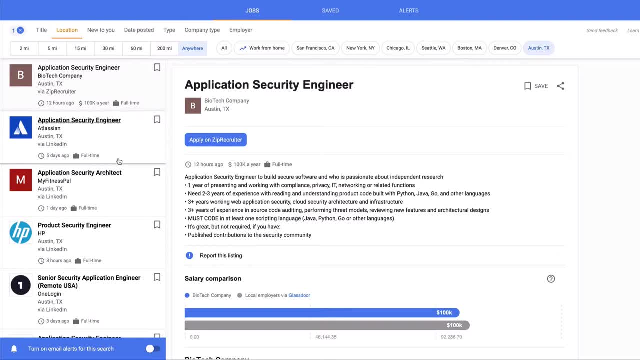 are a lot of different positions on the left-hand side with different titles, but that all tie back to application security. For example, application security engineer. application security engineer here as well. Application security engineer here as well. Application security engineer here as well. 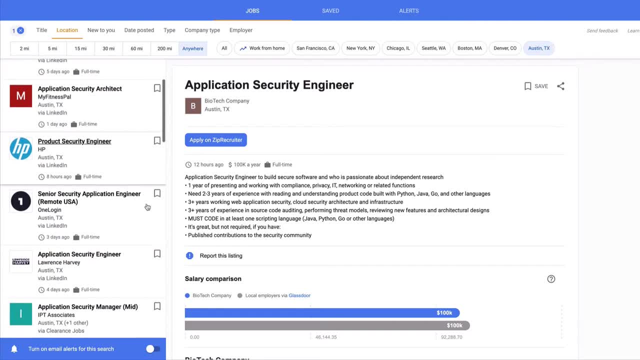 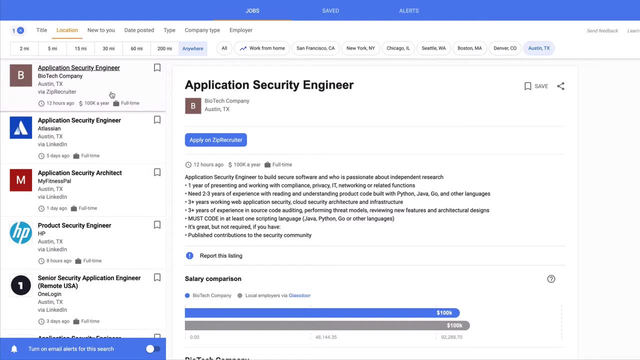 Application security architect here, product security engineer, a senior security application engineer, even application security managers and more. But if we click on these different jobs, we can look at the requirements And in some cases they also post the salary range. So this: 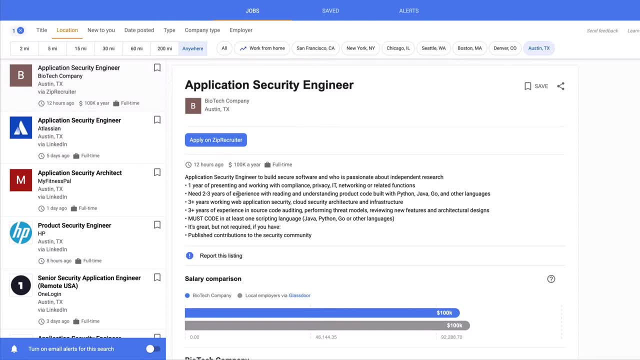 is for a biotech company And if we look at the requirements, it says: one year presenting and working in compliance. privacy, IT networking or related functions. two to three years of experience with reading and understanding product code with Python, Java, Go and other languages. web application security, cloud security. 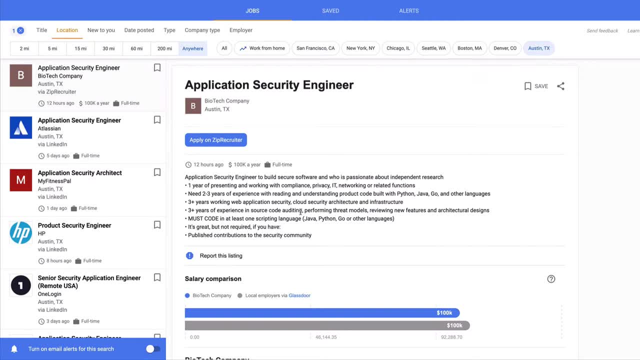 architecture and infrastructure, source code auditing, performing threat models, reviewing new features and architectural designs, And these are some of the topics that we will cover in the course, though not all of them, but that gives us a good idea for this job. 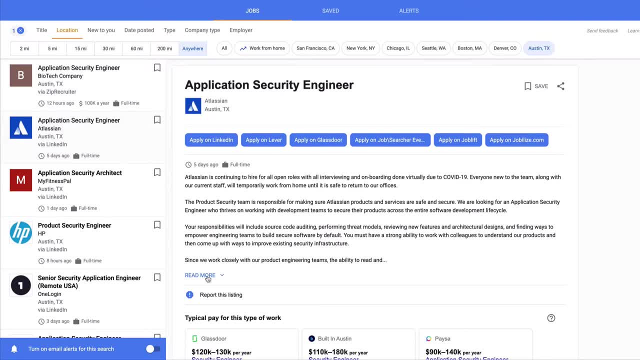 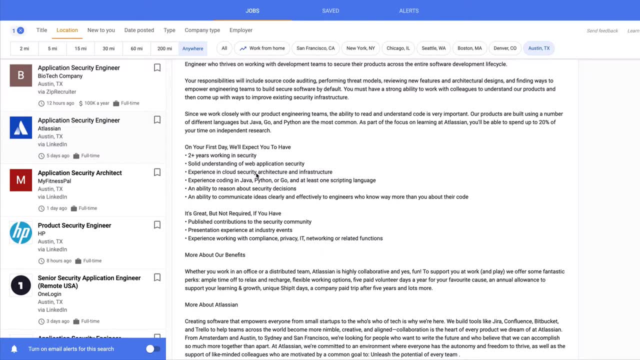 Next, we can look at a post by Atlassian for an application secure engineer. Again, we can look at some of the requirements Here. it does say a solid understanding of web application security, cloud security, architecture and infrastructure- something we will touch on in this course. 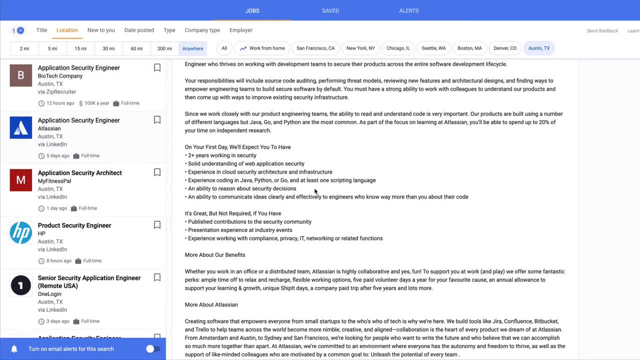 Again, experience, coding- and we've talked about this- An ability to reason about security decisions, ability to communicate ideas clearly and effectively to engineers who know way more than you about their code. This is an important topic that we will touch on more and more, And 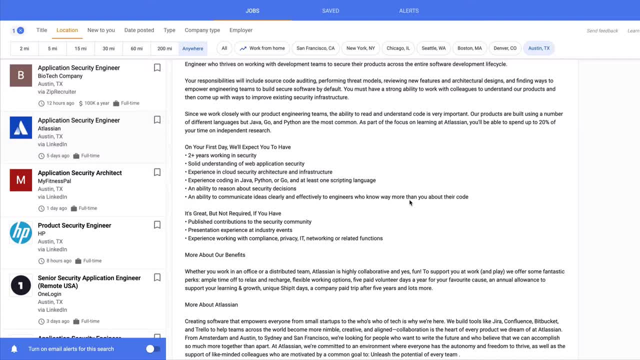 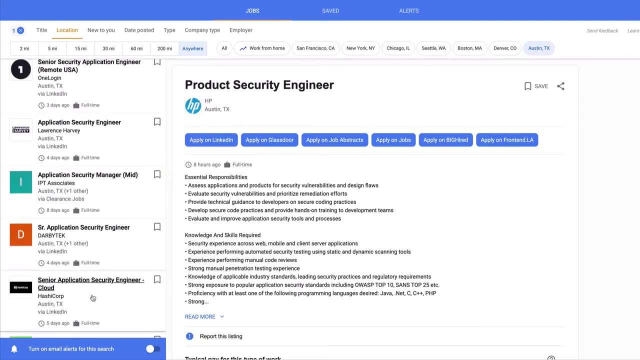 also something to keep in mind. being able to communicate to a group of engineers would be very important in this position. We can continue to look at different ones, For example one here by HashiCorp. This one is a senior application security engineer, but just to get an idea of 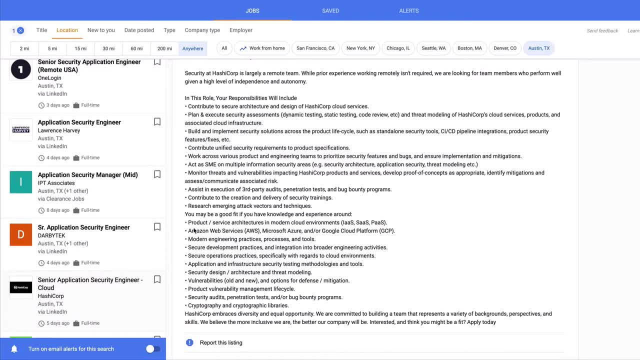 what that looks like. There are definitely a lot more requirements here. They even name out Amazon Web Services, Azure or Google Cloud Platform. so knowing cloud is important. Security design, architecture and threat modeling, vulnerabilities and options for defense and mitigation. 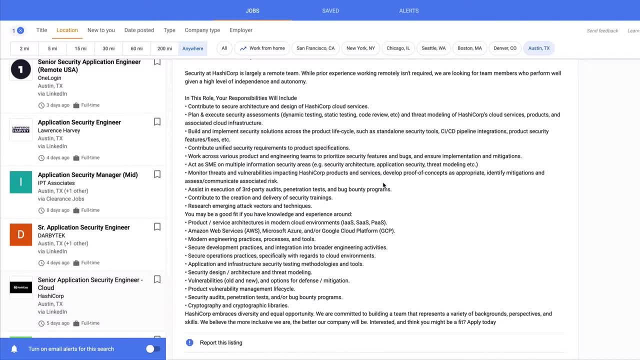 and a whole lot more. So so far, just by looking at two or three different postings. a lot of these will also include requirements to be familiar with cloud and cloud security, like AWS, for example, And this is a topic, like I said, that we do cover a little bit in this course. 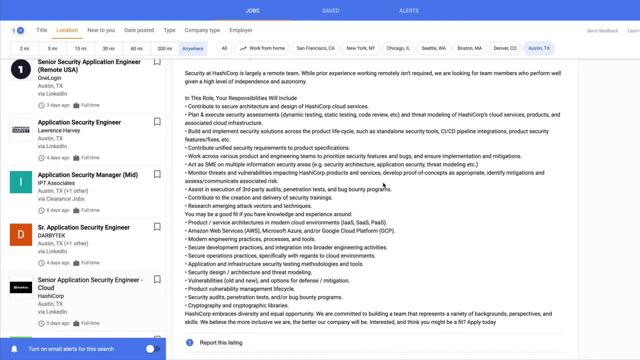 But if you see any position that piques your interest in particular, look at those requirements and compare to your current skill set And then at the end of this course, you will have a better idea of where your knowledge gaps are, so that you can focus in those areas And again, not all of. 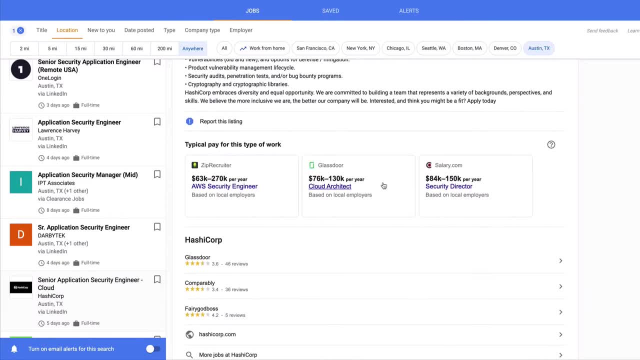 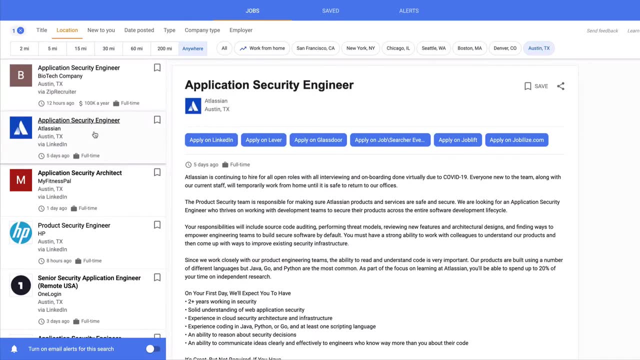 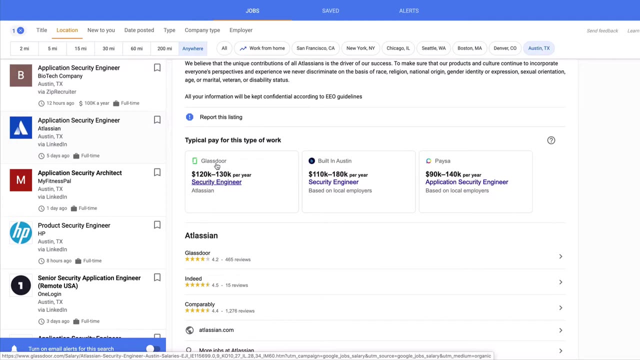 these postings have salary ranges, but you can get an idea by scrolling to the bottom and looking at the typical pay for this type of work. Each of these postings should have something similar, But also keep in mind that you can go to these respective websites, such as Indeed Glassdoor. 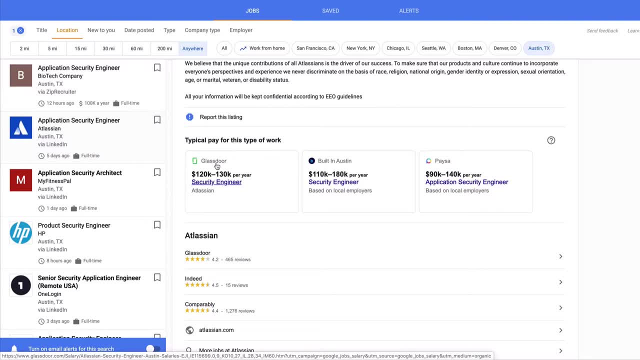 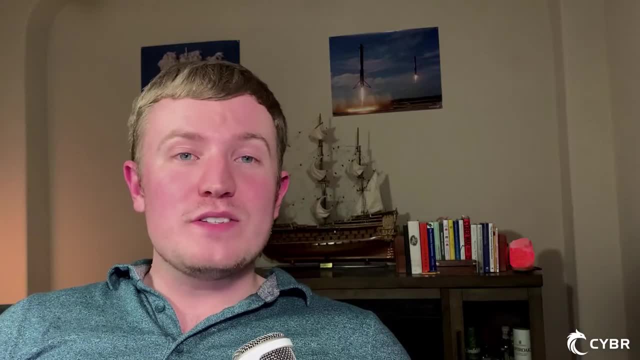 Salarycom, PESA and other ones, and you can put in your location, your experience level and other important factors and they can give you a salary range. So, looking at all these questions, here's what we can generalize so far. Salary ranges are always really hard because they depend on too. many factors, But when I looked at positions in Austin for entry level, most of them had a starting salary of just about $80,000.. And when I looked at positions in Austin for entry level, most of them had a starting salary of just about $80,000.. So getting to six figures is definitely achievable. 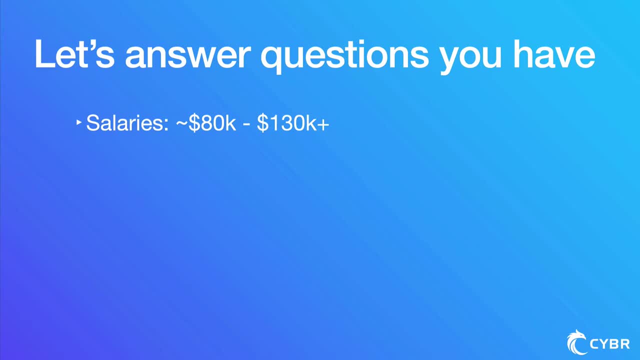 either right away or as you get more experience under your belt And as an application or software security engineer, you can expect to develop and write new or even modify existing computer applications or software or utility programs, And you have to do that following security best. 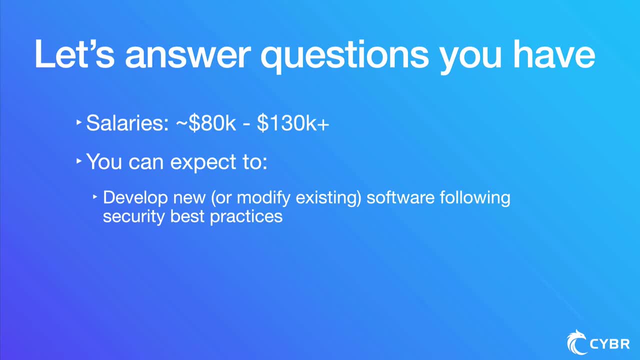 practices, So it's important that you understand what those security best practices are, And that is a big part of this course. You can also be expected to secure new or existing applications that others have not yet developed. So if you're looking to get into a new or existing application, 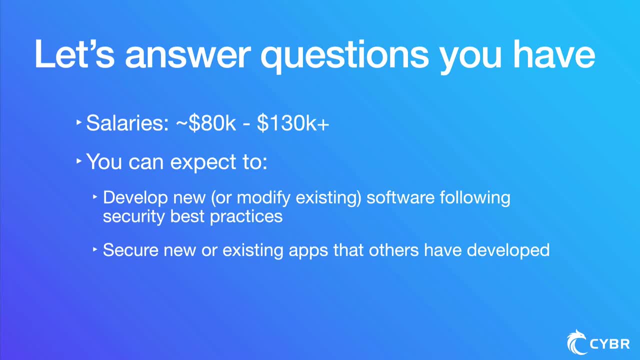 you can expect to get into a new or existing application that others have not yet developed, Which means that you need to be able to understand and analyze other people's code. ensure that this code meets software security best practices and that it aligns with your. 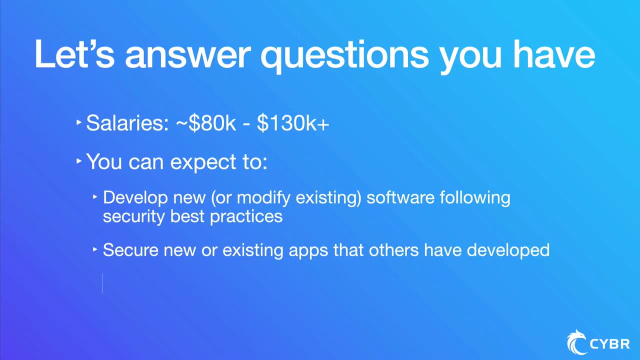 business's risk appetite. Now this all means that you need to put yourself in the shoes of an attacker and identify the potential different paths through your application that attackers can use to do harm to the business. So you need to be able to think through, not just the code. 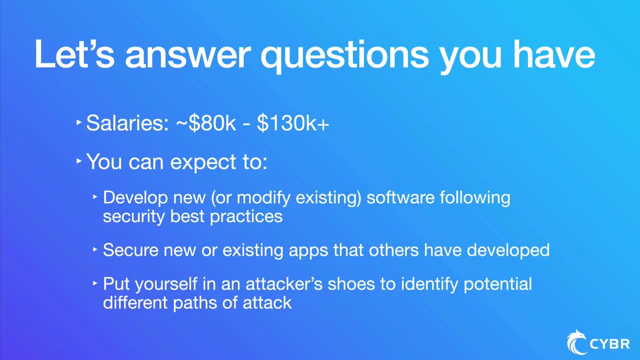 but the entire application as a whole, Because that application likely speaks to a database, likely has authentication and likely has a security system. So you need to be able to consider the userhistoire of your application when it comes to securing the product. Now, if you're looking to enter a threat transaction- CTV projects- I'll explain this. 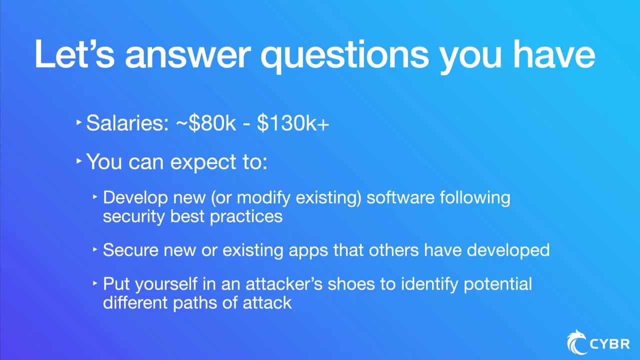 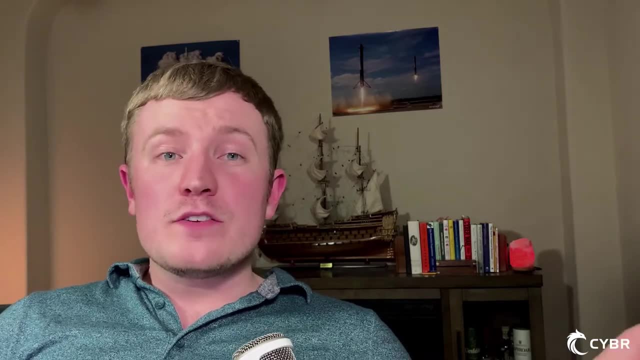 in a step-by-step way. that's more information with respect to this and the ways to do this. just check the information tab. What you want to keep in mind is that you aren't entirely only going to be checking a delicateness of a data structure, live scenarios or resources or 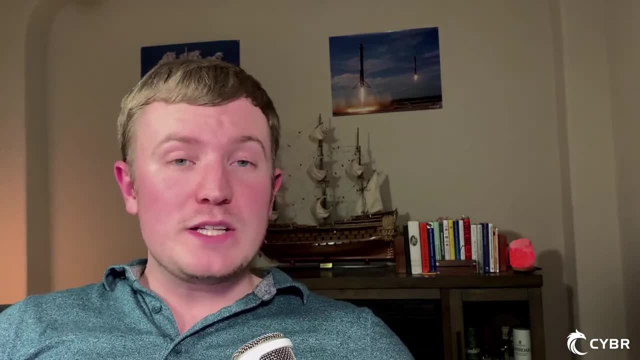 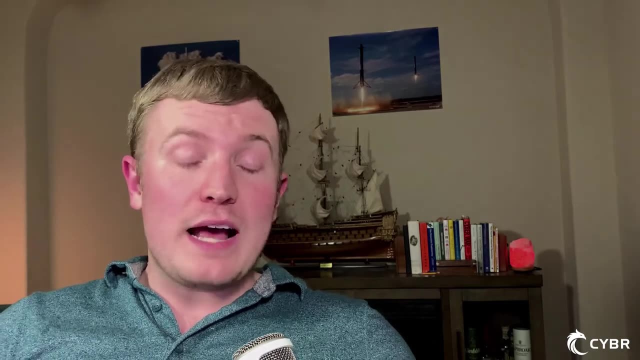 smelting your info, You need to also be aware of the alpha pass code already covering data and interactions. This is an important trick because you don't play with this hack for easy access. the fear of problems- So the big is which- or immediate danger and could causeоз. 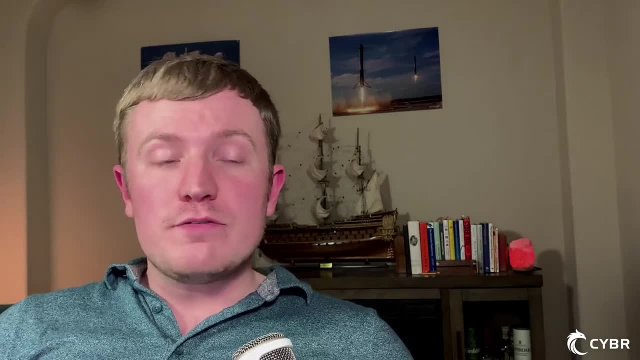 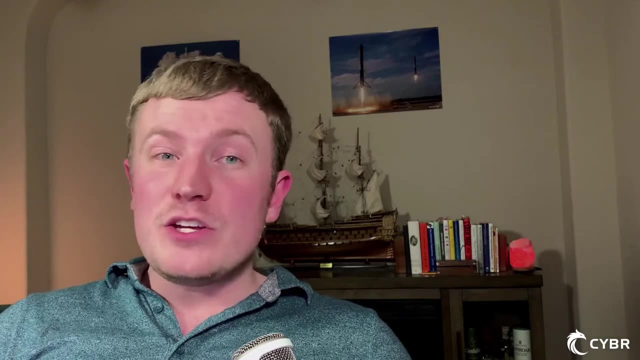 issues. So dis powin be how thisGL application can serve, and کمر highly recommend that you at least familiarize yourself with those different areas, even if you're going to specialize in application security specifically. that way you can speak about it. 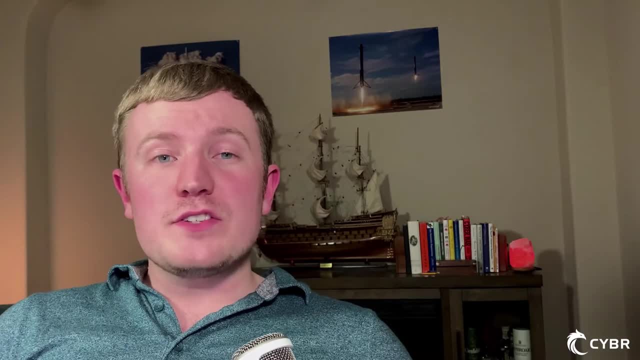 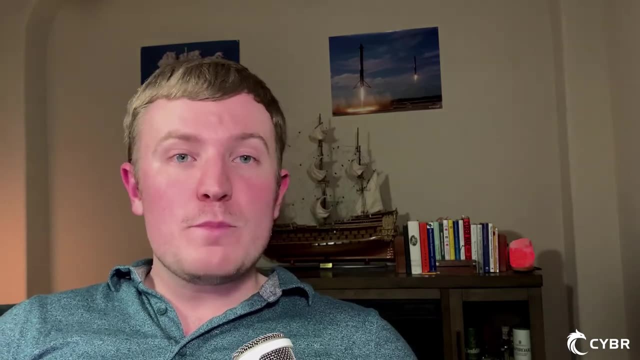 intelligently. Now, as we wrap up this lesson, in the next lesson we are going to explore something called the NICE framework and OWASP, And these two things will give us blueprints to better understand what's required from us to enter the application security field in terms of specialty. 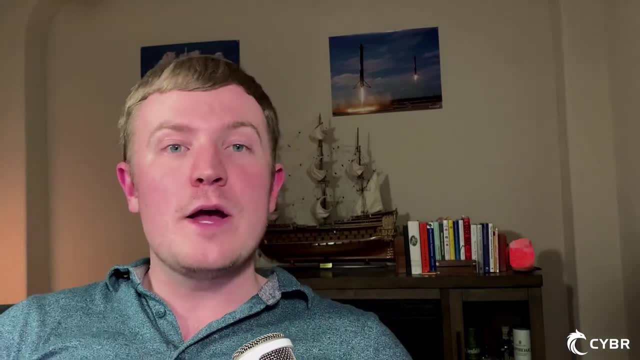 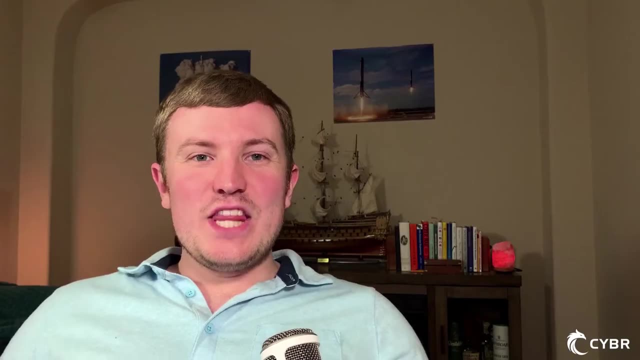 areas in terms of skills, knowledge, abilities and things like that. So go ahead and complete this lesson and I'll see you in the next lesson where we explore this in a lot more detail. In the previous video, we talked about application security as a job, and we even looked at different 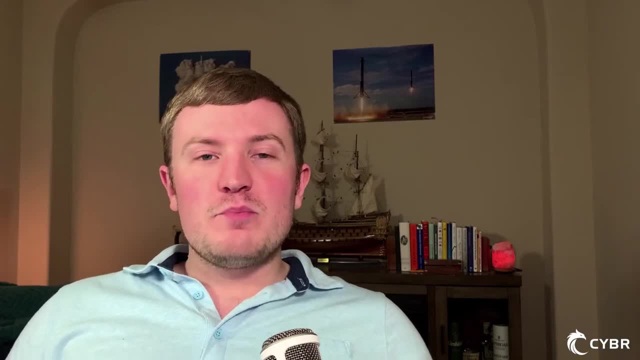 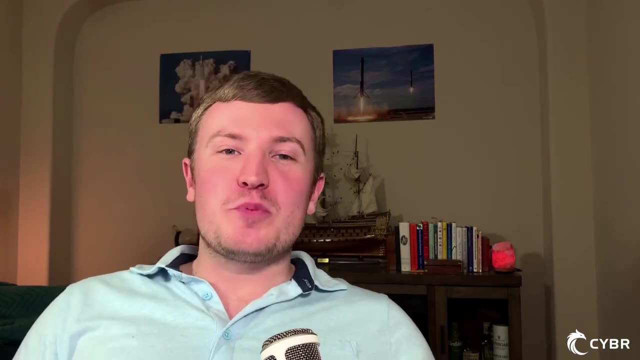 job postings to see what kinds of requirements we could expect. But wouldn't it be nice if there were a NICE framework that could tell us what to focus on? Okay, I admit that was pretty cheesy, but you do have to admit that it is a clever acronym. 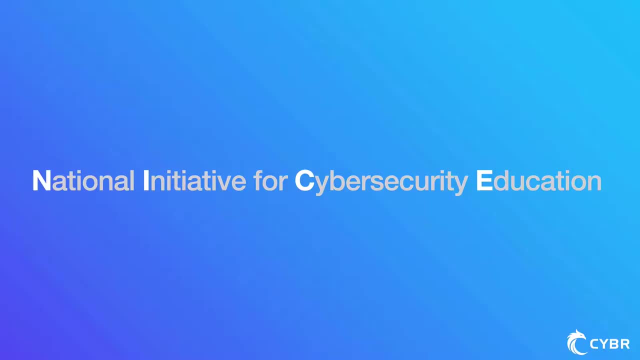 The National NICE Initiative for Cybersecurity Education came up with a cybersecurity workforce framework, but that takes way too long to say, so they've abbreviated it to just calling it the NICE framework. In any case, it was developed in partnerships with NICE, the Office of the 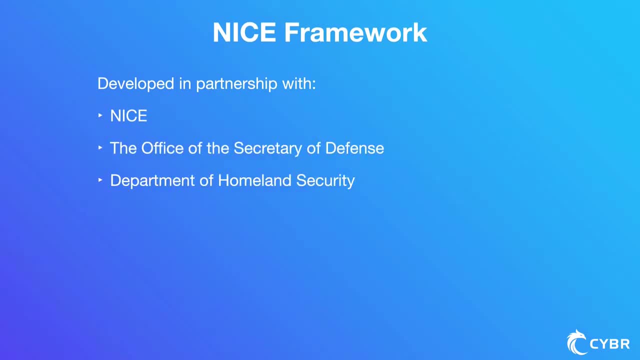 Secretary of Defense and the Department of Homeland Security to provide educators, students, employers, employees, training providers and even policymakers with a systematic and consistent way to organize the way that we think and talk about cybersecurity work, and to identify the knowledge, skills and abilities needed to perform cybersecurity tasks. 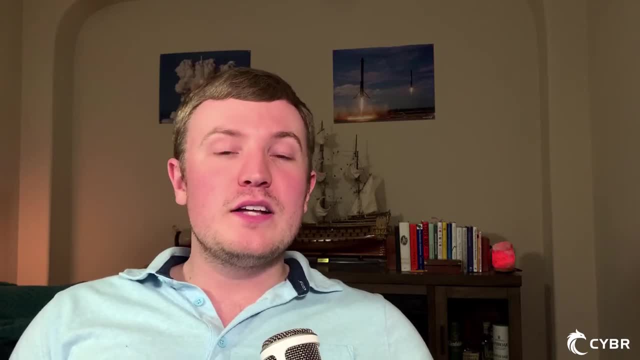 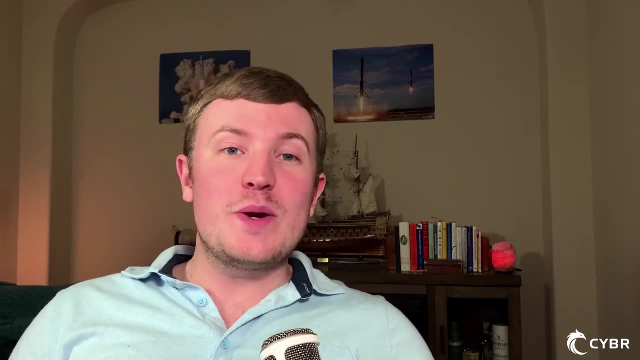 Again, way too much so, in short, let's just say that it's a blueprint to help you organize, categorize and describe cybersecurity work, And, in fact, let's go ahead and just pull up the framework online so we can see exactly what it's like Now that we're on the official website. 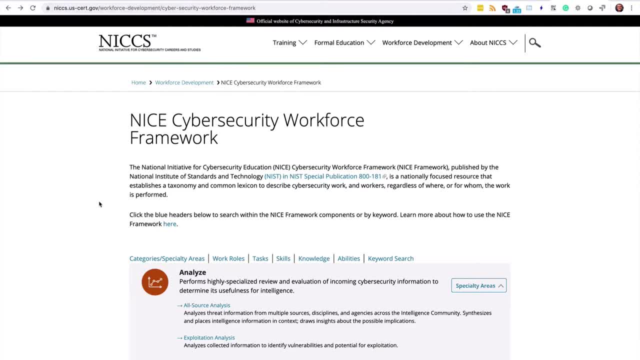 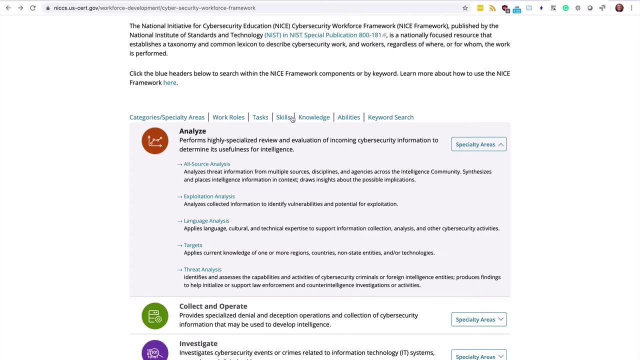 page for this and, by the way, you can go to this URL to follow along. we can now see the different categories and specialty areas, and then we can break it further into work roles, tasks and the SKAs. In our case, we're going to scroll down to the category that is called securely. 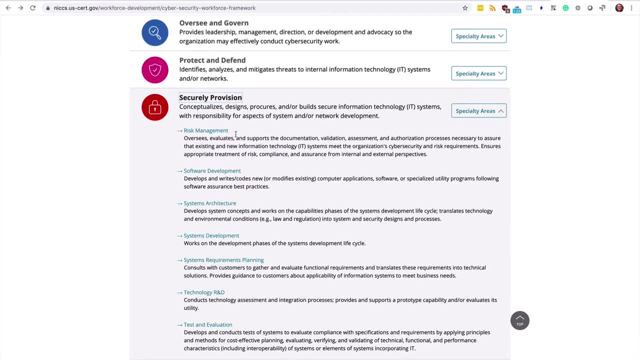 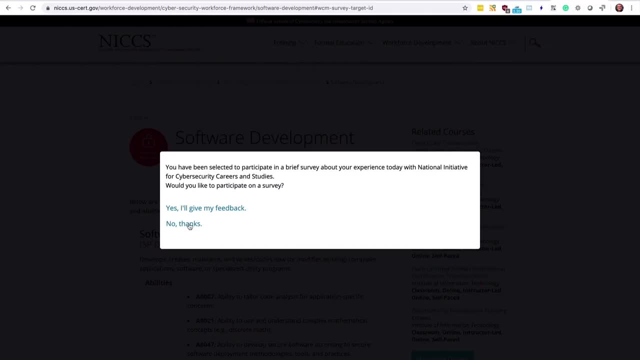 provisioned. From there you can see all the different specialty areas like risk management, software development and so on, and in our case we'll click on software development. You may be asked to enter for a brief survey. I'll just say no thanks in this case. 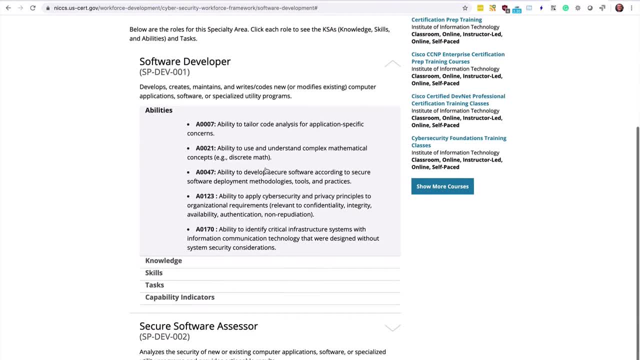 but once we're on the specialty area page, you can now see the different work roles. So in this case we have software developer and we have secure software assessor, And within those different work roles we have the special staff and we have the master staff and then we have the public. 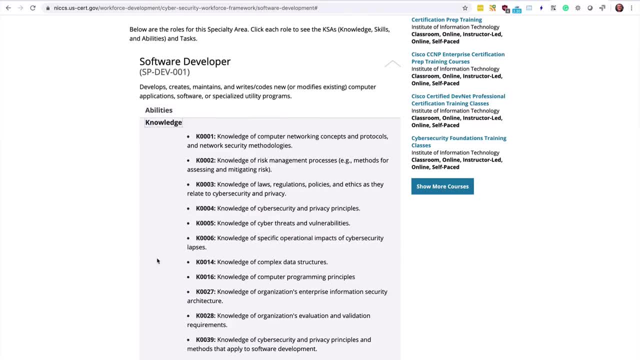 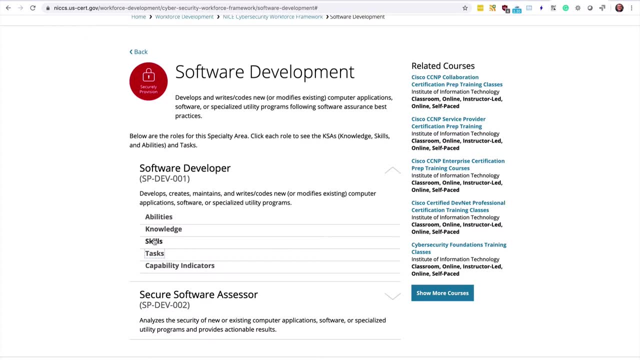 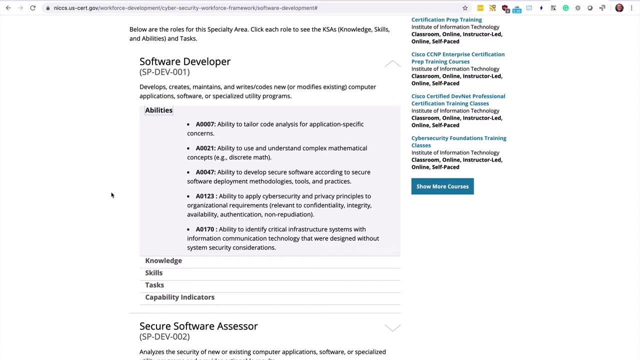 we have the abilities that are broken down here, the knowledge, the skills, the tasks. So these represent the SKAs, and then the tasks and then finally the capability indicators. Now, in this course, obviously we're not going to have the time to cover every single SKA or even task. 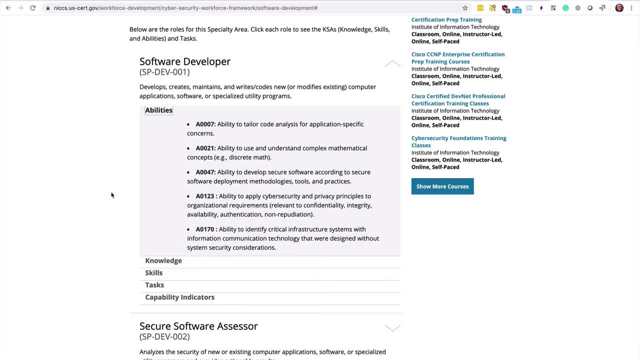 but you can then take what you've learned from the course and fill in your other gaps thanks to this framework, And I highly recommend that you spend more time looking over all of this after you've completed this lesson, so that you can familiarize yourself with these lists. 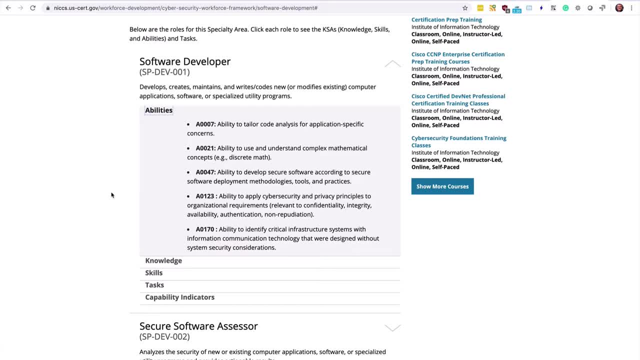 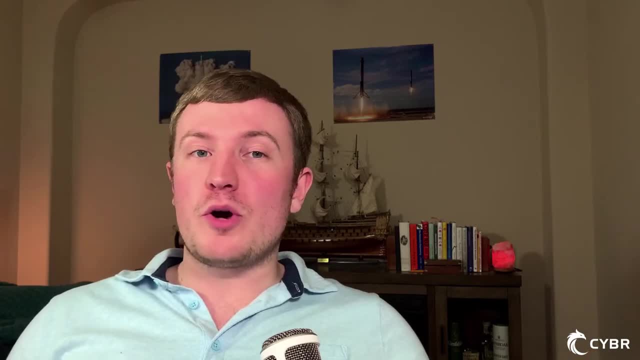 and so that you can take a good look at where you are currently and where you need to be in order to figure out what gaps in skills you need to fill Now, of course, comparing this list to what we looked at in the prior lesson, with different job postings. 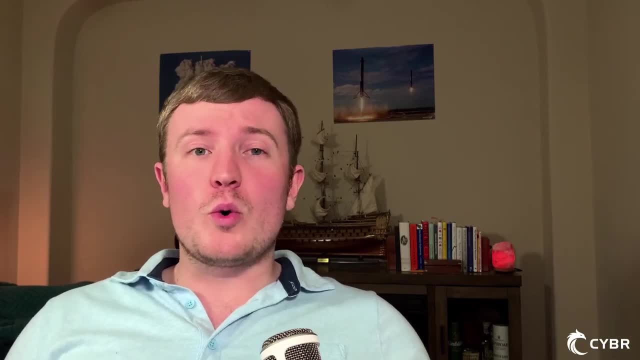 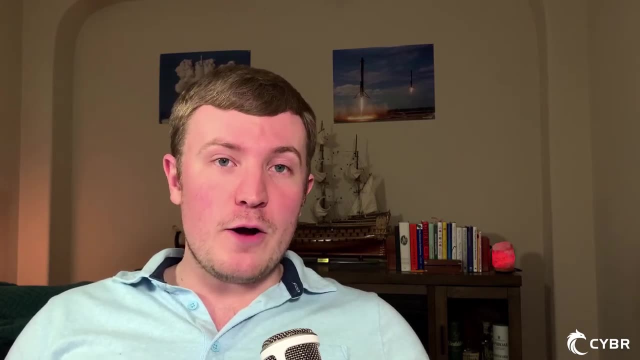 you'll start to realize that not all of the different jobs will require everything that's listed in these lists, So you don't have to have all the knowledge, skills and abilities that the NICE framework spells out, and don't worry about learning all of those. 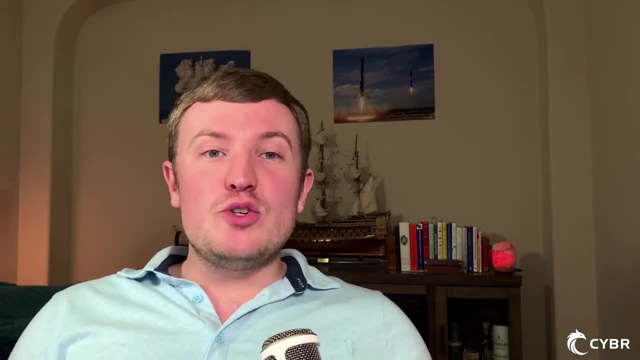 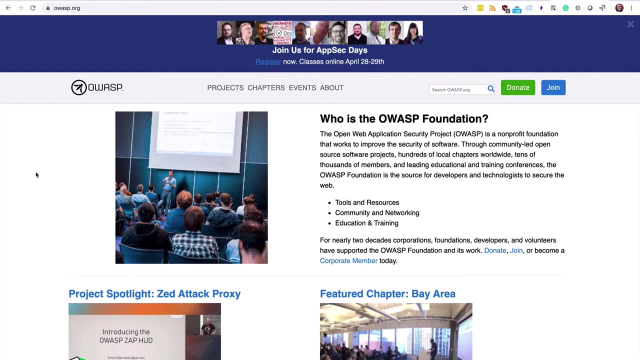 in a month or two months. That's not what we're saying here. Instead, use this as a frame of reference. So that's the NICE framework in a nutshell. Now let's take a look at OWASP, The Open Web Application Security Project. 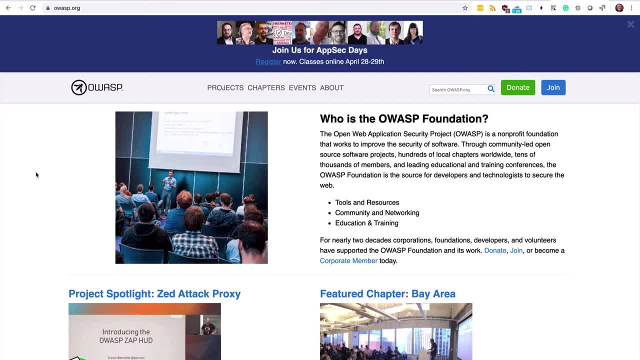 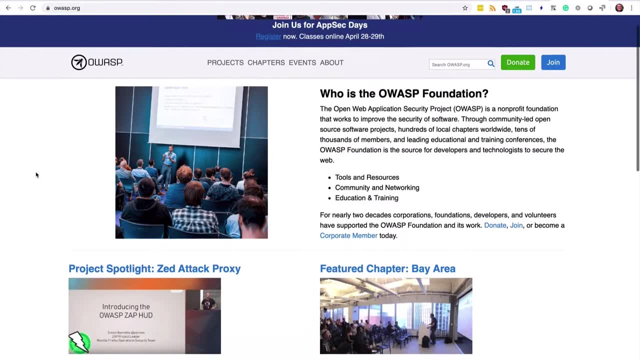 or OWASP for short, is a nonprofit foundation that aims to improve the security of software, and they do this by being vendor agnostic. They provide a breadth of resources and standards to help developers improve the security of software, and we will be leaning heavily on their work. 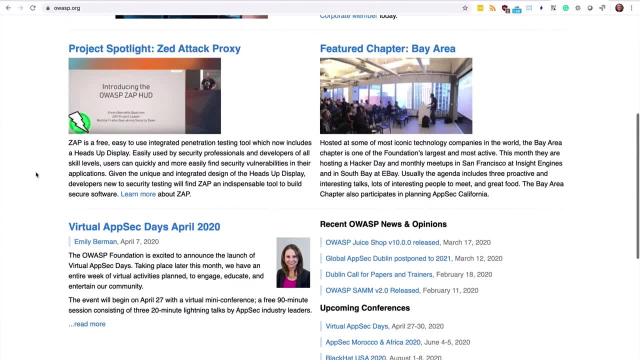 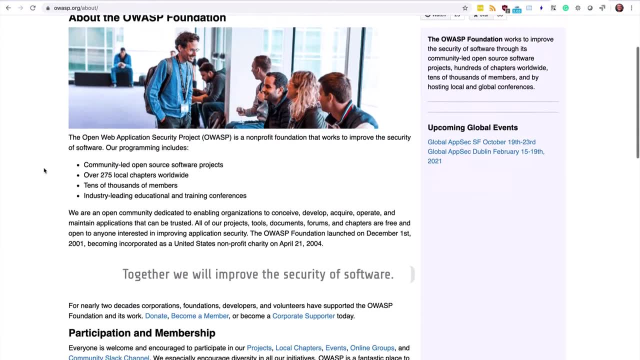 throughout the remainder of this course. That way, you can reference their projects during the course, but also after you've taken the course and when it's time to apply what you've learned on the job or even on personal projects. Plus, if you're in this industry. 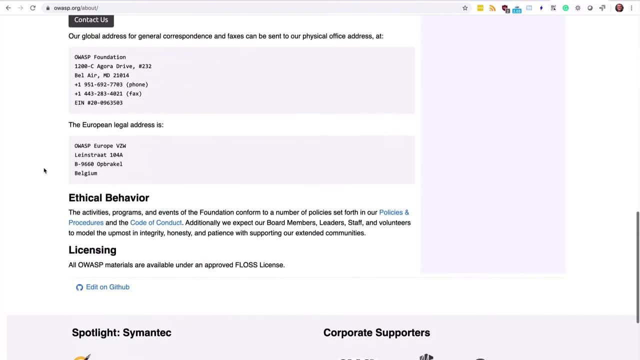 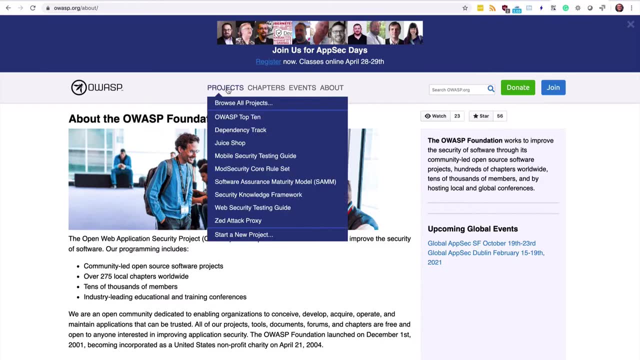 you will often hear people reference OWASP, so that the next time someone mentions it, you know exactly what they're talking about. Let's take a quick look at their projects so that you can see what I mean. They have a number of different projects. 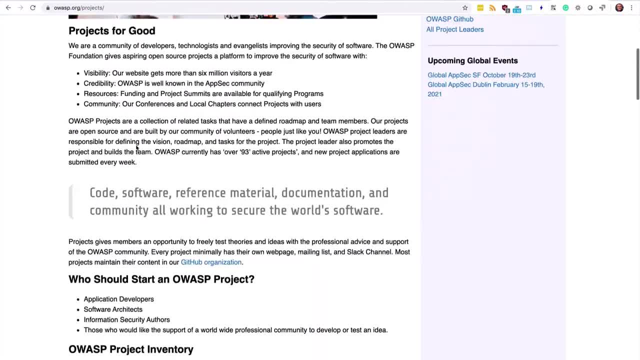 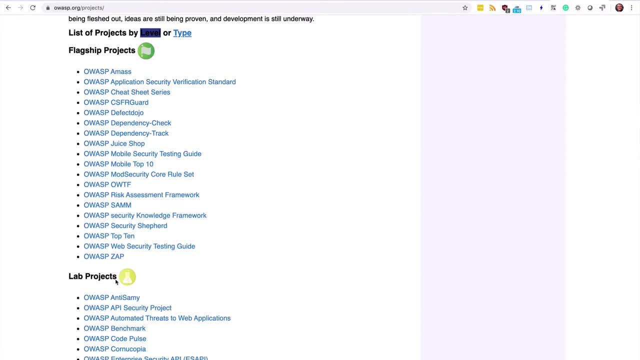 but let's focus on the flagship projects, And you can also scroll down and you'll see the section right here. So the flagship projects right now are labeled as green flags. They also have different lab projects, but if we focus on the flagship projects, 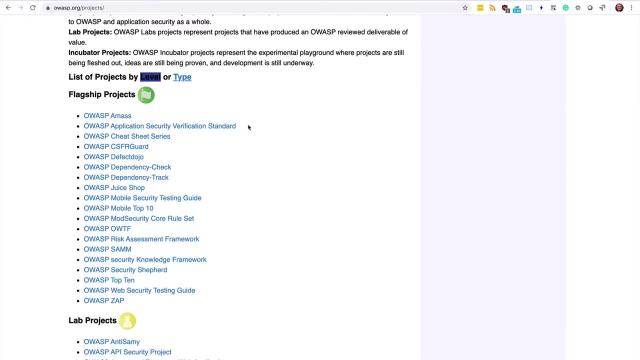 we will see multiple different types of projects, some of which we will explore in this course, For example, the Application Security Verification Standard. we'll look at some of the cheat sheet series. We'll also look at the Mobile Security Testing Guide, the OWASP Mobile Security Test Guide and the OWASP Mobile Security Test Guide. 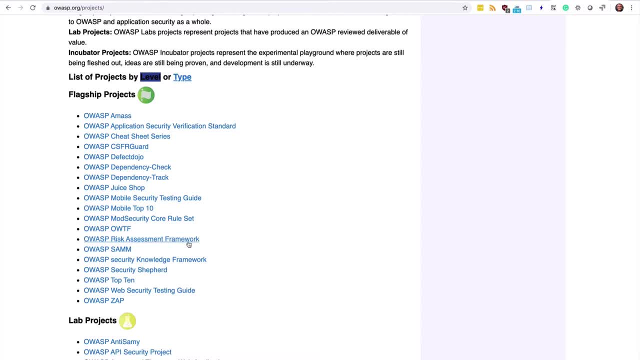 We'll look at the Risk Assessment Framework, the Security Knowledge Framework. We'll also look at the OWASP Web Top 10 and the Web Security Testing Guide. So these are some of the flagship projects that we'll take a look at, but feel free to also scroll through. 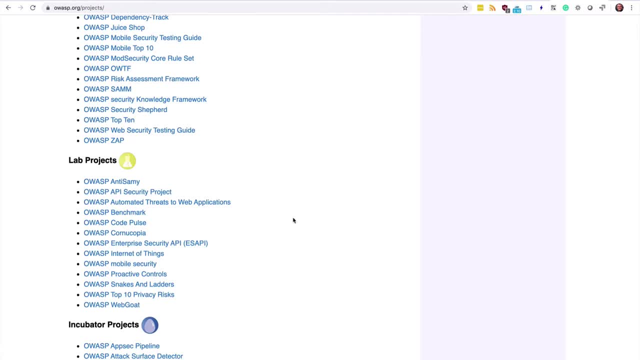 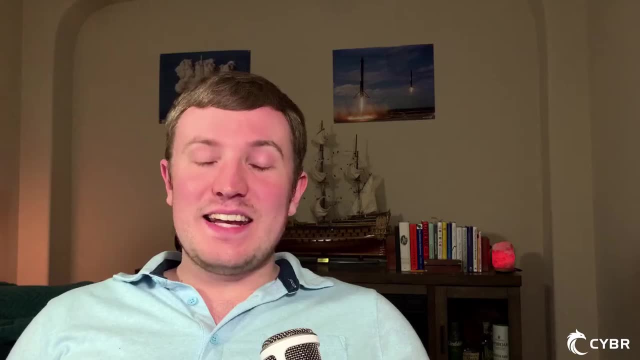 and look at some of their various projects, which can be extremely helpful, And, as you can see, this is a rich library that you can reference over and over again throughout your career. Now, I'm not gonna lie: looking at this list gets me pretty excited. 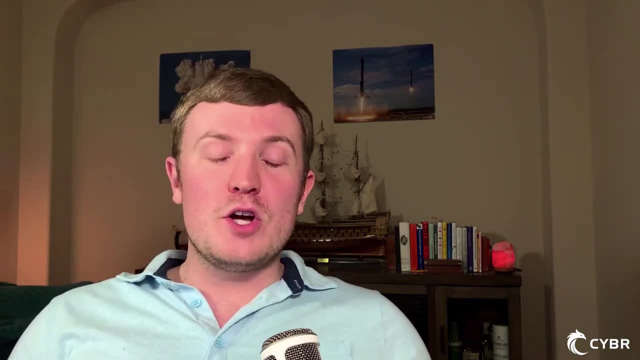 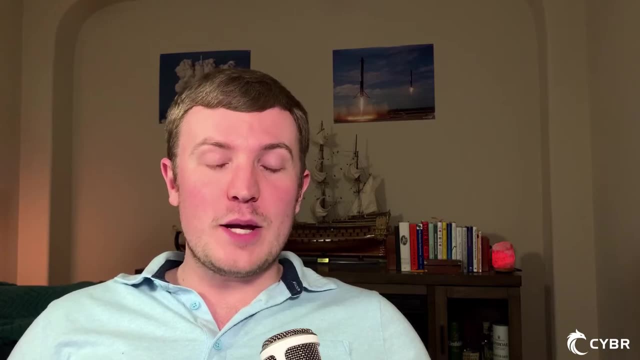 So I hope you feel the same way, because we are going to be spending time looking at these different projects. All right, go ahead and mark this lesson as complete and move on to the next, where we dive into critical concepts of application security To produce a secure application. 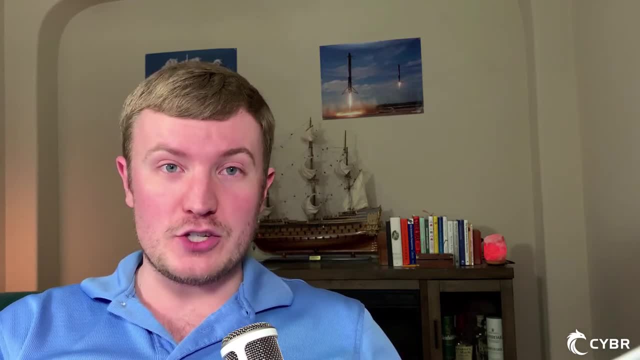 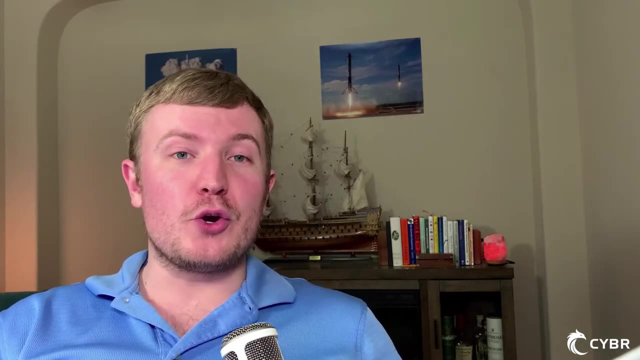 you have to first define what secure means for that application, because if you don't have this defined, then how can the team possibly know where to focus? And it's also much easier to build security from the ground up, baked into the application. 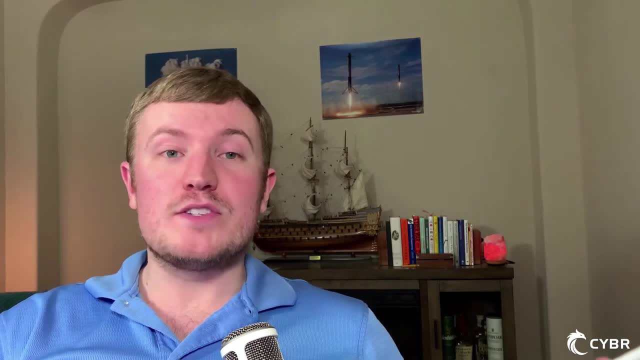 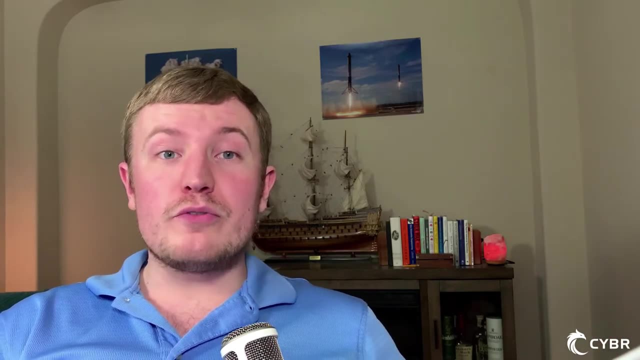 versus retrofitting that in an existing application. that was not built with security in mind, But of course, that's not always possible. Maybe you're inheriting an older application or you've got a set of APIs that are mature and that have drifted over time. 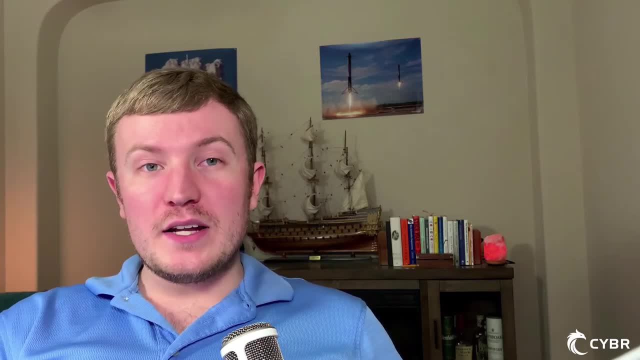 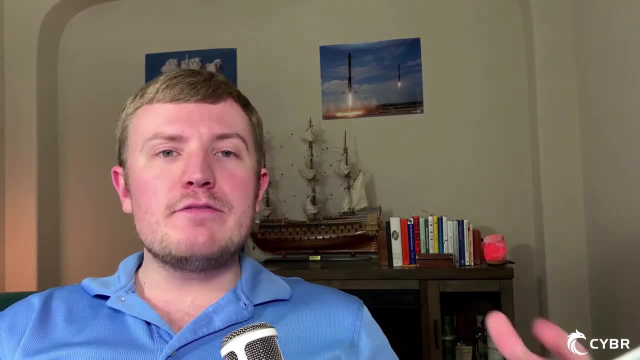 Regardless of the situation that you find yourself in, start with a baseline and then build on top of that. So that's exactly what we're going to do in this section of the course. We're going to start building that baseline, but even just building a baseline. 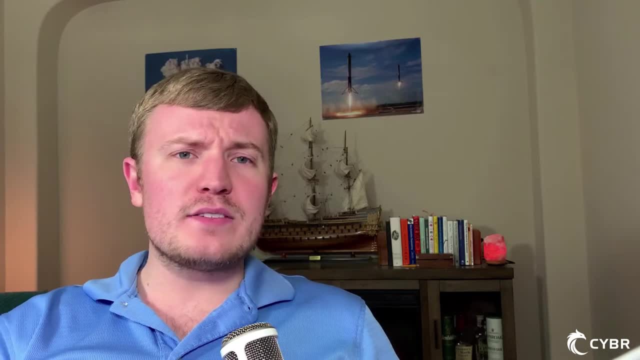 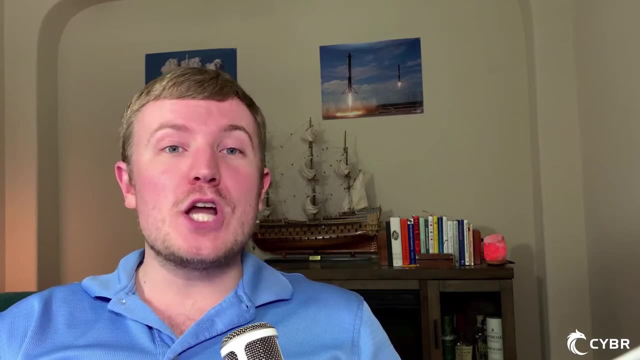 can seem like a very daunting task, because there are so many areas that we could focus on. And how do we know where to focus on first? Well, luckily for us, as we saw in the prior lessons, OWASP has a number of different projects. 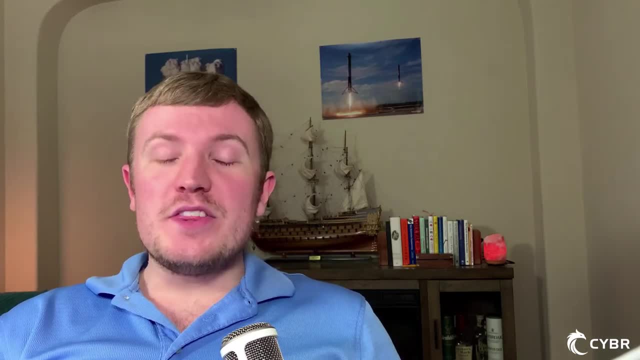 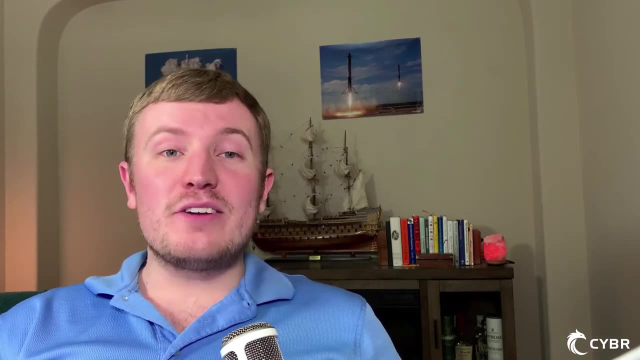 and some of those projects can help us with building that foundation. So in this lesson we're going to look at the OWASP Application Security Verification Standard- or ASVS for short, as a guide for setting our security requirements, baseline for our applications. 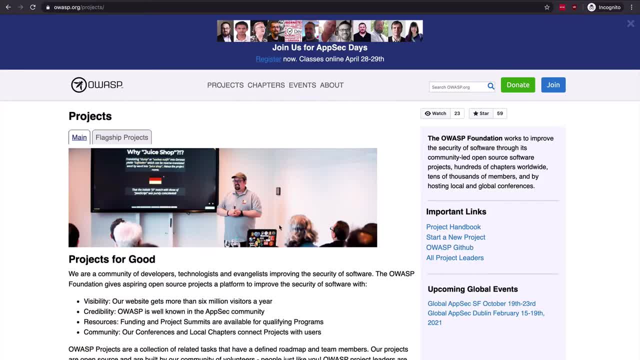 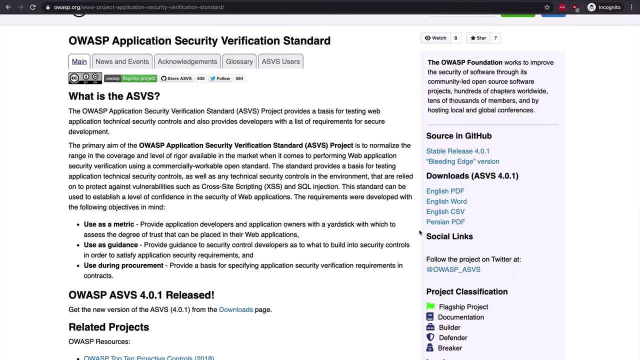 You can find this by going to projects and then browse all projects and scroll down until you see the OWASP Application Security Verification Standard, And on the right-hand side you'll find the different downloads. We've also got it pulled up here as a PDF link. 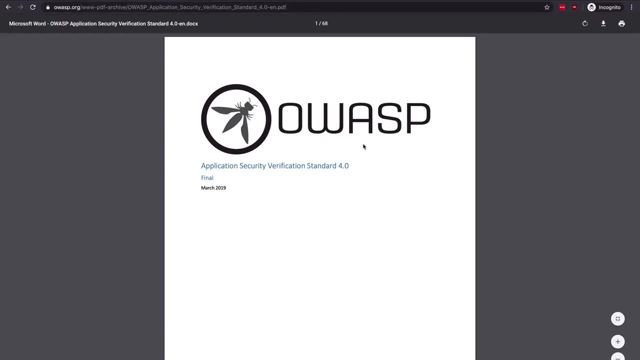 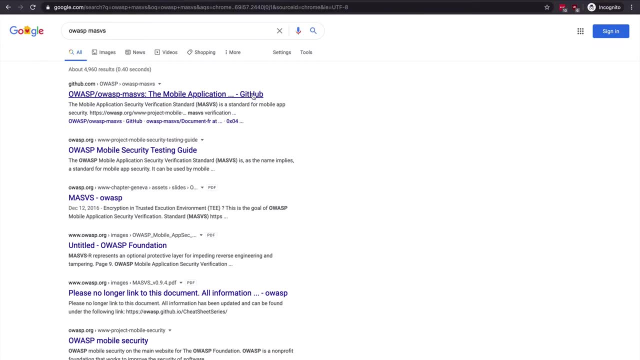 So if you go to this URL, you'll have the in-browser PDF version. As we go through this lesson, keep in mind that OWASP has separated standards for mobile application security. So, while this lesson is focusing more on web and cloud application security baselines, 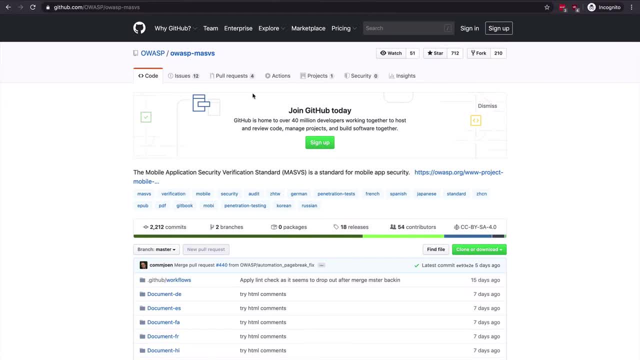 we will also look at the mobile application security verification standard in the mobile section of this course, And as we get familiar with these projects, it will be easier to look at mobile specific ones. So even if you're primarily interested in mobile application security, 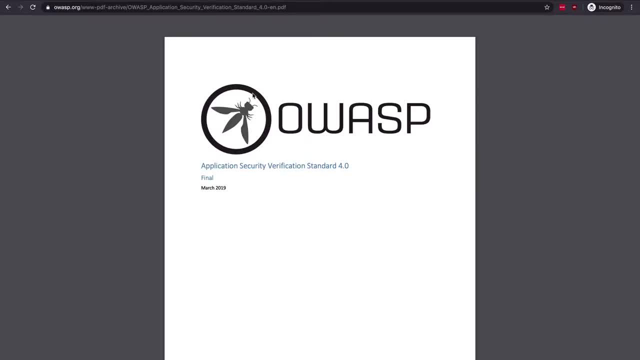 this lesson is still relevant Now. the Application Security Verification Standard, which I'll refer to as the ASVS from now on, is currently on version 4.0 from 2019, which is the latest version at the time of this recording in 2020.. 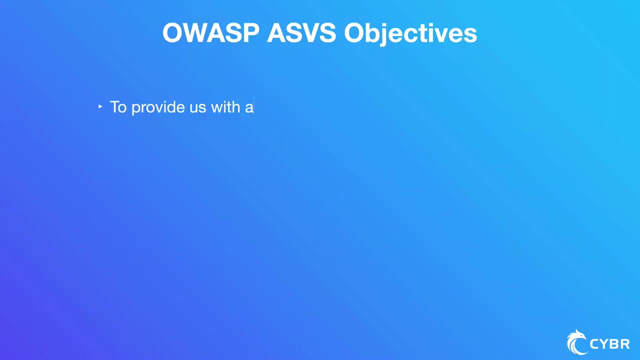 And it has these objectives: To provide us with a measurement on how much trust we can place in our web application security. to provide guidance as to what we should build into our security controls to satisfy security requirements. and to provide a standard for application security verification requirements. 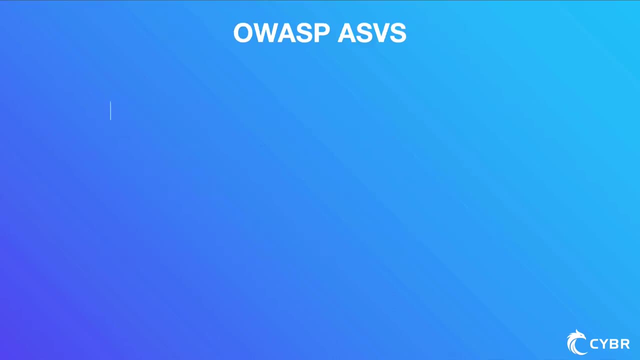 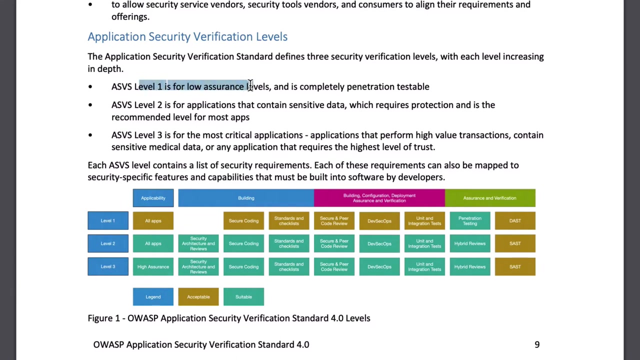 in contracts with third parties. So essentially, the ASVS is a catalog of security requirements and the verification criteria that we can use for all of our projects, And it does that with three different verification levels. ASV level one is for low assurance levels. 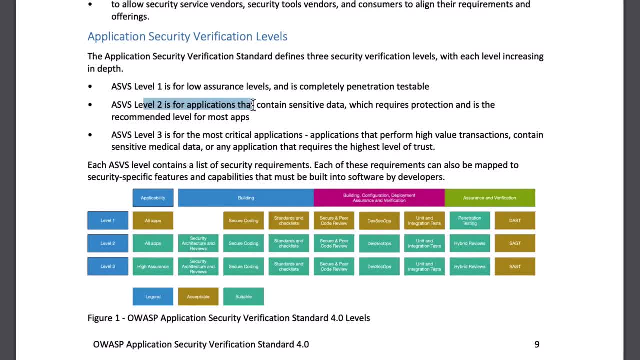 ASV level two is for applications that contain sensitive data and is the recommended level of security. ASV level three is the recommended level for most applications, And then ASVS level three is for the most critical of applications. Each level has a list of security requirements. 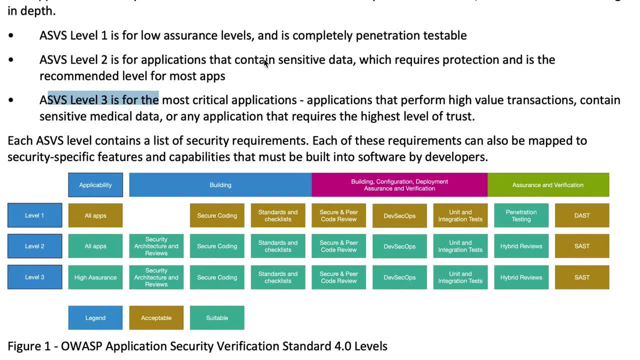 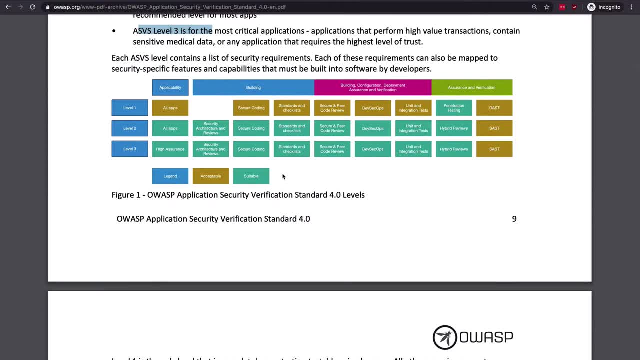 defined by this standard and this is what it looks like. Now this will make more sense as we look at the actual requirements, but using these requirements and levels, we can start to create our own secure coding checklist specific to our application. Now, if we determine that our API or application 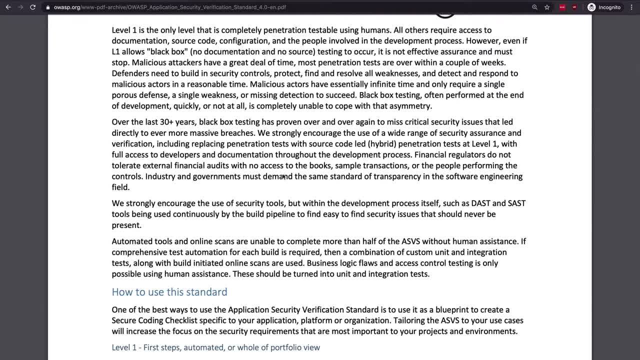 is at a level one because it doesn't contain or touch any sensitive data whatsoever, and that it can get by with the absolute bare minimum, then we will approach it differently than if we deem it to be a level two or level three. Level one is also useful as a first step. 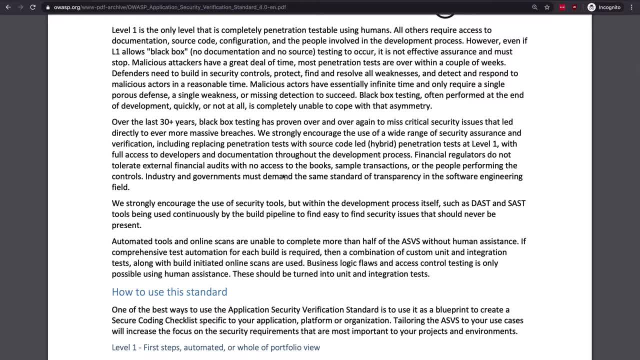 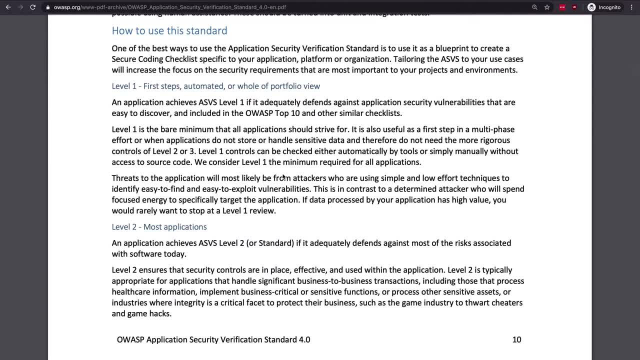 and a multi-phase approach, so it can act as a good starting point, but in a lot of cases it should not be your endpoint. Now. the ASVS summarizes level one as having security controls that can be checked automatically by tools or manually, without accessing the source code. 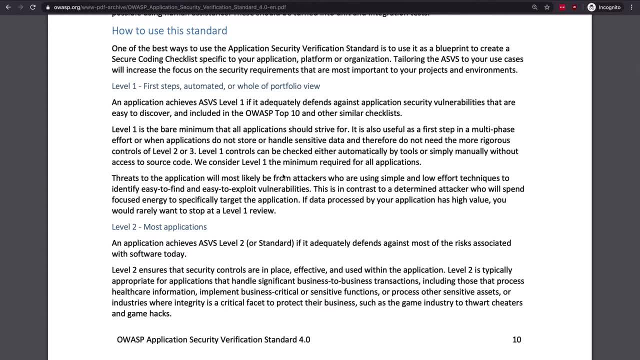 These security measures can thwart the most basic attacks who use simple and low effort techniques to identify, easy to find and easy to exploit vulnerabilities, but they will fall apart with the most determined attackers and more sophisticated attacks. Now the ASVS deems level one to be the absolute minimum. 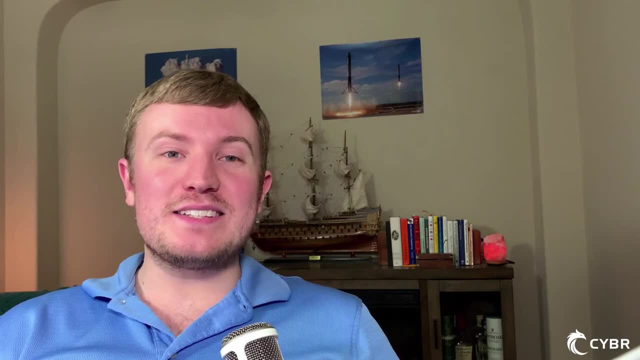 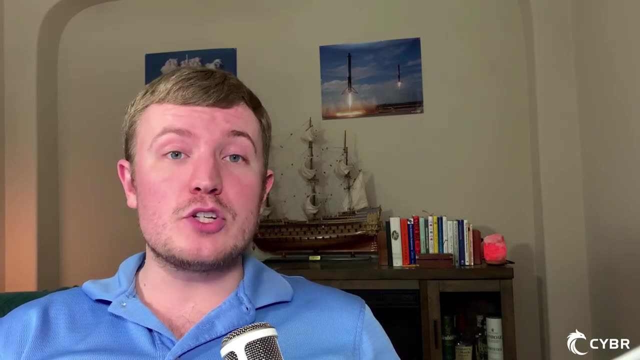 that all applications should strive for. The unfortunate reality is that many applications that are in production right now don't even meet level one requirements. So if you find yourself in that situation, that's fine. Just aim for level one, even if you need to be at level two or even level three. 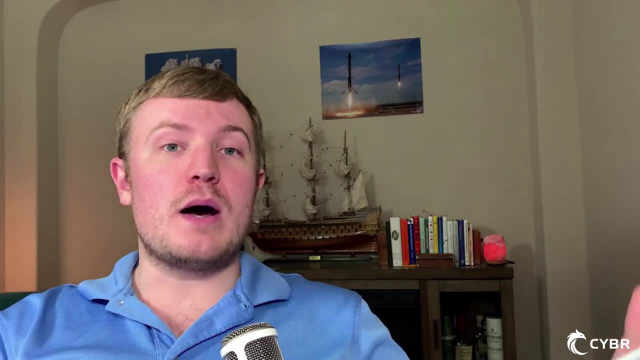 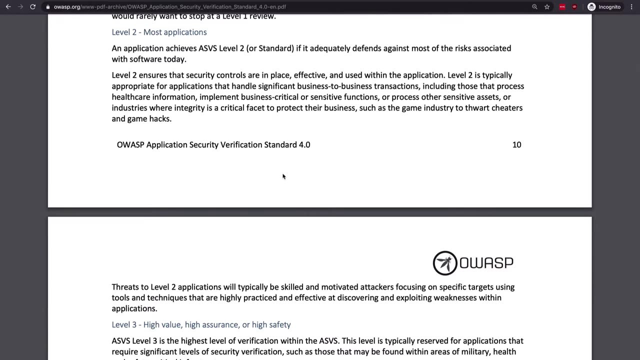 potentially start with level one and then iterate on top of that to get to the other levels. Level two aims to defend against most of the risks associated with software today. This is a level that many businesses should aim to have, especially to protect their business critical areas. 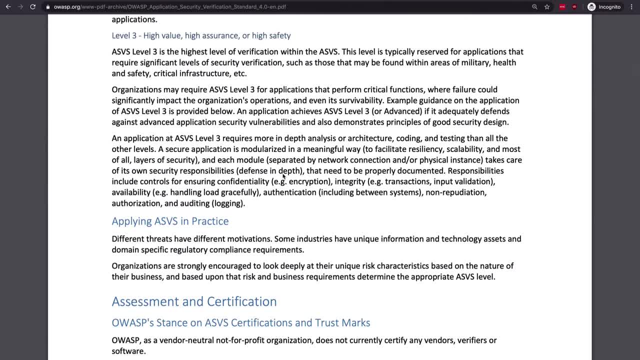 Level three is the highest level defined by the standard, and it requires in-depth analysis of architecture and code and in-depth testing that goes far beyond the automated tools or online scans. This is a level that you should attain if a successful attack would significantly impact your organization's operations or even its survival. 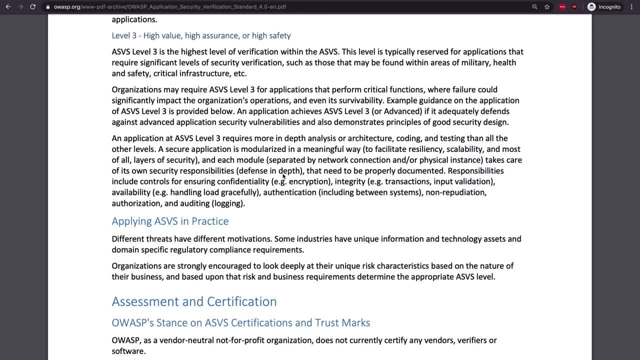 Now, this level, of course, requires much more investment, which is why the standard labels level two as the recommended level for most applications. But, at the end of the day, you're the expert in regards to your applications, So it is up to you to determine which level fits your needs. 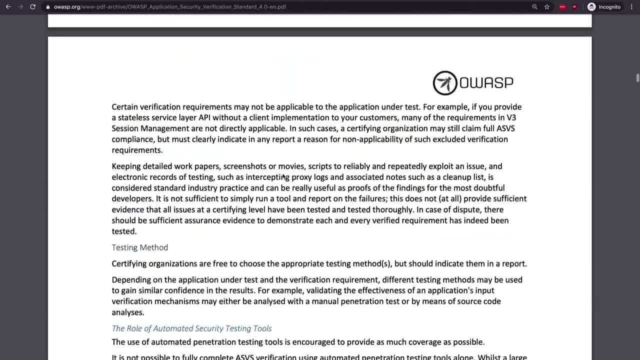 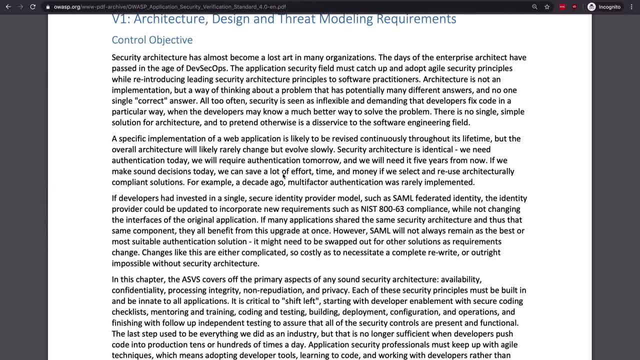 Let's get started. Let's get started. Let's get started. Since the list of categories and requirements is quite lengthy, we won't have time to explore all of them, but let's take a look at a few examples so that we can get the hang of it. 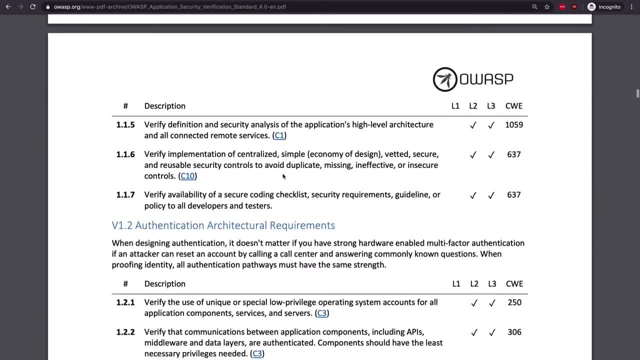 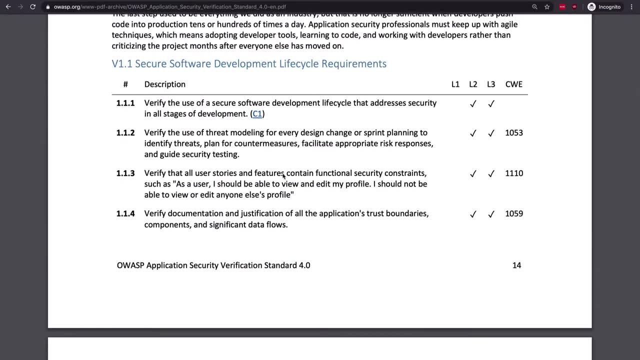 The ASVS contains categories such as authentication, access control, error handling and logging, web services and others. Each category contains a collection of requirements that represent the best practices for that category and they are written to be verifiable statements, For example with V1.1.0,. 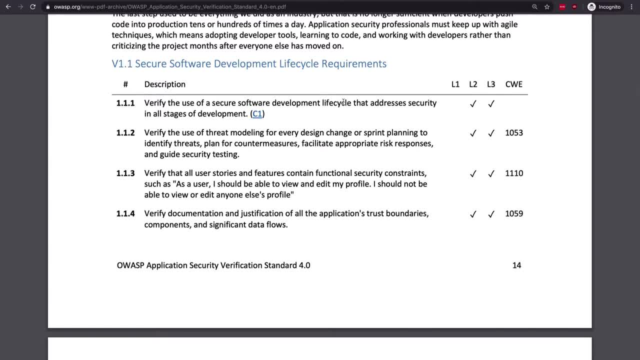 point one, which is to verify the use of a secure software development lifecycle that addresses security in all stages of development. For level one, it is not a requirement, but for levels two and three it is a requirement. So in this case, since we're verifying this statement, it's either: 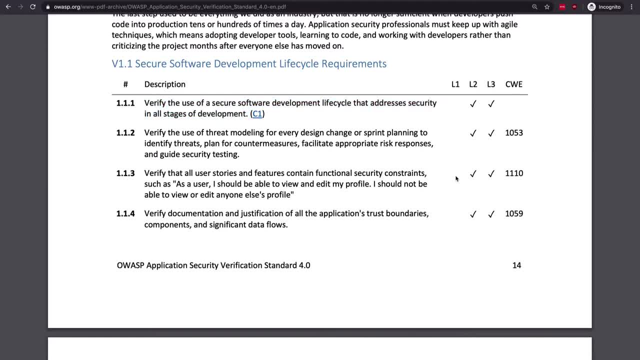 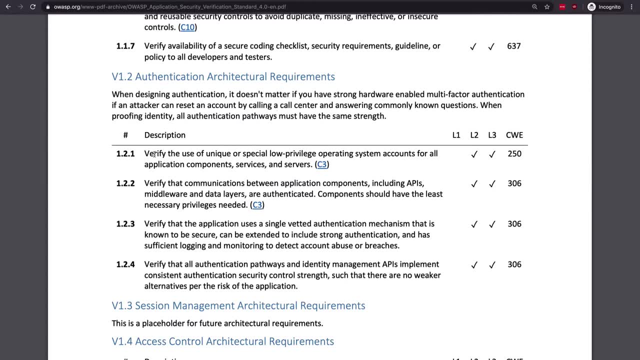 a yes or no. If yes, check it. If no, don't check it. If we go down to V1.2,, which is about authentication, architectural requirements, and we look at V1.2.1,, which is to verify the use, 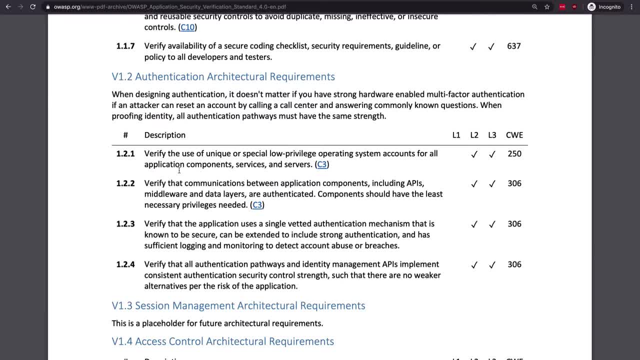 of unique or special low privilege operating system accounts for all application components, services and servers- Again, not a requirement for level one, but it is a requirement for level two and level three, And so you can get the idea. Now, obviously, there's a whole lot more to the 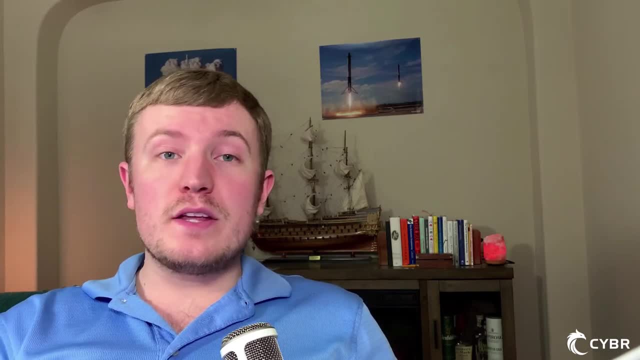 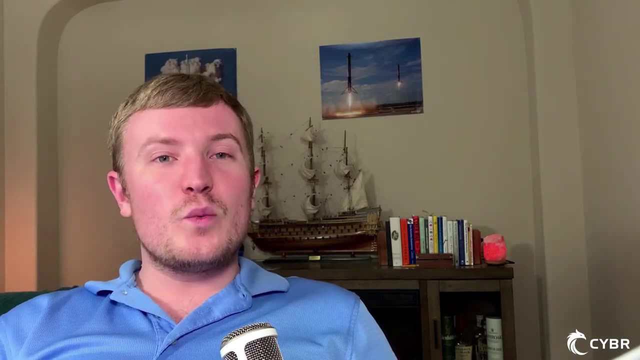 ASVS than we have time to cover in this lesson. So after marking this lesson as complete, please spend a little bit more time reviewing the requirements and getting more familiar with those requirements. In the next lesson we're going to explore another framework called OWASP SAM. 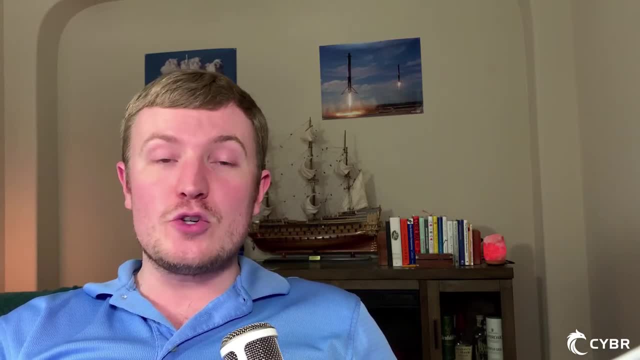 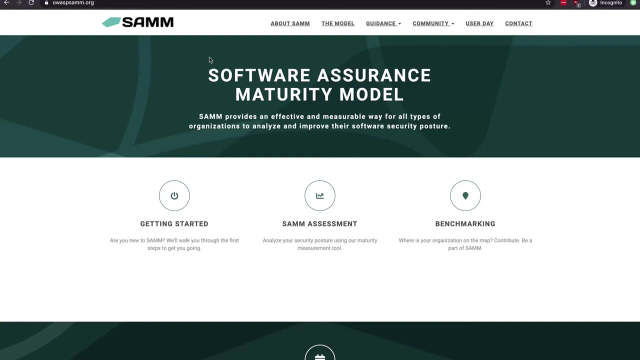 or Software Assurance Maturity Model, which was donated to and is now maintained by, OWASP. So go ahead and mark this lesson as complete and I'll see you in the next one. SAM stands for Software Assurance Maturity Model, and it's a model that helps understand the core building blocks of a secure software program. 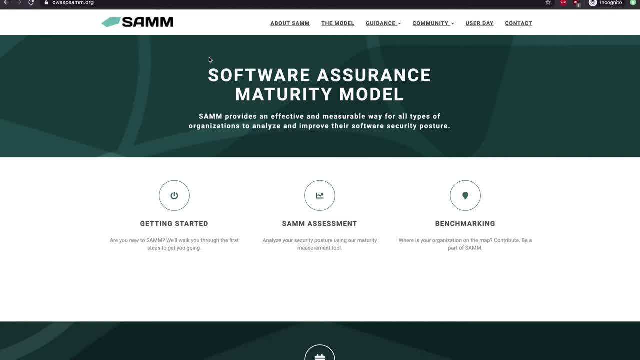 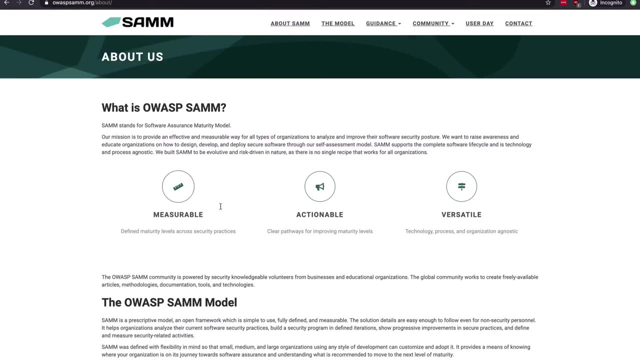 from a more macro point of view, It provides a self-assessment model for all types of organizations to use, whether you're large or small. It is technology and process agnostic and it supports the complete software lifecycle. It has three main characteristics: It is measurable, with defined maturity levels. 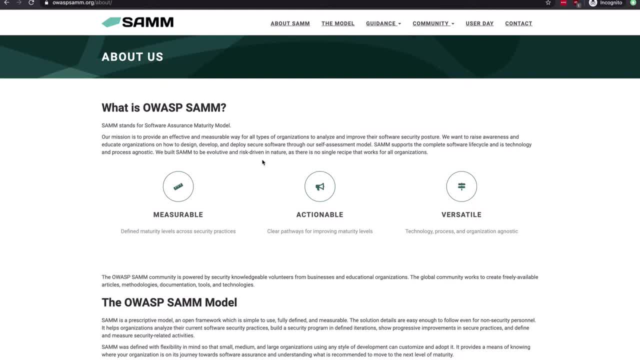 similar to the levels that we saw in the ASVS from the prior lessons. It is actionable, with clear paths for improving those maturity levels, And it is versatile by being technology, process and organization agnostic. This makes SAM a great tool to help analyze your organization's 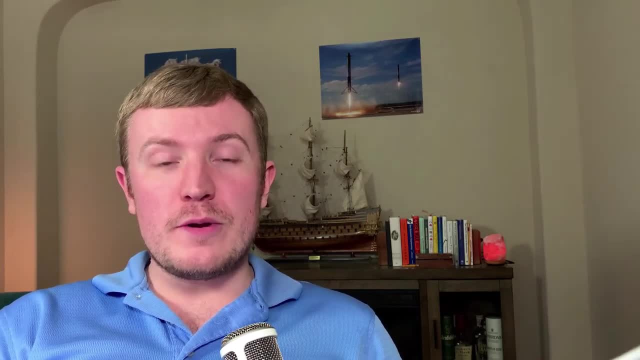 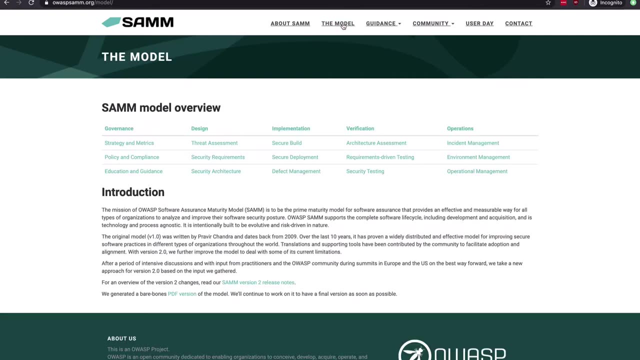 current security stance, so that you can define iterations to improve and then show progress towards those iterations with actual measurements. So let's take a look at how SAM is structured, And we're going to do this with a few different ways. The first way is by accessing it from the website, by going to the model And you can see. 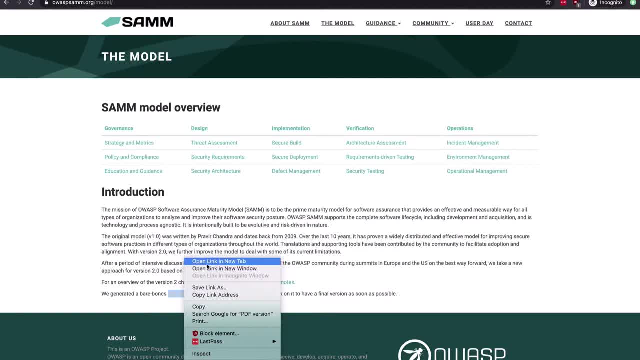 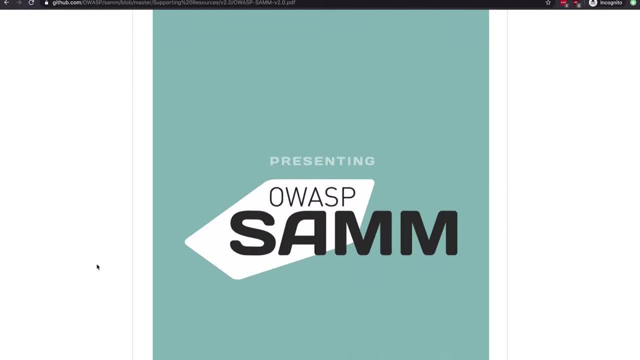 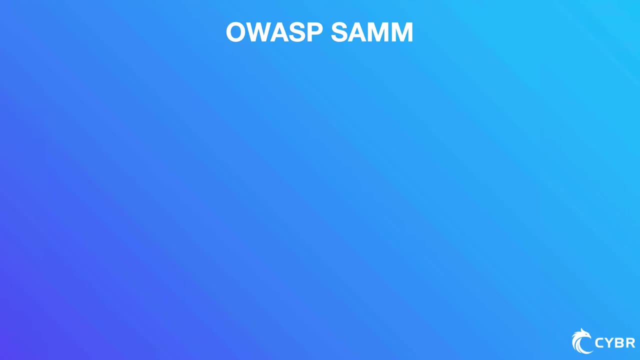 it here. They also have a PDF version. so this is the second way, And you can download or view the PDF from GitHub, And I've also tried to make it more legible. so let's take a look at that with the third way. At the highest level, SAM defines five critical business functions And those 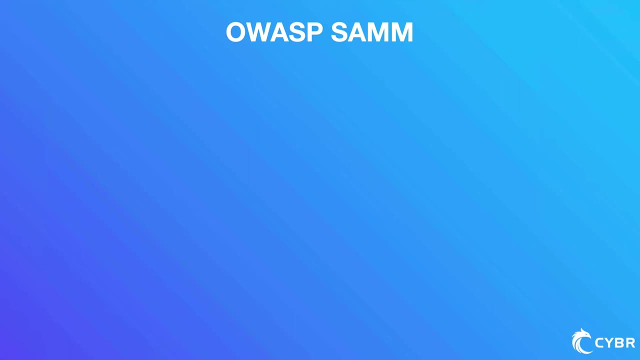 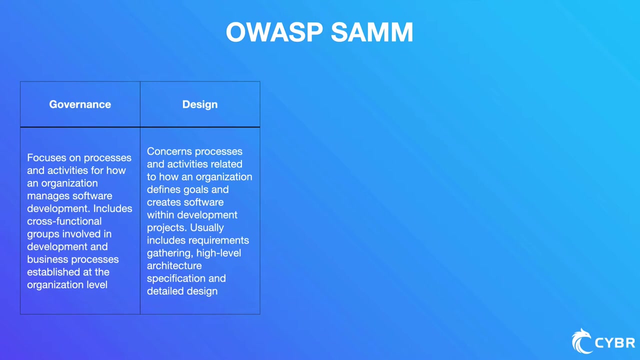 business functions are categories of activity related to software development. The first one is governance, And governance focuses on processes and activities for how an organization manages software development. It includes cross-functional groups involved in development and business processes established at the organizational level. The second one is design, which concerns processes and activities related to how an 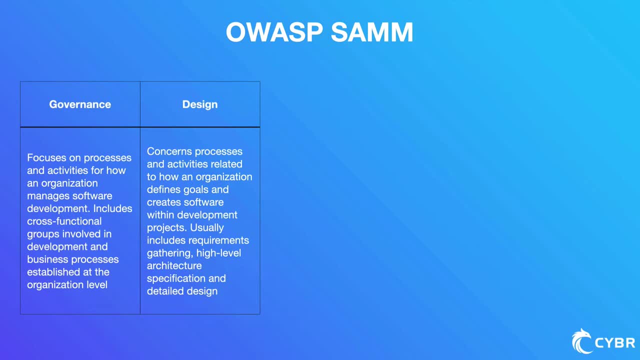 organization defines goals and creates software within development projects, And this usually includes requirements gathering, high-level architecture and design. And the second one is implementation, which is focused on processes and activities related to how an organization builds and deploys software components and its related defects, And the goal here is to ship reliably. 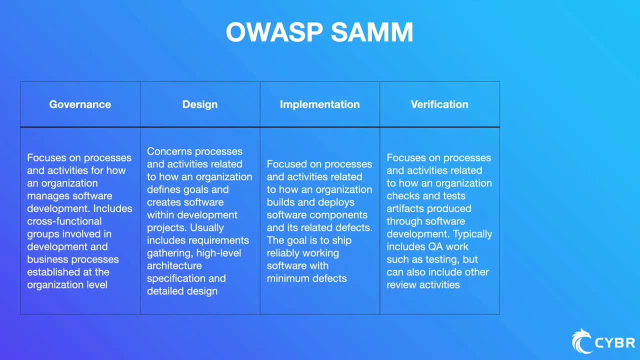 working software with minimum defects. Then we have verification, of course, which is the focus on processes and activities related to how the organization checks and tests the artifacts that we've produced through software development. This typically includes QA, which is the process that we use to do QA work, such as testing, but it can also include other review activities. 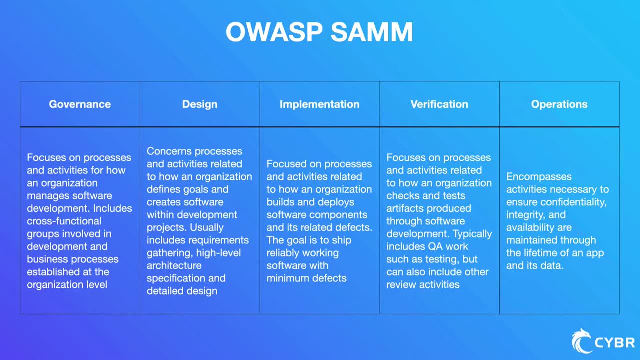 And then, finally, we have the operations, which encompasses activities that are necessary to ensure the confidentiality, integrity and availability are maintained through the lifetime of an application and all of its data. Now, for each of these business functions, SAM defines three security practices each, So there are 15 security practices in total. 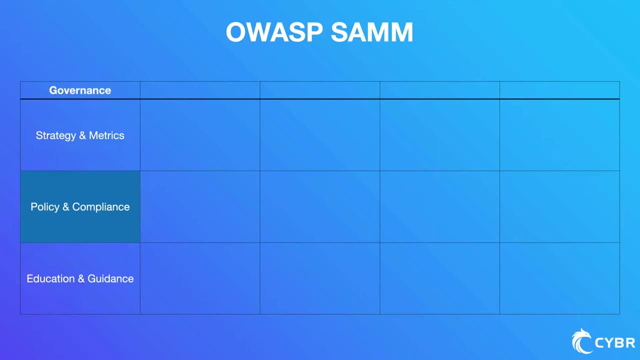 that are independent silos for improvement and that all map back to the five business functions of software development that we just looked at. So for governance, the security practices are strategy and metrics, which forms the basis of your secure software activities by building an overall plan. There are policy and compliance. 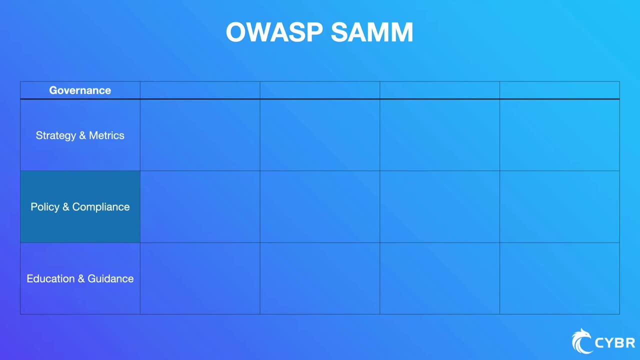 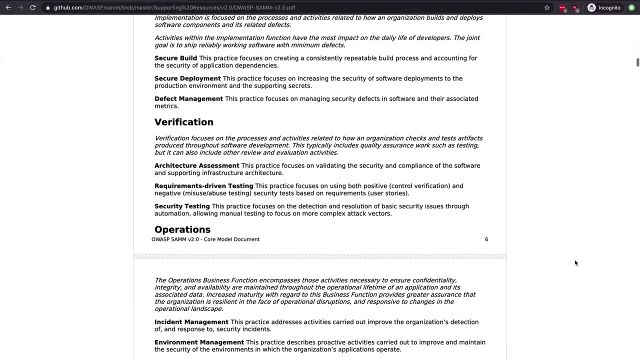 which drives the adherence to internal and external standards and regulations. and then education and guidance, which focuses on increasing the knowledge in the organization regarding secure software, just like we're doing right now. Now, keep in mind that I am pulling these descriptions and this chart data from the PDF and the website, So, if you're following along, 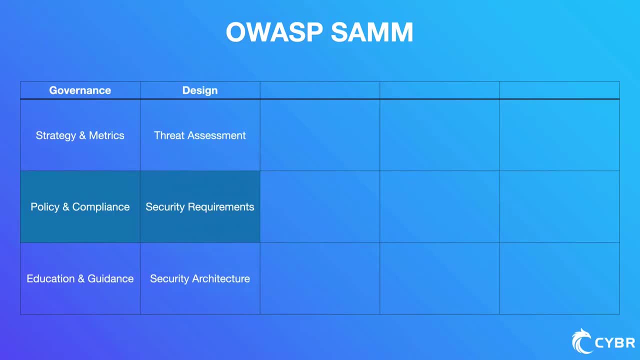 you can absolutely do that. Then, for design, our security practices are threat assessments, which focus on identifying potential threats in applications. Then we have security requirements, which focuses on defining appropriate security requirements for your software and your software suppliers, And then we have security architecture, which focuses on managing architectural risks. for 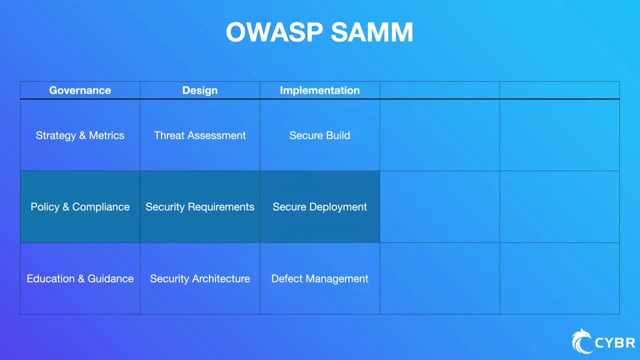 the software solution For implementation. we have security architecture, which focuses on managing architectural risks for the software solution For implementation. we have security architecture, which focuses on managing architectural risks for the software solution For implementation. we have secure build, which is creating a consistently repeatable build process. 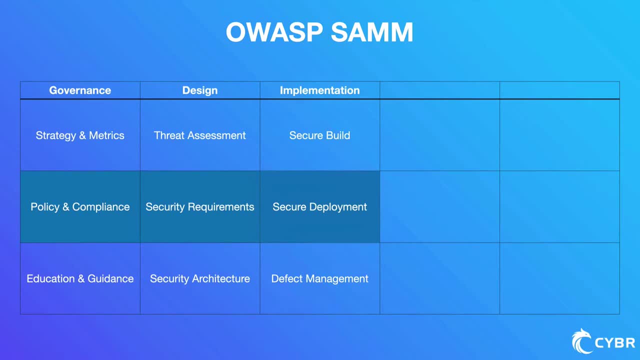 and accounting for the security of application dependencies. We have secure deployment, which is all about increasing the security of software deployments to the production environment and the supporting secrets. And then we have defect management, which is managing security defects in the software and the associated metrics For verification. 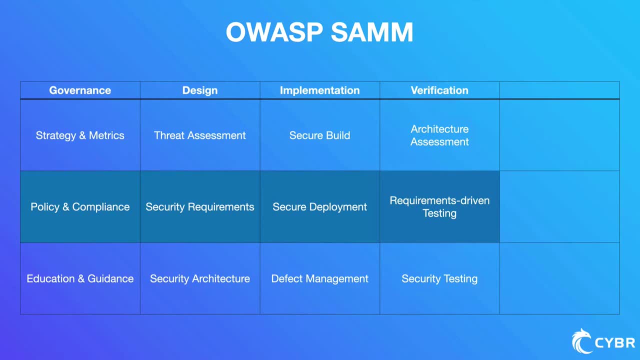 we have architecture assessment, which is validating the security and the compliance of the software and the supporting infrastructure architecture. We have requirements driven testing, using both positive- ie control verification- and negative, like misuse and abuse testing, or security tests based on requirements like user stories And, if you're. 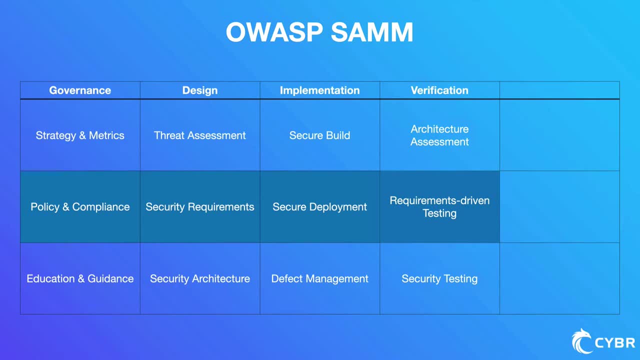 not familiar with that. we will look at this a little bit more in the future. And then, finally, we have security testing, which is detection and resolution of basic security issues through automation and allowing manual testing to focus on the more complex attack vectors. 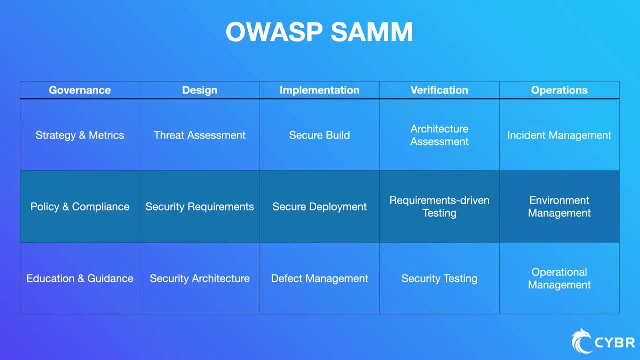 Finally, for operations, we have incident management, which addresses activities carried out to improve the organization's detection of and the response to security incidents. We have environment management, which describes proactive activities carried out to improve and maintain the security of the environments in which the organization's applications operate. 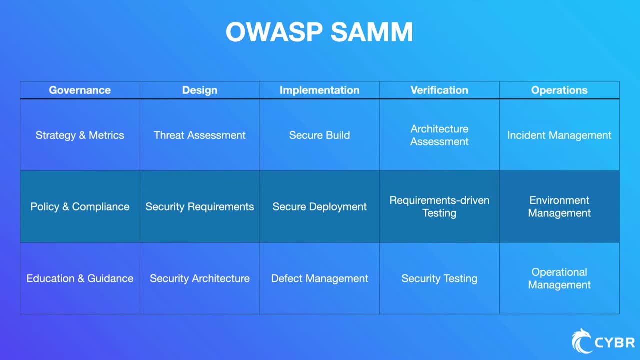 And then operational management, which focuses on operational support activities that are required to maintain the security throughout the product life cycle. So go ahead and take a look at this Now. for each of these security practices that we're looking at right here, SAM defines three different maturity levels as objectives, And the three maturity levels are more. 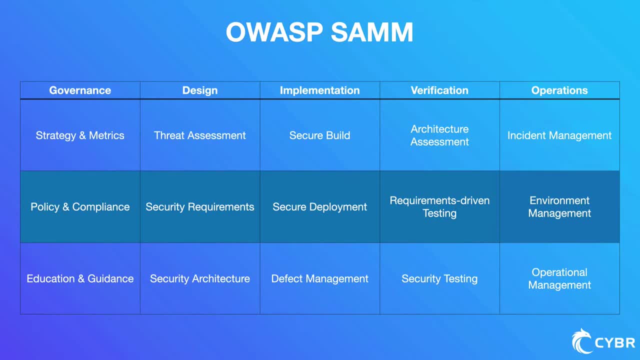 sophisticated to implement than the prior one, So level one is easiest. Level three is more sophisticated And so, as a result, they also have more stringent success metrics, And we saw varying levels of maturity in the ASVS. So this is not a new concept. 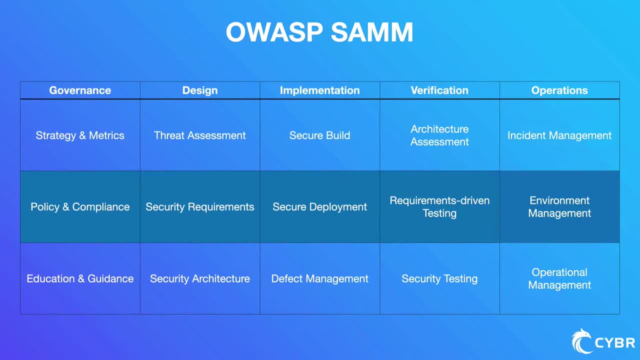 but an organization does not have to meet all of the maturity levels, since they may not all be relevant to the organization, And so you may choose to prioritize some over others. So it's important to keep that in mind and not feel overwhelmed when trying to implement this. 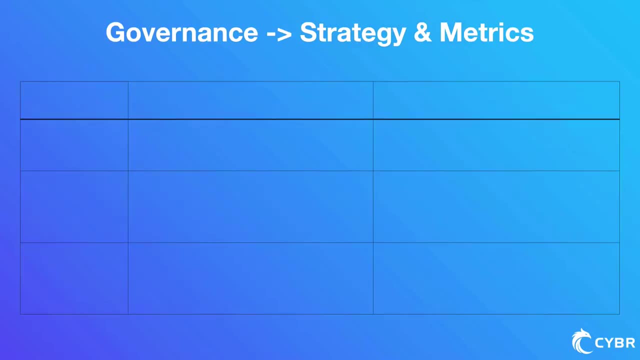 But so for each of these security practices we have the different maturity levels, but we also have two different streams, And we haven't seen this before. Streams have objectives to be reached and those objectives are tied to the different levels, So they also increase in. 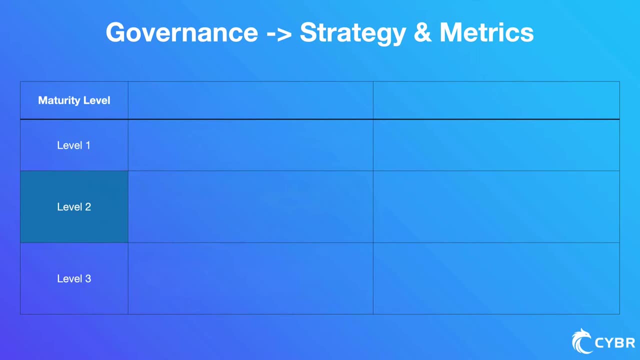 complexity. For example, if we look at the strategy and metric security practice, there are two different streams. Stream A is to create and promote, And level one aims to identify organization drivers as they move forward in the process. So, for example, if we look at the 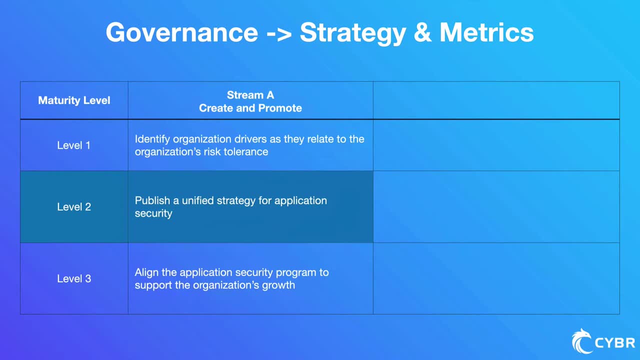 strategy and metric security practice. they relate to the organization's risk tolerance, Whereas level two is to publish a unified strategy for application security And level three is to align the application security program to support the organization's growth. But then for stream B we have measure and improve, And level one defines metrics with insight into. 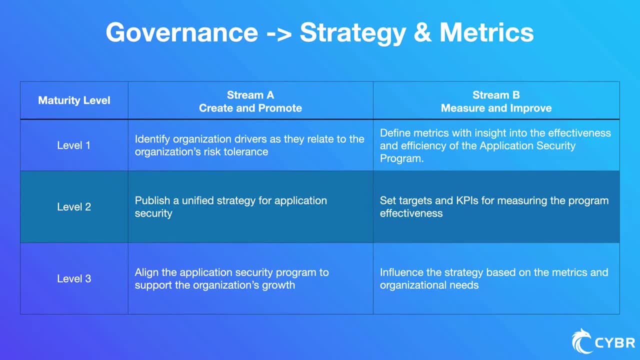 the effectiveness and efficiency of the application security program, Whereas level two sets targets and KPIs for measuring the program's effectiveness. And finally, level three is to influence the strategy based on the metrics and organizational needs. So, obviously, level three takes more time and is more sophisticated to implement, But, as you can see, that's a really 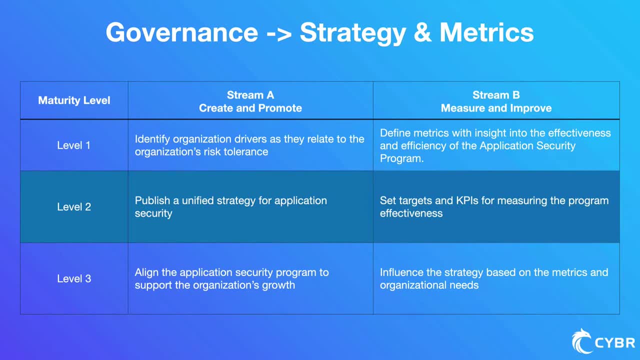 good goal to strive towards. So you can start with level one, then build on top of that to level two and then build on top of that to level three. But again, not all of these may be relevant to your organization, So keep that in mind. So Sam breaks down all of this into even more detail. 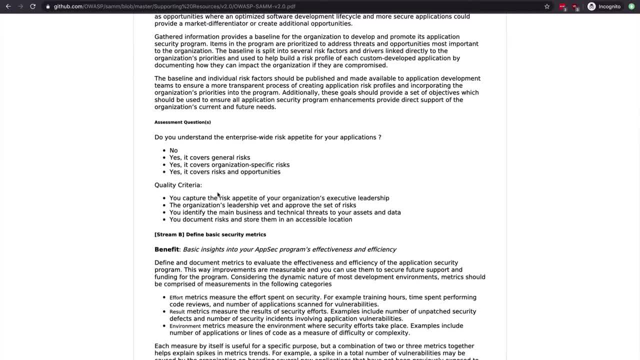 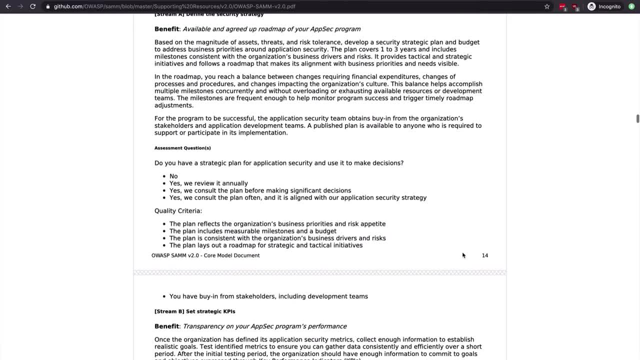 including assessment questions and quality criteria to measure the progress and whether objectives have been met or not. So instead of just looking at this theory, you can incrementally build towards that and you can show that to the rest of your organization, to your leadership and so on. 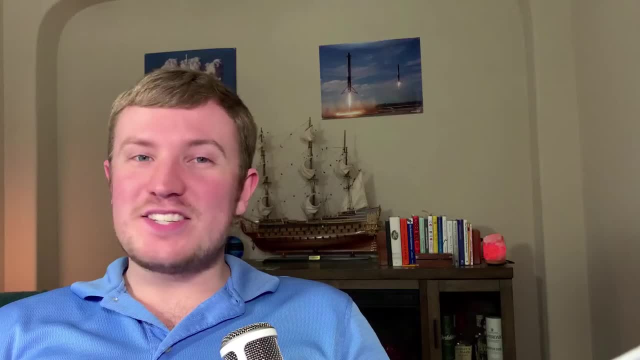 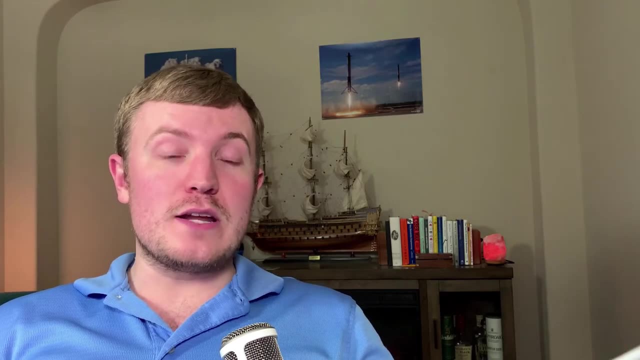 So this is a very effective and helpful framework. This is another lengthy document with a lot to chew on, So go ahead and take the time after completing this lesson to read through this document in a little bit more detail. Once you've got the hang of it, go ahead and move on to the next lesson, where we explore the top 10. 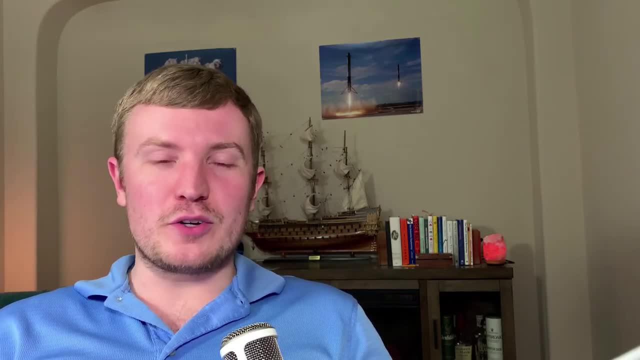 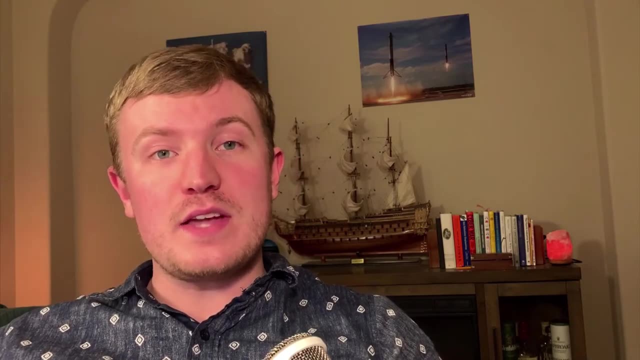 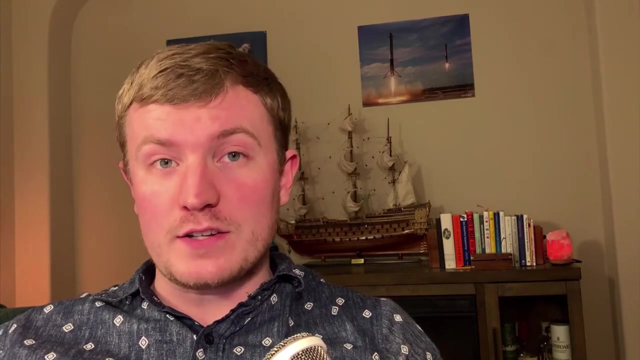 proactive controls that should be included in every single software development project. Now that we've looked at how to create a baseline for our applications with the ASVS and SAM, it's time to talk about the practical approaches to implementing some of the most important security requirements in our projects, Because all of the knowledge in the world 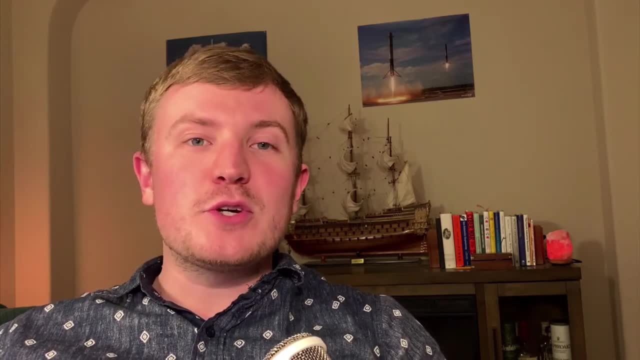 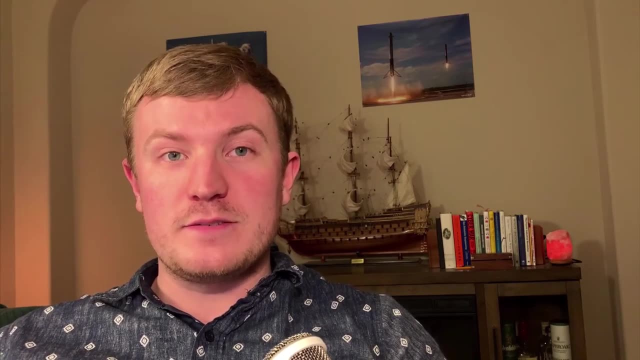 won't help if we can't apply it. So to help with this, let's look at the OWASP proactive controls, which is a list of security techniques that should be included in every software development project. The OWASP top 10 proactive controls can be found at this URL. You can also find it by going through: 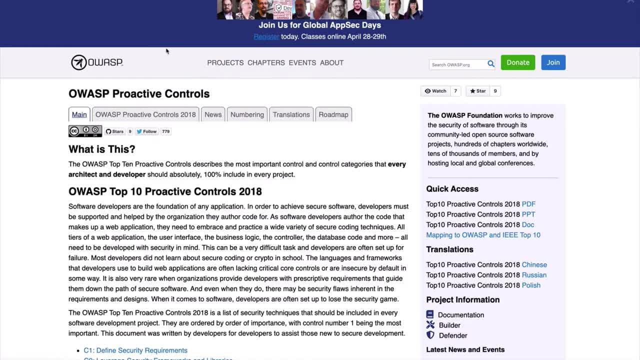 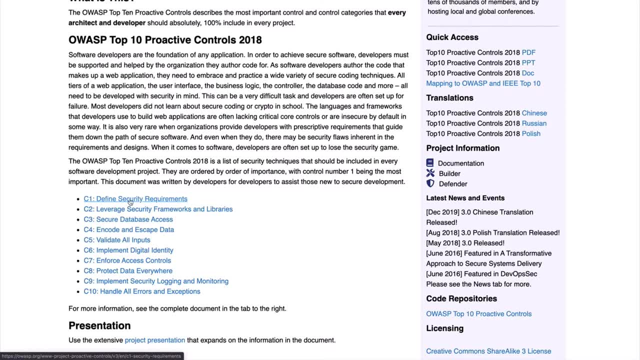 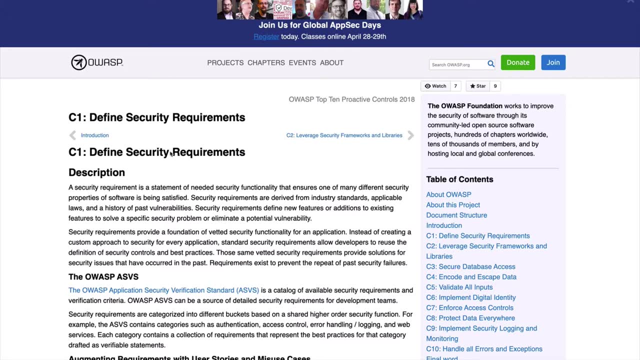 projects. browse all projects and look for proactive controls. This list is ordered in terms of importance, So we'll start from the very top with C1, defining security requirements. You may remember in the application security verification standard that some of the requirements had links with a C and a number like C1 for V1.1.1.. 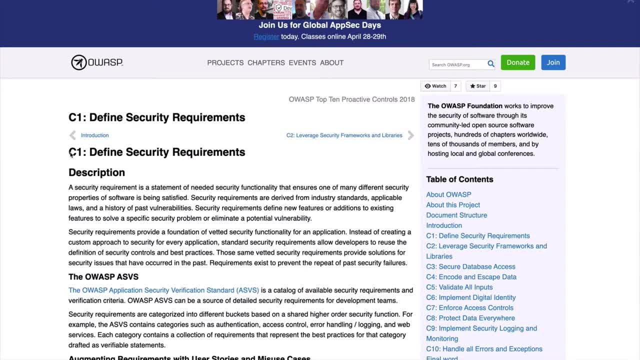 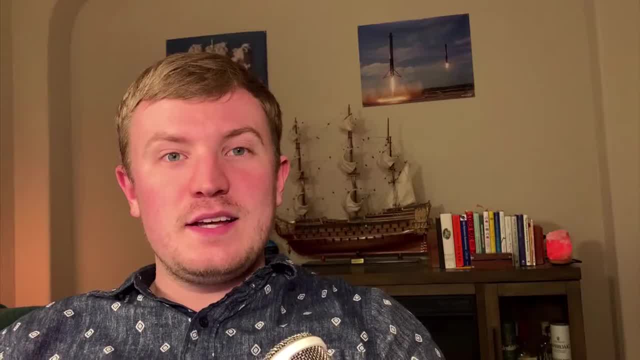 These map back directly to these proactive controls. So C1 maps back to defining security requirements, And so now we can start to see how these are all tied to work together. This control explains how to grab the requirements that we've seen in prior lessons. 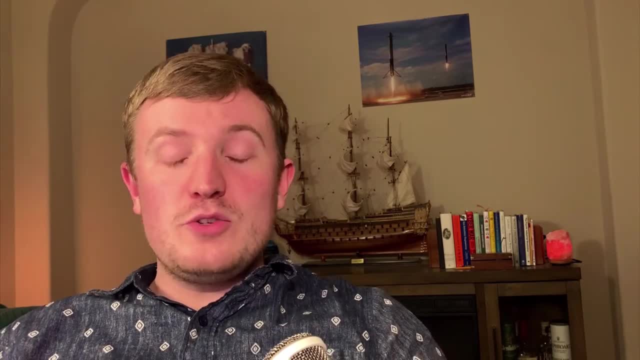 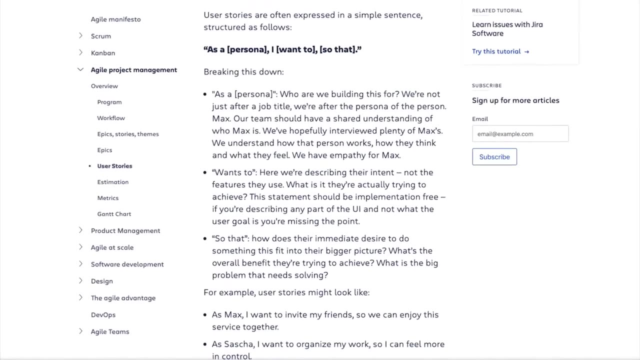 and to turn them into user stories and misuse cases. User stories, as long as you've been programming, for a couple of years at least- should not be a new concept. It takes the perspective of a user or even administrator, and it describes the functionality of what a user wants the system to. 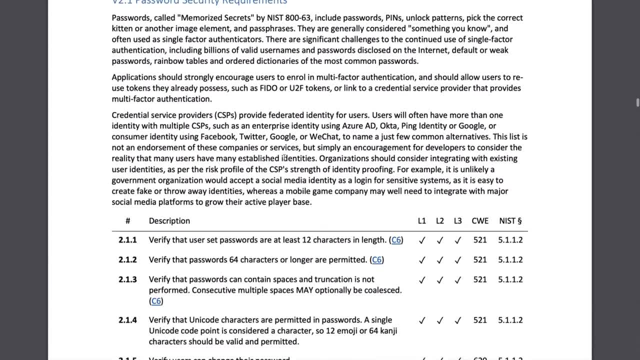 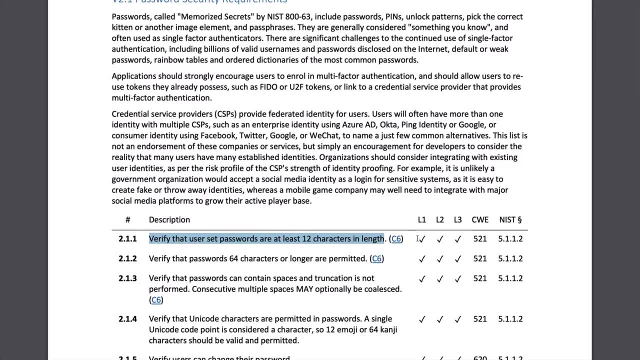 do for them. For example, if we look at V2.1.1,, which is to verify that user set passwords are at least 12 characters in length and this is a requirement for level 1s through 3, user stories. 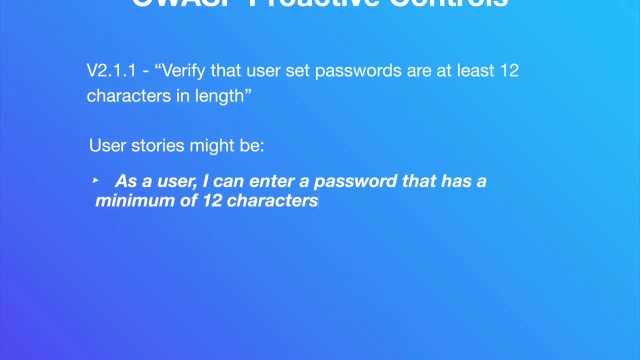 might be as a user. I can enter a password that has a minimum of 12 characters, And another one might be as a user. I can enter my username and password to gain access to the application, While a misuse case is a story focused on the attacker and their actions. So it might look like. 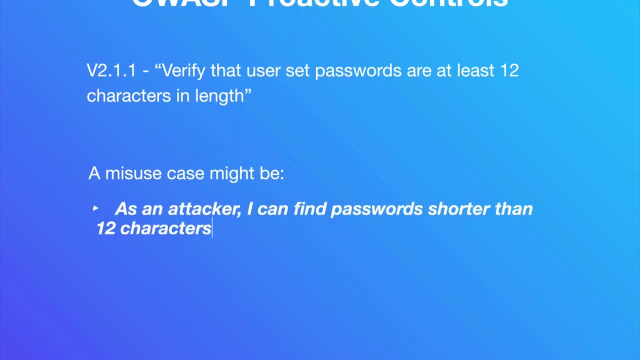 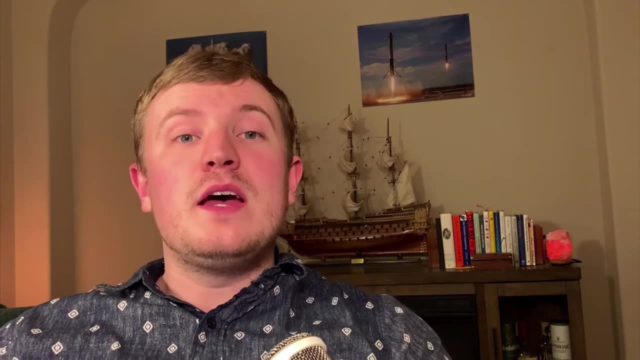 this. As an attacker, I can find passwords shorter than 12 characters. Breaking down those ASVS requirements into misuse cases or user stories helps make them more testable for us and for our teams. Now, at this point, you might look at me and you might say: 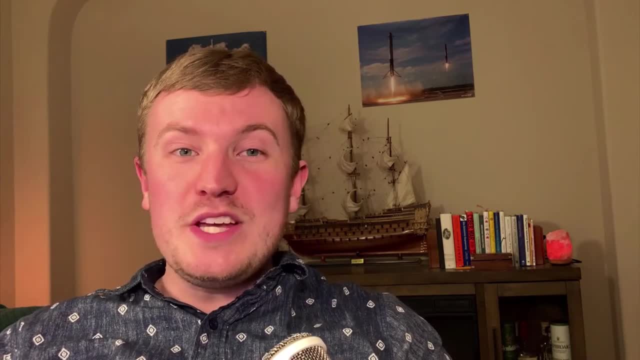 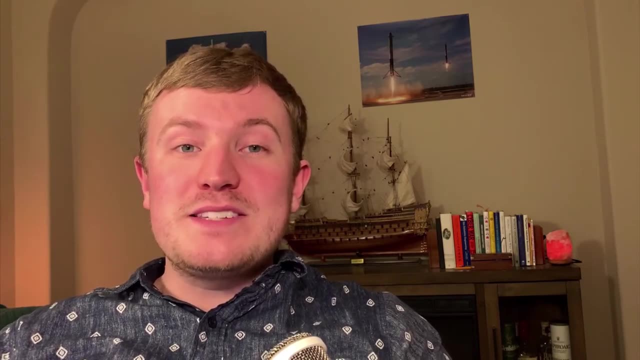 hey, Christoph, that's great, but it's literally going to take us weeks or even months to break all of this down into different user stories and misuse cases. But luckily OWASP is a step ahead of us because they've outlined four steps to implement the ASVS requirements. First, 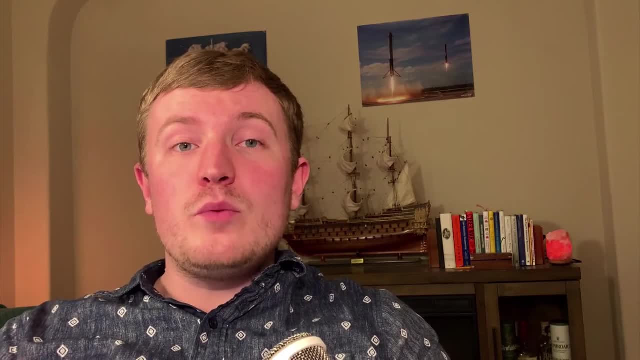 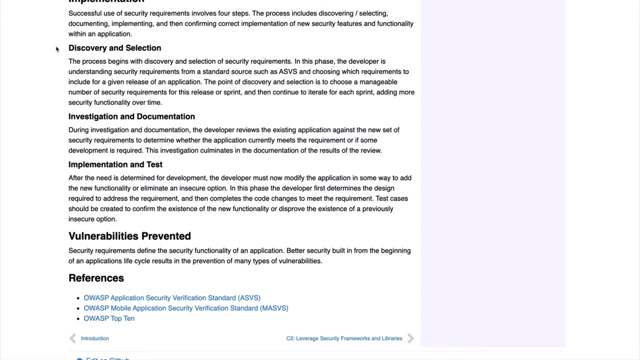 we talk about the step several times in the process. As we talk about these steps, think about how they will fit in your existing or even future development lifecycle. Step number one is discovery and selection. Now, you're not meant to tackle all of it at. 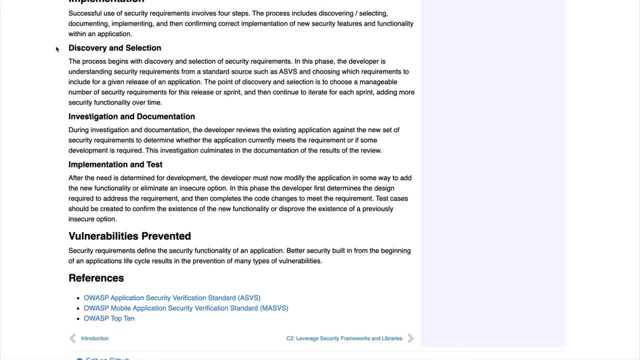 one time. Instead, look through the list of requirements from the ASVS and or any other custom requirements that you've deemed necessary for your application and prioritize those, Break them down into a manageable amount per release or sprint, and then continue adding more security functionality in each sprint over time. 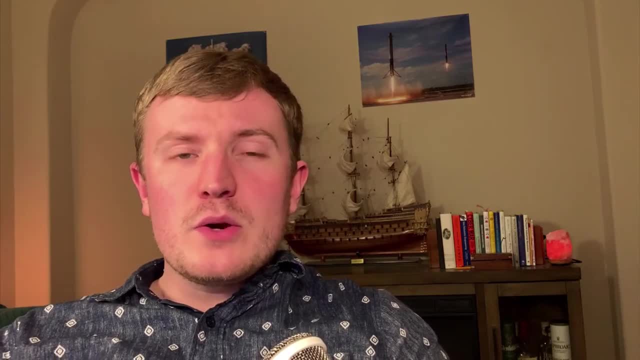 As we talk about these steps, think about how they will fit in your existing or even future development lifecycle. Step number one is discovery and selection. Now, you're not meant to tackle all of it at one time. Instead, As we will see in a different lesson on threat modeling, there is a different way of prioritizing. 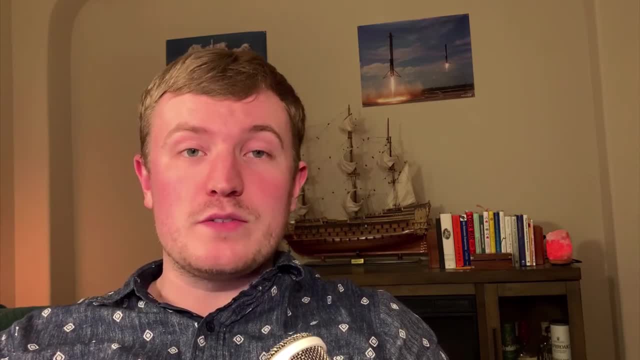 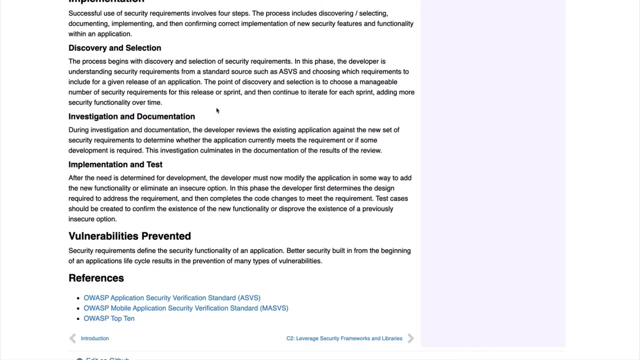 risk based on threats, so we will be revisiting prioritization in a future lesson. Step number two is to investigate and document. During the investigation and documentation phase, review the existing application and compare it against the security requirements that you've outlined as necessary, and then 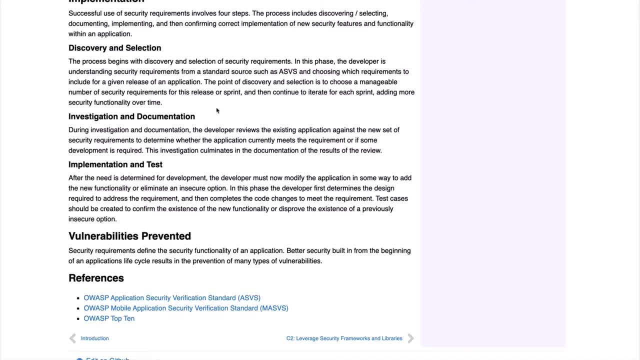 from there, figure out which requirements your application meets and which requirements still need development, and make sure to document the investigation so that it remains accurate over time. Step three is to implement. After you've investigated and documented your findings of deficiency, it's time to turn. 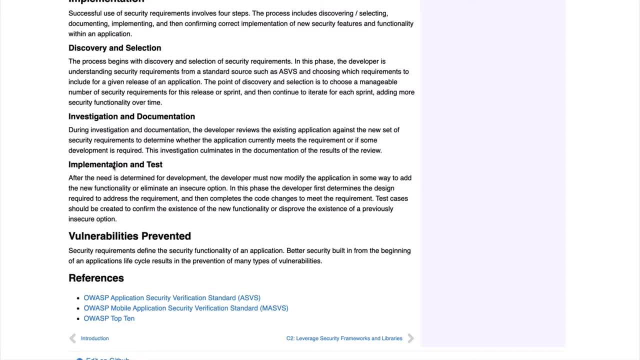 that into action, like we just talked about, and either modify the application to add the new security functionality or eliminate the insecure option. And then we've got step four, which is to test. Implementing the changes just isn't enough. as the final step you have to create those. 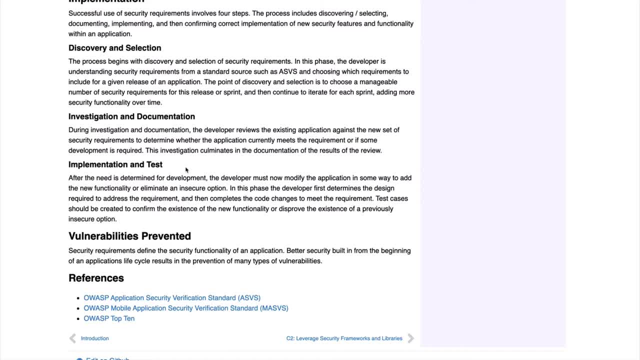 test cases in order to confirm whether the modified functionality solves that requirement or not, And if it doesn't, Then go back to the implementation phase. but if it does, then it's time to update documentation and then move on to the next requirement. 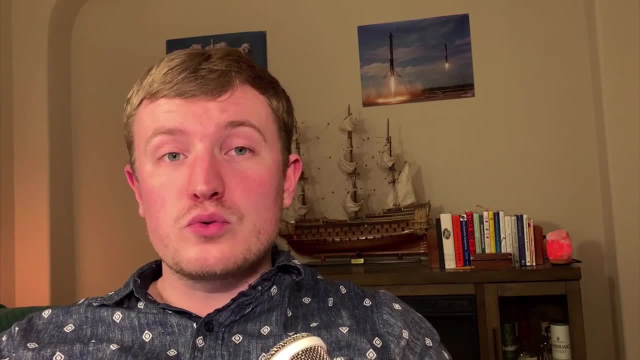 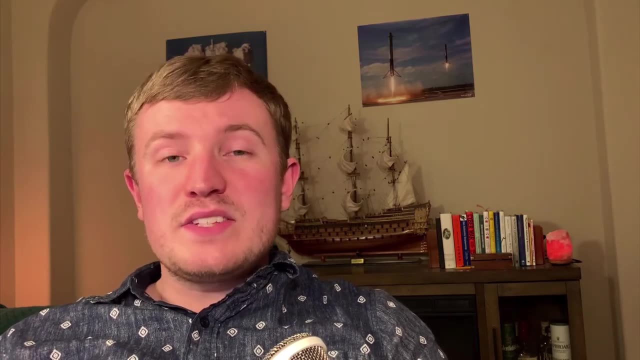 And, as we wrap up, control number one reflect on the fact that this control, which is deemed to be the most important out of the top 10 by OWASP, is not about a specific threat. Instead, it's about building a process that has security in mind from the very beginning. 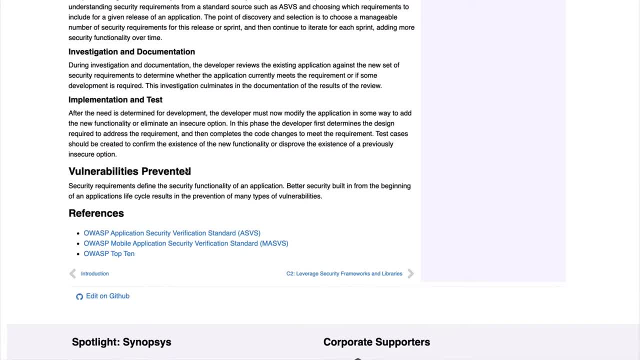 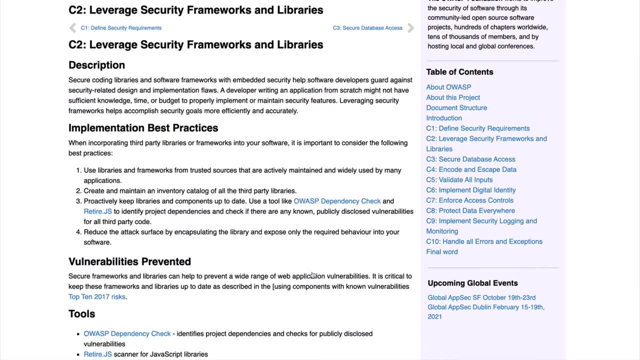 instead of being an afterthought. Alright, so that's control number one of the proactive controls. let's take a look at C2.. C2 is to leverage security frameworks and libraries. This control focuses on third party frameworks and libraries, which provide a ton of value. 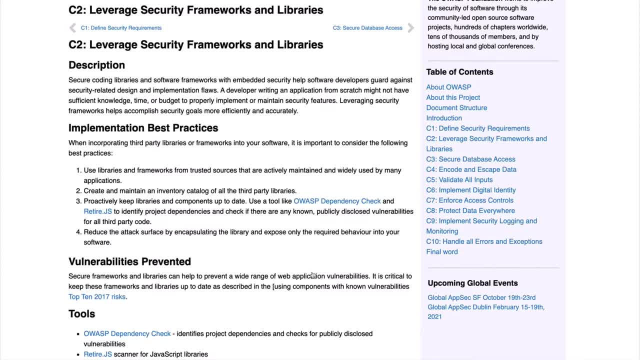 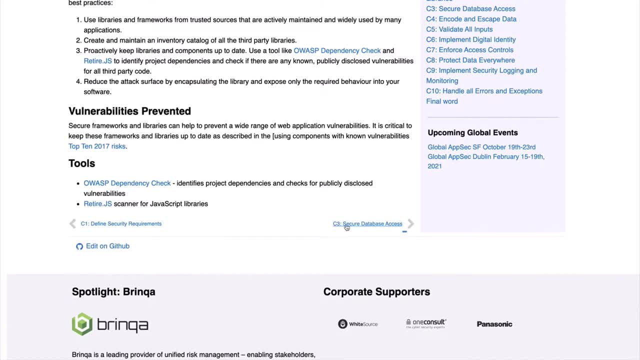 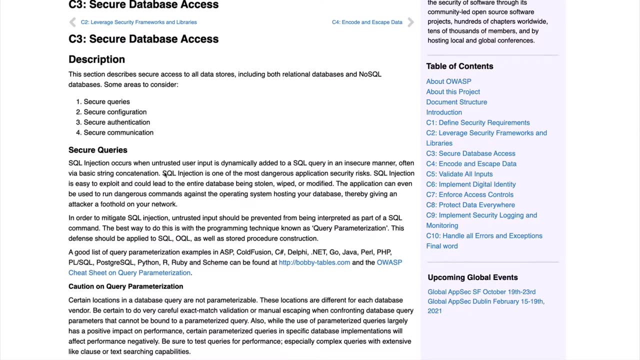 but can also introduce nasty vulnerabilities if it's not managed properly, and we'll talk more about this later in the course, but go ahead and review this control now or after completing. the lesson C3 is about securing database access. An important sentence to highlight on this page is that SQL or SQL injections depending, 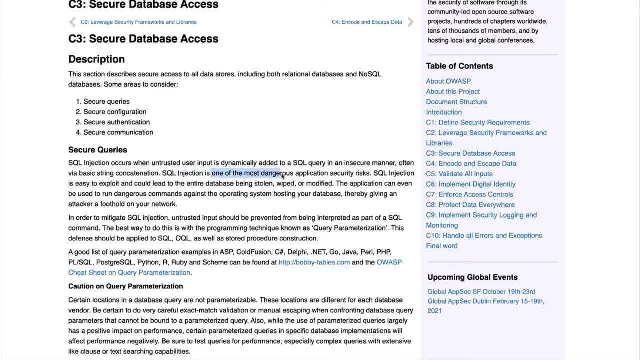 on if you come from Linux or Windows background. This is one of the most dangerous application security risks. Chances are high that you've heard of SQL injections, because they happen way too frequently and they can do serious damage, like exposing entire databases that can contain critical 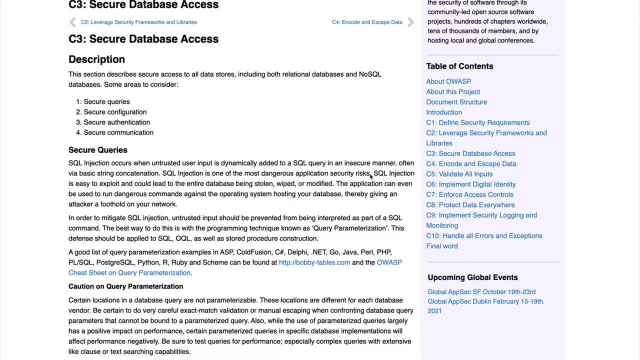 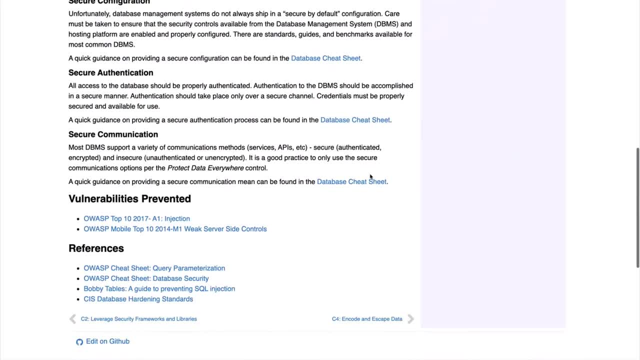 data such as passwords and medical or financial records, And this is another important topic that we will revisit in the course and that I recommend you spend more time reading about on this page. Next, we'll look at C4, which is encoding and escaping data. 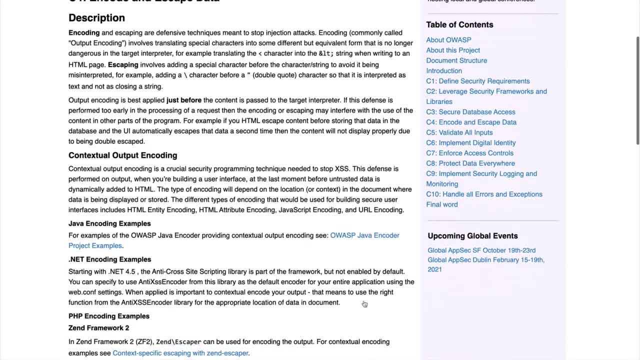 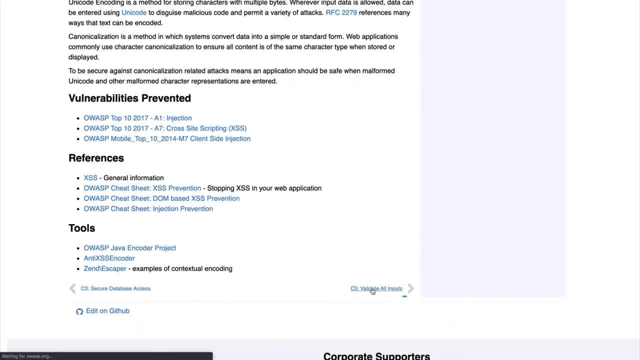 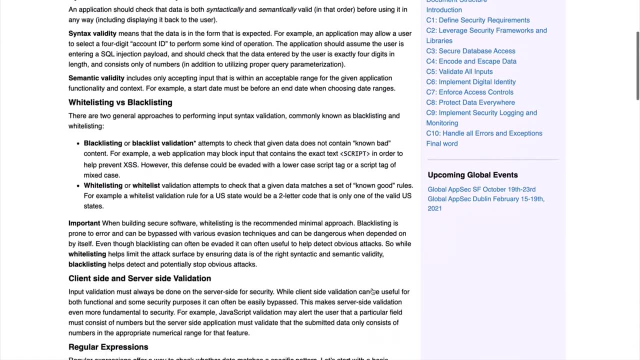 Again. you've likely heard of cross-site scripting attacks and encoding. slash escaping is a defense against these types of attacks. C5 is all about validating all inputs, which will also help defend against cross-site scripting, SQL injection, gaining elevated privileges or other forms of attack. so make sure you. 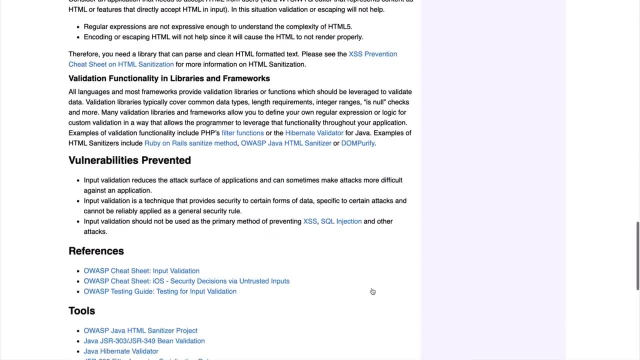 spend some time reviewing this page. Next we've got C6, which is implementing digital identities. C5 is a defense against all inputs, which will also help defend against cross-site scripting, SQL injection, gaining elevated privileges or other forms of attack. so make sure you. 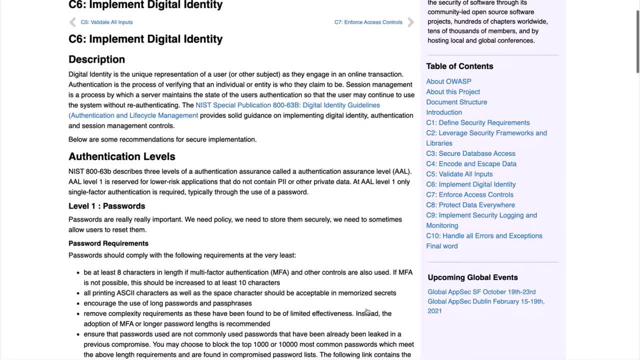 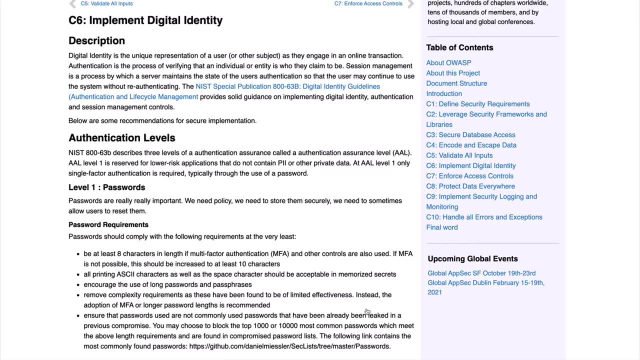 spend some time reviewing this page. Next we'll look at C6, which is implementing digital identity. C6 defines the digital identity as the unique representation of a user or other object as they engage in an online transaction. Authentication is the process of verifying that an individual or entity is who they claim. 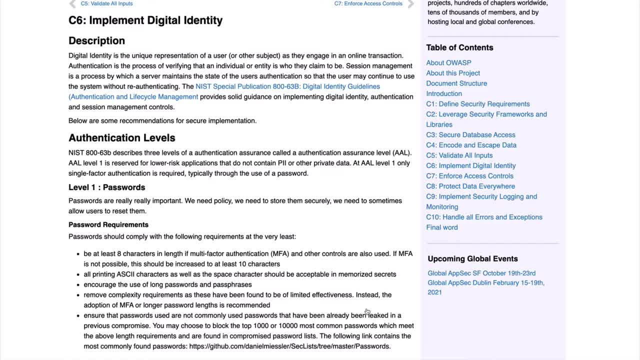 to be, while session management is a process by which a server maintains the state of that user's authentication so that they can continue using the system without having to re-authenticate, just like when you're browsing a website. Next we've got C6, which is implementing system authentication, which will also help defend against cross-site scripting or other forms of attack. so make sure you spend some time reviewing this page. 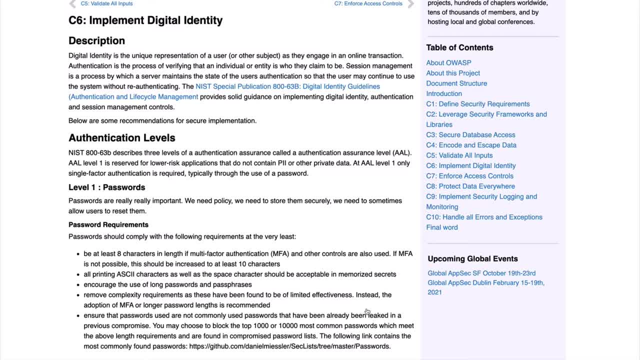 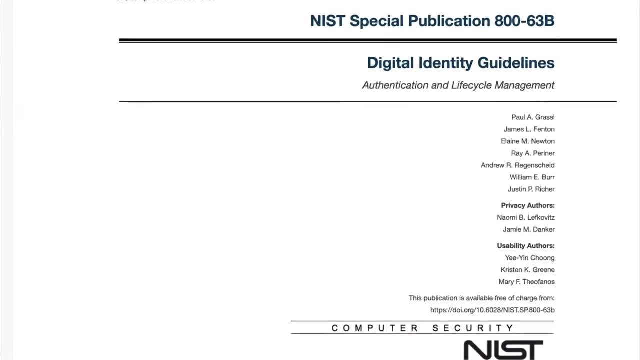 and all of a sudden it asks you to log in again. Now, what's particularly interesting on this page is that we revisit a level similar to what we saw in the ASVS, The NIST 800-63B, which is a guideline from the National Institute of Standards and Technology. 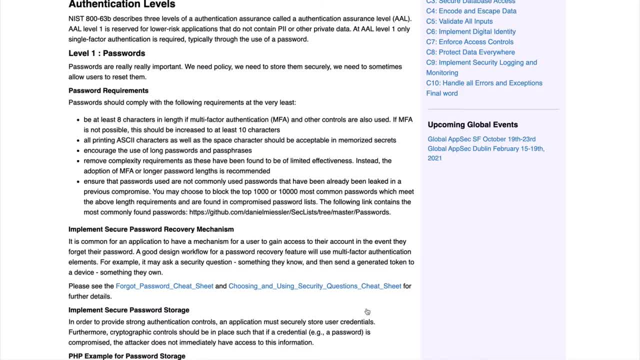 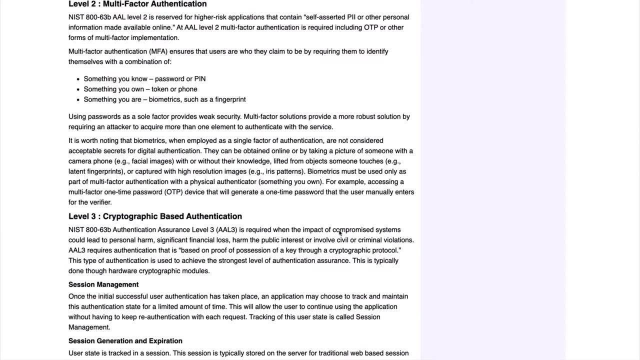 outlines 3 levels of authentication assurance, with level 1 being for lower risk applications. they only require passwords for authentication, but with other requirements listed below. Level 2 instead requires multi-factor authentication with a combination of a password or PIN, a token or phone and or biometrics. And then level 3 requires 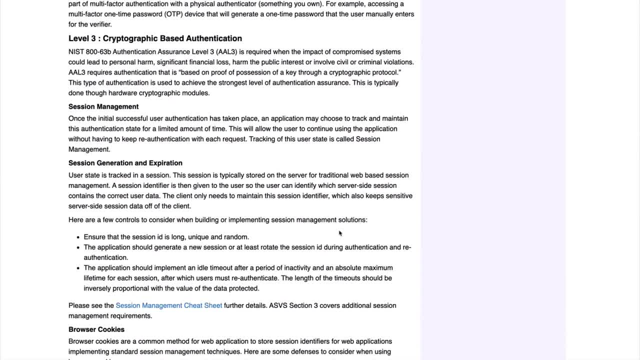 cryptographic-based authentication, which is providing proof of possession of a key through a cryptographic protocol, usually done through hardware cryptographic modules. Now be sure to read the rest of this page for more information on digital identities. But moving on, we then have C7,. 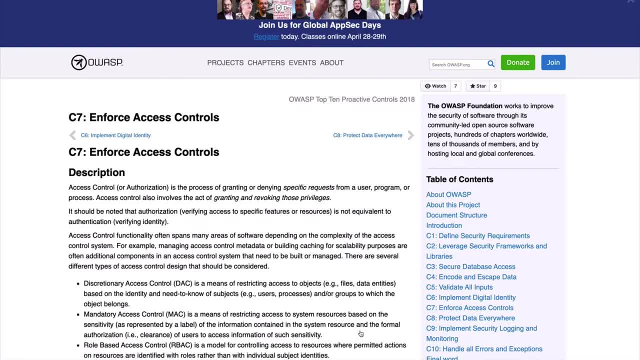 which is a key-based authentication protocol, which is a key-based authentication protocol. And then we have C6, which is a key-based authentication protocol, which is a key-based authentication protocol, is enforcing access controls, And this is different from authentication, since it looks 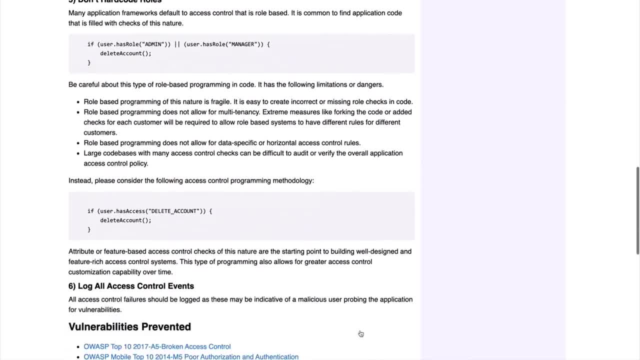 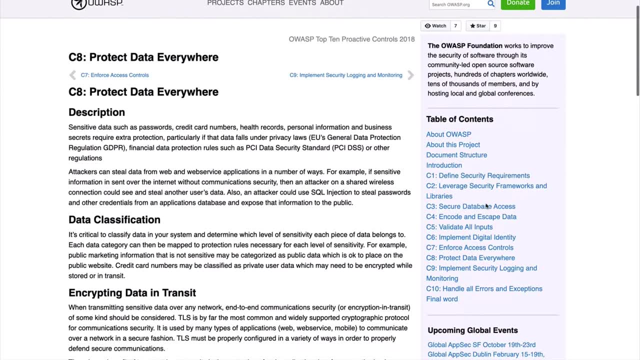 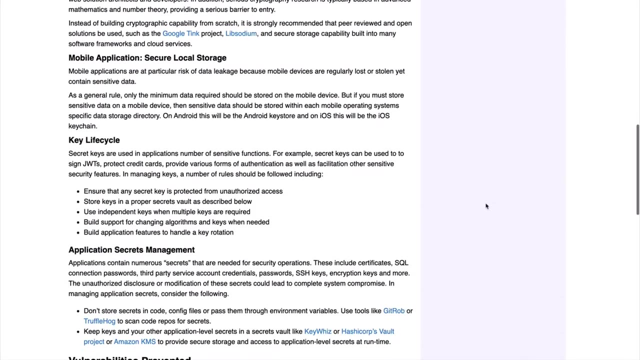 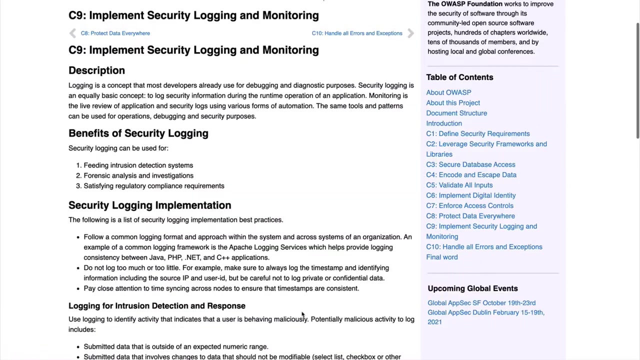 at processing access for specific requests, compared to verifying identity. C8 is to protect data everywhere, Data such as passwords, credit cards, health information, etc. This is where understanding concepts such as encryption in transit, at rest and in use comes into play. Now C9 is about implementing security, logging and monitoring. This is something else. 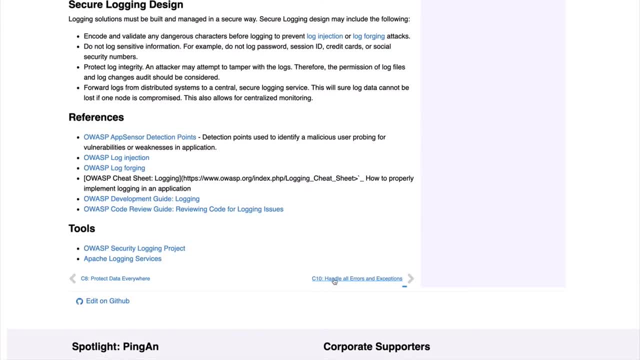 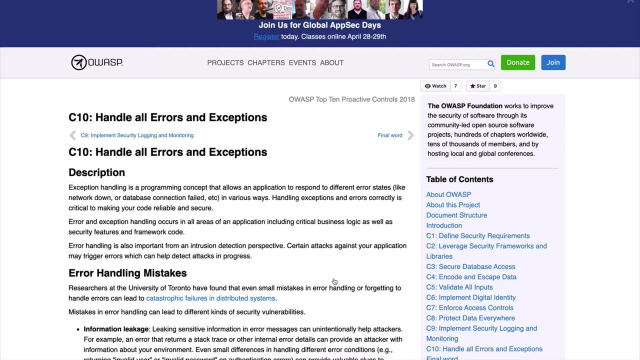 that we'll definitely take a look at again in the course. And then, finally, C10 is handling all errors and exceptions. If you've ever used an application that crashed or gave you an error message and it contained what seemed like sensitive information, then you'll immediately know why this control is important. 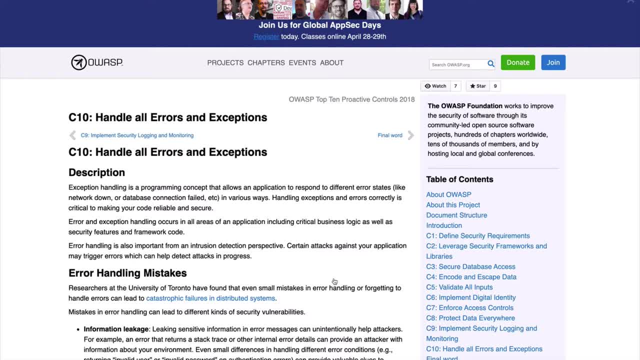 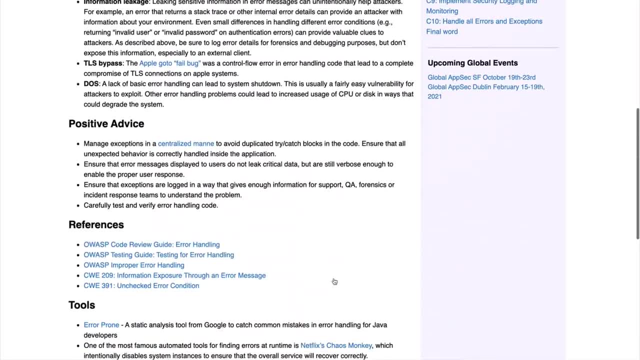 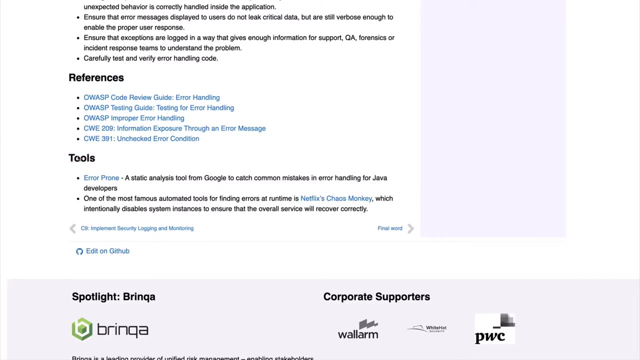 If we don't handle failure gracefully, attackers can use that to their advantage, Like maybe they see an error code that shows them that there is a vulnerability. Now, one more observation before we move on is that each of these controls have references and to tools. I highly recommend that you start looking at those, or at least bookmark them for when you're. 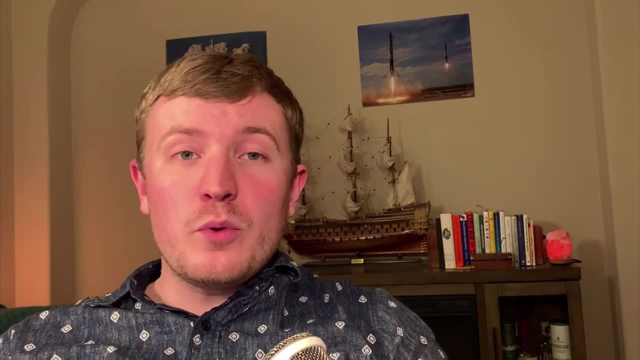 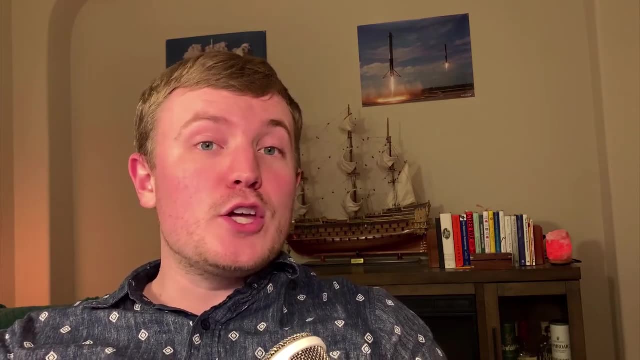 ready to review them Now. again, this is a starting point, but as you go through this list, think about your custom application and organization and think through any other controls that you may want to add in your checklists And, of course, if you're already working on an application or project. 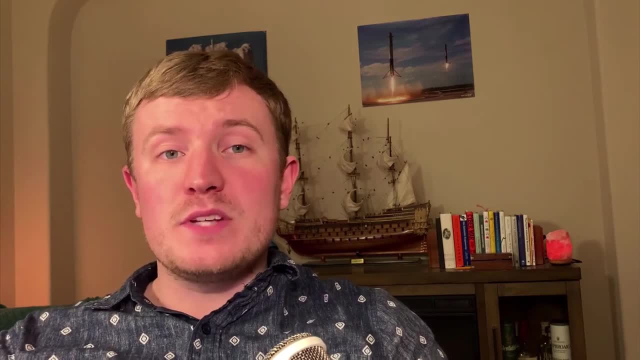 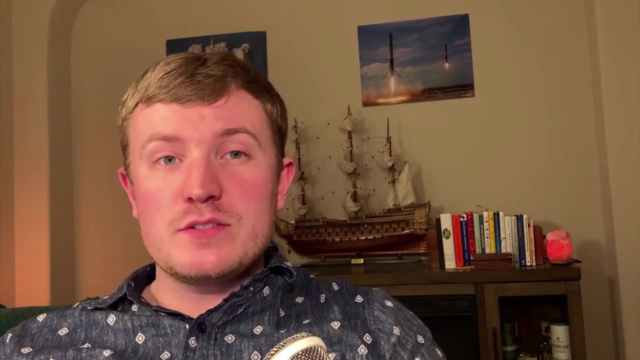 or, if you have one in mind for the future, think about how these top 10 controls can be applied to your projects. Now, these are topics that we're going to explore again in the web, mobile and cloud sections. So, while I went through this list rather quickly, please take some time after. 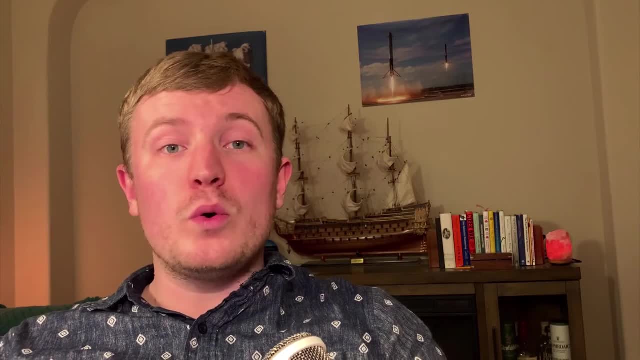 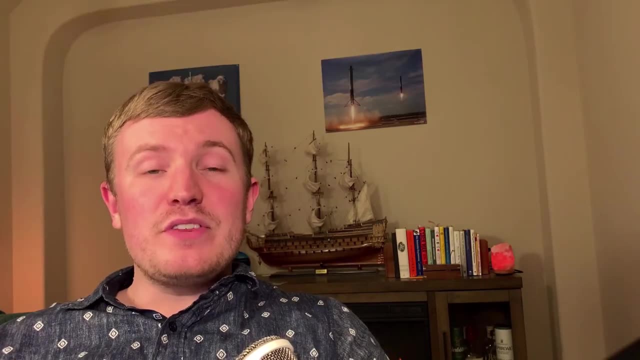 completing this lesson to briefly review them, And don't worry, we will revisit a lot of these proactive controls After that. go ahead and mark this lesson as complete and I'll see you in the next one. Everything we've looked at so far has helped us come up with a baseline for what 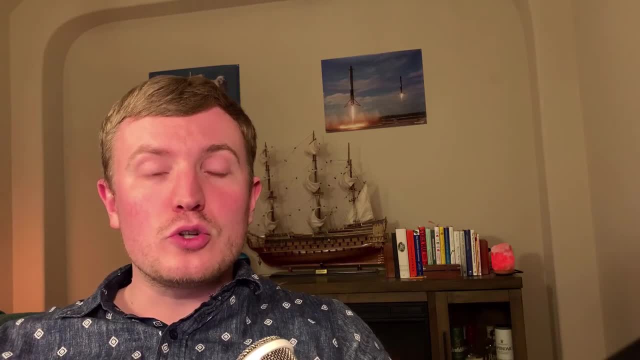 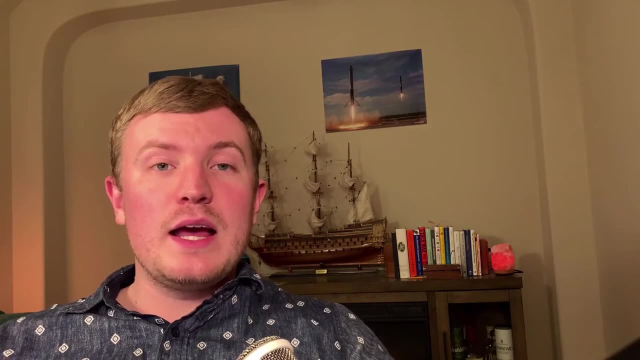 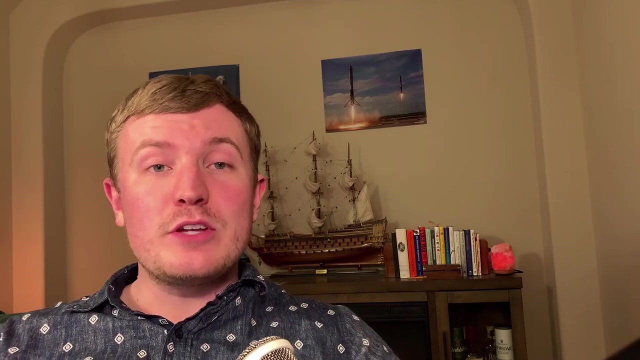 application security means and how to approach such a large undertaking in smaller, incremental steps. But at the end of the day, every organization and every application has its own customer requirements. So we're going to look at another project that helps us create threat models specific to our requirements. These threat models are important to create and consider even before we start testing, because if we don't know where to focus, then we'll probably end up fixing vulnerabilities that are not the highest threats and not the highest priorities, which is a waste of time and a waste of effort. Or worse, what if you release a vulnerability into production and 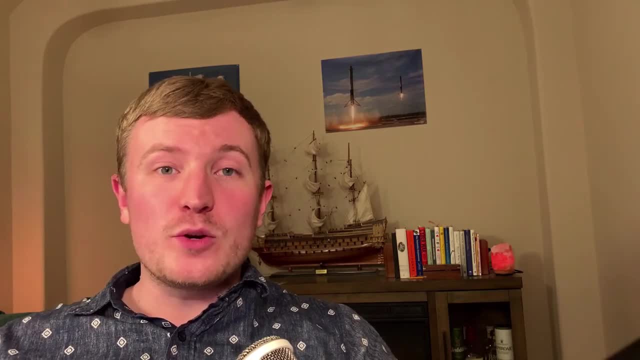 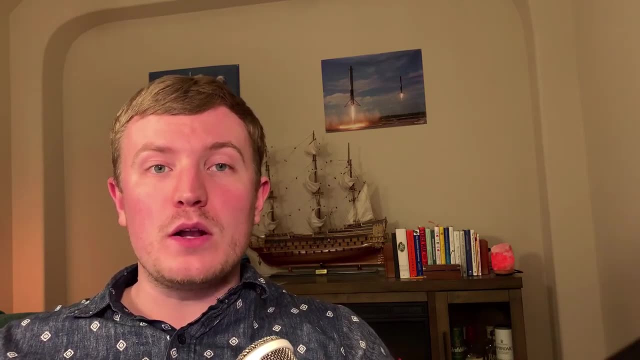 someone compromises it, You don't want to be figuring out how to respond to that and how to figure out its severity in the heat of the moment. Instead, if you have threat and risk modeling up front, you have a playbook that helps you react to that compromise. Now one thing to keep in mind. 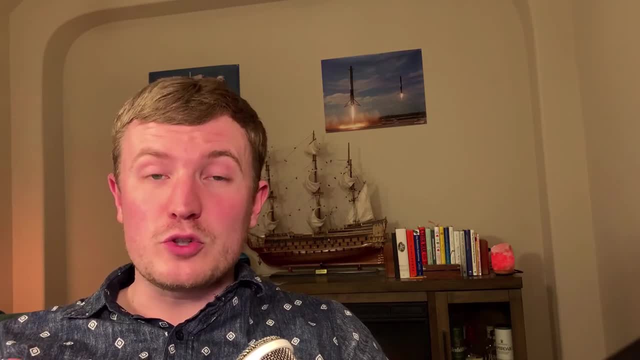 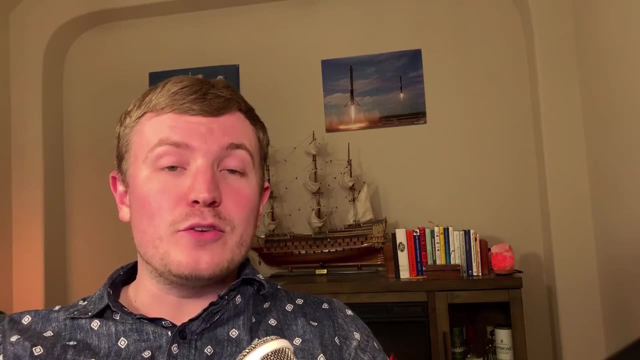 especially depending on the organization that you're part of, especially if it's a larger organization. you're probably not going to be the one creating that threat and risk model. Instead, it will be handed down to you. I still think it's important to understand where and how that comes. 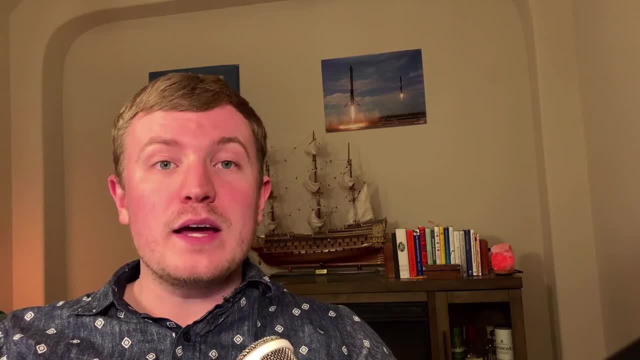 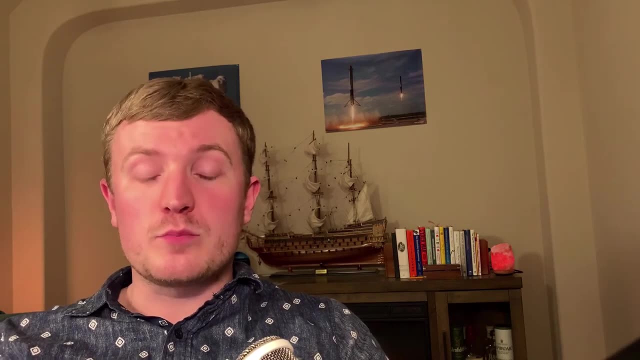 from since. you will inherit that, and you'll have to apply that in fixing the most important vulnerabilities first. Now, the risk modeling approach that we're going to cover today is from an OWASP project as well, So this is what it looks like. It builds on top of: 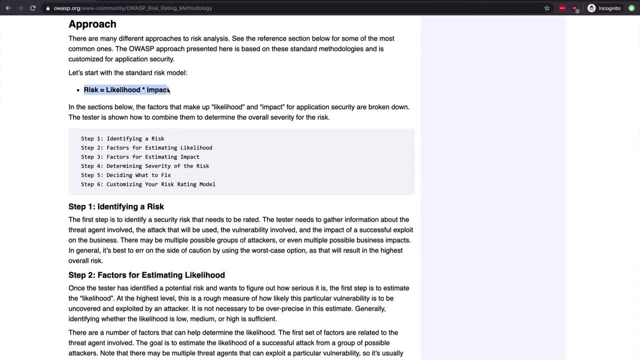 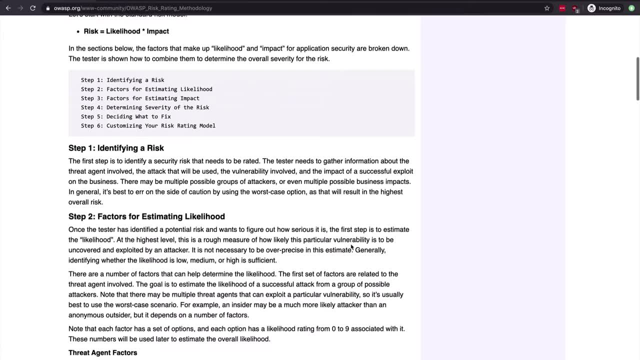 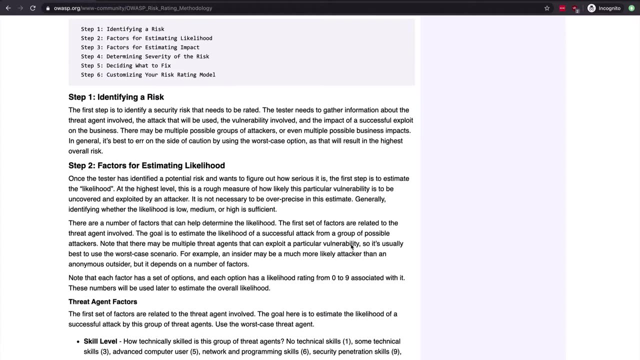 the standard risk model of risk equals likelihood times, impact, And it solves for this equation using six different steps. The first step is identifying risk. With step number one, a tester needs to think through different scenarios and will usually want to look at the worst case scenarios. Once we've identified a potential risk, we need to estimate. 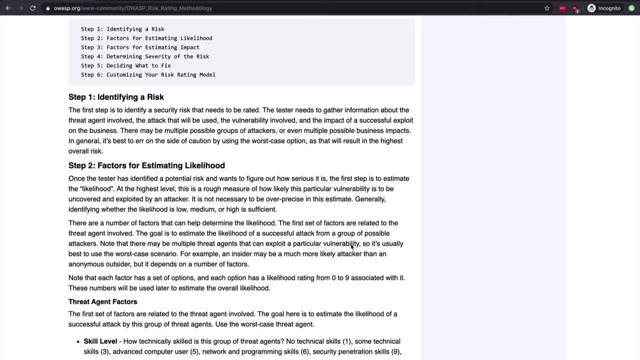 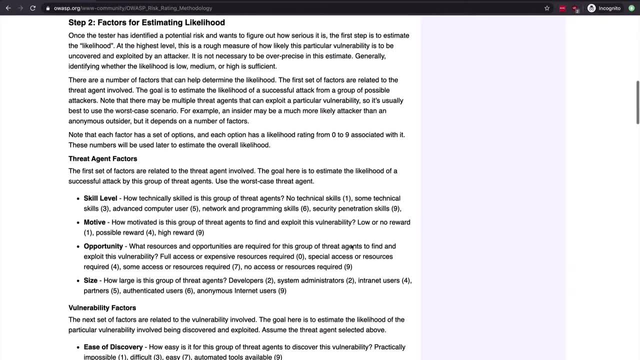 how likely it is to happen by using a low, medium or high rating, And we get these ratings by ranking different factors. Let's take a quick look at what I mean with step number two of factors for estimating likelihood For there to be a threat. there has to be at least one threat agent. How? 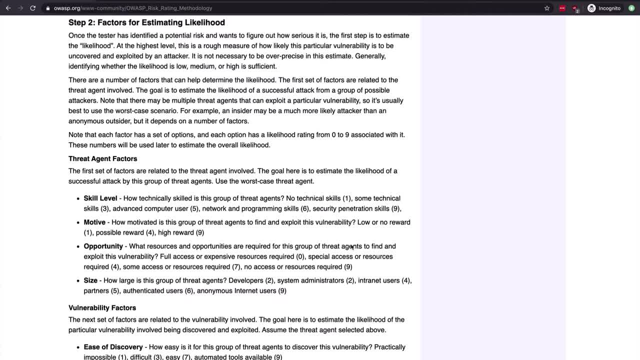 technically skilled. is this person or group of people? What kind of motive might they have? Is there a lot of potential reward, where rewards are often tied to money but not always? And what kind of resources and opportunities are required for that threat agent to 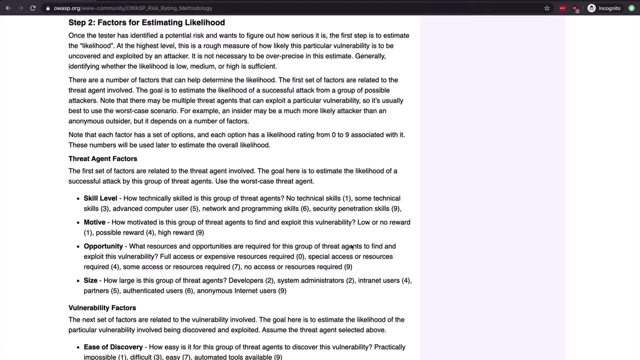 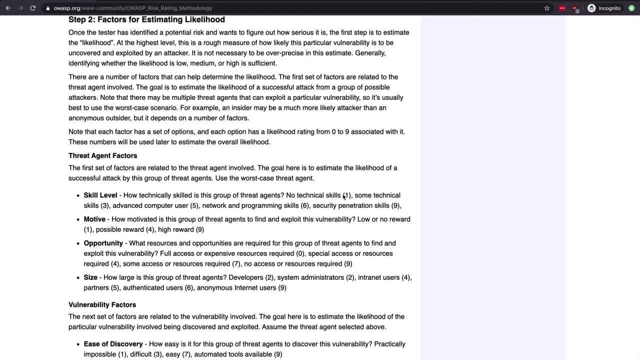 find and exploit this vulnerability? And how large is the group of threat agents? Is it just one person or is it a full team? All of these factors are very important to determine And, as we can see, each answer comes with a ranking number from zero to nine. 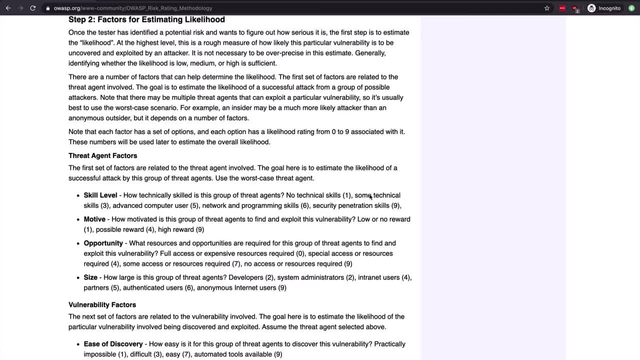 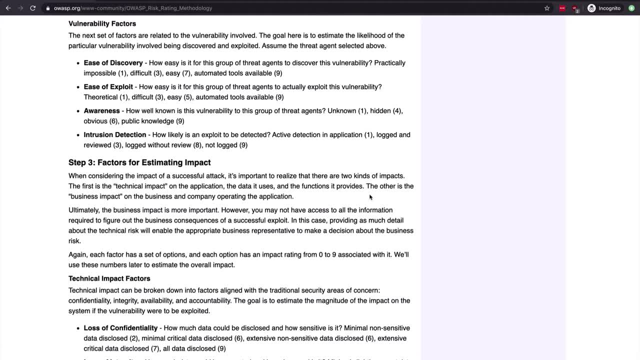 nine being the highest likelihood and zero being the lowest likelihood. Next, we look at vulnerability factors, And we do that with the goal of estimating how likely it is that a particular vulnerability will be both discovered and exploited. So to do that, we need: 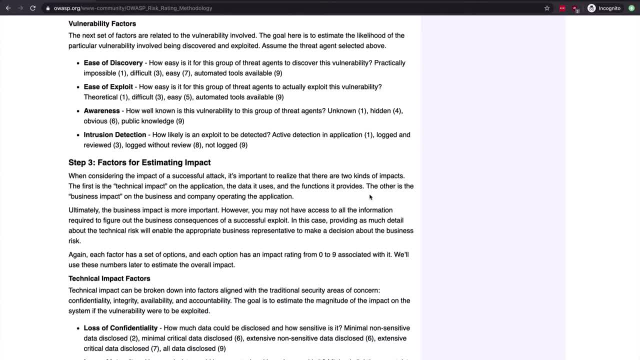 ease of discovery, which is how easy it is for the threat agent to discover that vulnerability, And rankings suggested here are practically impossible. difficult, easy and automated tools available, meaning that the threat agent could run an automated tool to find that vulnerability. 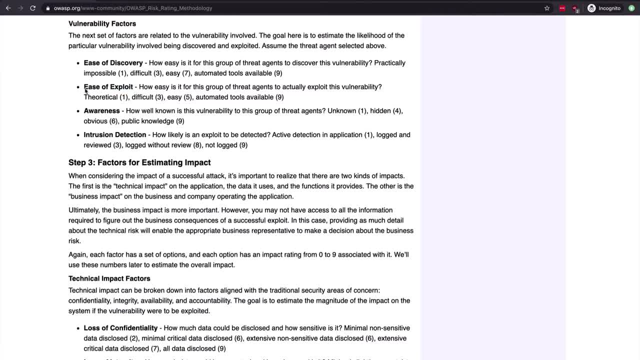 Then there's the ease of exploit, And this is different because perhaps a vulnerability might be easy to find, but maybe it's not so easy to exploit. And then we do have awareness where we're ranking, how well known that vulnerability is. And finally, how likely is it to be detected? Will it be detected by our application? 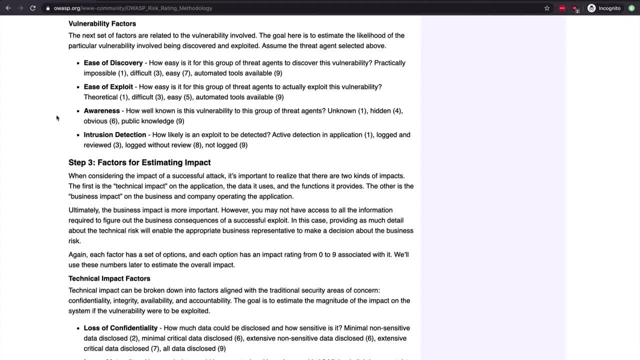 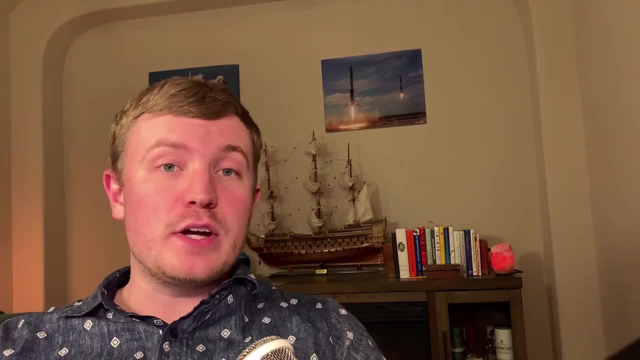 will it be logged and then later reviewed- logged without a review or not logged at all? After going through step two, we'll have enough information to determine the likelihood, but that by itself is not enough, because, even if something's extremely likely to happen, 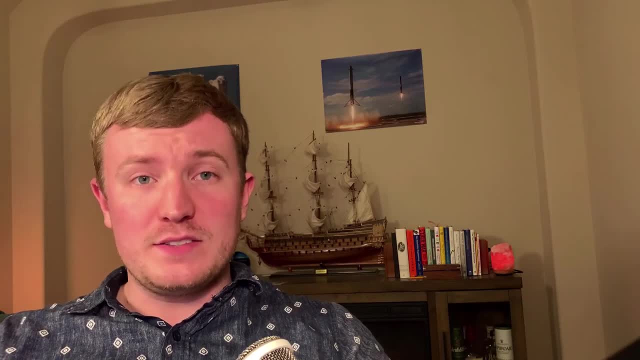 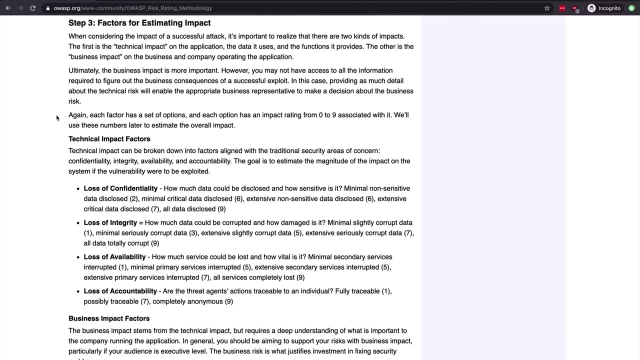 if it has virtually no impact, then it's probably not worth spending time on. So with step number three, we're going to look at estimating the impact, And OWASP reminds us that there isn't just the technical impact on an application that a successful attack brings. 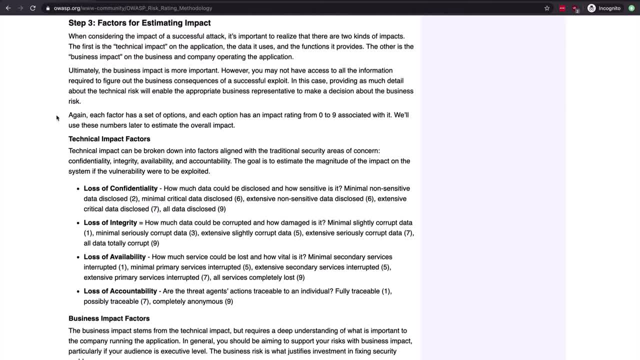 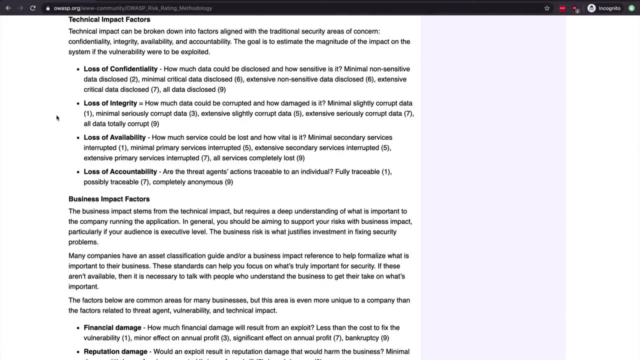 but instead there's also the business impact. So when estimating that impact we have to put both of those factors into the equation. The technical impact factors take into account the magnitude of the impact on the system if the vulnerability were to be successfully exploited And there is the loss of confidentiality. 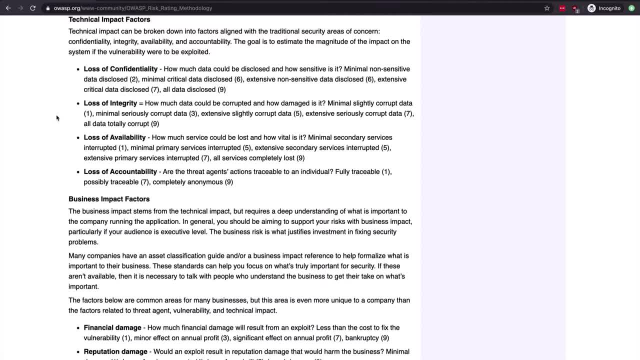 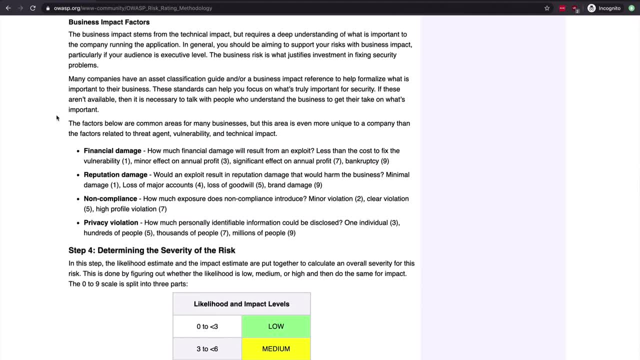 the loss of integrity, of availability and of accountability. On the other hand, the business impact factors. instead, take a look at financial damage, reputation damage, non-compliance or even privacy violations. Now, these are a great starting point, but, as always, keep in mind that 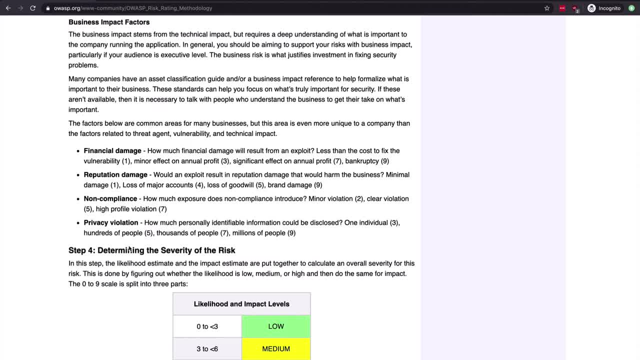 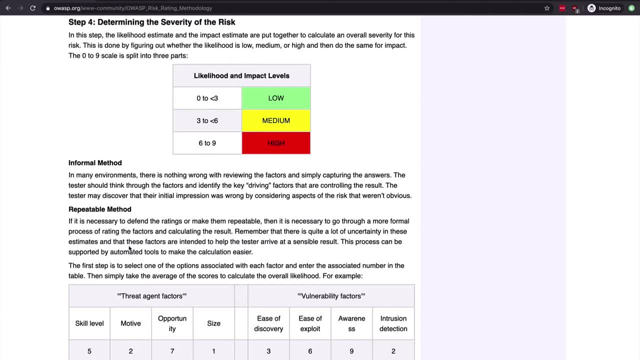 we can add our own custom ones for our business or for our technical impacts, And we're now at step number four. With step number four, we can look at all the ratings that we've worked on to this point and give them that low, medium or high impact. 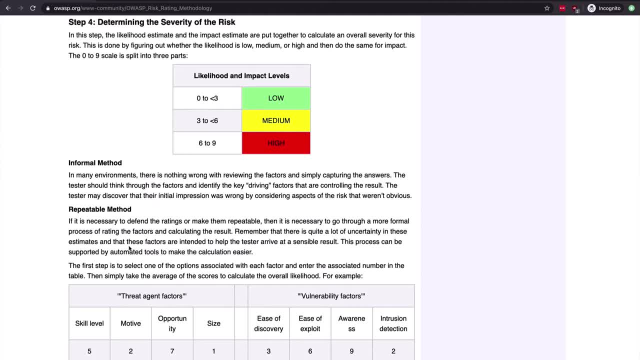 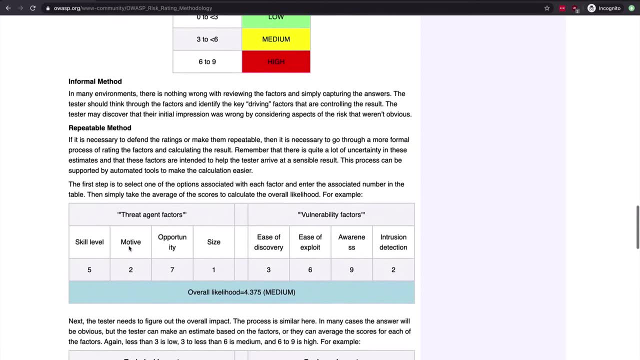 Low is for zero to less than three, medium is for three to less than six and high is for six to nine. And this is a fairly simple model. but OWASP does outline a more advanced calculation that they call the repeatable model. Please take a quick look after. 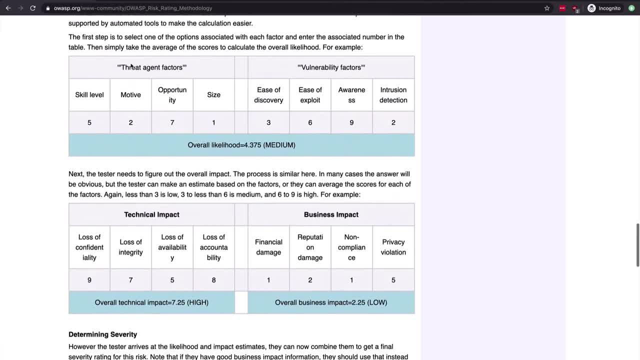 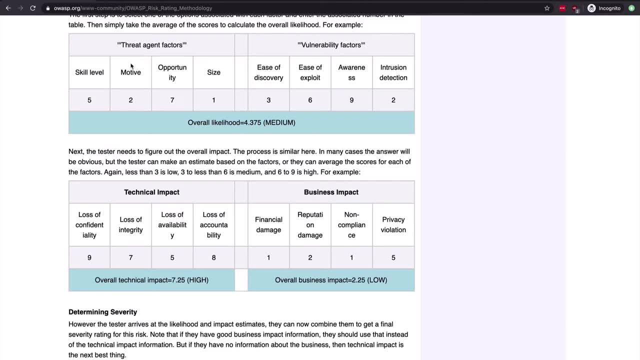 completing this lesson to get familiar with how it works. But as we move on, let's say, for the sake of example, that a certain threat that we're evaluating has a medium likelihood of being exploited, just as in this example. It also has a high technical impact, but it does have a low. 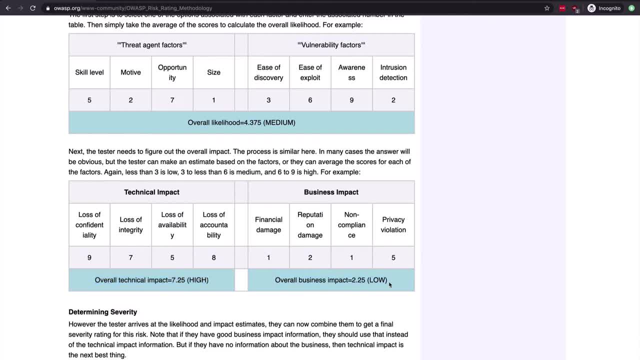 business impact. In that case, OWASP recommends going with the business impact over the technical impact, as long as we can trust that business impact analysis. So even if the technical impact would be high, like in this case, since the business impact is low, we would overall set. 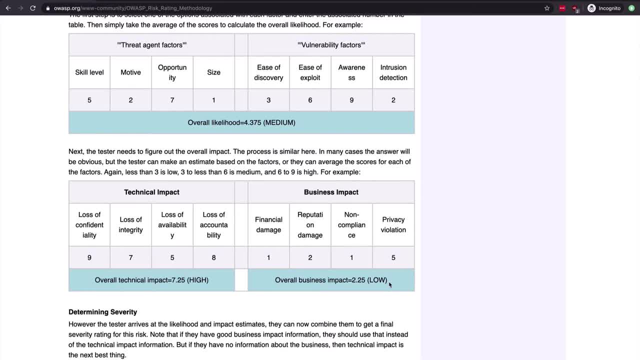 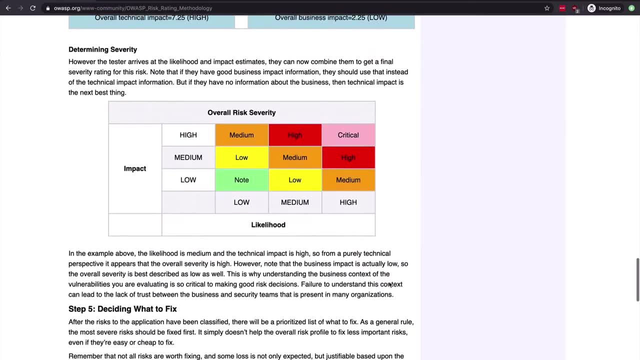 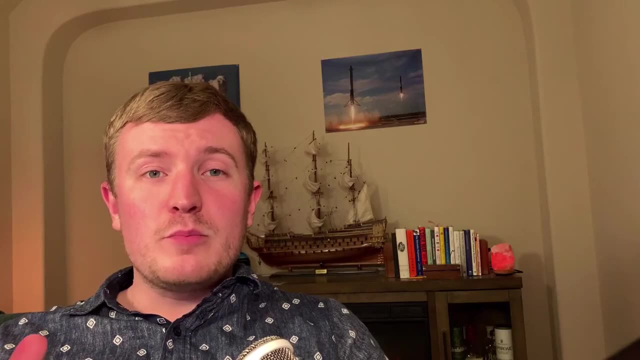 the severity to low And we could have an opposite example where the technical impact is low but the business impact is high, making that overall severity high. And going through this exercise is important because it helps us decide what to fix first, which leads us to step number five. Now, even if you could fix a bunch of low severity risks, 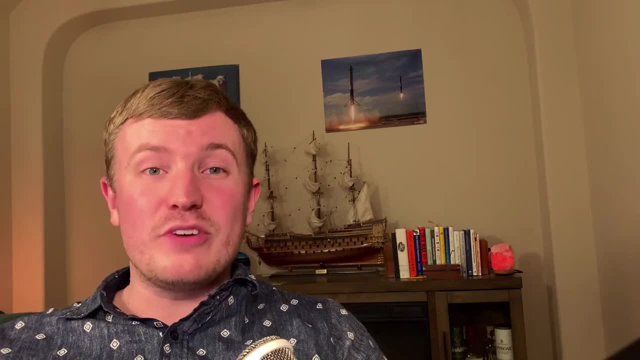 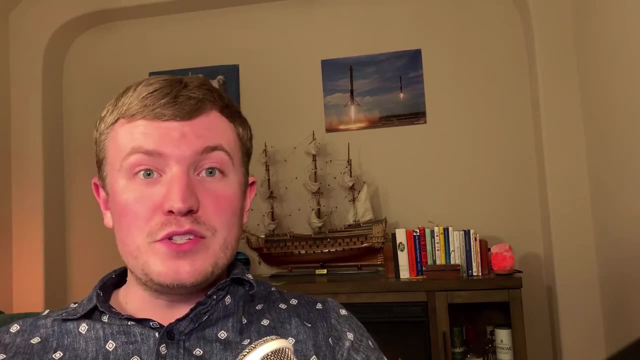 in a short period of time and just one or two high severity risks in that same period of time. you still want to go after the high severity risks, And I say that because- and I'm guilty of this myself- but a lot of us will tend to go after the low hanging fruit. 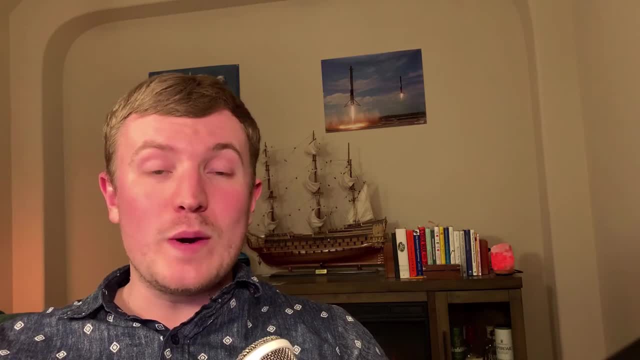 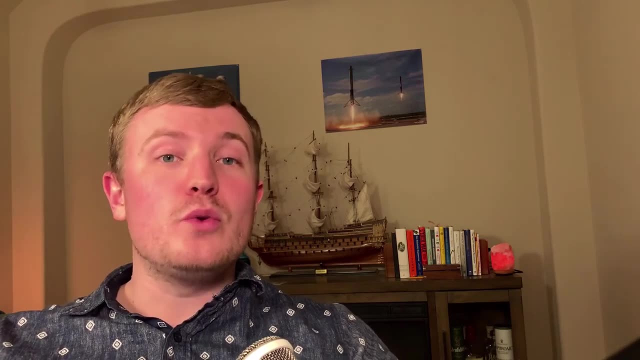 So we might look at an easy vulnerability to fix, even if it's low impact. we might think, oh, you know what, I'll start there and then work up to the high severity and longer tasks. But you want to do the opposite? All right, now let's wrap up with risk number six. 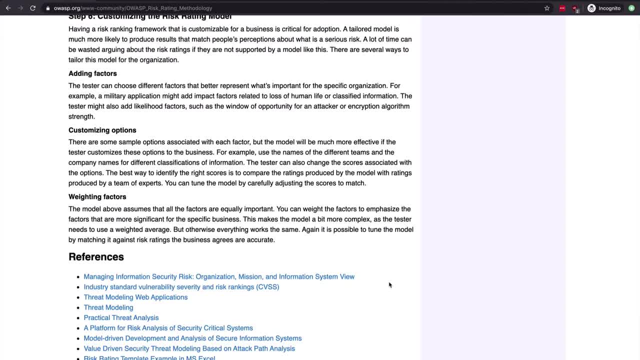 which is to customize the risk rating model, And we've talked about this throughout the course, but it bears repeating here, especially if you just grab what you see on this page and you don't attempt to customize it to your organization, it won't be effective. 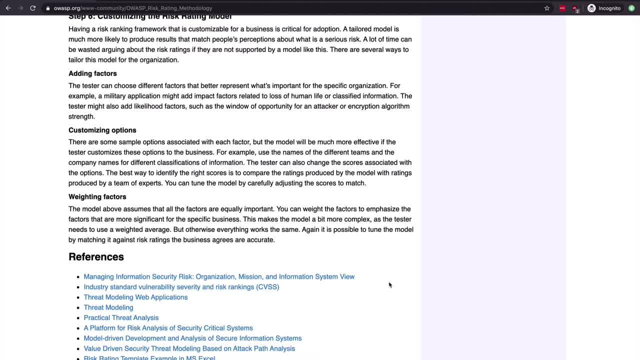 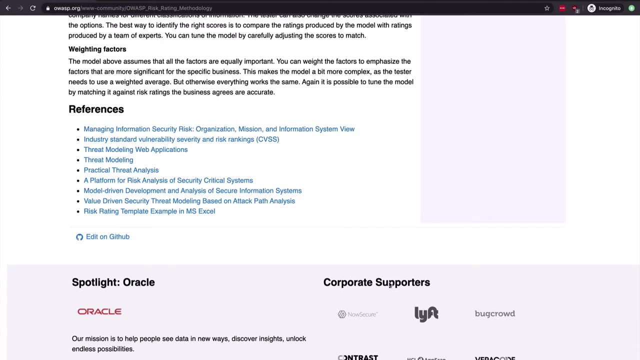 in convincing leadership and it won't be effective in stamping out the biggest threats. Take what's here and customize the different factors and options until it makes sense for your organization and your application, And, as you can see here, this page provides many references that go into much more detail for risk and threat modeling. 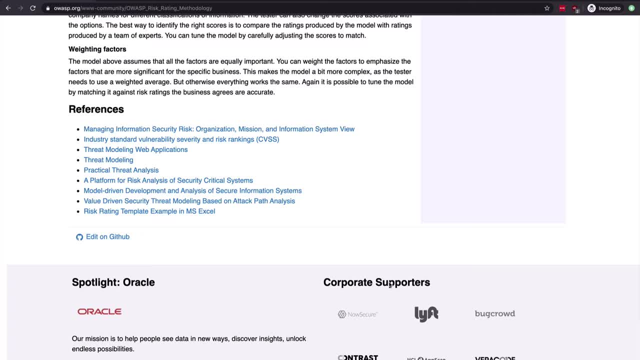 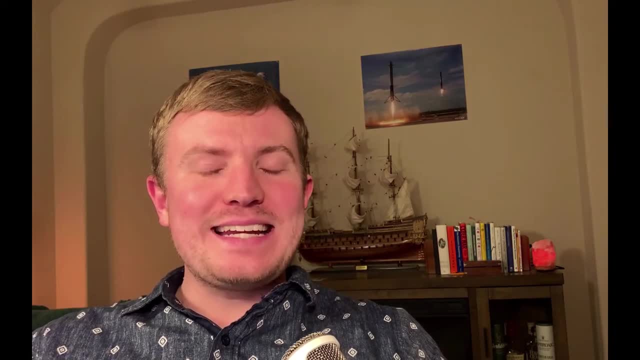 Be sure to save these resources for when you tackle threat modeling for your app and your organization. Now, with that in mind, let's go ahead and mark this lesson as complete, and I'll see you in the next one. One more peg that we're going to add in order to support our baseline: 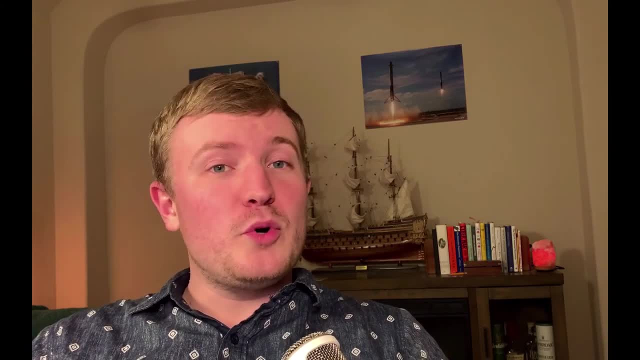 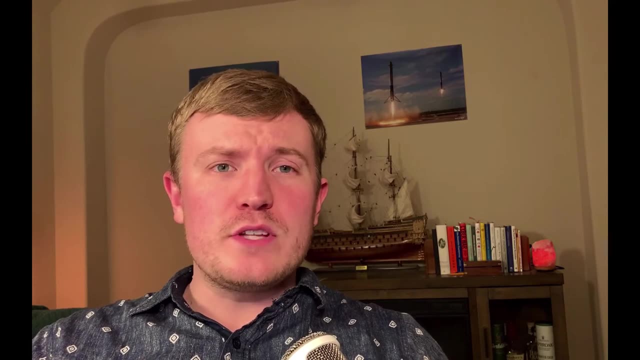 is exploring the OWASP cheat sheet series. Up until this point, we've looked at the application security verification standard, SAM, proactive controls and threat modeling. Just between those different projects, we could spend weeks, weeks or even months going through everything, only to just forget all about it when you actually 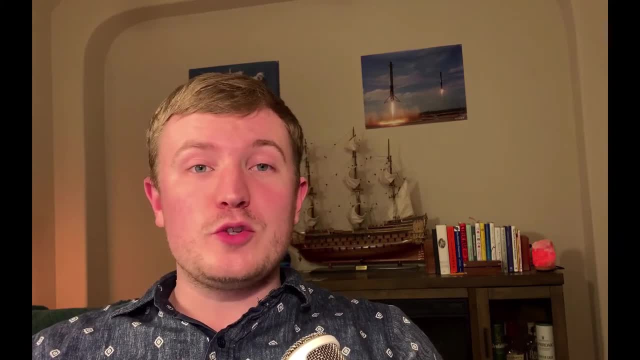 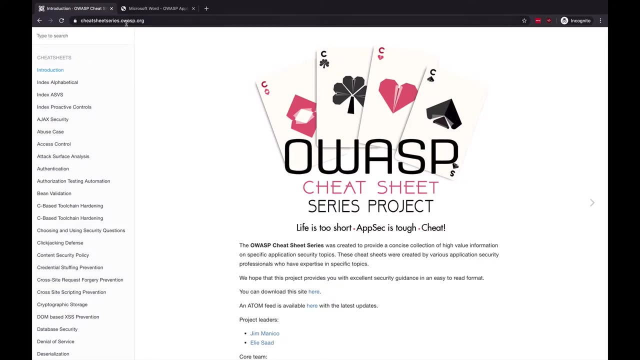 need it. So the awesome group at OWASP created this cheat sheet that we're going to look at in this lesson, and I highly recommend that you bookmark it and continuously reference it. You can find the cheat sheet at this URL. On the left hand side, we have a convenient table. 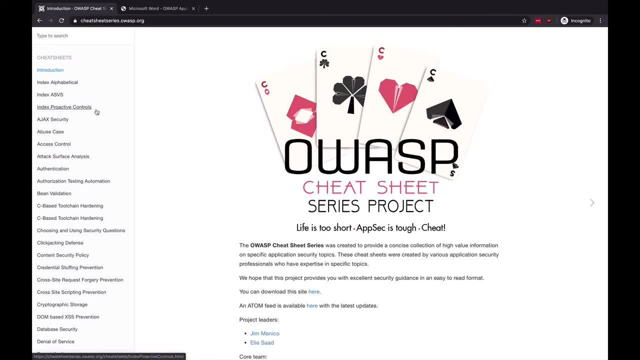 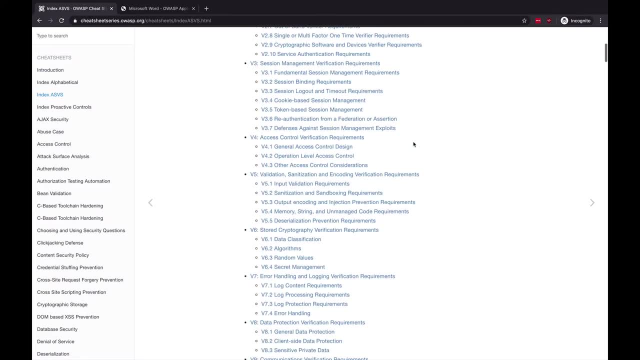 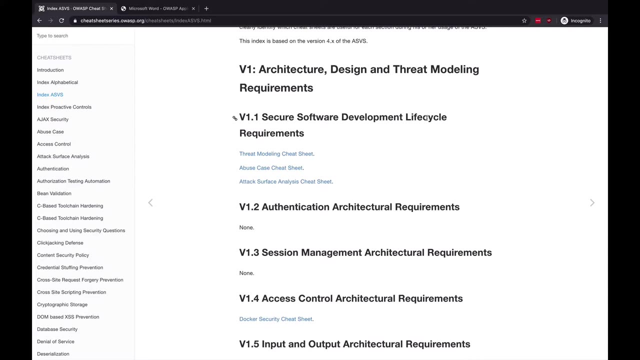 of contents. that lets us quickly jump to relevant areas. Let's start with the index for ASVS. So for V1.1 of secure software development lifecycle requirements. they link to the threat modeling cheat sheet, the abuse case and the attack surface analysis cheat sheets. 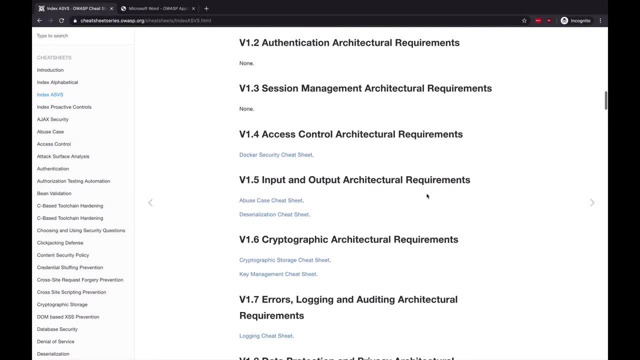 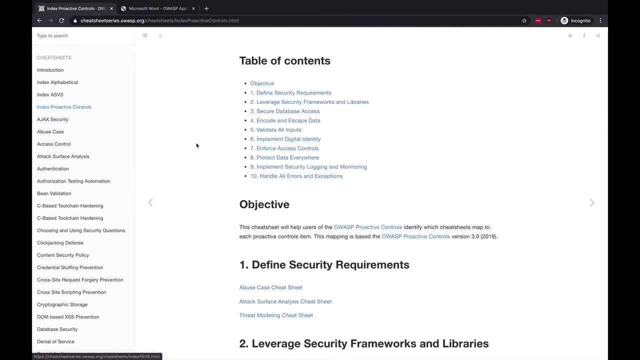 So this makes it very easy and convenient to go from the requirement that we're solving for to the cheat sheet associated with it, And the same thing goes for proactive controls, which has its own index. Now you'll quickly notice on the left hand side that not all of the 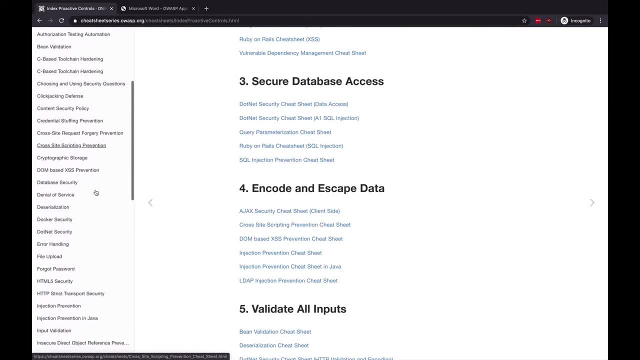 features that we're going to be looking at are linked to the same thing. So if we're going to look at some of the features that we're going to be looking at on the left hand side, that not all of the cheat sheets may be relevant to you, depending on the language that your application is coded in. 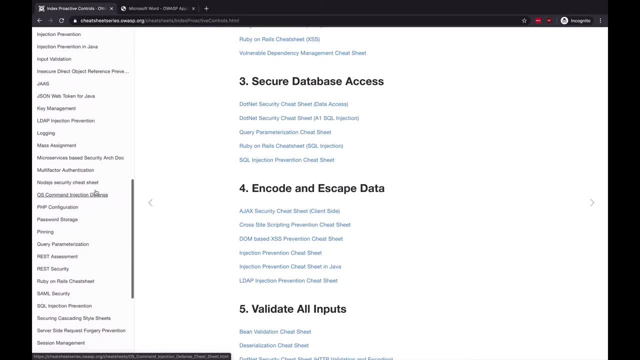 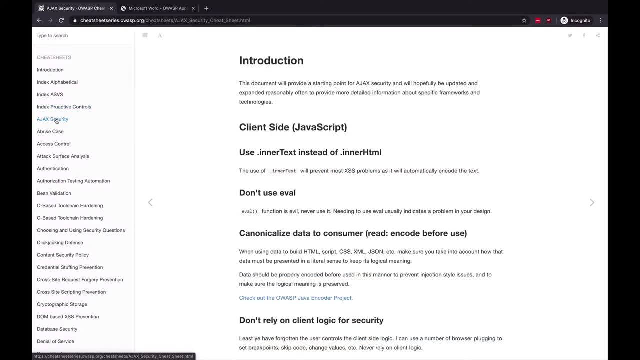 Some of these are specific to PHP or Ruby on Rails or NET and so on, But let's take a look at a few of these cheat sheets so that we can get the hang of it. And let's start with AJAX security. Here we'll find a number of strong 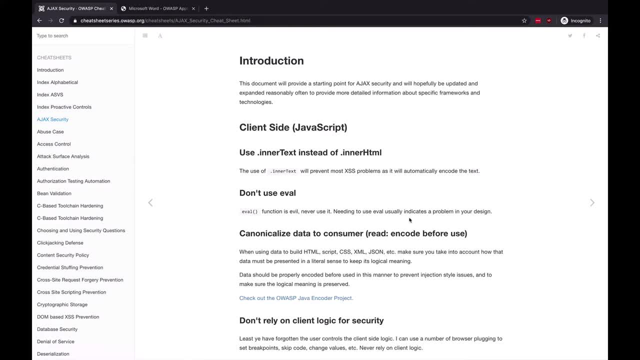 straight to the point rules that can help us stay out of trouble, For example, the use of inner text instead of inner HTML. This can help prevent most cross-site scripting problems, as it automatically makes it easier for the user to use the text that they're using. 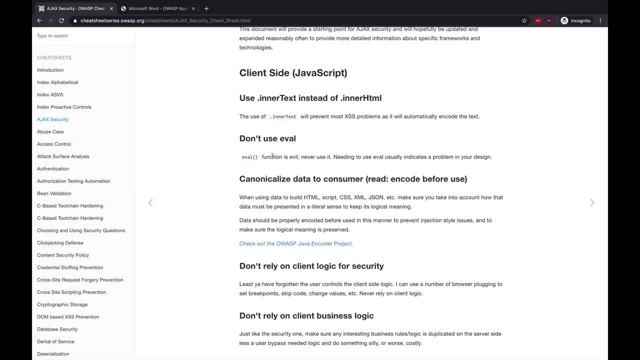 Here it says: don't use the eval function because it's evil and to never use it If you're not familiar with JavaScript. eval executes JavaScript code. so if a malicious user manages to slip in bad code and that gets executed, well, you get the idea. 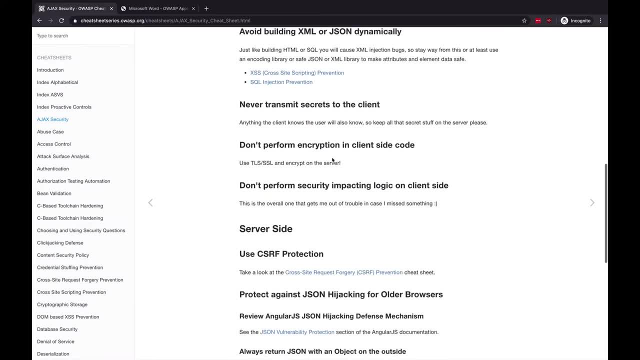 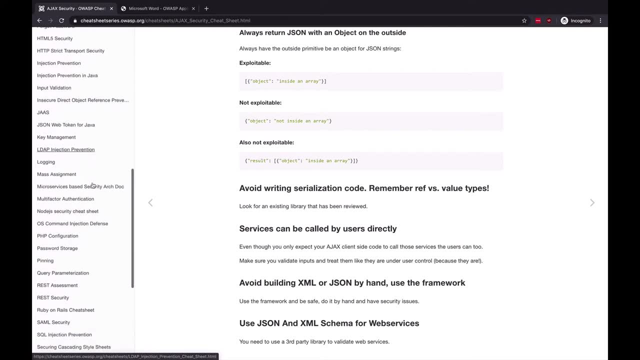 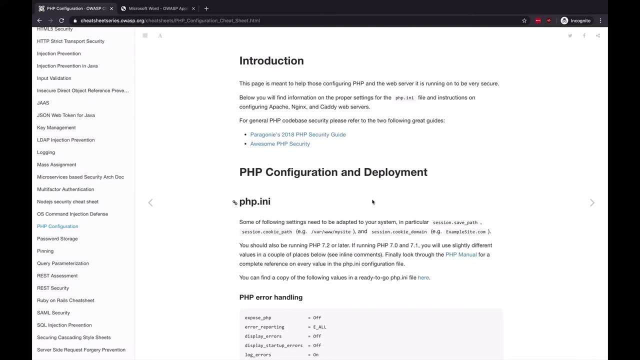 And there are a few more to look over if you're using JavaScript and AJAX calls. We'll also take a look at another one, which is called PHP configuration. It includes a list of important configurations to be aware of and to modify, since often times the defaults. 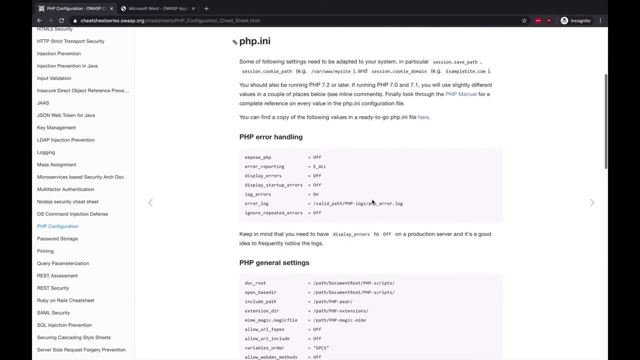 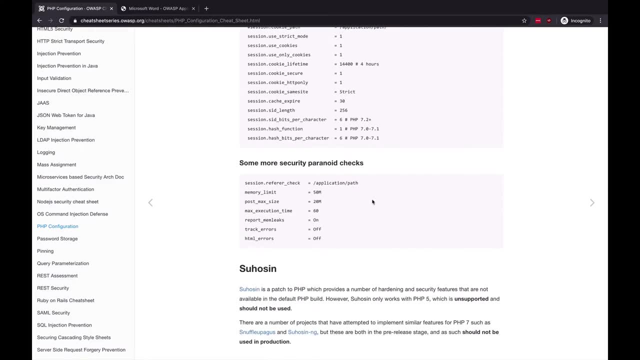 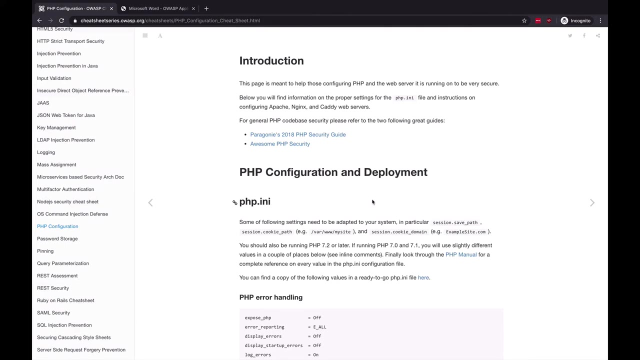 do not focus on security, and instead they focus on ease of use. So this is another example of what you'll find in these cheat sheets, and I do encourage you to mark this lesson as complete and then explore relevant ones in more detail. Also, be sure to bookmark this page, because you'll be able to use it. 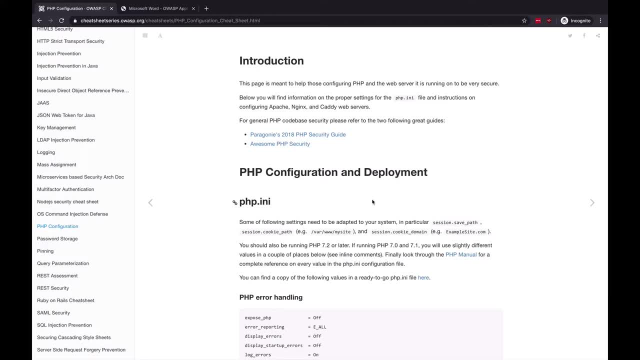 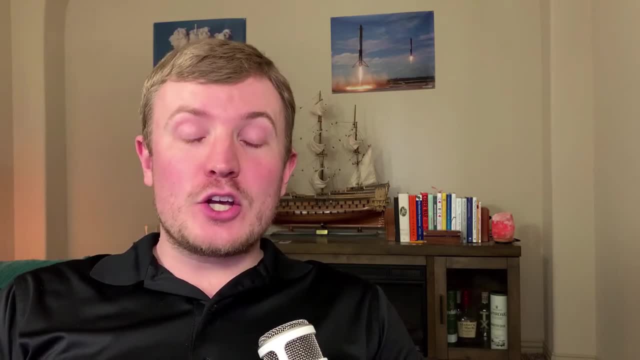 over and over again in the future. Then, once you're ready, I'll see you in the next lesson. Would you believe me if I told you that the vast majority of web applications in production today contain known vulnerabilities? And by known vulnerabilities I literally mean? 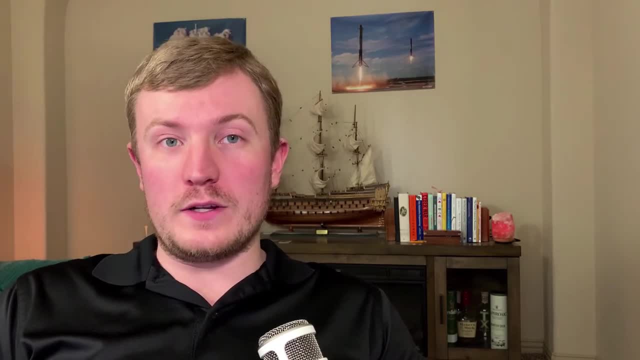 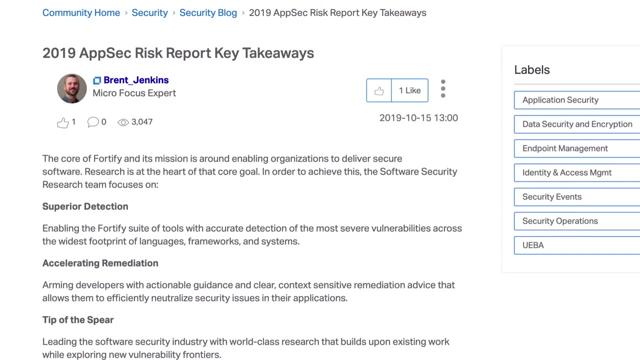 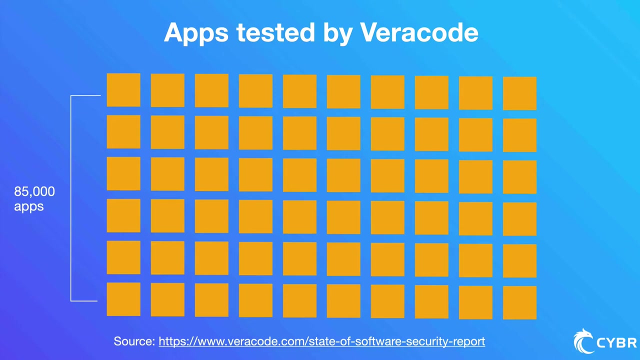 vulnerabilities that have already been found and publicly reported. Well, you don't have to take my word for it. A Micro Focus 2019 Application Security Risk report found that nearly all web apps have bugs in their security features. A Veracode State of Software Security- Volume 10 report from 2019. 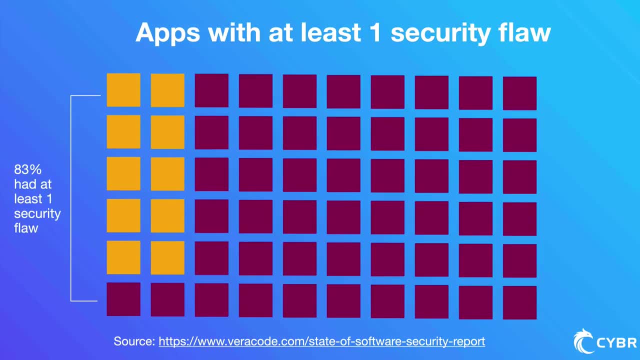 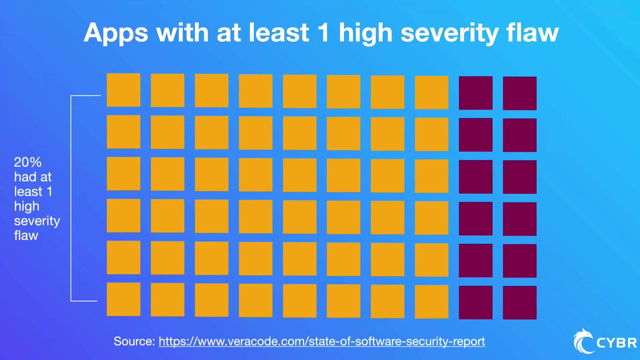 shows that 83% of the 85,000 applications that they tested had at least one security flaw. Many had much more, as their research found that a total of 10 million flaws and 20% of all applications had at least one high severity flaw. 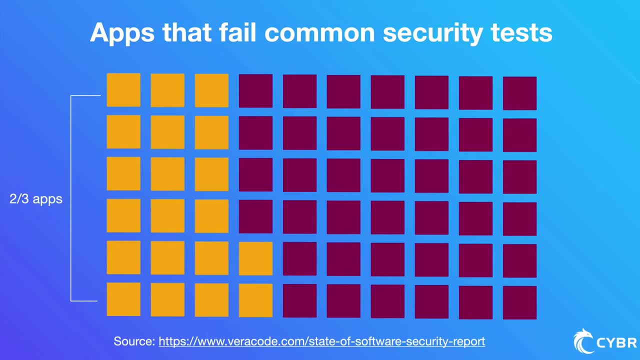 In fact, two in three applications failed to pass tests based on the OWASP top 10 list and the SANS top 25 most dangerous software errors. And these stats only account for known vulnerabilities and, to be fair, I'm sure that there are a number of them that are false positives. 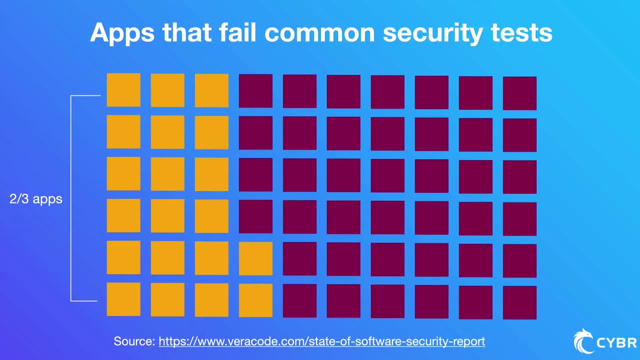 meaning that they tested positive with the automated tests, but in reality, if a human being checked them, they wouldn't actually be vulnerabilities. But on the flip side, these stats also don't account for zero-day vulnerabilities. A zero-day vulnerability is unknown or unaddressed. 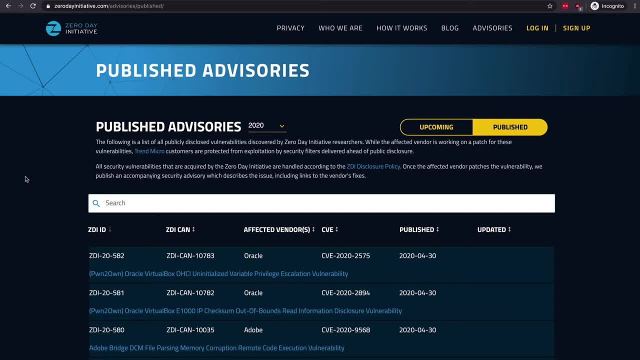 so, for example, if you're looking to exploit an application and you find a vulnerability in that application that no one else has, then you can continue to exploit that vulnerability until it is addressed. As a side note, zero-day vulnerabilities are exploited all the time. 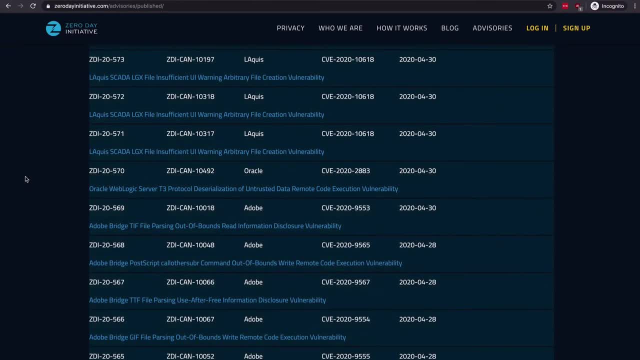 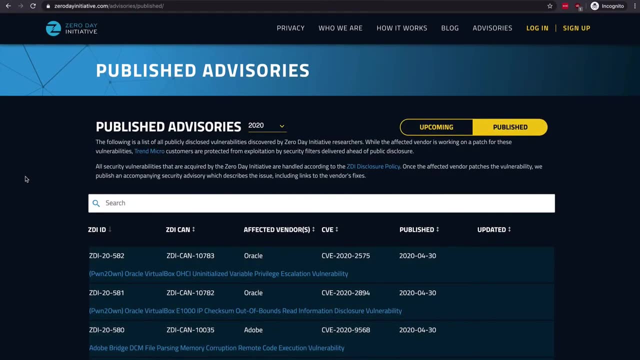 and there's a black market for them, since they can be sold and, depending on the vulnerability, it could be sold for a serious amount of money. However, in more recent years, organizations have started to offer bug bounty programs in order to reward the findings of zero-day vulnerabilities. 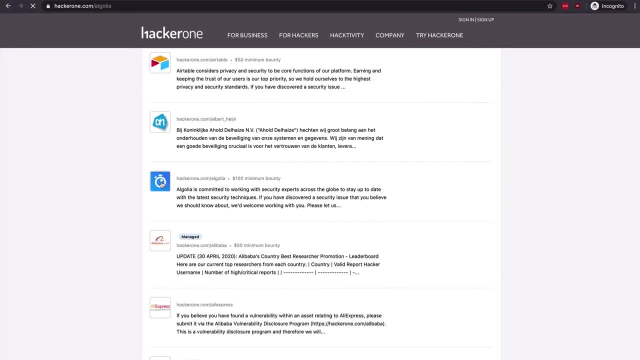 to help avoid having these sold or even exploited, and so you can continue to exploit those vulnerabilities. However, in more recent years, organizations have started to offer bug bounty programs and instead to give the organizations a chance to fix them before they become public knowledge. 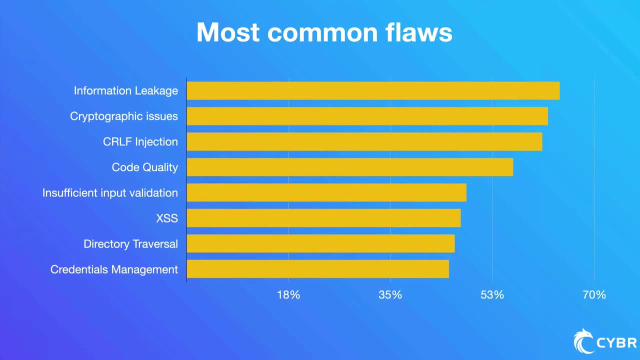 But going back to the Veracode report, the most common types of flaws that they found were information leakage, cryptographic issues, CRLF injections, code quality, insufficient input validation, cross-site scripting, directory traversal and credentials management. Now we're going to explore some of these in a bit more detail in the next lesson. 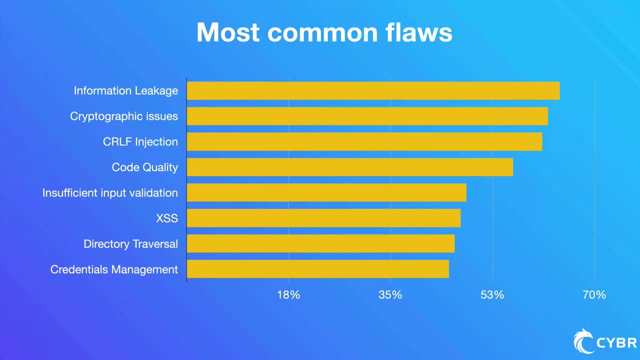 but let's talk about the top three, just so we can make sure that we understand what they are. Information leakage refers to an application revealing sensitive data, such as technical details of an application, developer comments, environments or user-specific data. That data can then be used by an attacker to exploit the target application network. 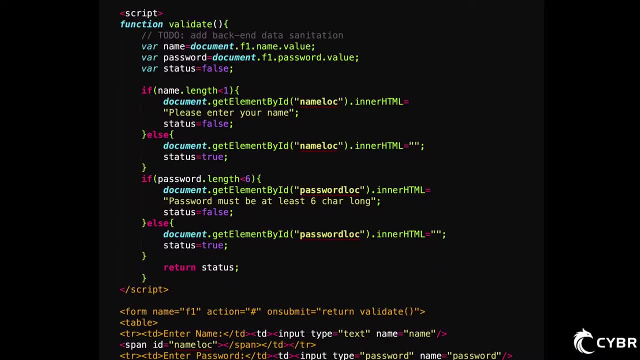 or even users. A basic example of this would be if a developer had added HTML or script comments to their code that contained sensitive information, and then they never removed it before it went to production. So in this case we can see that the validate function in JavaScript. 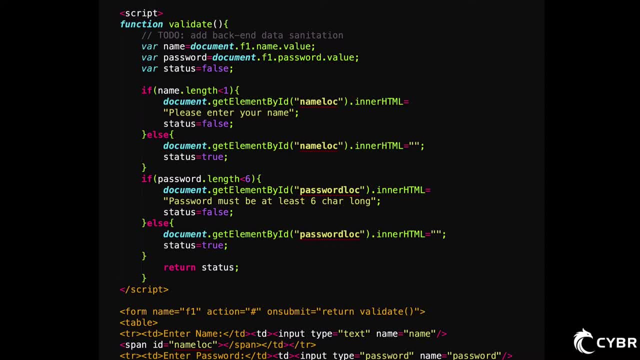 has a comment that says to do add backend data sanitation. So if I'm an attacker, I may look at this, and I may assume that the developers never went back and added data sanitation, or they haven't gotten to it yet, And so that means that I may have a 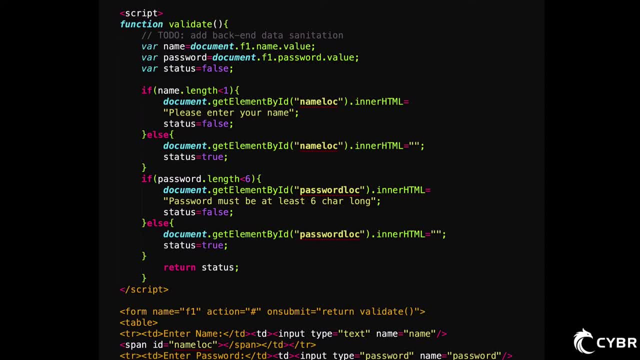 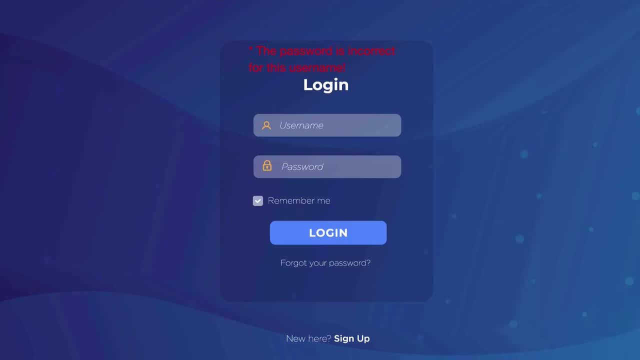 potential entry point. Another example of this would be improper application or server configurations or differences in page responses, Valid versus invalid data, And if you've ever accessed a broken webpage that released information about the database, web servers or whatever else, then that could be considered information. 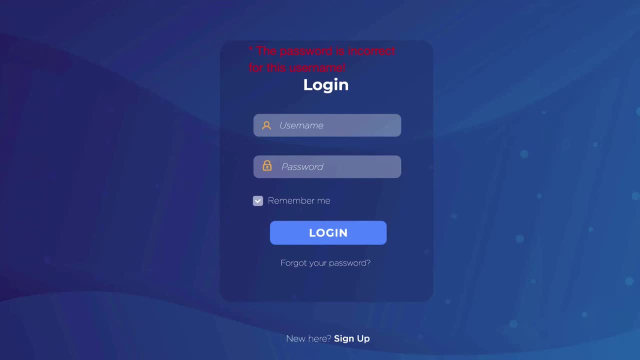 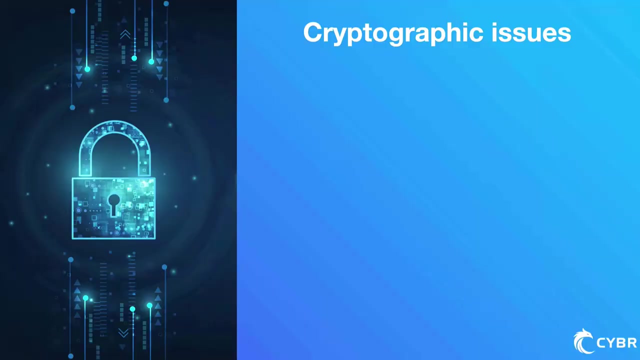 leakage. So information leakage by itself may not be a breach in security, but it can give crucial information to an attacker that can then be used to exploit your application or its infrastructure. The second one was cryptographic issues, And cryptographic issues can be problems related to encrypting the wrong data. 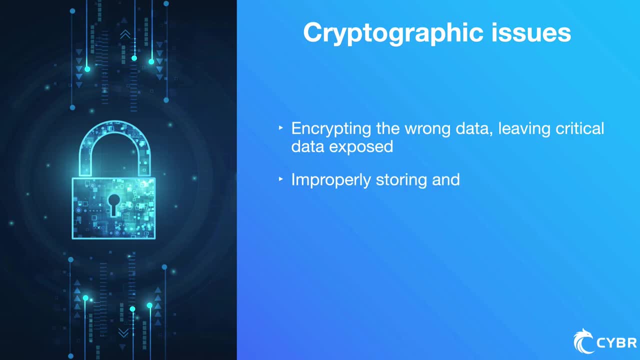 critical data exposed Improperly storing and managing crypto keys. So perhaps you're storing those in a GitHub repository and so other people have access to those keys, Or maybe they're even publicly displayed because they weren't private repositories And also using bad algorithms, or 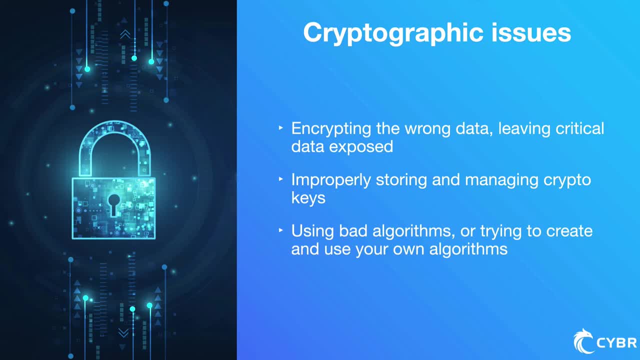 trying to create and use your own algorithms Unless you really, really, really know what you're doing. don't try to create your own. That doesn't make any sense. There are others out there that are working very well, So stick to those. don't try to create your own. 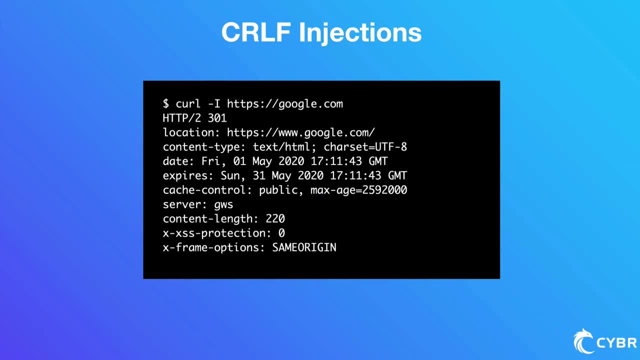 Next we have CRLF injections, and these were the third most found flaws. Now these can be very nasty attacks, because the HTTP protocol uses what's called CRLF character sequences to signify where one header ends and another header begins. It also signifies where headers 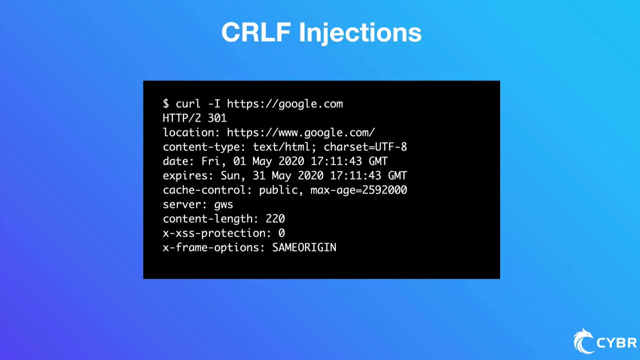 end and the website content begins. So in our example here, these are headers returns by Google. They have the location, the fact that it's returning via HTTP2, the content type, the date, the cache controls the server that's returning it, the content length. 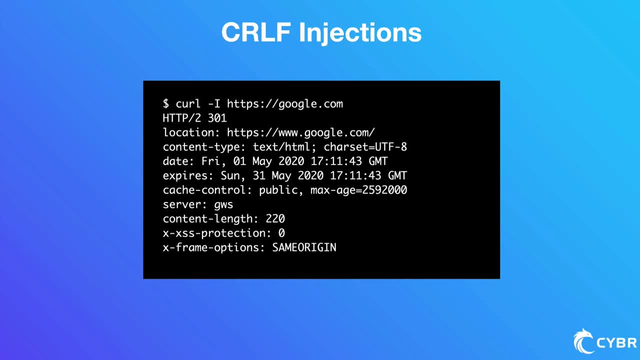 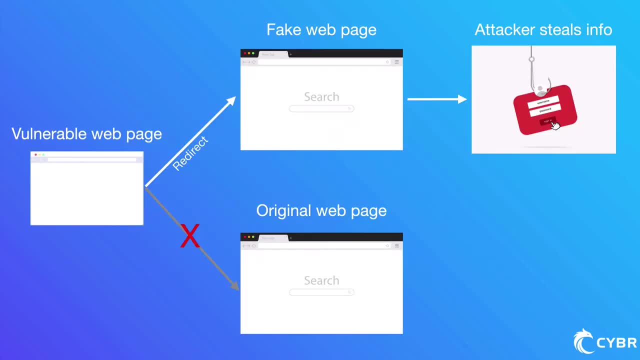 and cross-site scripting protection flag, X frame options flag and things like that. There are many more, but these are just the ones that curl return to us. But if attackers can insert their own CRLF, they can do all kinds of things. 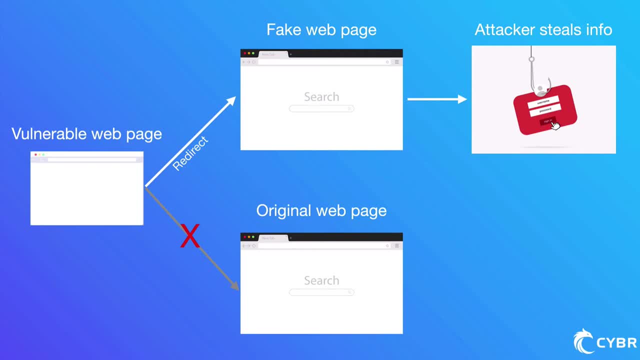 including redirecting users to a different website, where they might create an identical version of your webpage and use it for phishing, And they could also run unwanted commands on servers or do a whole lot of other things. And something that we haven't really talked about much to this point is chaining attacks together, So we've talked about cross-site. 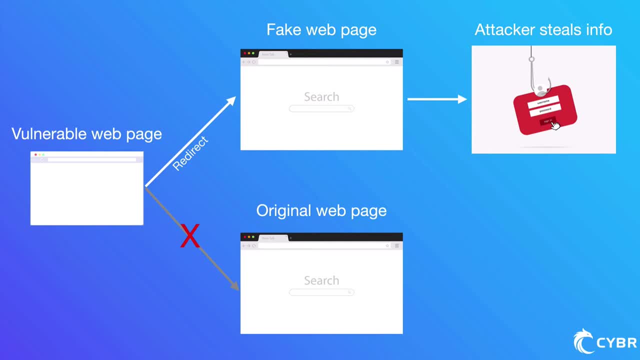 scripting attacks a little bit, but what if an attacker uses CRLF to inject JavaScript code? In this case, they're chaining a CRLF injection with cross-site scripting. This is something that you would see a lot in the real world, where one attacker may not use one specific attack method. 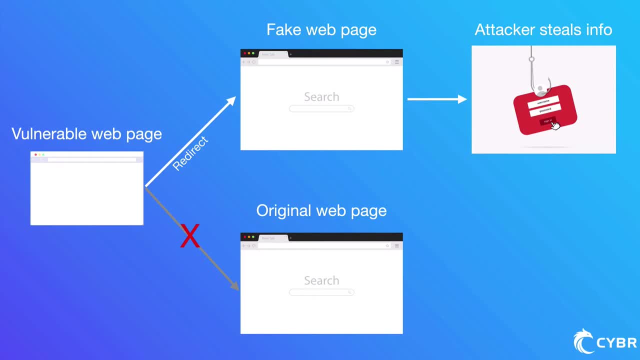 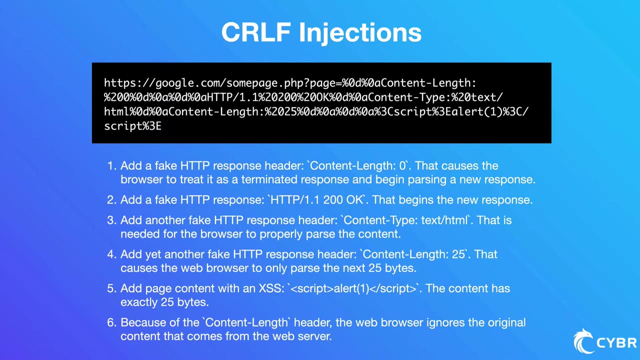 they might use one attack method to gain access to something else, which then opens it up to other attack methods, And that's called chaining attacks. So let's take a look at what a CRLF injection might look like. First, we add a fake HTTP response header of content length 0. And I 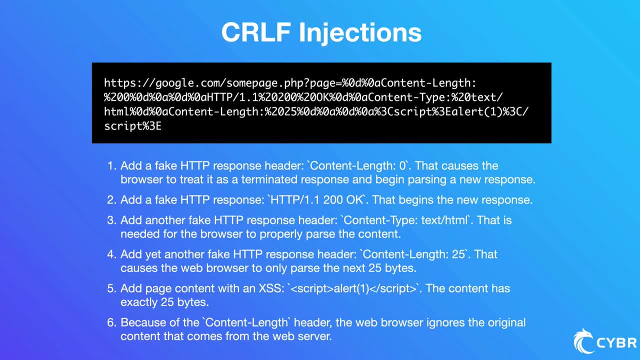 know it's hard to see because of all the encoding, but in this case we cause the browser to treat it as a terminated response and begin parsing a new response, because the content length is 0. Then we add a fake HTTP response with HTTP 200. OK, and that begins a new response After that. 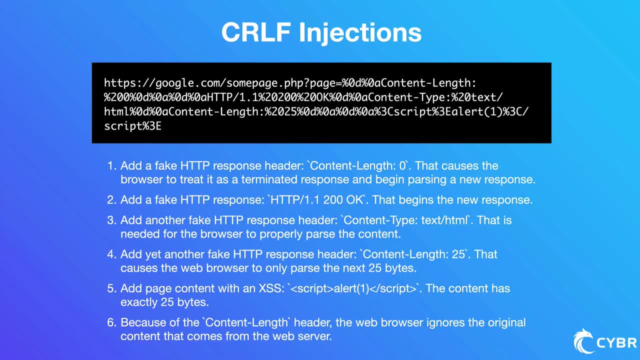 we add another fake HTTP response header of content type, text and HTML. that's needed so that the browser knows how to properly parse the content. And then we add another fake HTTP response header that says content length: 25.. So in this case the browser is expecting 25,. 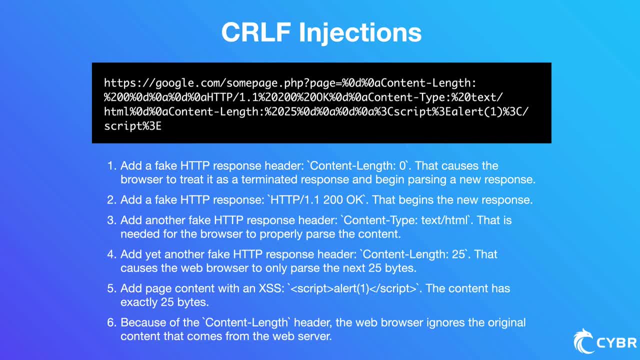 and those 25 bytes are the cross-site scripting attack. that, in this case, is very basic. It just creates an alert box And in this very, very basic example, just because of that first content length header that we injected, the web browser ignores the original content that comes from the web. 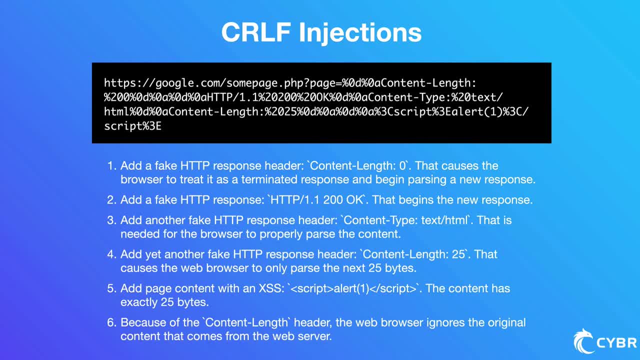 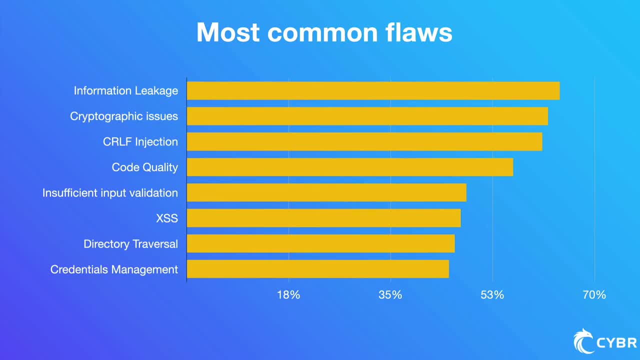 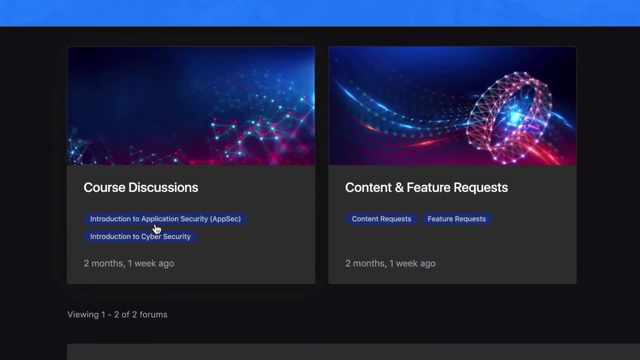 server and instead displays our content that we injected in this HTTP URL. So go ahead and research the other varicode, And if you can't find a good explanation or if you'd like clarification, please use our forums and either myself or someone from our community will be able to help. We're also going to look. 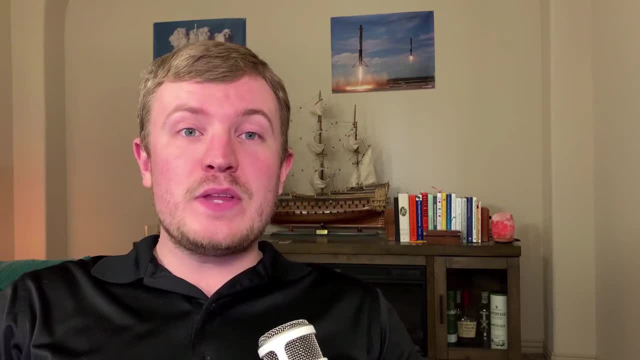 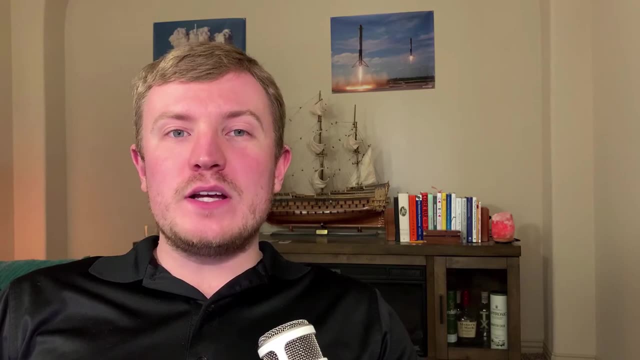 at more common vulnerabilities and attacks in the next lesson, including examples and prevention methods. Looking at reports from prior lessons, we can start to see a pattern in the types of vulnerabilities that can be exploited and which ones are the most common. Organizations like OWASP. 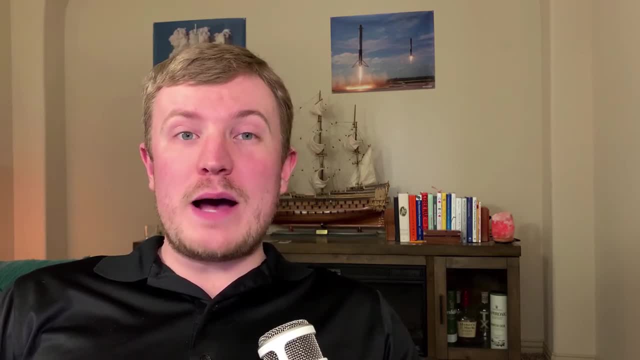 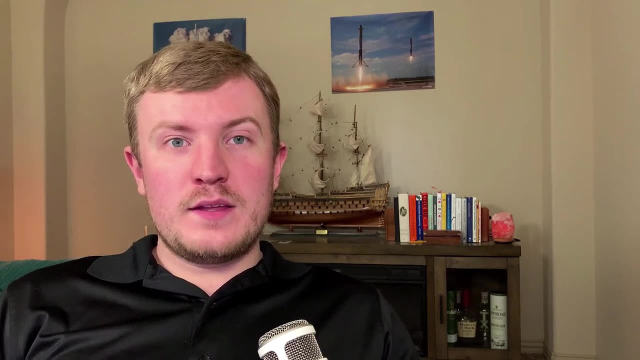 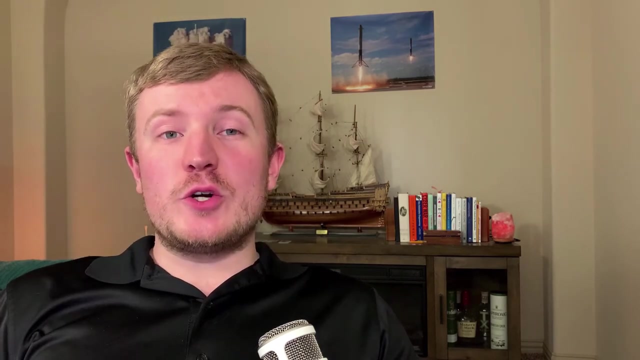 SANS and others have created lists of the top web application security risks so that developers and organizations from around the world can work to minimize these risks, Because we have to understand how our applications can become attacked in order to create the most effective defenses. So let's take a look at the OWASP top. 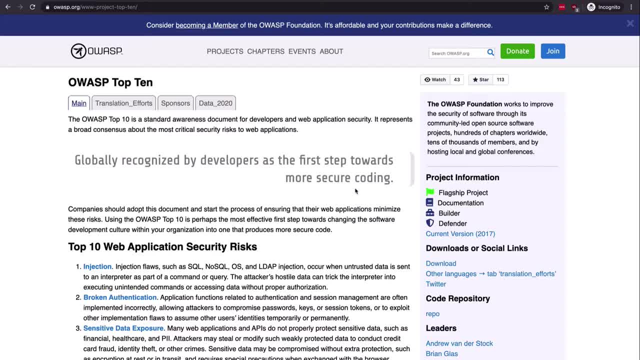 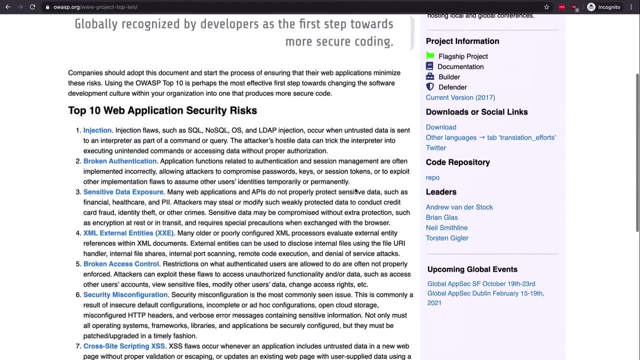 10 web application security lists so you can see what I mean. Keep in mind there are other lists, like the SANS list and other ones out there, but we'll be focusing on the OWASP top 10.. The top 10 web application security risks are: 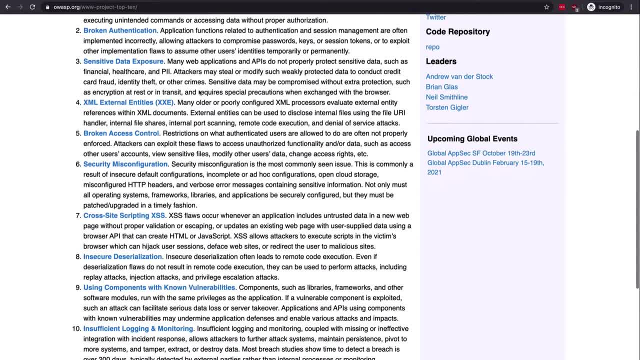 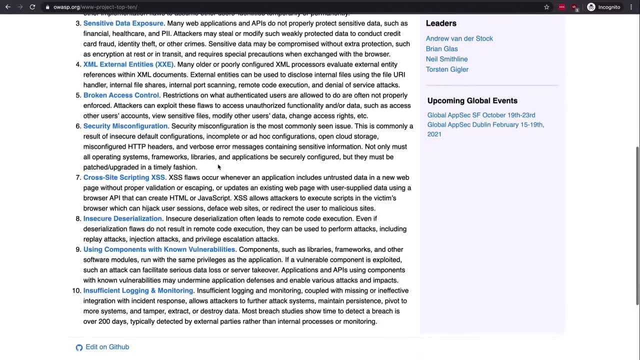 number one: injections, broken authentication, sensitive data exposure, XML external entities or XXEs. broken access control, security misconfiguration, cross-site scripting or XSS, insecure deserialization and using components with known vulnerabilities and, last but not least, insufficient logging and monitoring. Some of these should already 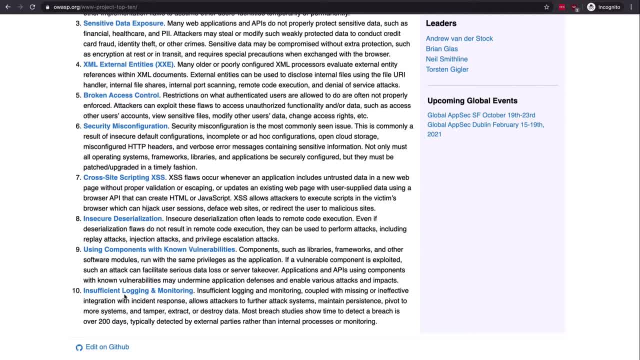 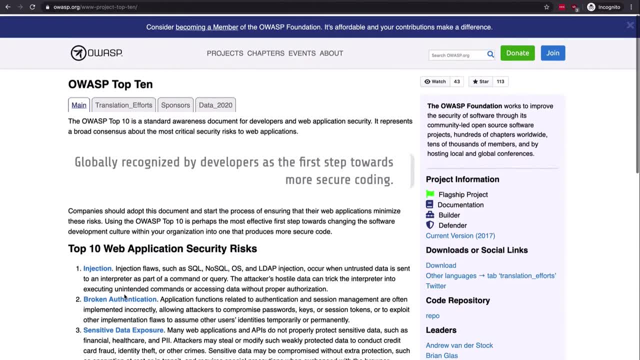 look familiar because they were covered in the OWASP proactive controls list that we reviewed in another lesson. So let's take a look at the OWASP top 10 security risks, But this list goes into much more detail about each security risk. Now keep in mind that this list is from 2017,, however, OWASP is planning on collecting data. 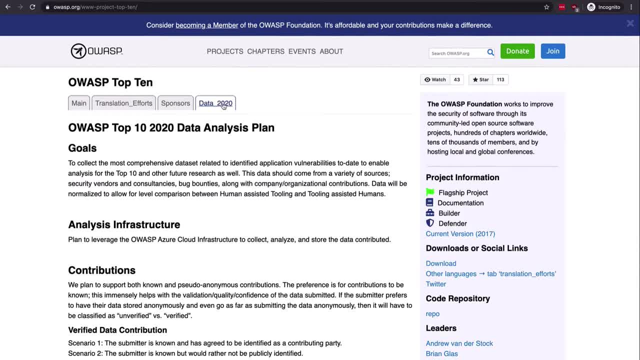 in 2020 to see what has changed since then, and you can see more information about that on this tab labeled data 2020.. So, while this is a great starting point for us, we can't just rely on this list or other lists As application security engineers. 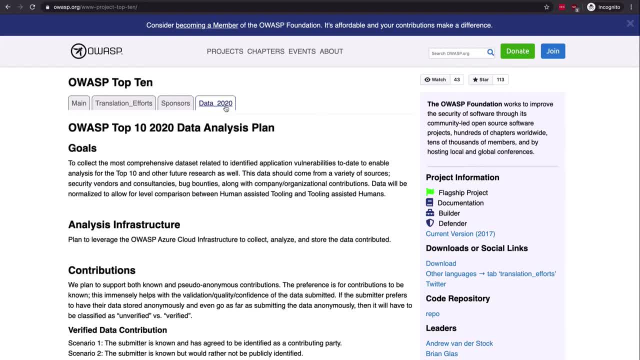 we have to constantly look out for what's happening in the industry and we can't just rely on one or two top 10 lists. I'm just throwing that out there as a disclaimer. Don't get overwhelmed, but also don't think it just stops here. In any case, clicking on each of these, 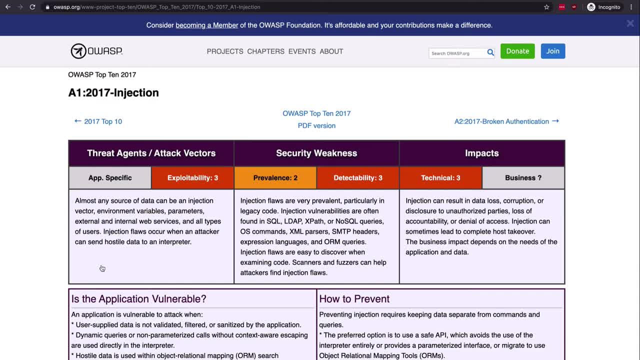 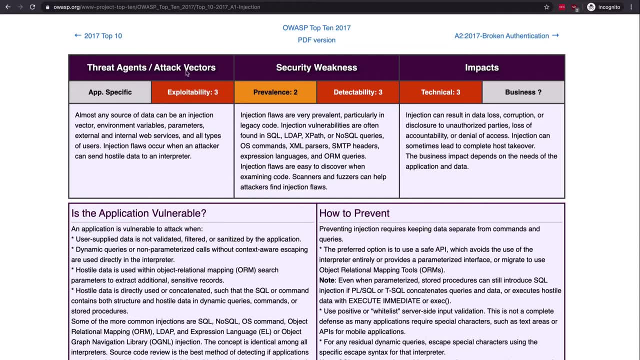 brings up their individual cards, For example, if we click on the injection one, here's what we can see At the very top, we'll see something familiar to us. We have threat agents and attack vectors, we have security weaknesses and we have the impacts. 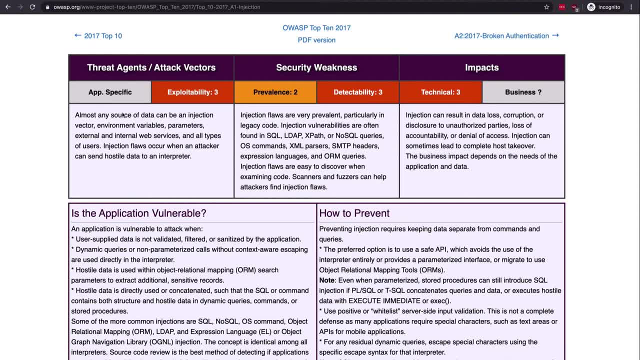 In the threat agents and attack vectors. they include factors that are specific to our application, which only us can determine, And then we also look at a rating for exploitability. The security weaknesses show the prevalence as well as detectability And then under impact. 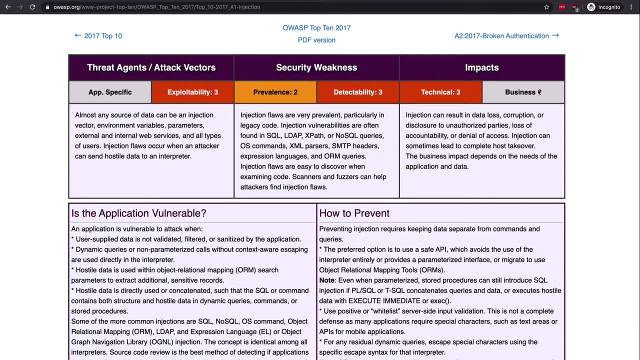 rating. we have the technical impact and the business impact, which is also something that only us can determine. Now, of course, these are specific to your application, as we saw in the threat modeling lesson, but OWASP aims to give us a general idea for each of these. 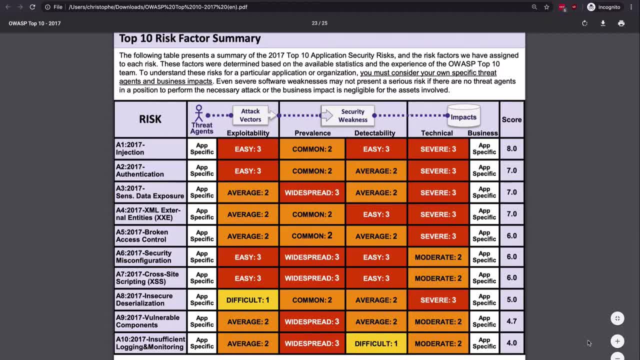 And there is also a PDF version. In the PDF version they explain how they calculated these and they'll also show them all in one table so that we can see how they ordered them in terms of highest to lowest risk. So if you want more information on that, please check out the PDF document. 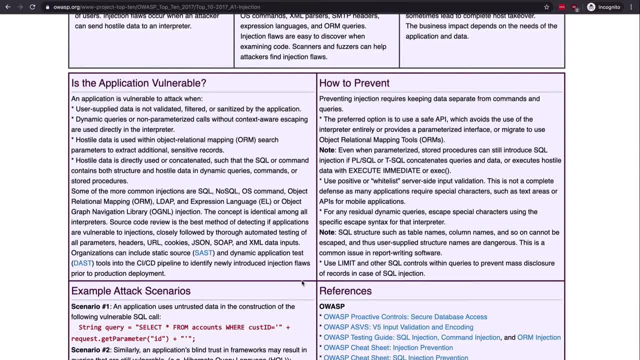 Next, we get guidance on how we can determine whether our application is vulnerable to this form of attack. So, in the case of injections such as SQL, or SQL injections, as you may have heard of them referred to instead, our application is vulnerable if user-supplied data is not validated, filtered or sanitized by the application. 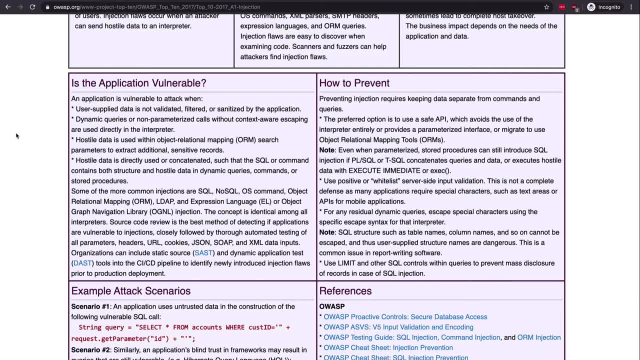 This is a recurring theme that you will hear over and over again. but never, ever trust user data. You have to assume that the user-inputted data is malicious. And they show some examples of what these attacks look like, but let me go ahead and show you in a little bit more detail. 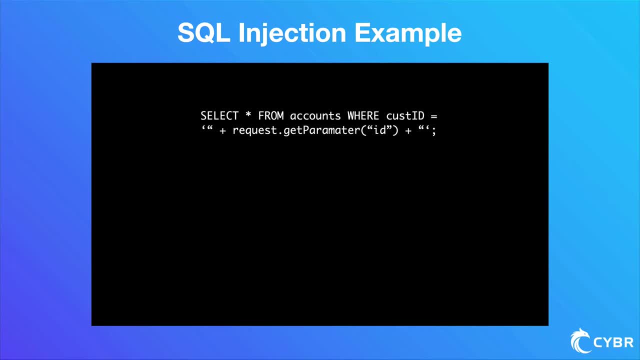 Let's say that we have a SQL query that says select everything from the accounts table where the customer ID equals a user-inputted ID. In this case, the attacker could modify the ID parameter to instead be a SQL injection, which would look something like this: 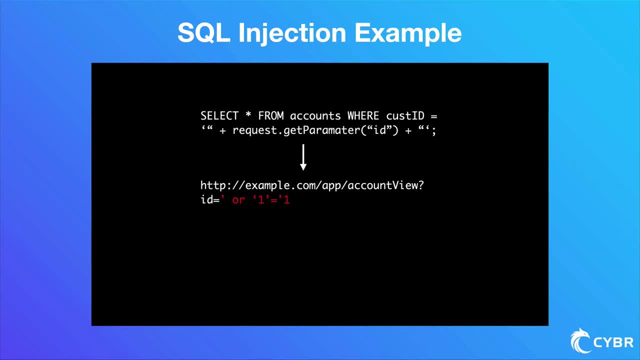 The red part of the query has a single quote, then a space, then OR, then another space, then a 1 in single quotes equals single quote 1.. Now this looks pretty weird, especially if you've never seen a SQL injection before, But what will happen is because of the lowercase i. 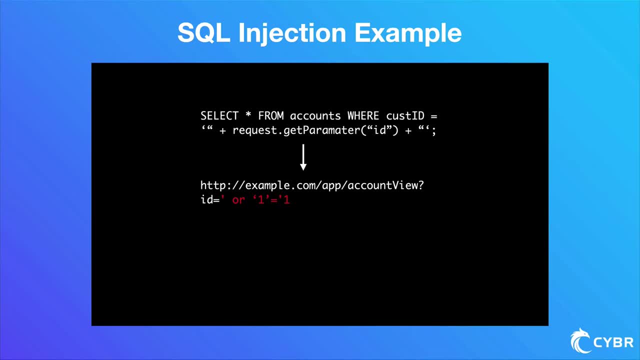 but what will happen is because of the lowercase i. but what will happen is because of the lowercase i. this URL is structured this way. our code would grab that query and this is what the SQL query would look like. Again, we have to select everything from the accounts table where customer ID equals. 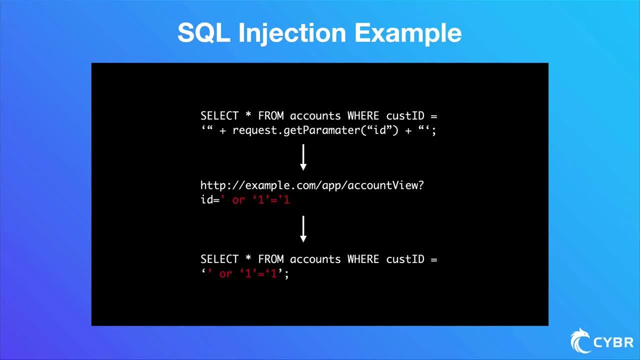 that data inputted by the user. So what's going on here? Well, with the first quote that's in red here, we're actually telling the SQL interpreter to run an or statement. So we're saying the customer ID equals blank, or one equals one, and one always equals one, which means that this will always 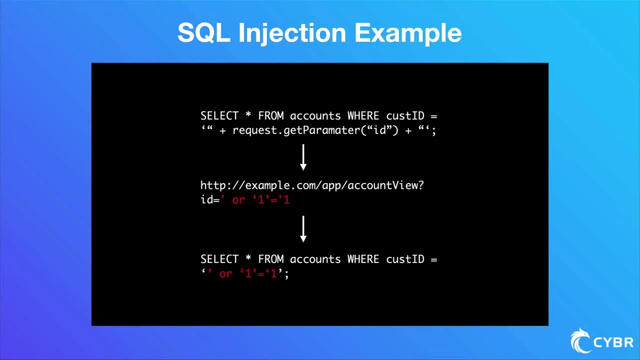 return true. So in this case, the database would actually return every single customer ID and since we're grabbing all of the rows from that accounts table for every single customer ID, if we have, let's say, a million different customers, this query would theoretically return every single bit of information. 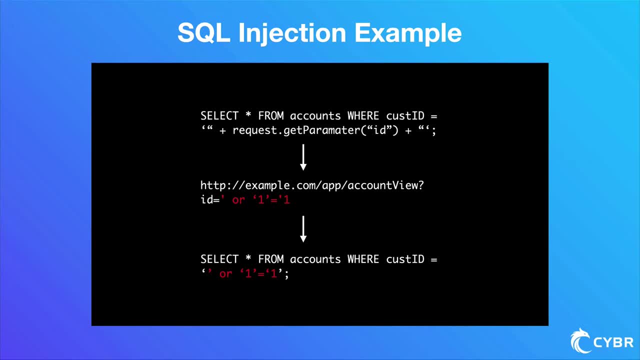 in that accounts table for literally all of those million customers. Obviously big problem, and that's one way that you end up with your username, email or passwords on the black market for sale. The other thing is, injections could also be used to modify or delete data, which could cause even 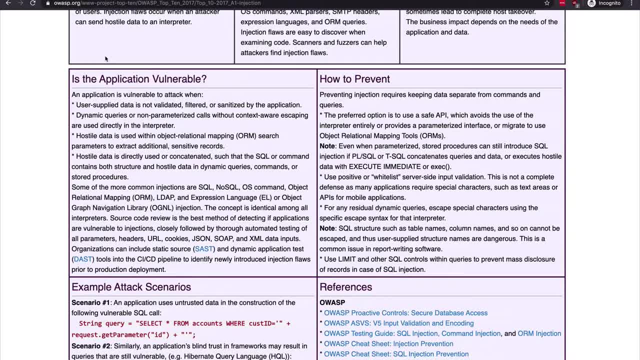 more harm, especially if you don't have proper backups. So, to defend against this type of attack, OWASP specifies ways of preventing them. For example, we have to always assume that any user supplied data is always going to be dangerous, as I mentioned earlier, and so we have to use techniques. 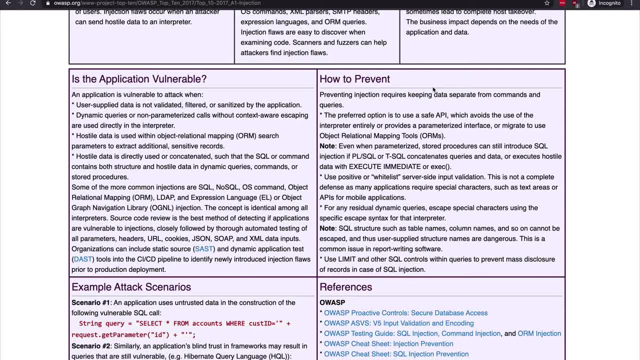 to validate, filter and sanitize, But thankfully, most frameworks and languages will contain methods that do this on our behalf, especially if they're modern. We just have to make sure that they're properly being used, because that may not be the default or it may not be what we see on an online tutorial, So if we just copy, 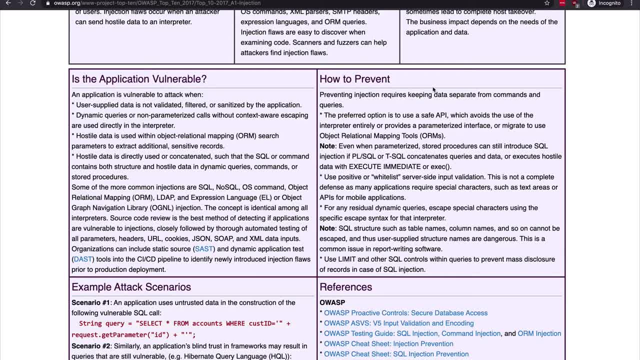 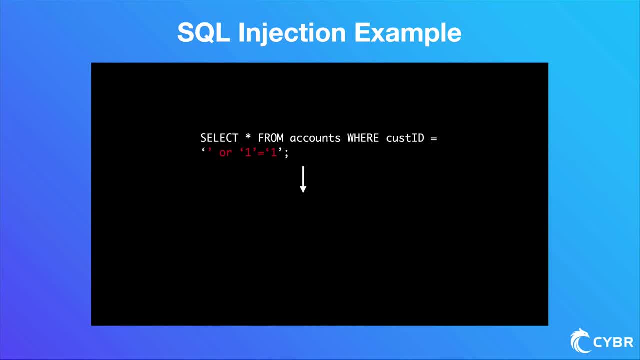 and paste that code without checking it, we could be introducing that vulnerability. So, going back to our SQL injection example from just earlier, a method that we could use to clean up user inputs would escape the single quotes in order to make that information available. So if we were to 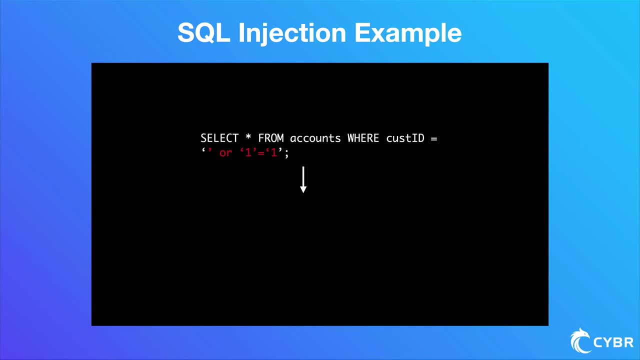 run a simple single quote, we can do that in a single query, So if we have that exact same query instead. in this case, after all the data sanitation, this is what it would look like. We're putting a backslash in front of every single user inputted single quote. What this does is it turns it into 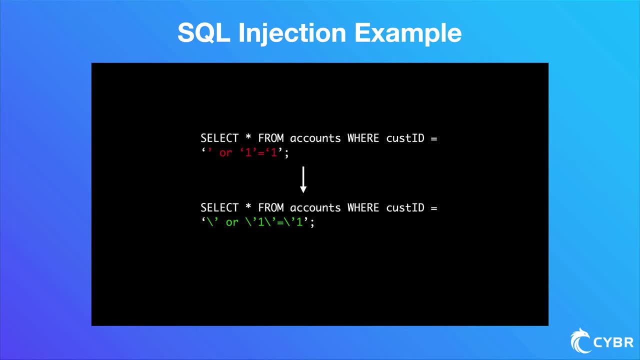 a string instead of running that or statement. So now we're not escaping. we're not looking at customer id equals blank or one equals one. we're looking at an entire string, or at least one string in one string least, that's the way that the database engine would interpret the statement. so now we've turned. 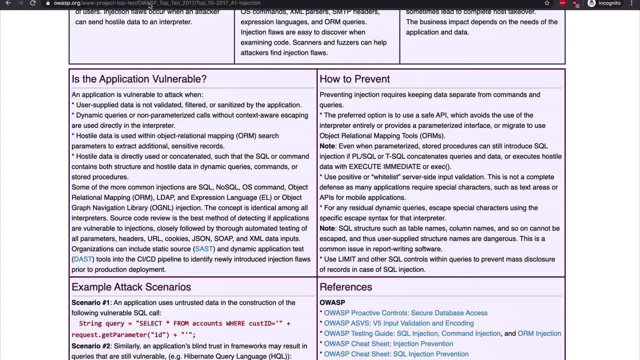 that injection into a harmless string. there are other ways of also limiting the impact of a successful attack. so we can add multiple different layers of defense and if that first or second layer of defense fails, we can limit how many records are being returned with a limit. sql. 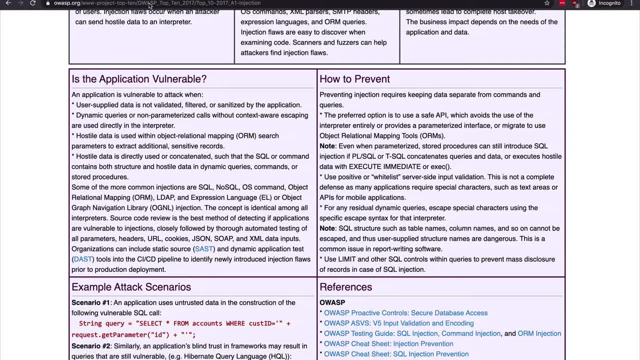 statement, for example. so even if that one equals one is always true- we could limit the customer records return to just one, because if you're looking at an account page, there's really no reason why you would want to see more than one account returned, unless it's an organization or 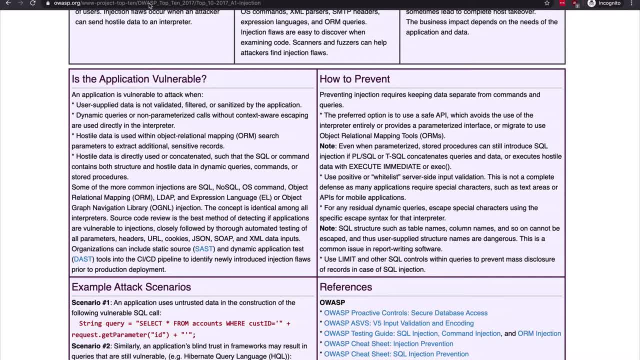 something like that. but if it's an individual account, there's no reason that would happen, so your sql statement should just have a limit of one. the problem with that is there are injections that can bypass that limit statement, so this is really a fail-safe as a last resort, but it's not. 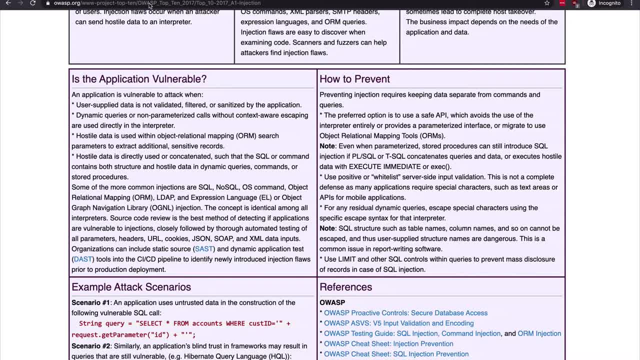 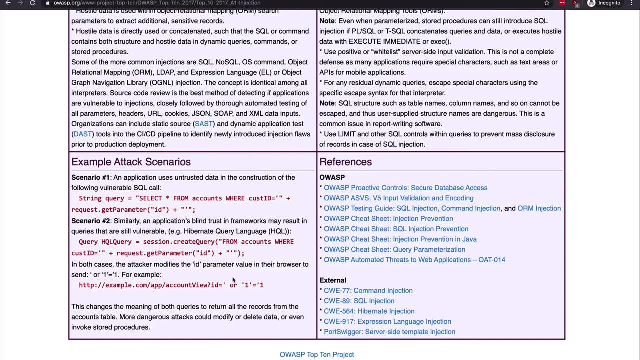 something to use by itself. it's something to use in addition to other techniques. as i said and as you can see here, there are other example attack scenarios, so we looked at one of these in other pages. there may be multiple different types of examples for the different 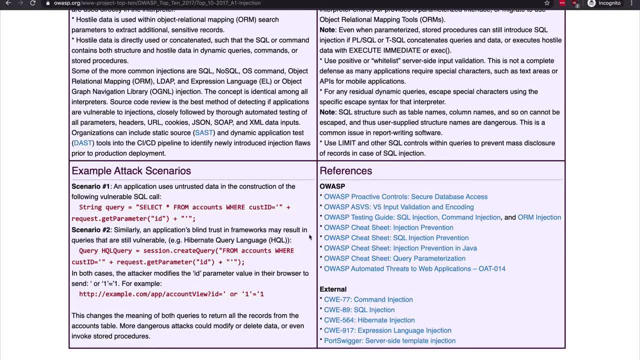 attacks, which is very helpful, and then, of course, there's a ton of different amazing references that OWASP has put together for us. there's some references from OWASP, but they also include references that are external, so we can take a look at those. so sql injections are really nasty. 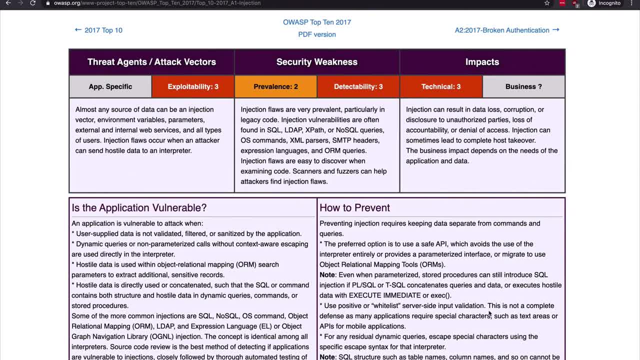 attacks, and the problem is they're still being used fairly frequently, and they're still being used frequently today, for example. some fairly recent and high-profile examples of sql injection attacks include companies like target yahoo, zappos, equifax, epic games linkedin, sony and many others. 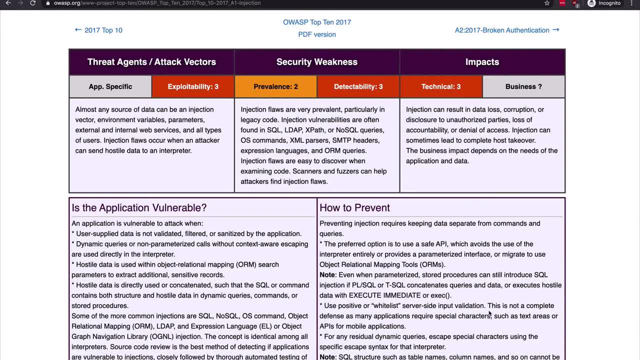 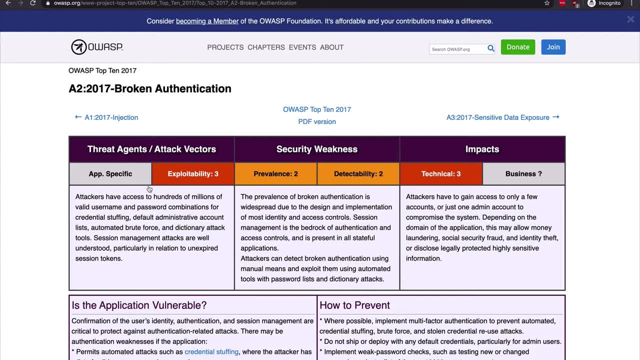 so these types of attacks are still definitely being used. the second vulnerability that we'll look at today is broken authentication. because so many applications have been compromised over the years, username and password lists have become very easy to get a hold of. if improper authentication is used for an application, attackers can use those lists to do credential stuffing attacks. 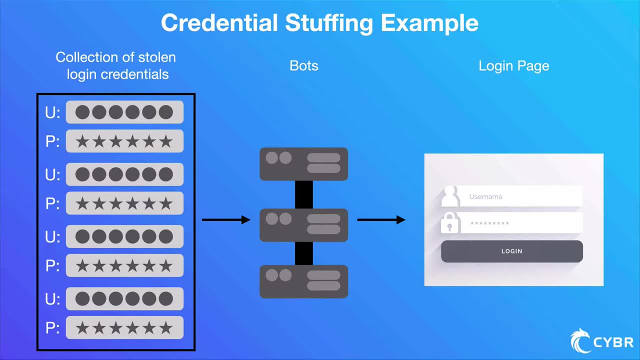 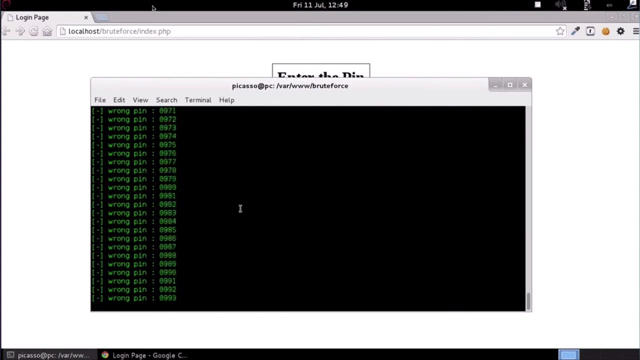 which attempt the username and password combinations of millions of records to see if any of them work on your application. other attacks try to use default username and password combinations, or you can have automated brute force attacks which try millions of passwords to see if any of them work, or dictionary attacks that create combinations using words in the dictionary. 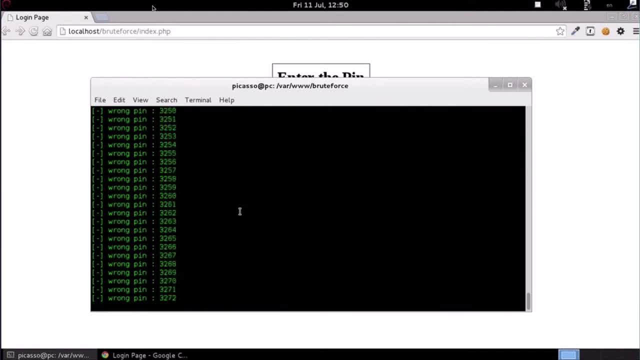 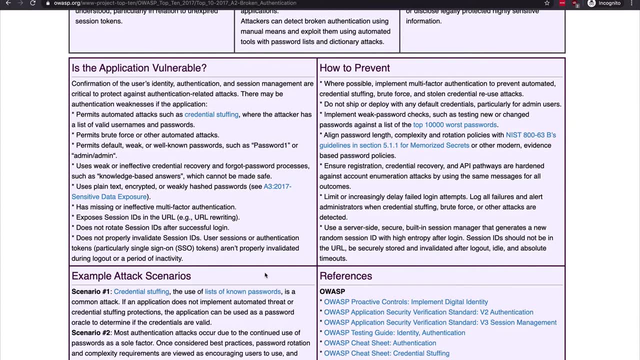 and all it takes is one admin or high value account to do that, and you can do that with sql injection to be compromised for authentication attacks to be worth the effort, and in this case, an application is vulnerable to this type of attack if it allows automated attacks. 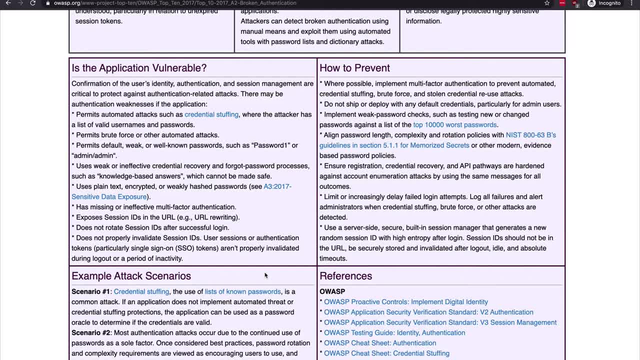 or if it allows brute force attacks, default, weak or well-known passwords, such as password one or admin admin combinations, or if it uses weak or an ineffective credential recovery and forgot password processes. so even if your login methods are super solid but your forgot password process is weak, that could be used to hijack an account other ways that your application 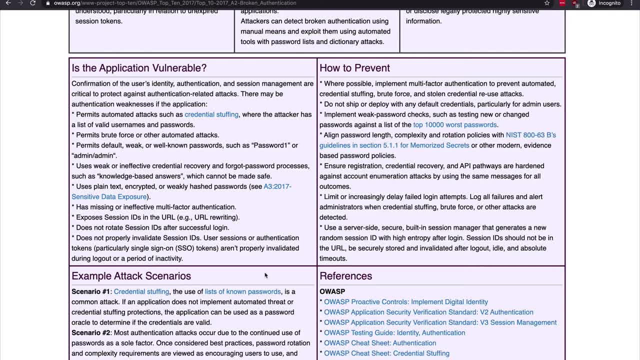 would be vulnerable to this is if you use plain text passwords or weakly encrypted and hash passwords, or if you have missing or ineffective multi-factor authentication, if you expose session ids and urls which can be used for something called url rewriting, or an attacker can steal your session if it does not properly rotate session ids after successful login, or if 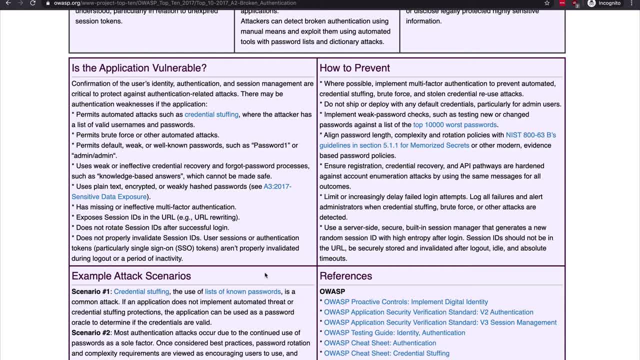 it does not properly validate session ids after logout or after inactivity. again, if you spent some time reviewing the proactive controls from a prior lesson, a lot of these should sound very familiar and the ways of preventing will also look familiar. but the overall recommendations here are to implement multi-factor authentication wherever possible. passwords alone are becoming 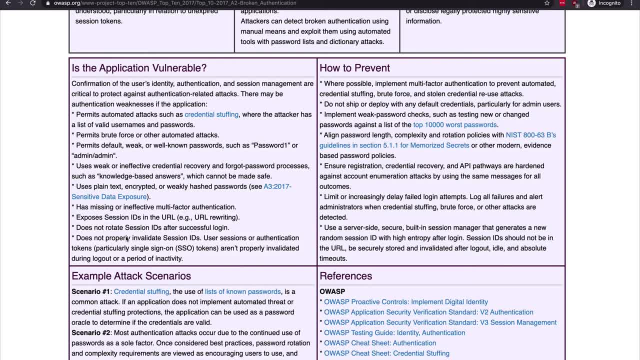 less and less secure when it comes to authentication, and adding another layer like multi-factor authentication makes it much more difficult to compromise accounts. also, don't ship or deploy with any default credentials. don't implement weak password checks, such as testing new or changed passwords against a list of the top 10,000 worst passwords. 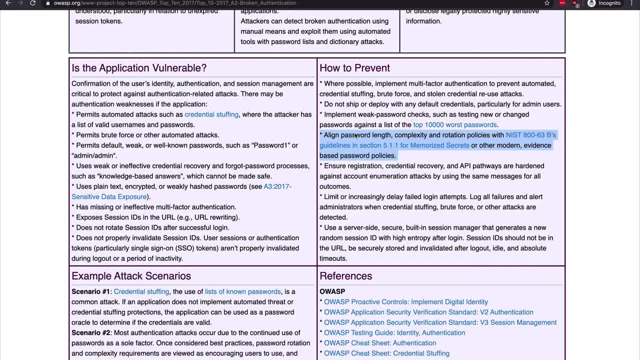 implementing weak password checks by enforcing a certain password length and by checking for common passwords. ensuring that the registration credential recovery and the general api pathways are hardened against enumeration attacks, where enumeration attacks consist of fining, finding patterns that can be exploited. for example, if you've ever seen a login form. 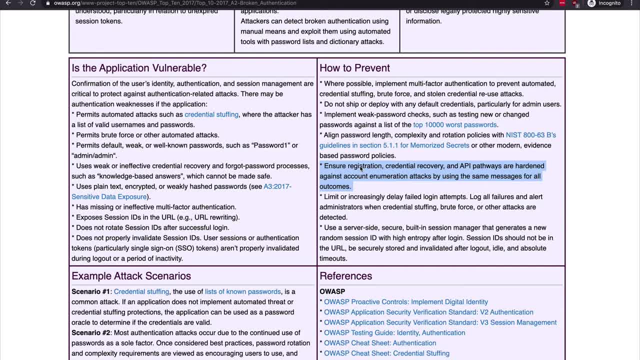 that tells you whether the username or the password are wrong, as in, your username is correct, but the password is incorrect. while these kinds of hints can be helpful to the users of the application, it's also helpful for the attackers, because now they know that they have a correct username and all they have to do is find the correct password, which. 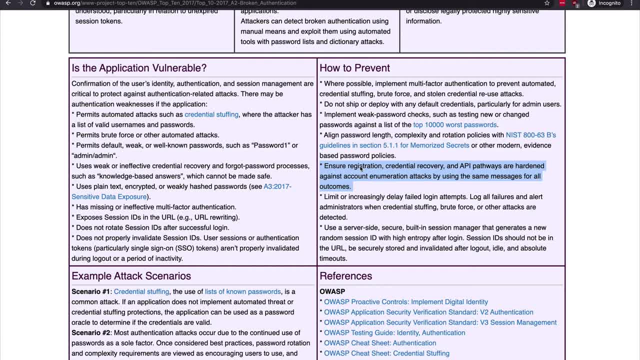 drastically reduces down computational time, because now they only have to guess one variable instead of two different variables. so having generic messages such as your username or password is incorrect prevents attackers from knowing whether they have a correct username or not. another important protection method is to limit or increasingly delay failed login attempts. 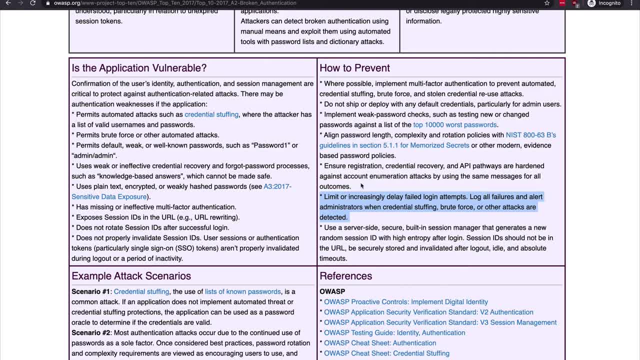 and then also log all the failures and alert administrators when there seems to be credential stuffing, brute force or other attacks happening. it frankly baffles me how many platforms still don't prevent brute force attacks on their login pages, because even wordpress, for example, at least at the time of this recording, does. 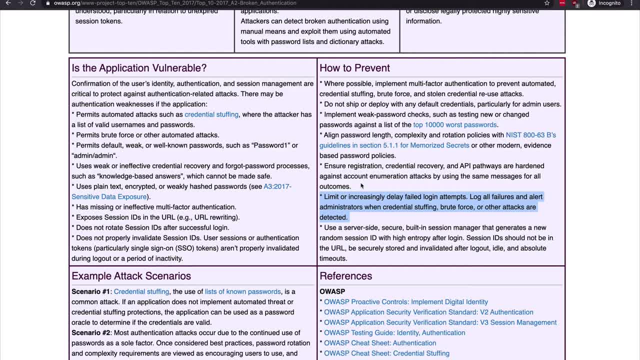 not prevent brute force attacks on fresh installations. you have to either code it yourself or you have to use plugins to turn this protection on. this means that attackers can try millions of combinations for username and passwords without anything preventing them. now there are, of course, other ways of preventing authentication attacks, but these are the common. 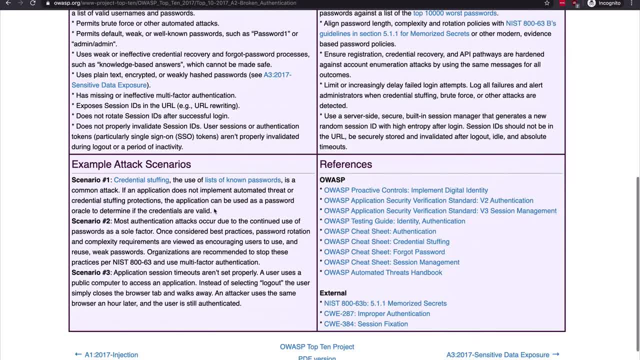 prevention methods. so go ahead and take a look at some of the example attack scenarios here and feel free to check out the references for more information. in talking about credential stuffing attacks, there was a fairly recent example with with the company called nest. you may remember in 2019 that some nest 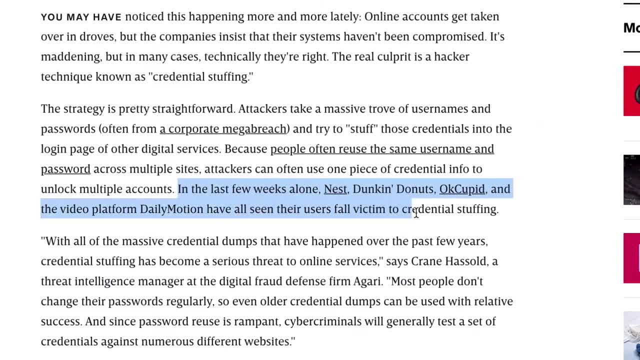 users were horrified when strangers started speaking to them through their nest cameras. one of the ways that the attackers were gaining access to these devices was by using credential stuffing attacks. so, in response to these issues, nest forced certain users to change their passwords if they were using compromised credentials. 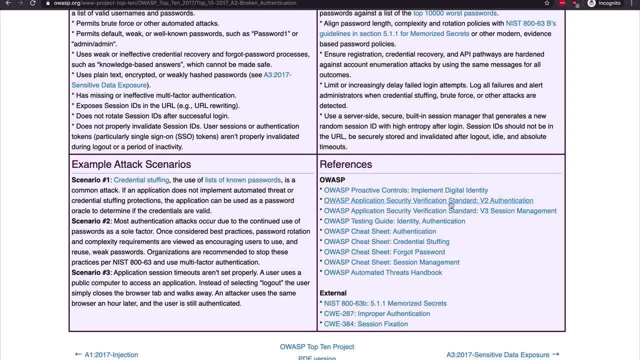 also as a quick reminder, you will see the application security verification standard being referenced and linked to in these documents, because many of the requirements we explored in prior lessons help prevent these types of attacks. we're simply looking at why those types of requirements are so important to have when working on applications. 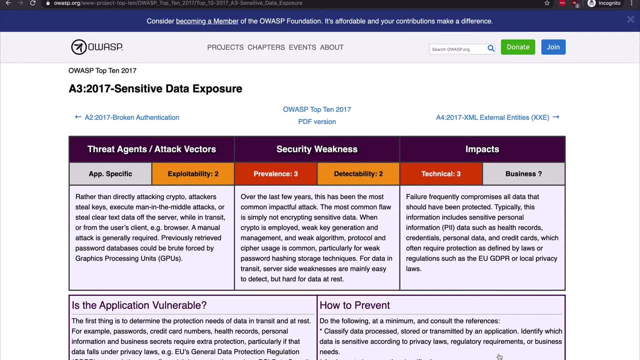 okay, so we've looked at a couple of the top 10 security risks so far, and there are still eight more as we complete this lesson. go ahead and review them, as we've been doing, and if you have any further questions, please use the forums for this course. otherwise i'll. 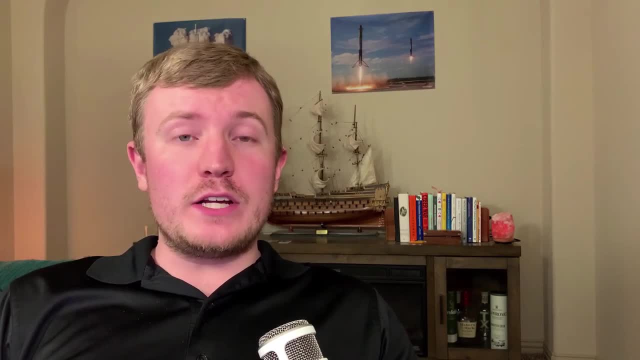 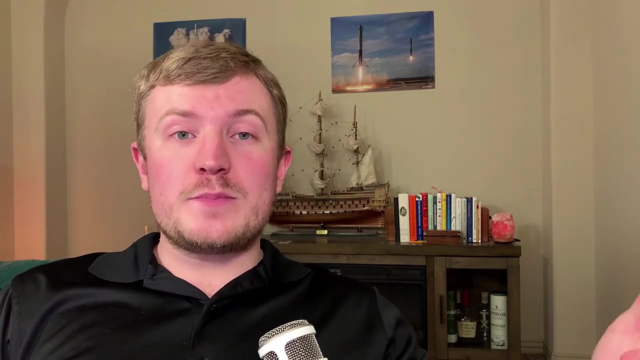 see you in the next lesson. type of attack that i want to include in this course is called a dos, or denial of service attack. you may have heard of it referred to as a ddos instead, which is simply a distributed denial of service attack, and while, at least up to this point, OWASP has not explicitly 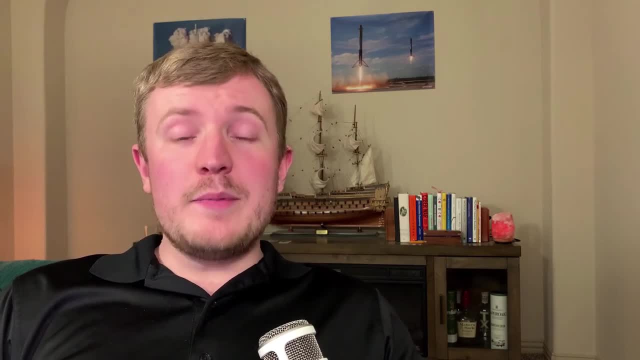 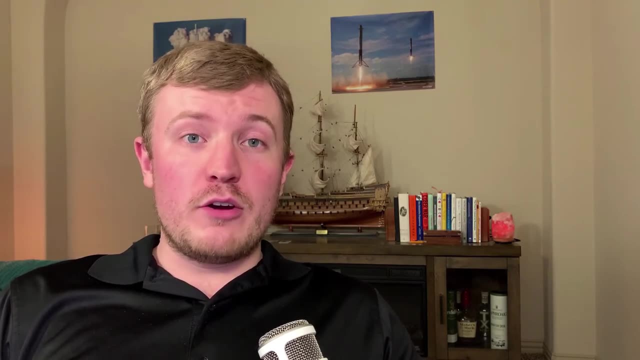 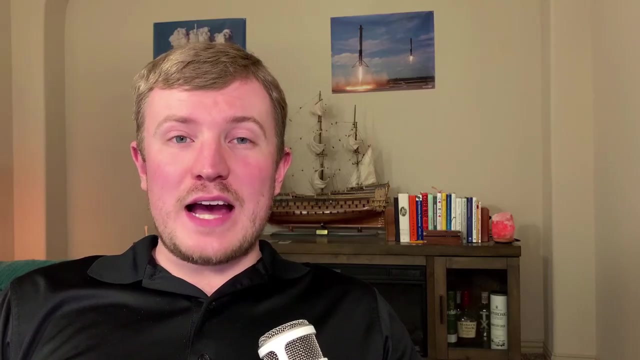 called out dos attacks in their top list that we've looked at. i'm including dos attacks because they're fairly common and not that difficult to do, so they've been an obvious choice for attackers for many, many years now. what can stop do's and don'ts? denial of service attacks are a tremendous problem because they 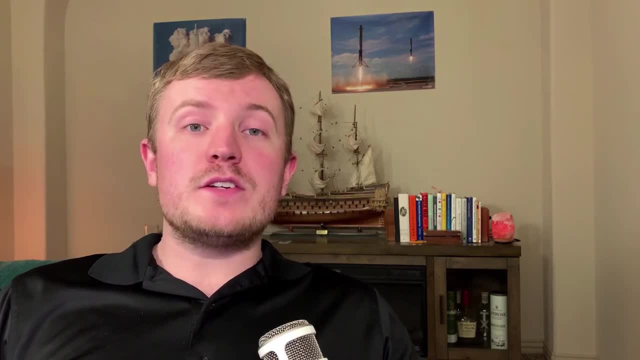 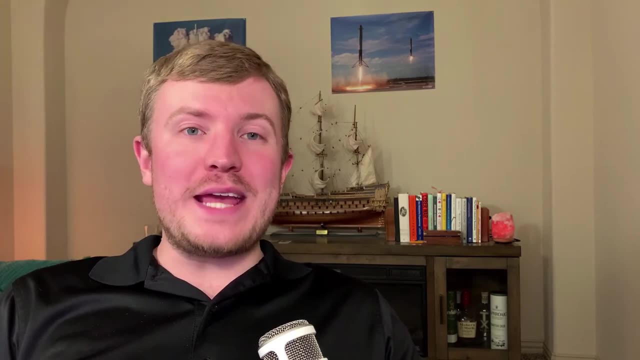 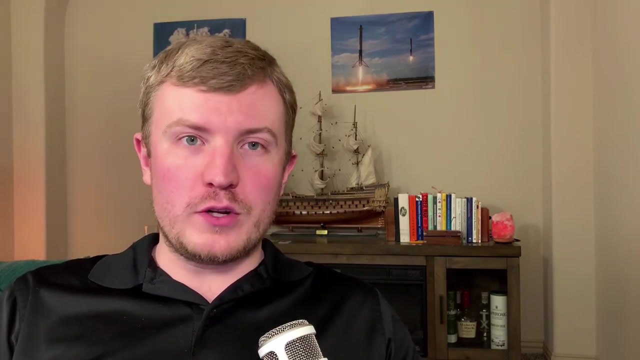 can cost a lot of money to organizations by causing disruptions to your applications and therefore causing disruptions to your customers, and it can also result in unwanted behaviors, like revealing sensitive information because your systems are malfunctioning, when they're crashing or just overloaded, and that can result in information leakage, which we've seen in. 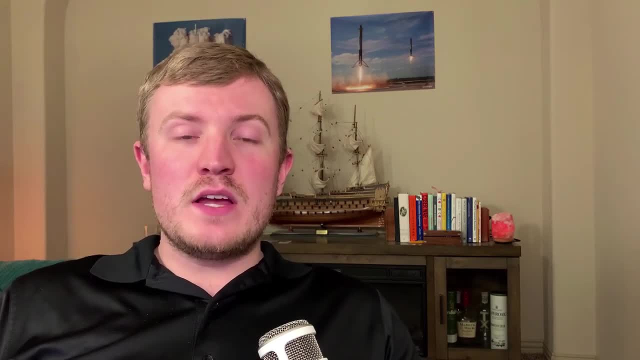 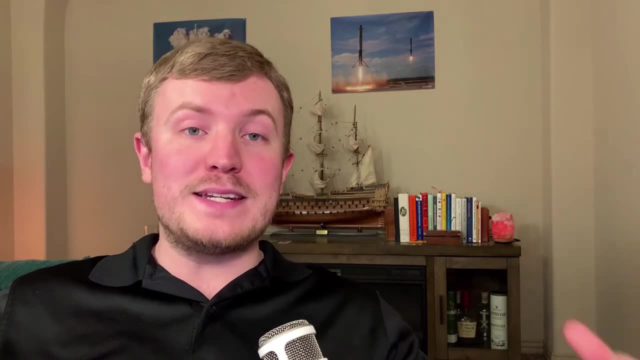 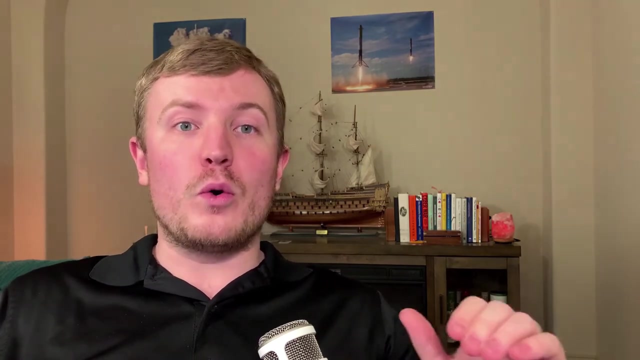 prior lessons. and the problem with denial of service attacks is they don't always have to do with a vulnerability in your code base. Instead, it could just be that the attack is so tremendous that it overwhelms the infrastructure powering your application. So, even if you haven't coded in any vulnerabilities or have any security issues, 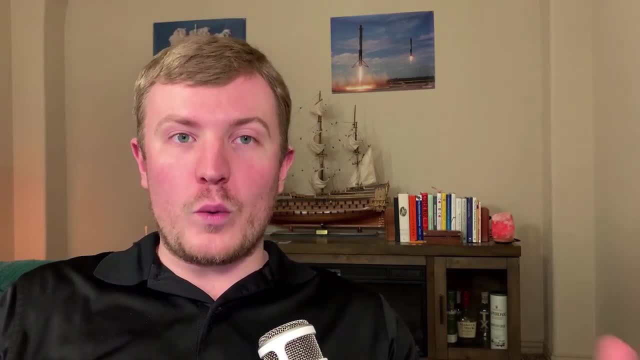 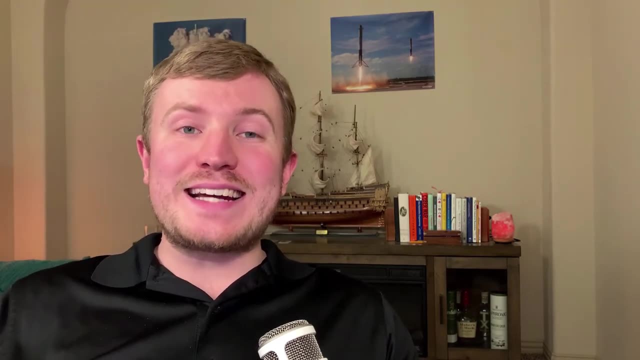 in the application itself. if there's an overload of requests and your infrastructure can't handle it, then it will bring your application to its knees. With that said, though, there are ways to protect against these types of attacks, and we're going to look at that in this lesson. 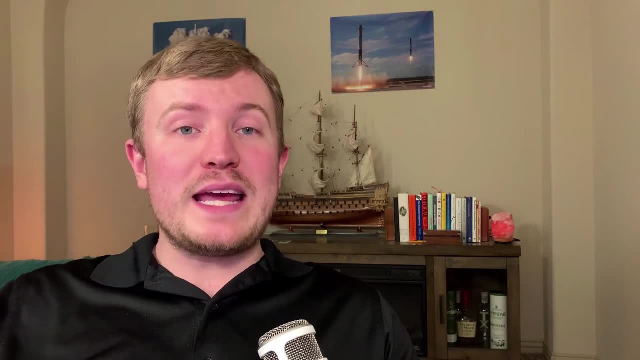 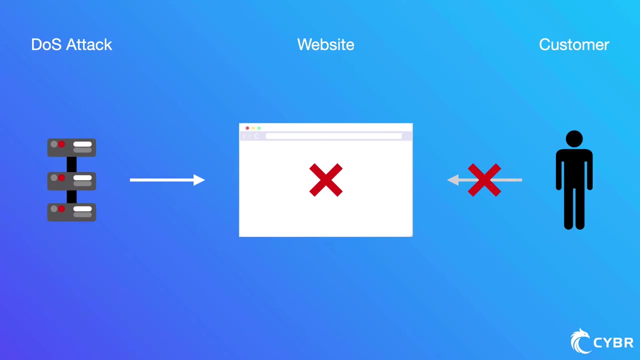 But first let's back up for a minute and let's talk a little bit more about what a DOS or DDoS attack is. The point of a denial of service attack is to deny service to legitimate users, and this could happen to websites, email or really any service that relies on computers. 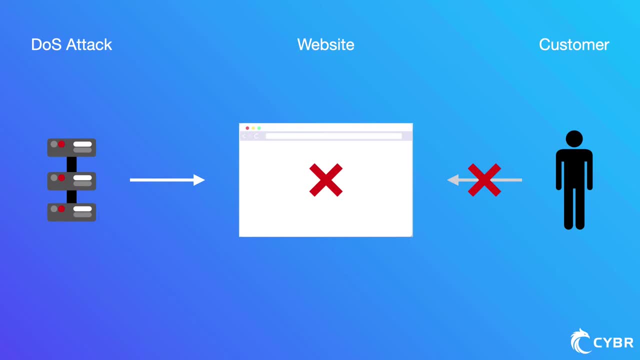 or a network, And an attack like this is accomplished by flooding the system with so much traffic that the underlying systems can't handle any more requests. A distributed denial of service attack is the same thing, except the attacker is using multiple different machines to attack the same target. The end result usually means a much larger attack. 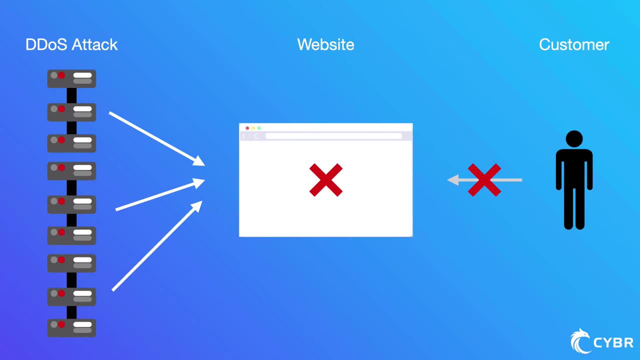 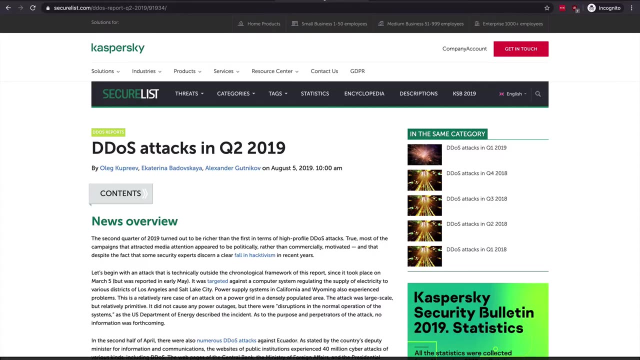 and a harder attack to defend against, because the requests are coming from so many different locations, so you can't just block one IP address. for example, Research from Kaspersky's secure list shows that in Q2 of 2019, there were more high profile DDoS attacks than in the 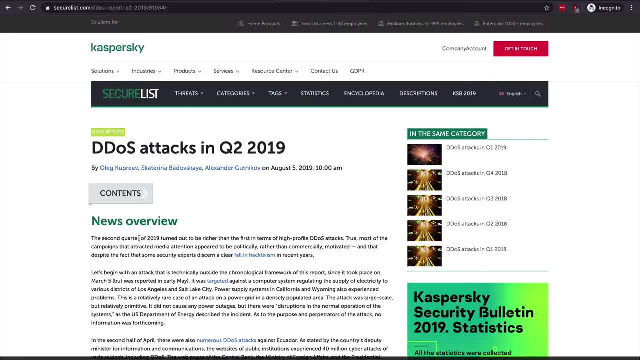 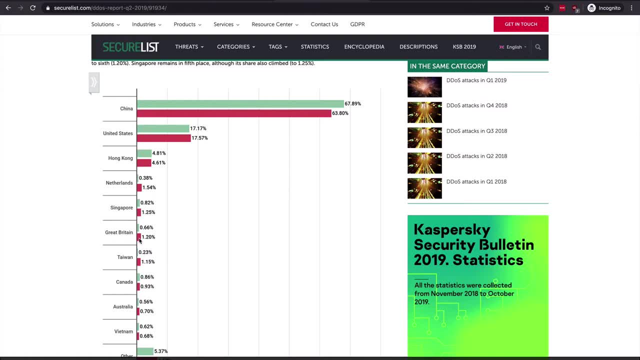 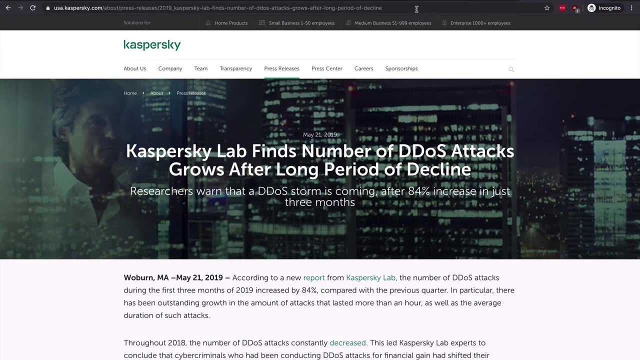 prior quarter, and some of which were political in nature versus commercial. Another interesting fact is that China and US ranked as the top two targets for DDoS attacks, with 63.8% and 17.5% of the attacks respectively, and Q1 also had seen an increase in attacks by 84% in just three months. 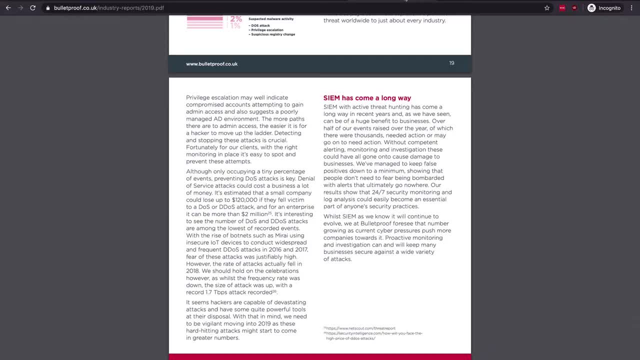 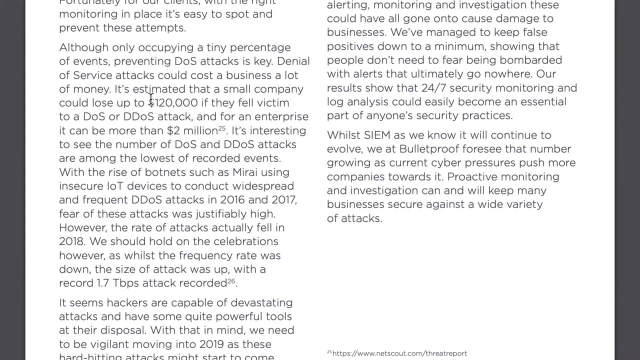 as compared to the prior quarter. Now, according to a bulletproof 2019 annual cybersecurity report, a DDoS attack could cost a small business up to $120,000 and up to $2 million for an enterprise organization, And other reports that I've seen have placed these costs even higher than this. 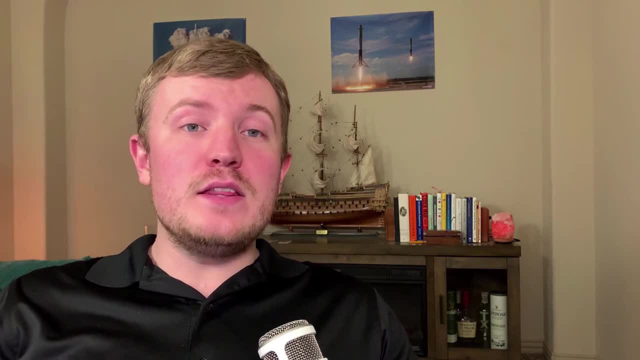 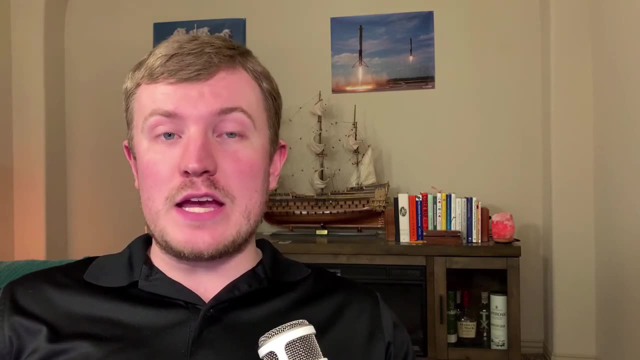 And one reason for the sharp increase in attacks in these recent years has to do with the rise of the internet of things. More and more devices are becoming connected to the internet, but their security, honestly, is often times laughable, And that's because the internet of things is so. 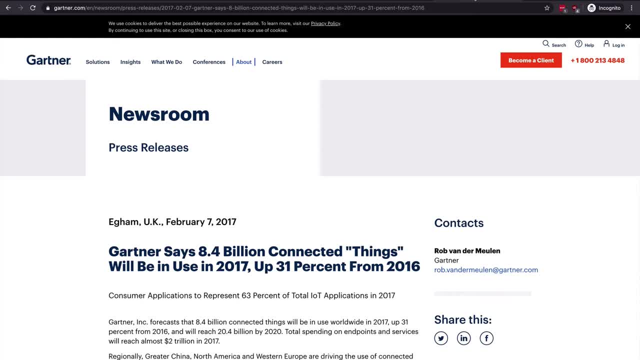 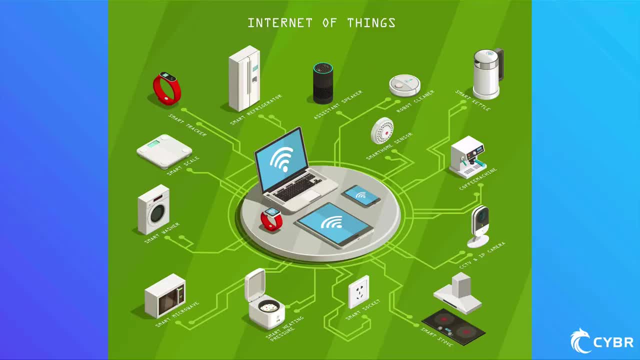 vulnerable. According to a press release from Gartner, the number of IOT devices that are estimated to exist is 20.4 billion by 2020, so this year, Think about connected refrigerators and other appliances, baby monitors, thermostats and all kinds of other devices Outside of IOT. 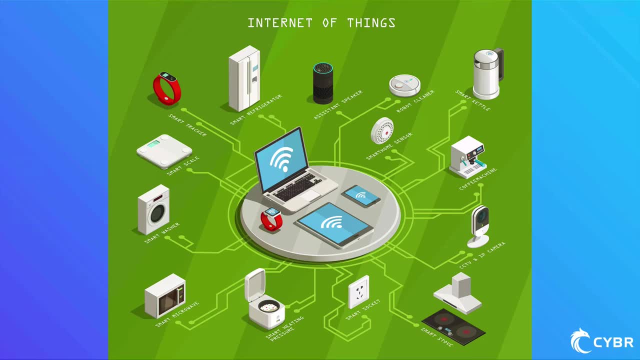 there's also your computers and your devices, like your phone, your laptop, PC, etc. And these devices can become compromised and then turned into malicious bot farms called botnets. As these devices are compromised, the threat agents can control them with simple. 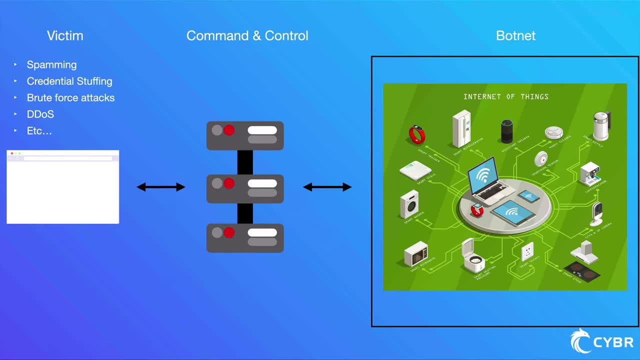 commands and have them do whatever they want, from spamming to brute force attacks, DDoS attacks and everything in between. So what can we do to defend against these types of attacks? Let's start by understanding them a little bit better. If we consider the OSI model, which 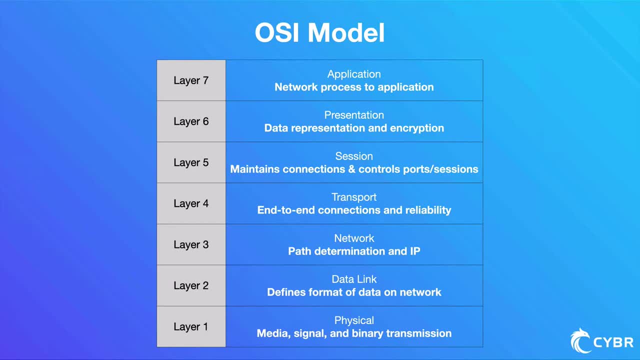 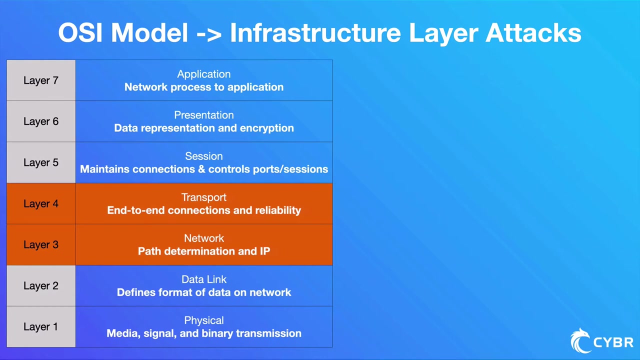 you might be familiar with if you come from a more networking background. we can group attacks as the infrastructure layer and the application layer attacks. There are other types, but we will focus on some of the bigger ones for this lesson. Let's start with the infrastructure attacks. These types of attacks are usually at layers 3. 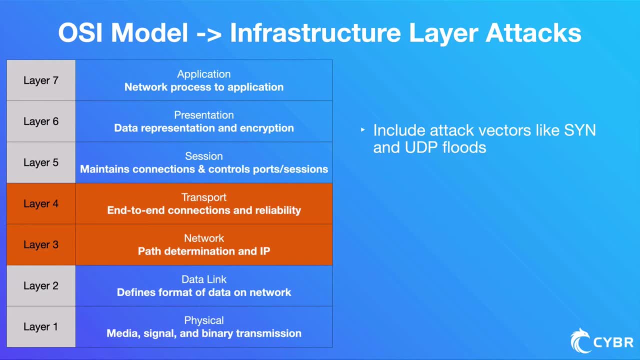 and 4, and they include attack vectors like SYN and UDP floods, And if you're not familiar with either of those, I do recommend a quick lookup or feel free to ask in our forums. In any case, these attacks are usually larger in volume and their aim is to overload the 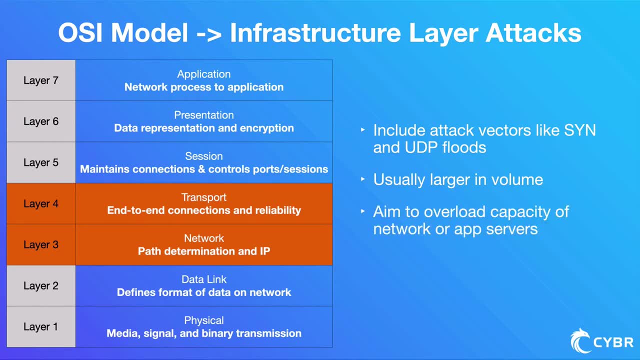 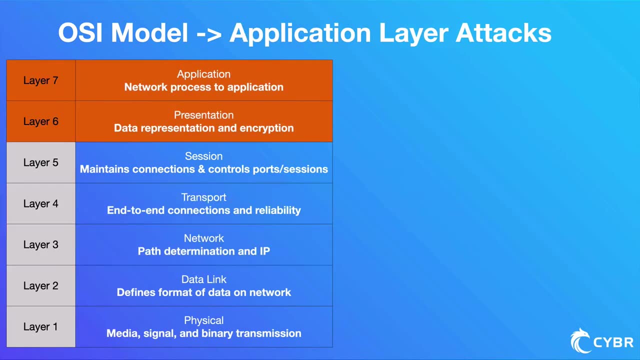 capacity of the network or the application servers. Fortunately, these attacks are not only easier to detect, which typically makes them easier to defend against. On the other hand, we have application layer attacks, which are usually at the layers 6 and 7.. 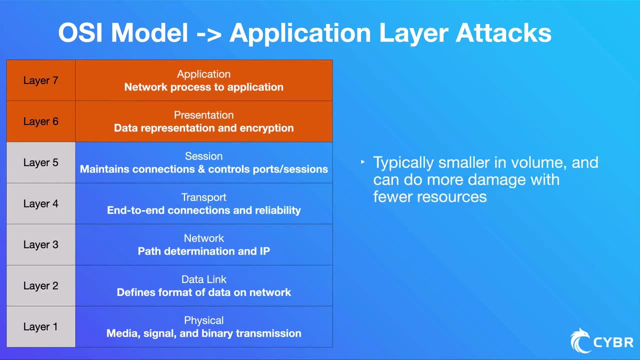 They're typically smaller in volume, but they can do more damage with fewer resources and they can be difficult to defend and prevent because the traffic can be made to look legitimate. For example, a flood of HTTP requests to a login page could take down the ability for users to 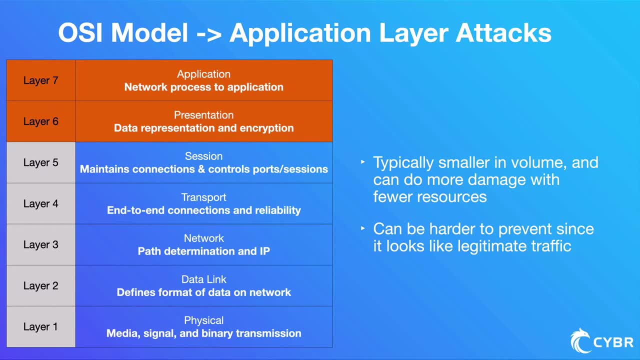 or even potentially take down the entire application. But using bot requests versus legitimate requests can be difficult, depending on the sophistication of the attack. So now that we know the two different main types, we can start to look at defense mechanisms. The first one that I recommend is reducing the attack surface area. 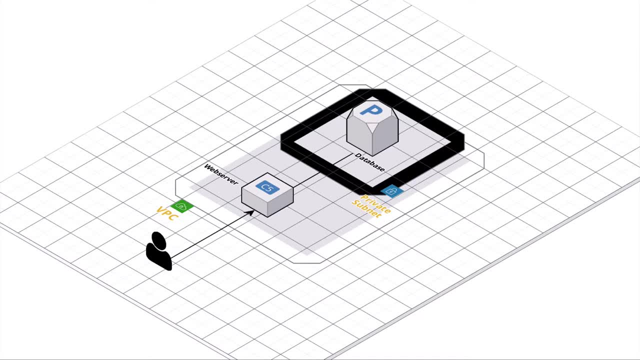 by limiting the exposure of your application and its resources to the outside world, And you can do this by hiding resources in private networks, like hiding databases, and making them only accessible from inside those networks, which is a best practice. So if you're using a bot, you can. 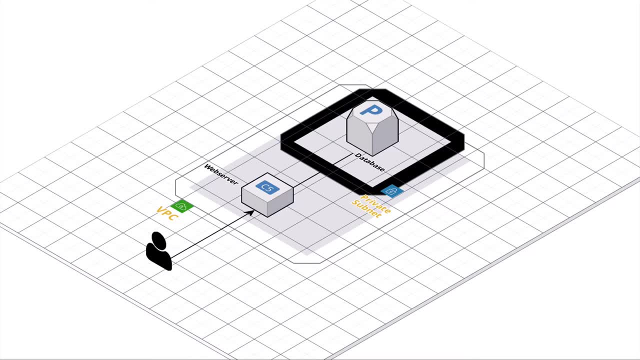 do this for other reasons. anyway, This doesn't mean that the attacker can't take down your database by making your application run expensive database queries over and over again, but at least they can't attack the database directly. We can also do this by restricting ports and protocols that 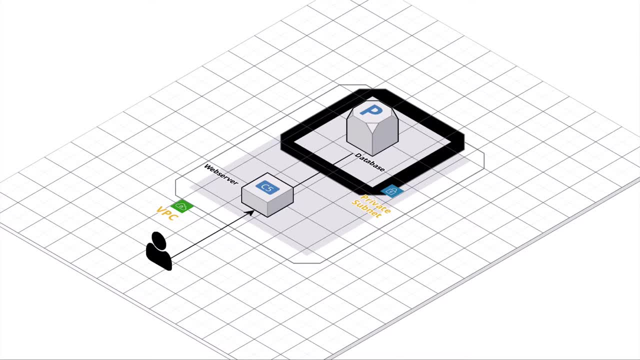 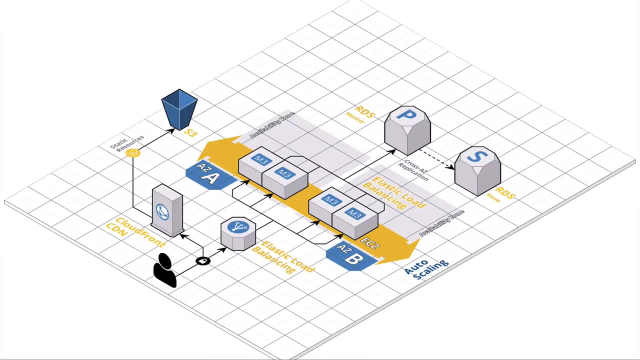 aren't absolutely necessary for your applications. Again, these are things that you should be doing anyway to reduce the potential of other types of attacks, but it's worth repeating here. Another way of restricting the surface area is by using CDNs and load balancers. 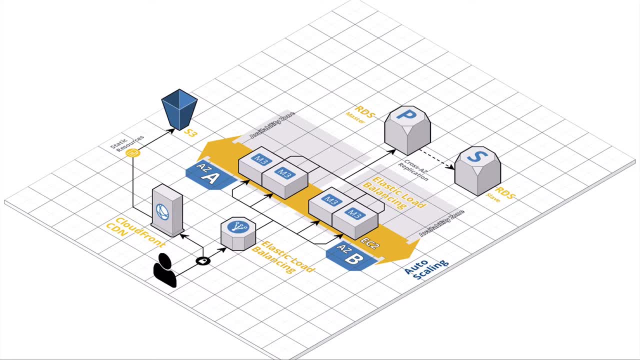 in front of your web servers or other resources. So if you're using a CDN like Cloudflare or Cloudfront, then the traffic goes through those servers before reaching your application servers And they will have other defense mechanisms included for free or for an extra charge. 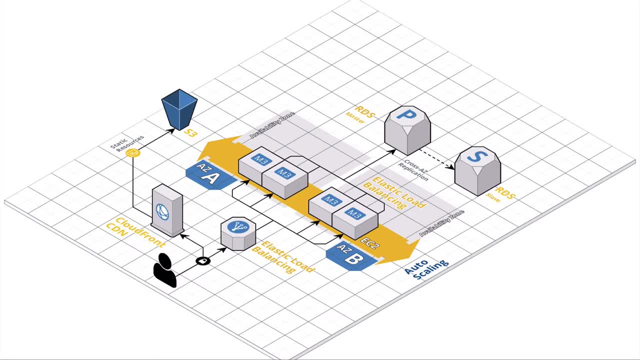 Now I mentioned the use of load balancers in front of resources and, as the name implies, load balancers are typically used to load balance between servers. So if you have four web servers serving traffic for your application, the load balancer chooses which server to load balance. 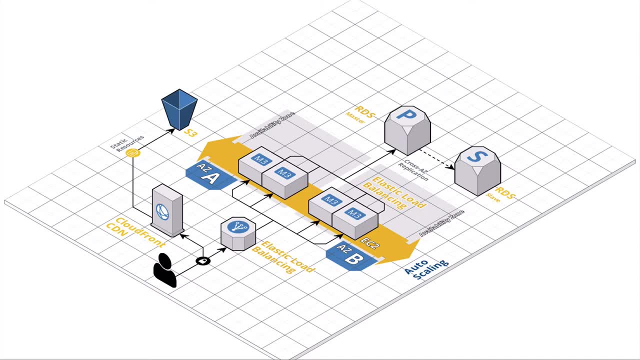 And by having four servers you can theoretically handle more users at one time. But if the attack overwhelms all of those servers, you could have automated scaling that spins up additional ones to handle that additional load. And this can work, sure, but it also means a higher bill. 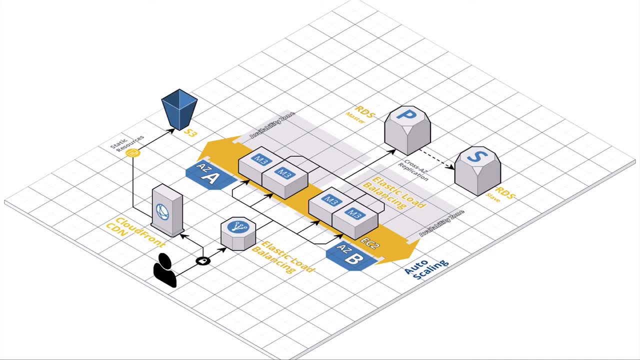 especially if your application is hosted in the cloud. So if your scaling policies end up having to spend, let's say, 10 more servers, that automatically increases your cost 10 times for the duration of the attack. You could always use a load balancer in front of just one web. 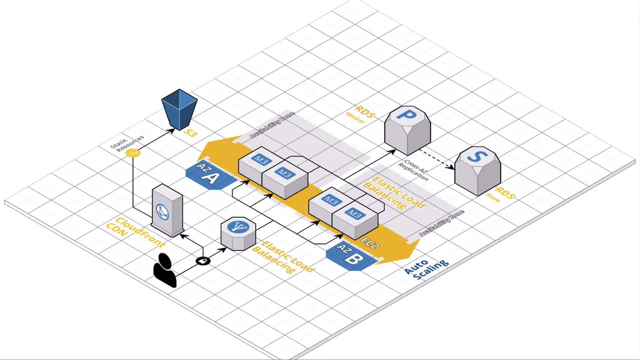 server and it doesn't have to be in front of multiple web servers, while still providing some of these benefits. But of course, at that point it won't be able to balance the load between multiple different web servers. You still just have one, unless you're scaling it out. 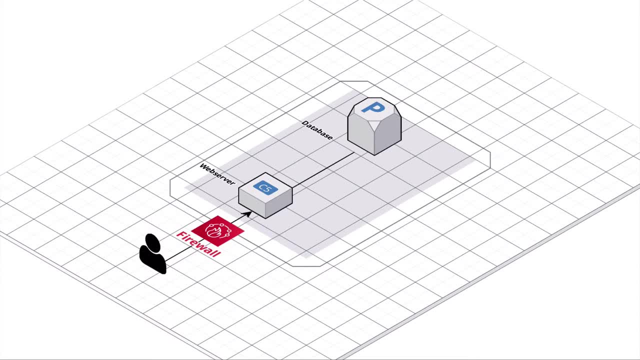 One more method that we'll mention here is using something like firewalls or other services that can detect abnormal traffic and prevent it from making connections. So if your system knows that you're using a load balancer, then you can use a load balancer to scale it out. 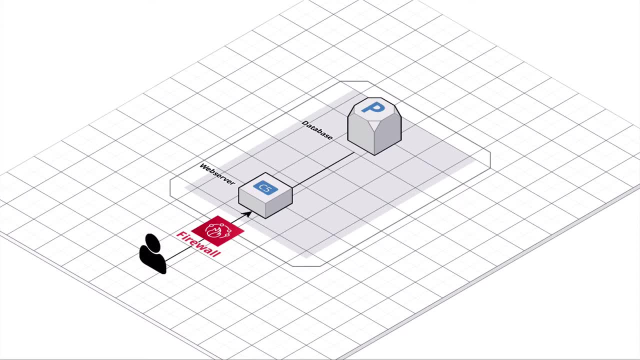 If your system knows what the normal traffic pattern looks like, it can detect whether something weird is going on, And this can get pretty advanced, and, of course, there are premium services that are available for this very reason. Of course, many of the security features and 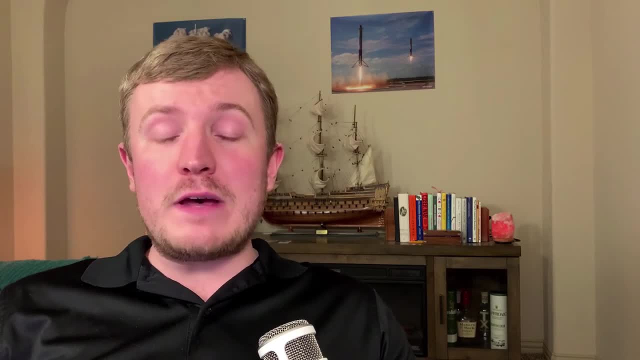 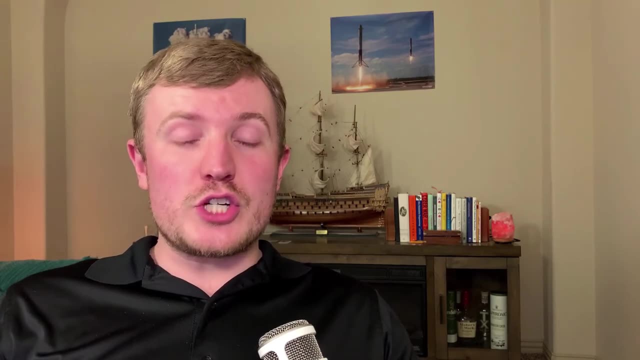 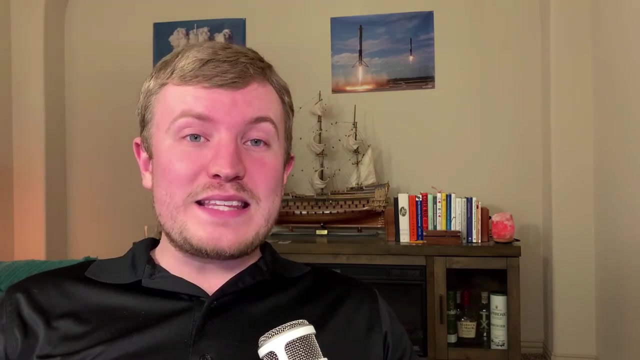 implementations that we've talked about in prior lessons can help defend against DDoS attacks, For example, preventing brute force attacks, credential stuffing attacks, even SQL injections. those security mechanisms can also help defend against DDoS attacks. Frankly, this is another topic that I could spend hours talking about, because 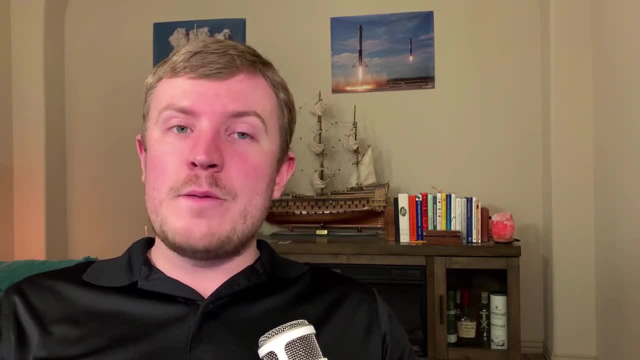 I've had the experience of dealing with DDoS attacks in the past and they're not fun. But now that we've covered the basics of DDoS attacks, let's mark this lesson as complete and I'll see you in the next one. 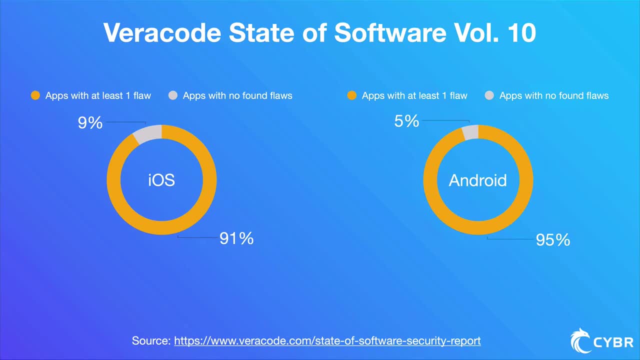 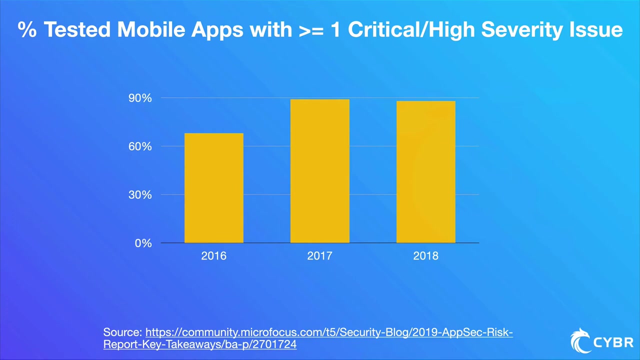 91% and 95% of applications for iOS and Android respectively have some sort of security vulnerability, according to a report by Veracode. A different report by Micro Focus states that 88% of the mobile apps that they tested had at least one critical or high severity. issue in 2018, which was up 20% from 2016.. Considering our reliance on mobile applications for our day-to-day personal and professional lives, these are pretty scary statistics, especially when you consider the fact that many of us have applications on our phones. 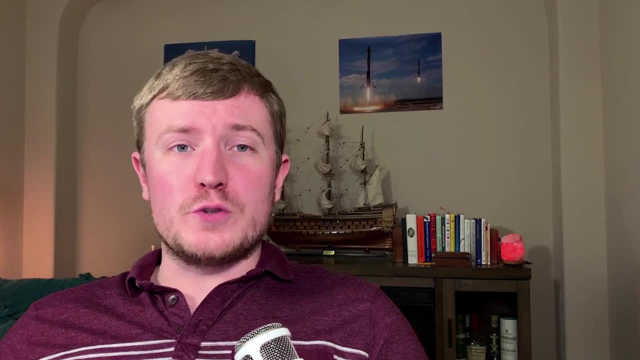 that control our home security, that could provide access to personal banking and personal finances, that contains images and that can be used to control our home security. So let's take a look at some of the applications that we've tested, and I'll see you in the next one. 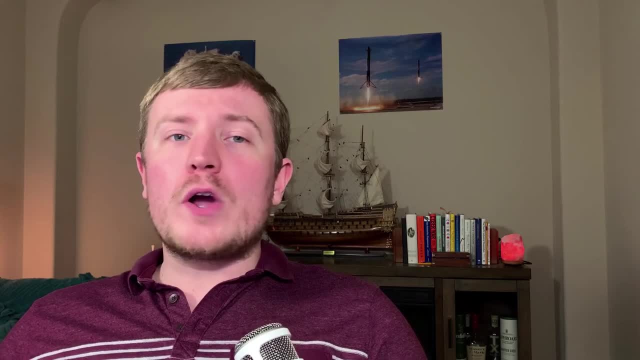 So let's take a look at some of the applications that we've tested- and I'll see you in the next one: images, videos, text messages and all kinds of personal information that, if it landed in the wrong hands, could do some serious harm. 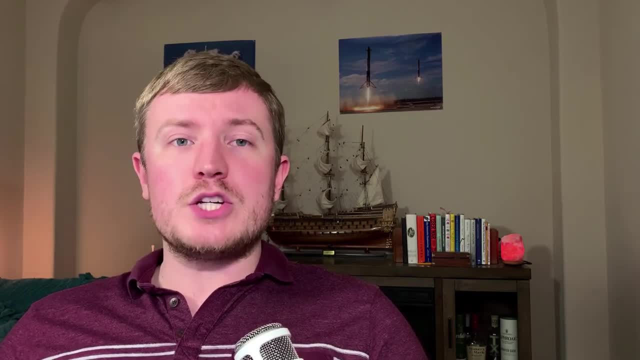 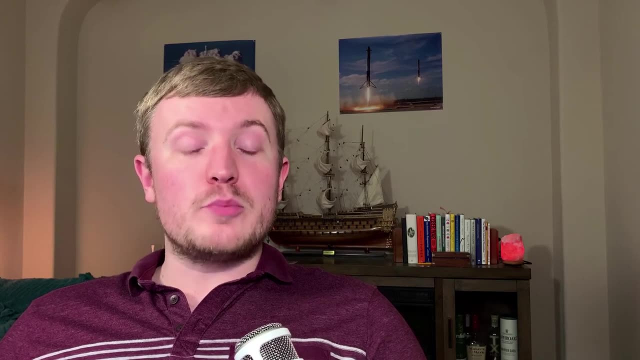 So, as we build our mobile applications, just like we would with web applications, we have to think about security from the very beginning, And we can do that by taking into account the two major platforms, which are iOS and Android, And both of these have unique values and they also provide unique perspectives. 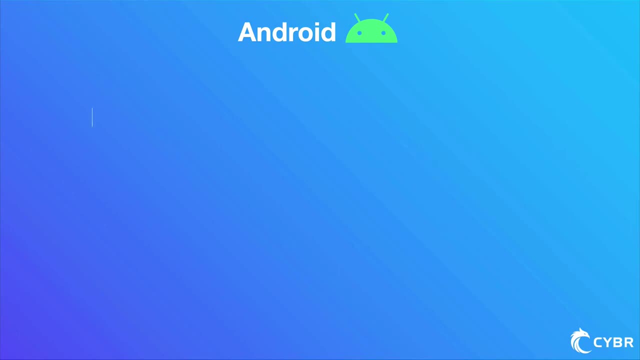 when it comes to security. With Android, we have an open-source. open-source platform that gives owners of devices the ability to mess around and customize code, which is fantastic because it provides more flexibility, but it can create weakness in the device's security. 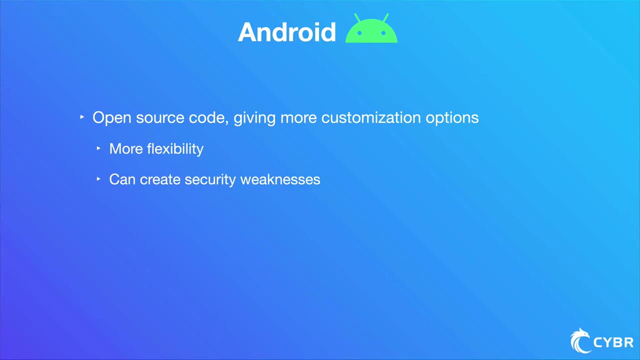 because we can introduce flaws and vulnerabilities when making modifications. There are also many different manufacturers with their different flavors of software and hardware, which again provides much more flexibility, but potentially at the cost of security. When it comes to updates, some providers or manufacturers may restrict which updates you receive. 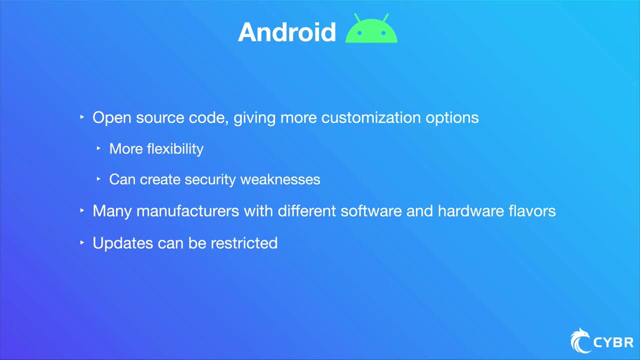 making it difficult to get the latest version, which is a critical step in keeping your devices secure. Android devices do have the most market share when compared to any other mobile device, including iOS devices, and this can be regarded as a weakness, because more users means more attractive targets for hackers. 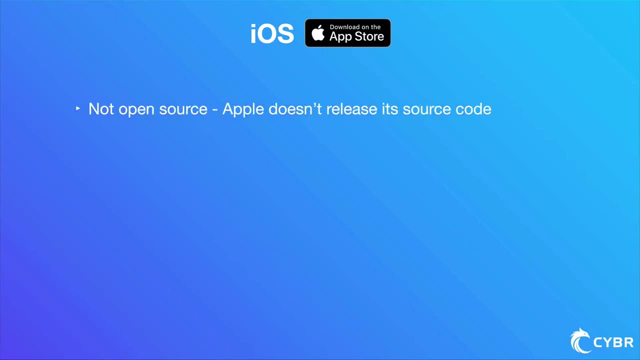 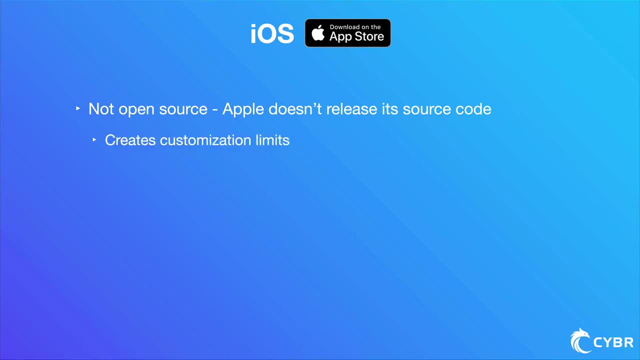 It can create limits, which many users and developers don't like, but those limits can be a positive when talking about security. Apple devices are tightly integrated between the software and hardware, which reduces the number of variances, And iOS releases are pushed to all devices much more quickly. 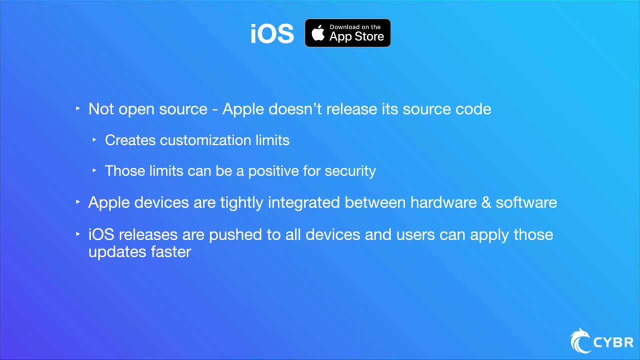 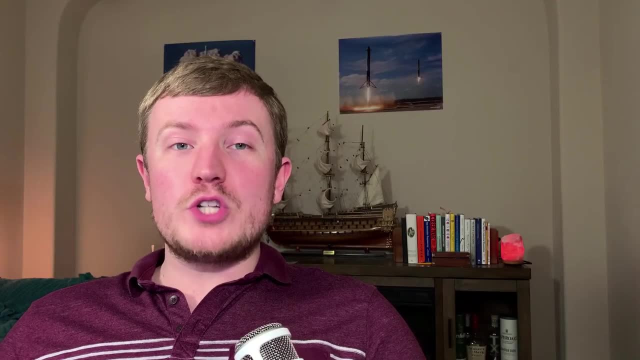 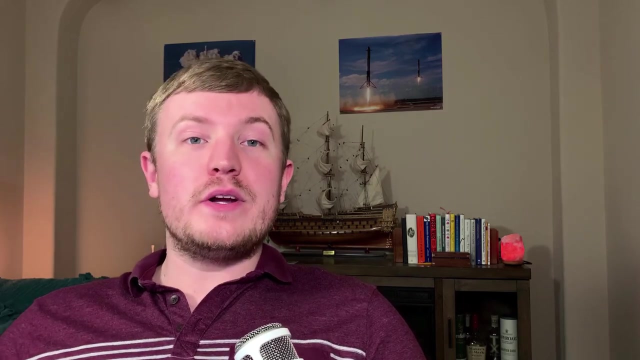 and since there aren't a huge number of manufacturers and different custom devices, users can receive and apply those updates much faster. In any case, both of these platforms have their own share of security risks and threats. So when developing mobile apps, we have to consider that and we have to do it from. 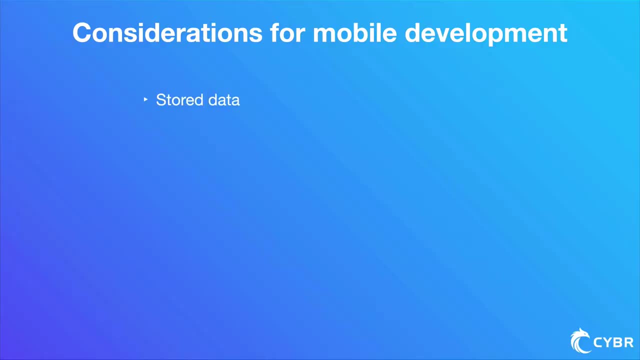 the very beginning, We have to think about how data is stored and transferred. We have to think about the APIs that our app is talking to and the vulnerabilities that may be present there. We also have to consider how application permissions can be exploited, how to handle. 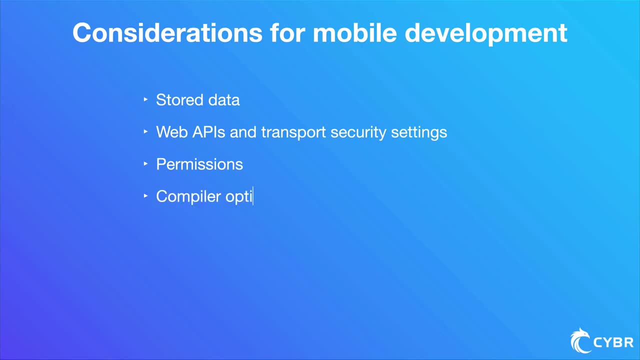 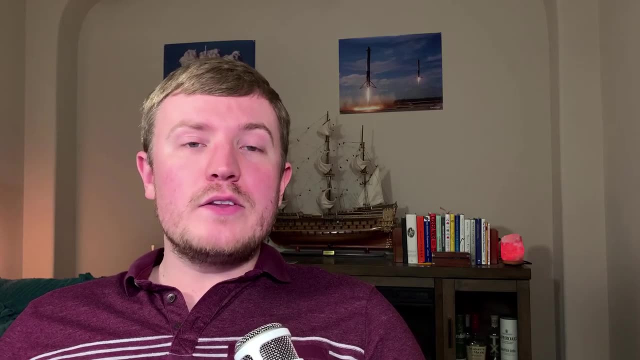 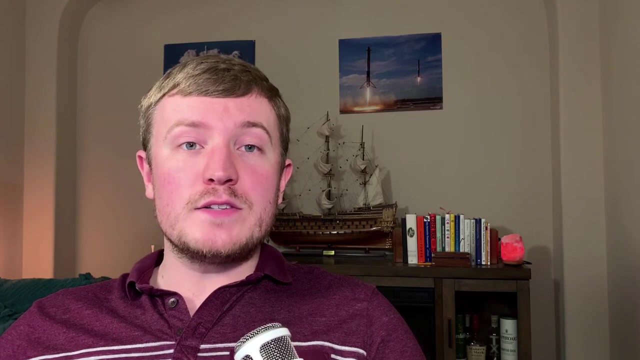 user authentication and authorization and anything else that may get exploited. In short, we need to think like an attacker, and in the next lessons we're going to explore different frameworks that help us build mobile application security requirements baselines, as well as look at some of the top mobile risks and ways of preventing against them. 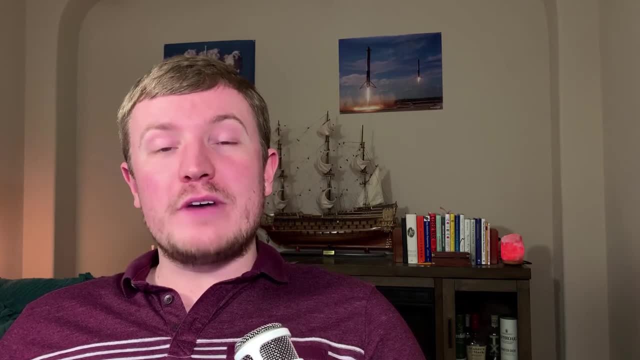 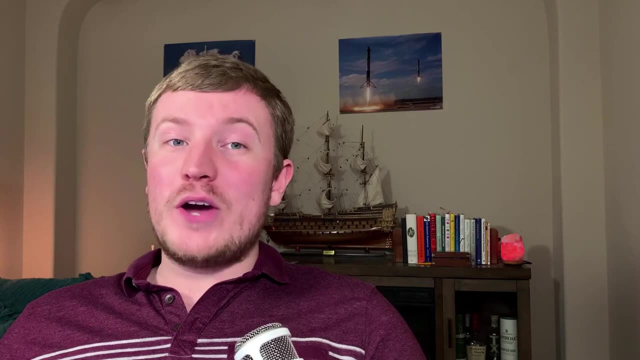 And later in the course, we'll take a look at testing tools to help us find issues in our code, and we'll also look at simulation tools that will teach us how to build more secure software. So go ahead and mark this lesson as complete and let's get started. 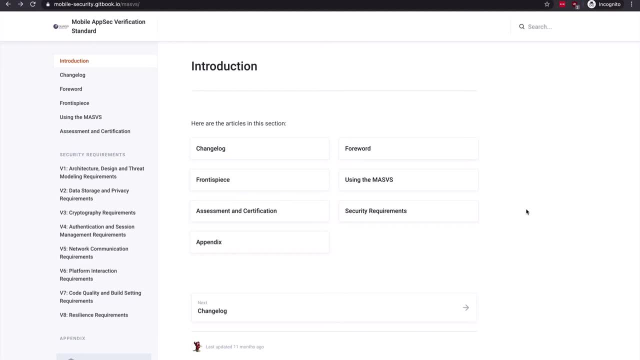 We've looked at the OWASP Application Security Verification Standard before, but that version was focused on web applications, So in this lesson we take a look at the mobile version. While the mobile ASVS or MASVS is very similar to the 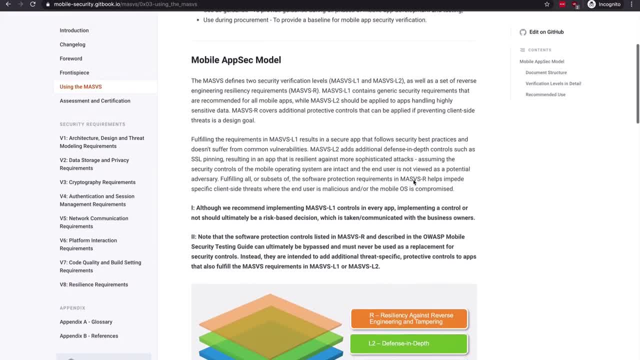 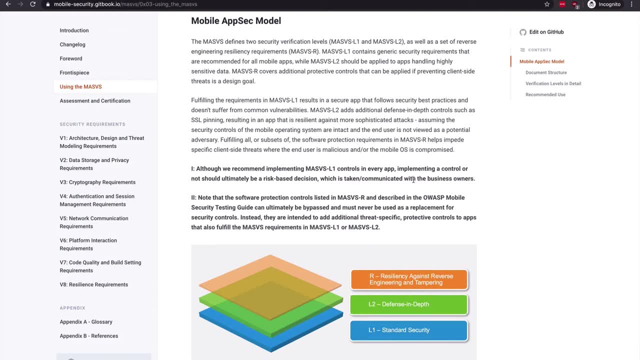 ASVS that we've already seen. there are a number of differences. For example, the ASVS had three different verification levels, while the mobile version has two. The first level is the recommended level and the second level is the recommended level. The ASVS has three different verification. 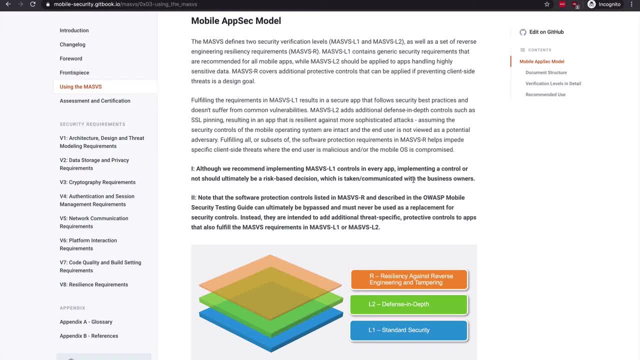 levels, and the second level is for applications that handle highly sensitive data, such as banking or healthcare apps. Also, the mobile version has a set of reverse engineering resiliency requirements which we don't have in the web version, and they aim to prevent client-side 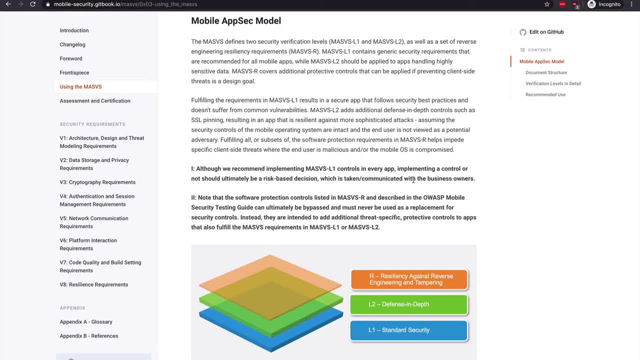 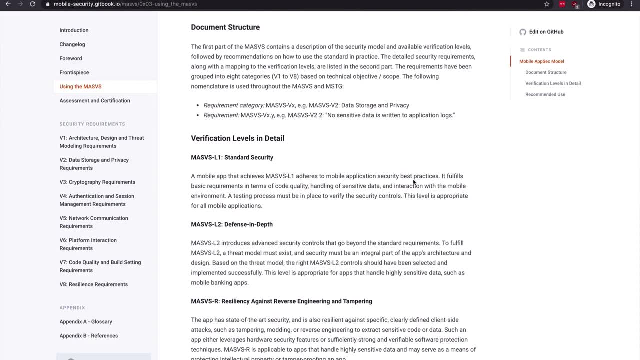 threats. These are meant to be used in addition to the L1 or L2 requirements and not as a replacement. The requirements are grouped in eight different categories which can be viewed and navigated to on the left-hand side. It's also important to keep in mind that the MASVS 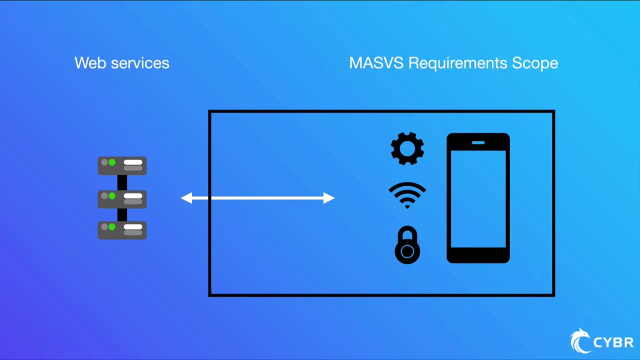 covers requirements to protect mobile applications on the client side and the network communication between the application and the remote endpoints, as well as generic authentication and session management, But it does not have requirements for the remote services, like the web services that are used by the application, such as APIs, for example. That's when the regular 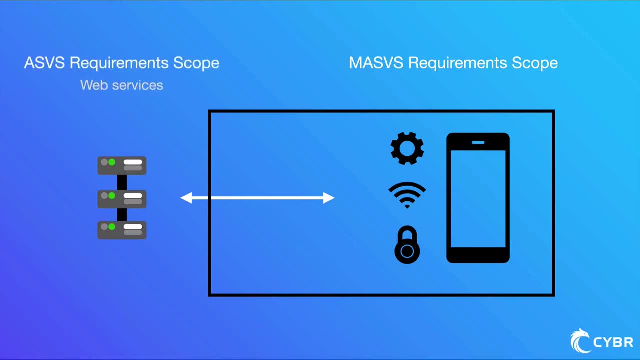 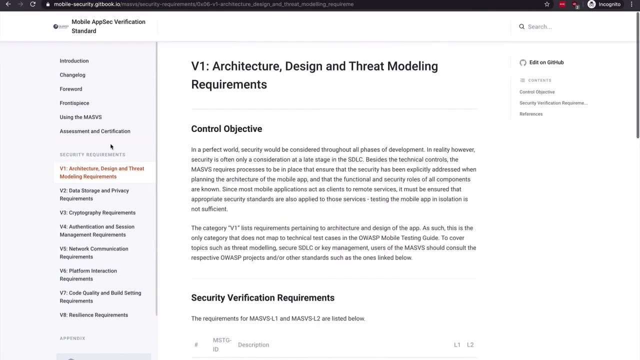 ASVS is used to protect mobile applications on the client side, and the network communication between the software and project is the one that is most important. We'll start with V1, which is all about architecture, design and threat modeling requirements. Just like with the ASVS, we start our requirements by creating processes to integrate security. 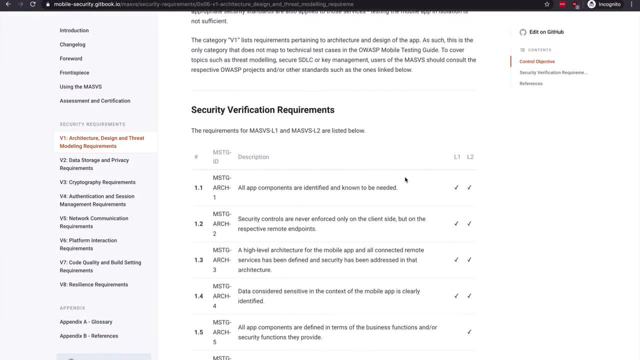 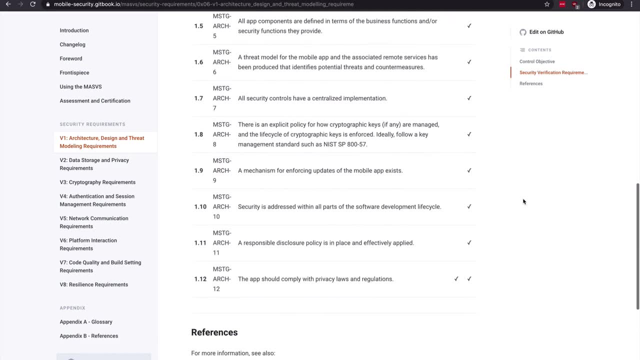 throughout our software development lifecycle. This will help prevent only considering security at the very end of development, which, as we know by now, is usually very hard to do by now, is not a security best practice, and some of the references that we have at the bottom here. 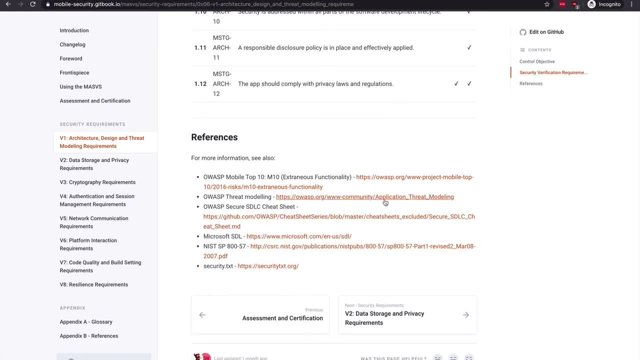 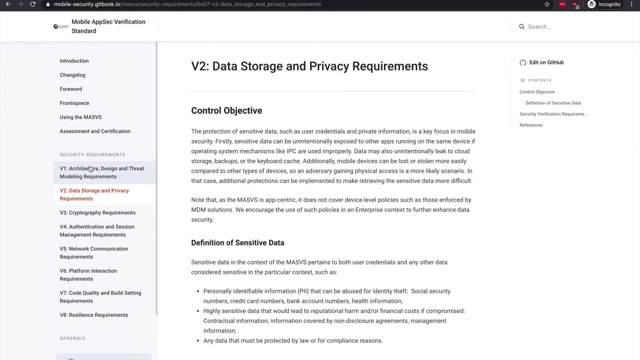 should look very familiar, such as the OWASP threat modeling that we used to figure out which of these requirements are high, medium or low priority for our application and for our organization. Next, for V2, we talk about data storage and privacy requirements. Data used by mobile. 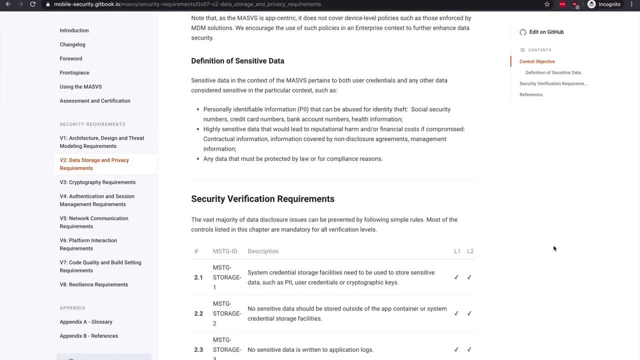 applications has unique security considerations. For example, how do we keep data protected if a mobile device is stolen? How do we make sure that the data stored in the phone's keychain is properly encrypted? You can't assume that the keychain is encrypting it for you. 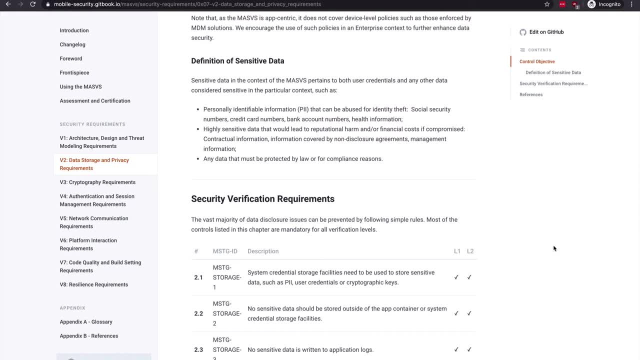 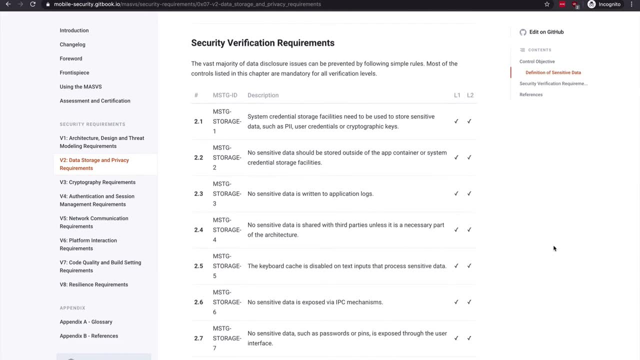 and we have to be mindful of data such as those keychain entries that persist even after an application is uninstalled. Understanding how data is stored on devices, but also how data is transferred to and stored in a mobile device, is important. For example, how do we keep data? 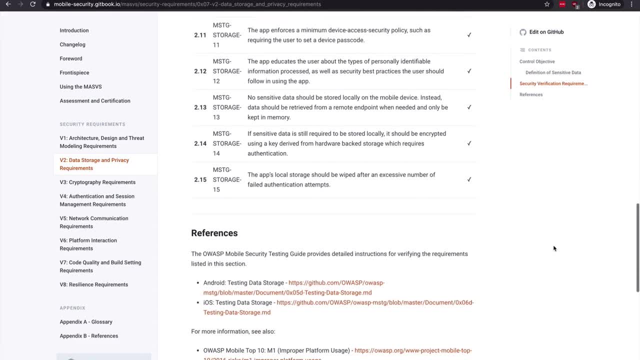 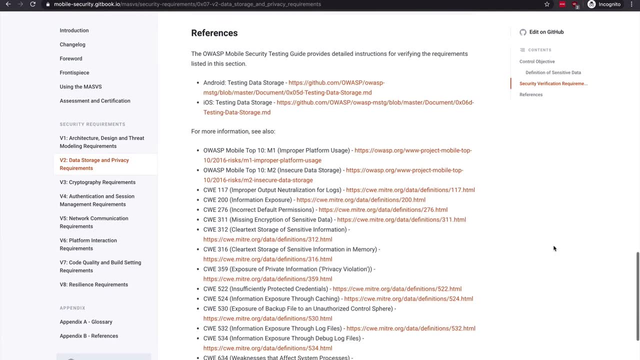 in the cloud is critical to making sure that the data is secure, and these requirements will help us with that. It also depends on whether you're developing for Android or iOS, and OWASP gives us references for both of the platforms, Like here, we have Android testing data storage and iOS. 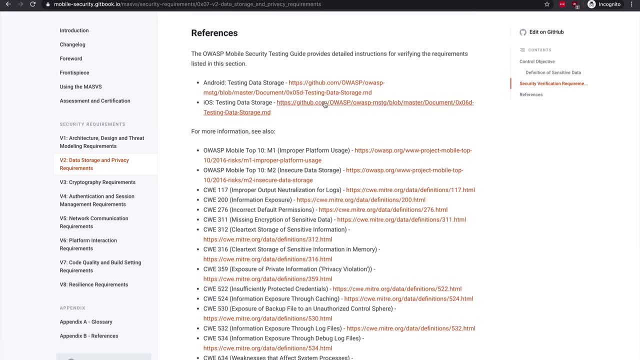 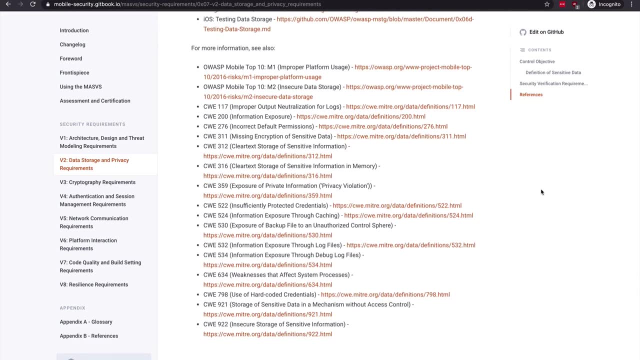 testing data storage with two different links. There's something called the OWASP mobile security testing guide, which we will review in a later lesson, and other references that you may have already heard about. For example, if you're using a mobile device, you may want to make sure that. 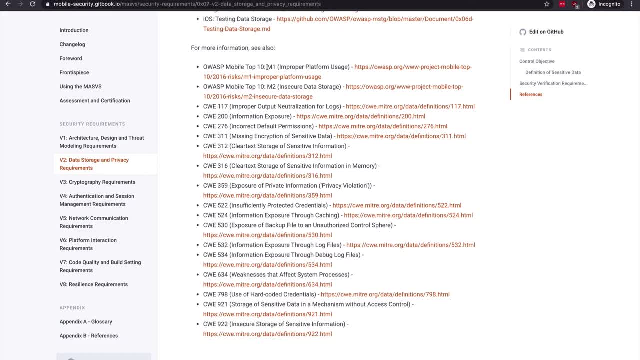 you include links to an OWASP mobile top 10 list. This is a list similar to the web top 10 that we've already reviewed, but this one is focused on mobile applications. Now the other requirements focus on cryptography, authentication and session management requirements. network: 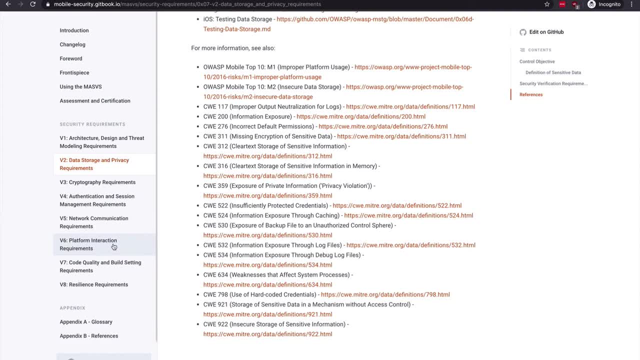 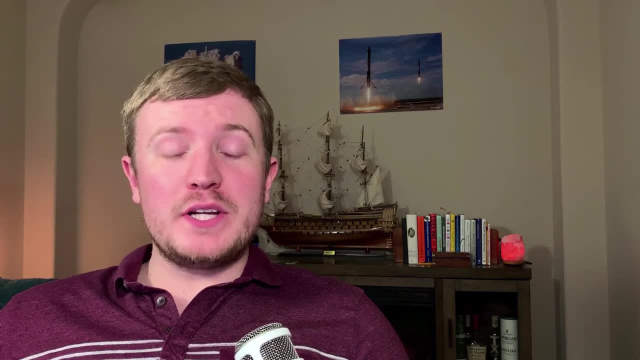 communication requirements, platform interaction, code, quality and build settings, as well as resiliency requirements. Please take a look at these after completing this lesson and, as always, if you have any questions at all, please reach out in our forums And once you're ready, 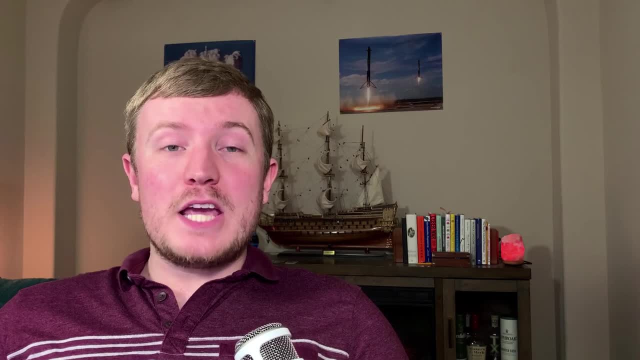 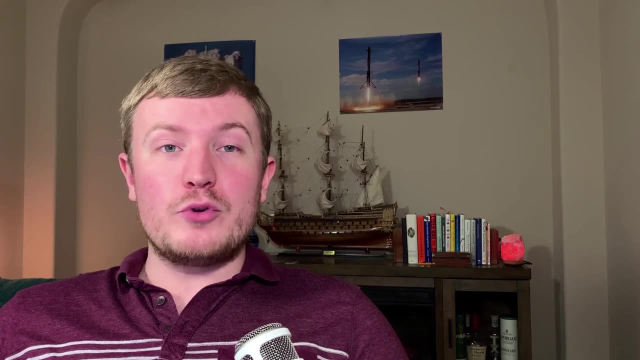 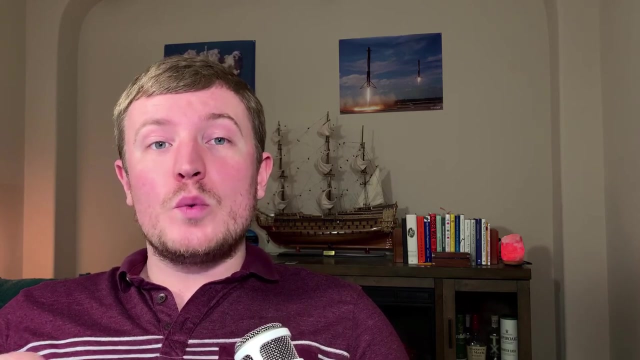 let's move on to the next lesson. Just like for web applications, OWASP has created a top 10 list of mobile application security risks, And this is an incredibly helpful starting point for building a baseline understanding of mobile app security. And, as we saw in the prior lesson with the MASVS, 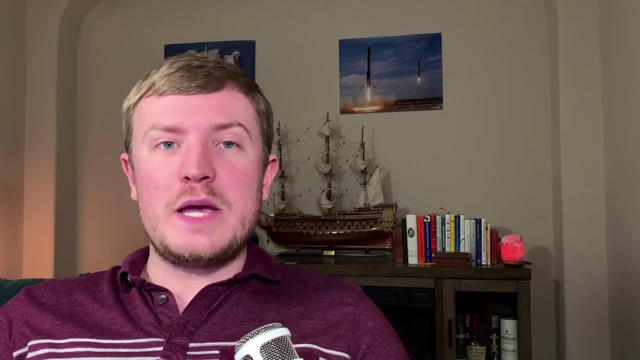 framework. a lot of the requirement categories link to these pages because they aim to protect our mobile applications. So if you have any questions at all, please reach out in our forums and we will be happy to answer them. And that's it. Thanks for watching. 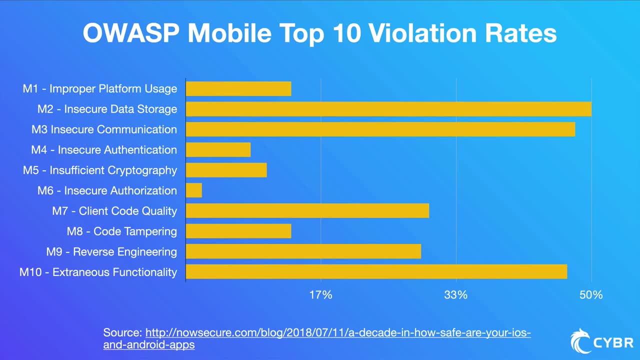 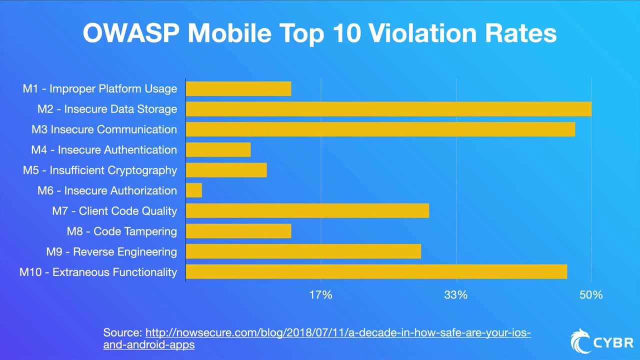 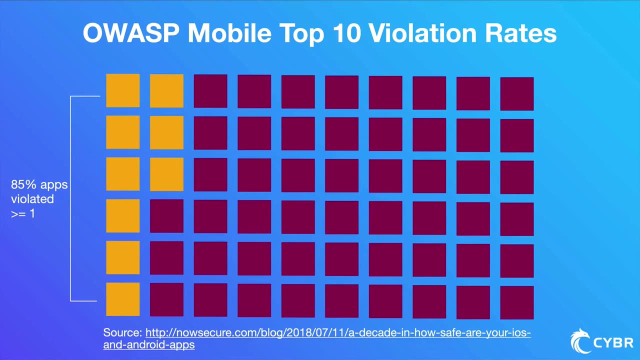 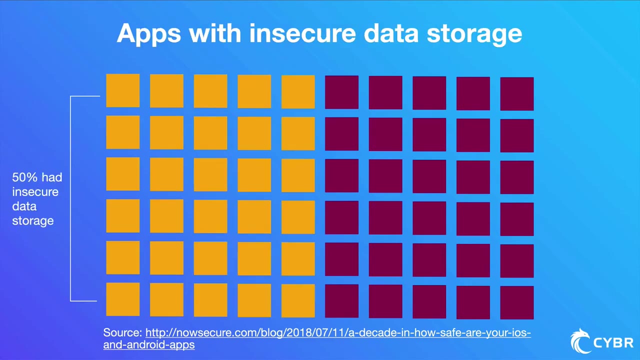 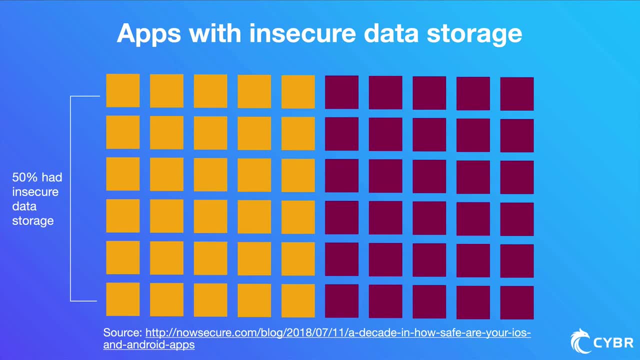 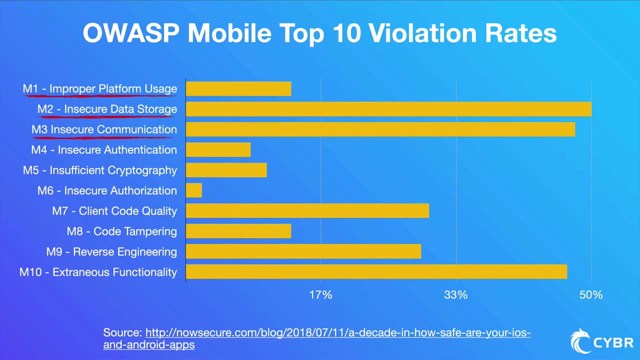 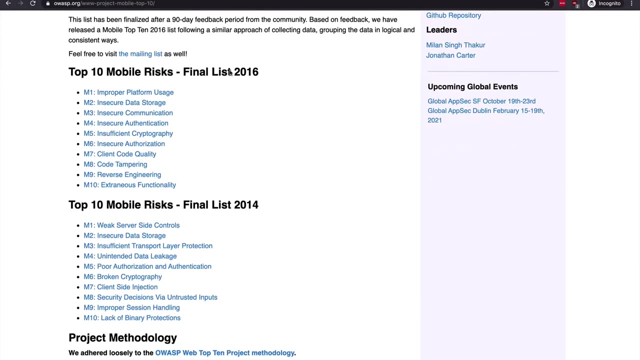 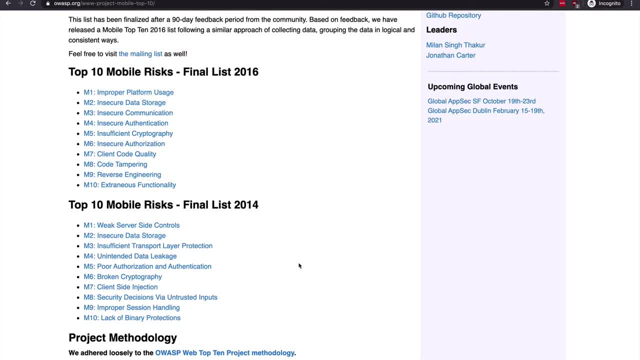 list by list and see which risks are still current in the 2016 list and which ones have either evolved or disappeared. But for this lesson, we will be focusing on this 2016 list. Let's start with the first risk, which is improper platform. 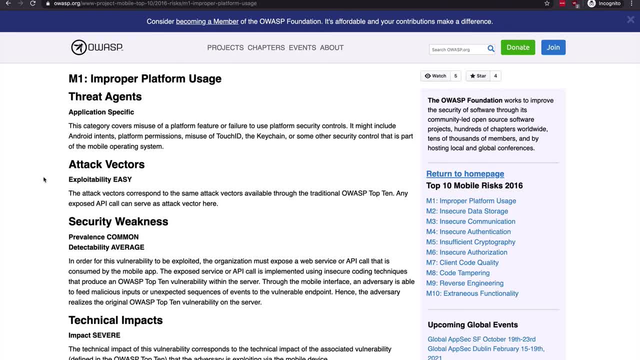 usage. Each platform, whether it is Android or iOS, has a certain way of doing things, and failure to follow best practices can lead to vulnerabilities, whether in the mobile application itself or with the web services that are powering that mobile app, For example, if we do not properly implement touch ID. 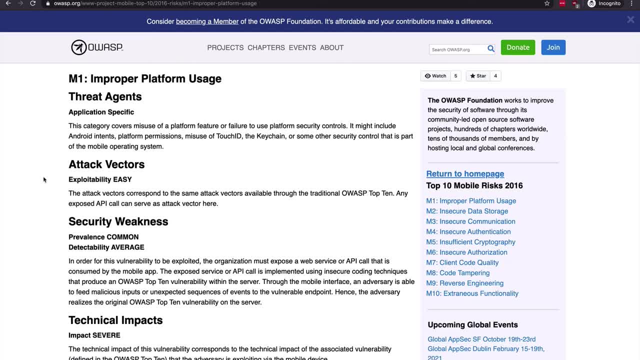 security for iOS applications. it's possible that malicious users could bypass this security mechanism to access an application such as a banking app. Now, this is not just theory, but it's also a risk If you're using a mobile application and you're using a touch ID. there are examples of people bypassing touch ID because it wasn't. 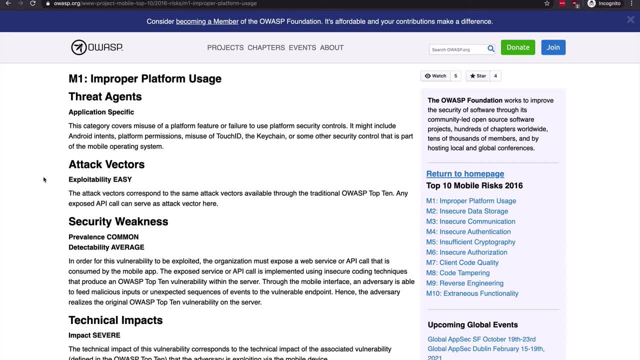 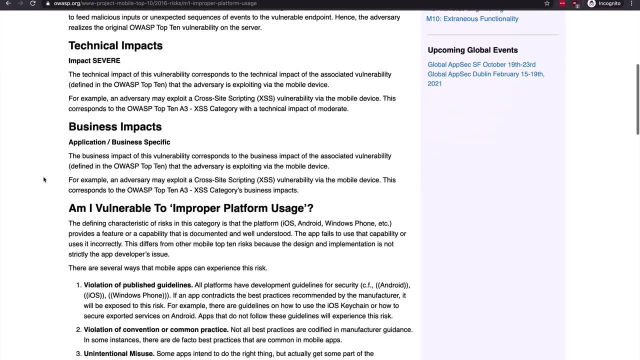 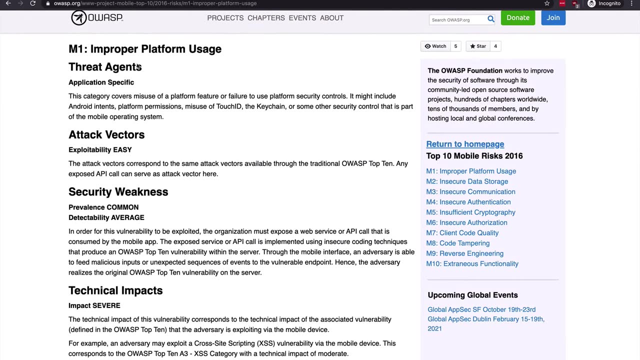 implemented correctly. This page helps us understand different and important factors as they relate to improper platform usage, and this should look very familiar to the risk and threat modeling ratings that we saw in a prior lesson. We have threat agents, which are going to be application specific. We also have attack. 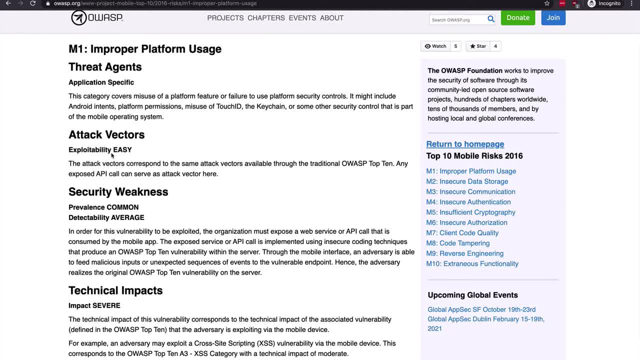 vectors, with the ranking of how difficult or easy it is to exploit these attack vectors related to this risk, which, in this case, OWASP rates as easy, with an explanation of what they are. A lot of the issues associated with the improper platform usage are tied to web services and, since we went over the OWASP top 10, 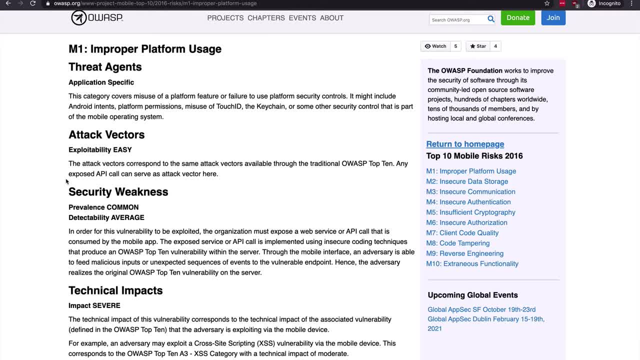 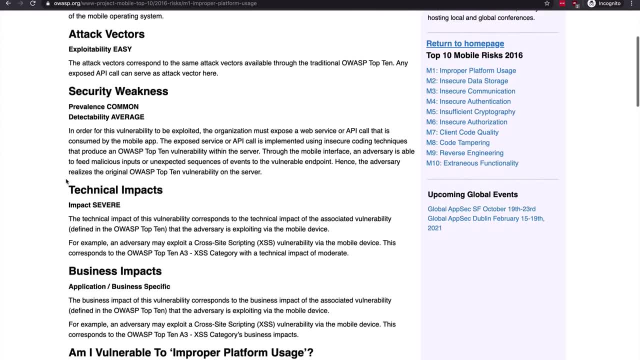 web application security risks in the prior section of this course. please refer to those lessons if you haven't already watched them or if you don't remember what they are Now. when it comes to the security weakness, OWASP provides a preference and detectability. The prevalence labels this risk as being 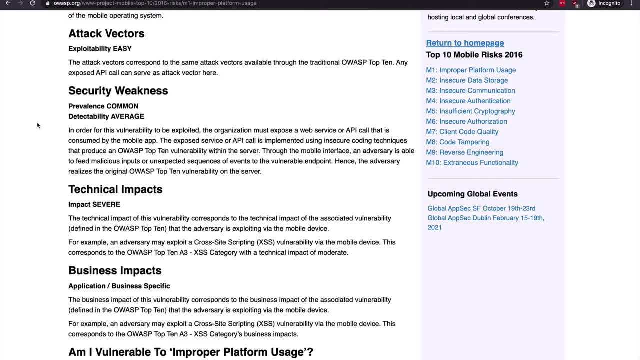 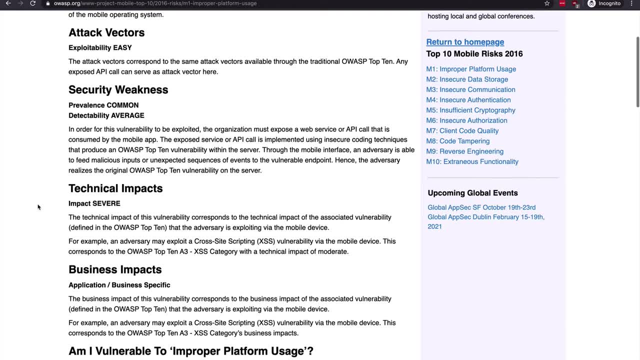 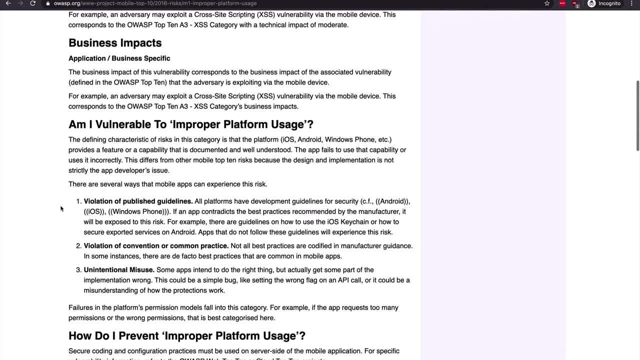 common with an average difficulty of detecting it in your code. The technical impact lists it as severe, but it does depend on which vulnerability is exploited and business impacts, as we know, is highly dependent on the application and the business. Next, OWASP lists a few ways of figuring out. 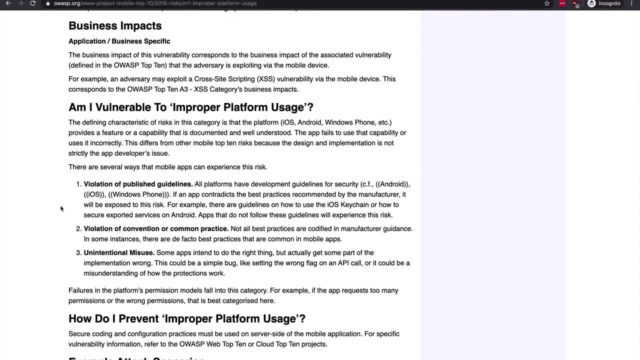 whether your application is vulnerable to this risk. In this case, they list three separate ways. The first is a violation of published guidelines. Each platform, again, has a different way of doing things, and developers can sometimes cut corners to make it easier, faster or for whatever other reason, and doing this can result. 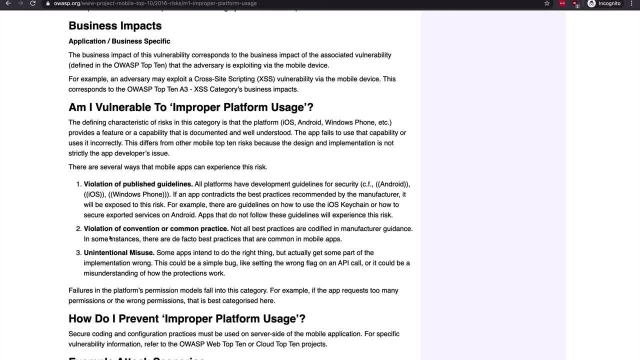 in creating vulnerabilities. The second one is a violation of convention or common practice. Many tutorials or documentation can leave out important details or can be misinterpreted by the developer, and the end result is improper implementation that opportunities for users to use the performance that they're looking for. 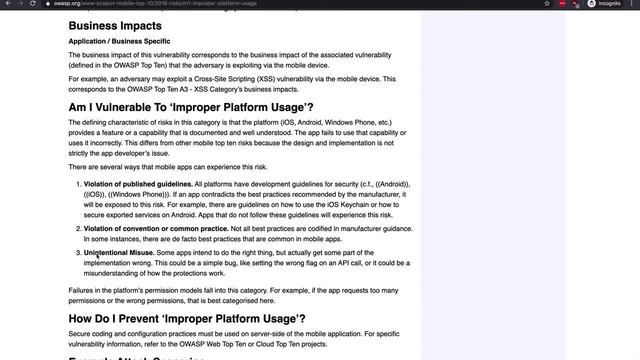 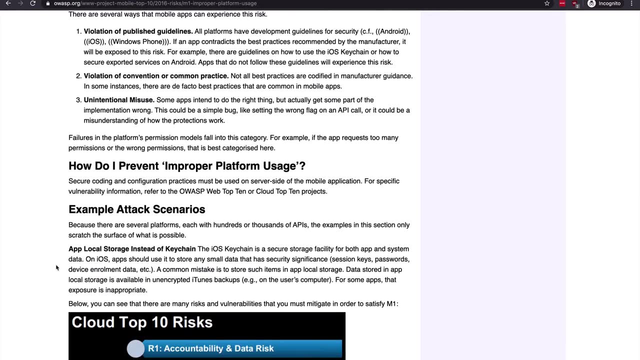 opens up the app to vulnerabilities. The third is unintentional misuses. In some cases, you may be following best practices and all of your intentions are good, but maybe you missed something important or introduced a bug. To help, and following this section, they list ways of preventing improper platform usage. 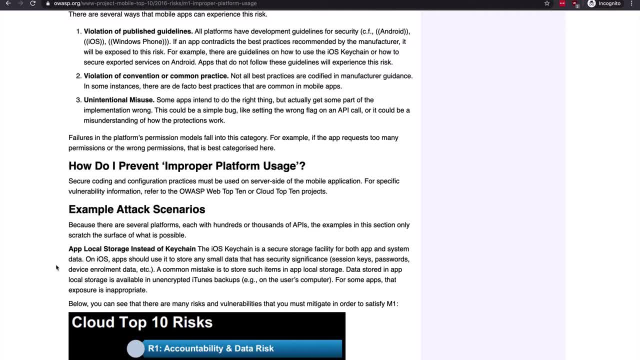 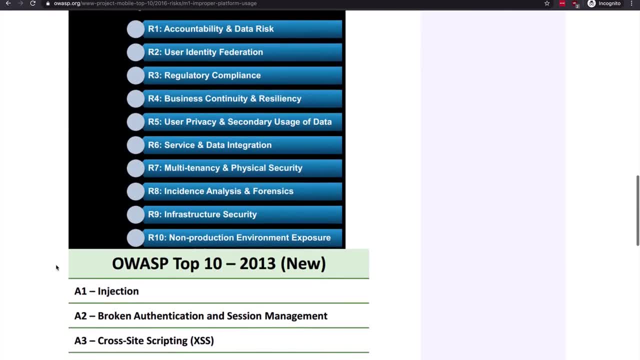 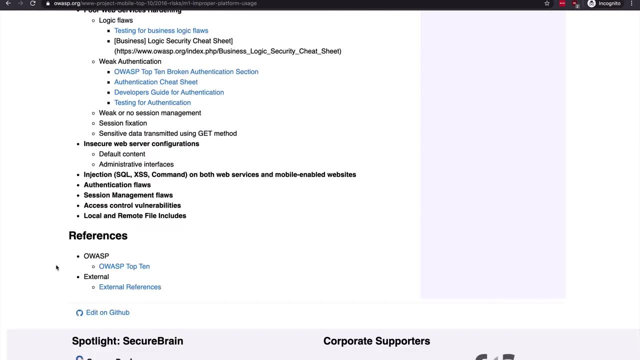 which, in this case, refers to the OWASP web top 10 list that we've talked about. Then they provide a helpful list of attack examples so that we can see what kinds of attacks could take advantage of this risk. Finally, there is a list of references that we can look into in order to continue researching. 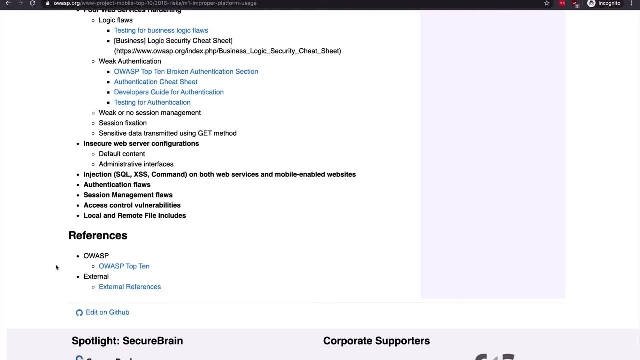 relevant information. This page, overall, is structured a bit differently than the web application risks that we saw in the prior section, but it still follows a very similar format, which makes it easy for us to understand and follow. And now that we've reviewed the first risk, let's go ahead and take a look at the second. 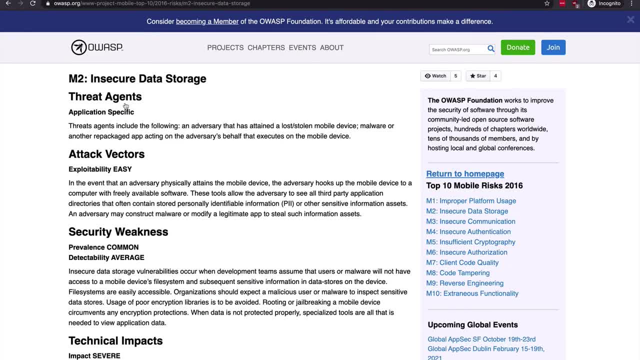 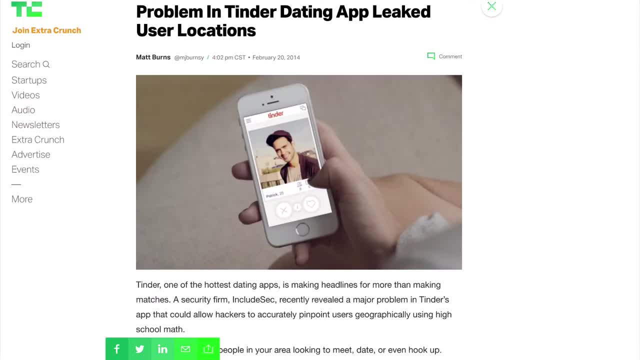 risk, which is about insecure data storage. If you remember, this was the highest found violation in the NowSecure report that we saw earlier. An example of this happening is in 2014, with an app called Tinder, which was a very popular dating application. 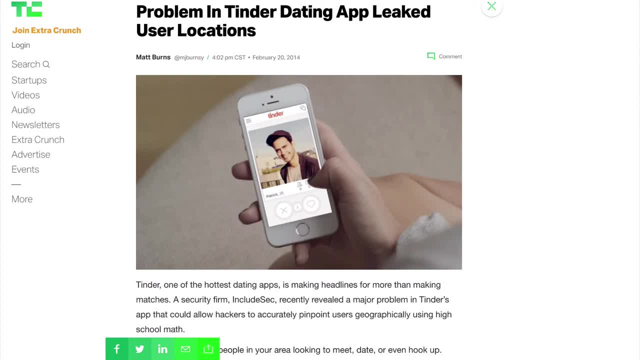 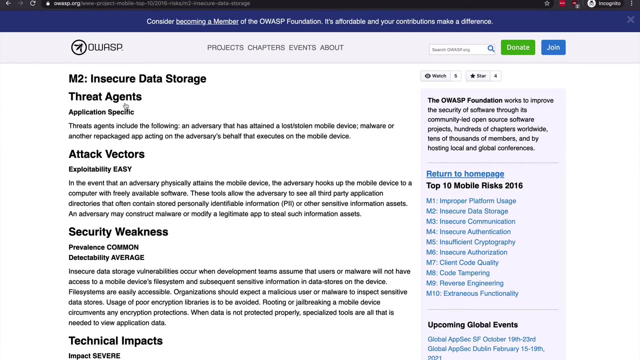 However, it was sending users exact locations in order to figure out which users were near your location. Except, the location, data was not encrypted properly, and so people figured out how to find this data on their smartphones and see exactly where it was. So insecurely storing data can result in identity theft, privacy violation, fraud. 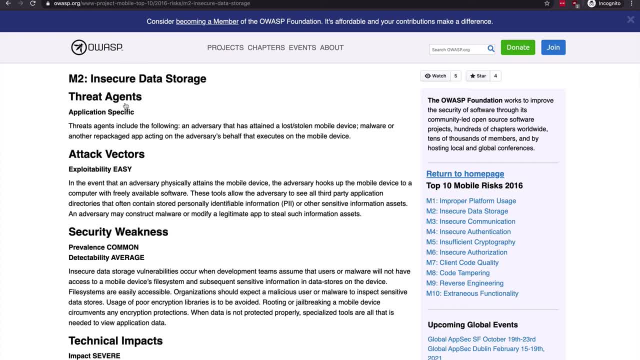 reputation damage and other losses or damages. And this risk is not just relevant if someone's phone gets stolen. it can also be exploited by malware or other means, like the example we just talked about, And just because you store something in the keychain- SQL databases, cookies, SD cards- 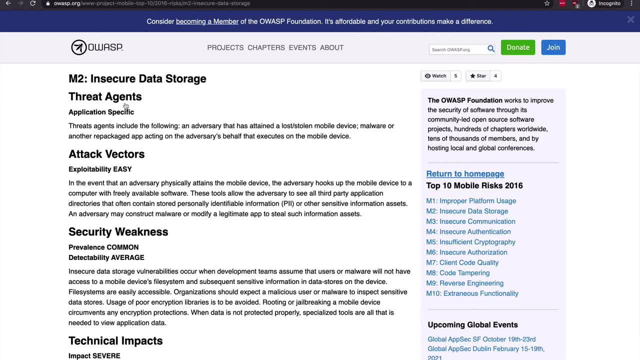 on the cloud or really anywhere else. You can't assume that it's being encrypted. You have to assume the opposite and you have to plan accordingly. Now, in the case of this risk, the exploitability factor is easy, because if an attacker gets 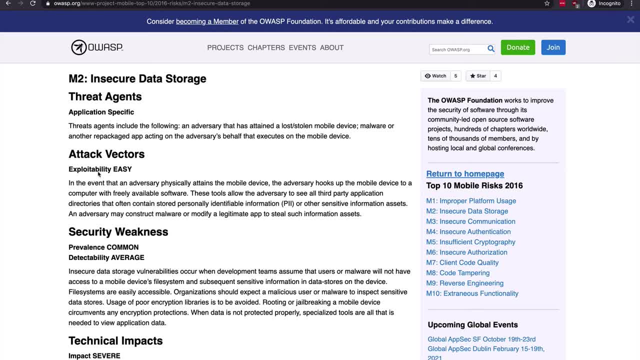 physical access to the mobile device. they can literally just hook that device up to their computer and with freely available software they can see all third party application directories and go through them, But they don't even have to have physical access to the mobile device though. 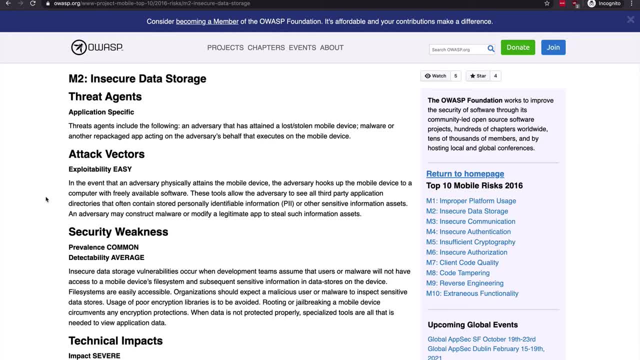 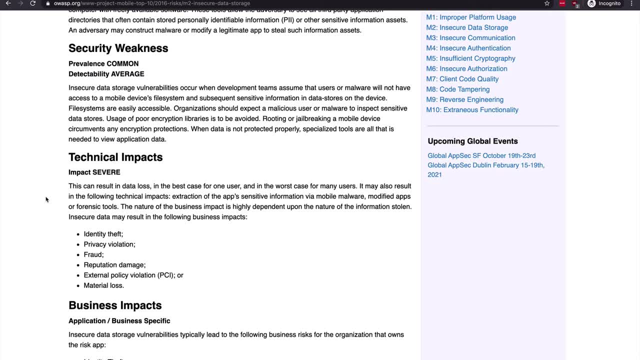 They could create malware Or modify the application to send them this information. The security weakness prevalence rating is common and the detectability is average. We can check that important data is being encrypted using similar tools that would be used to exploit the vulnerability, and we can also check which encryption libraries 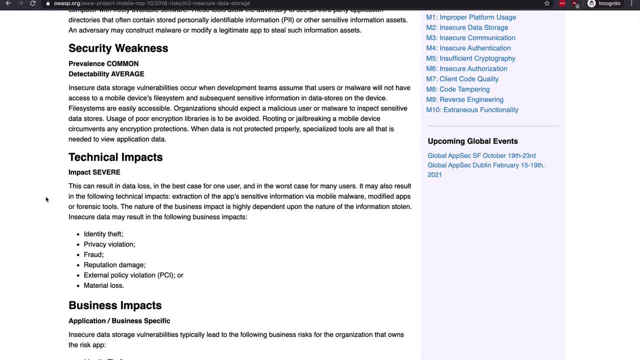 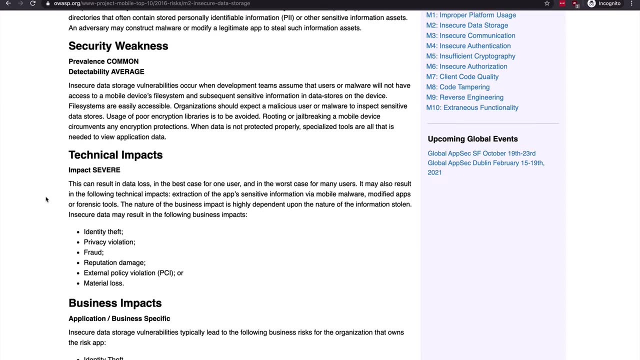 are being used to make sure that they're strong enough and that they don't have any known issues. Again, we've talked about this, but never, ever, use your own encryption. Use popular encryption libraries that have been vetted by experts. And these are just a couple of ways that we can detect problems with storing data. 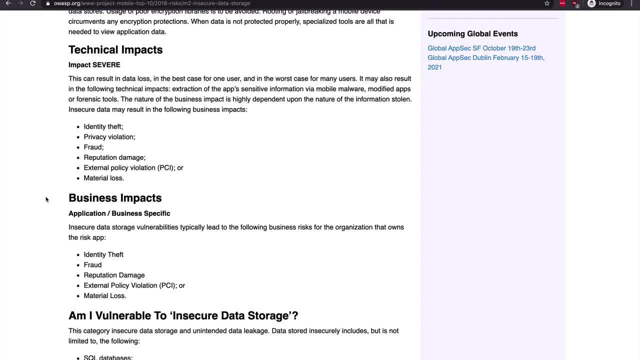 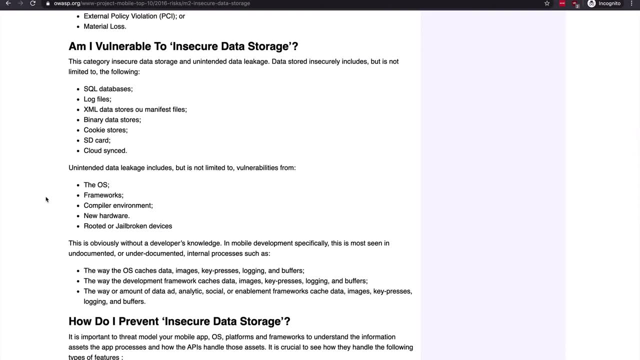 The technical impact can be severe and the business impact depends, as usual, but that could certainly also be severe. Determining whether your application is vulnerable to this and preventing the risk requires that you check how and where your important data is being stored. 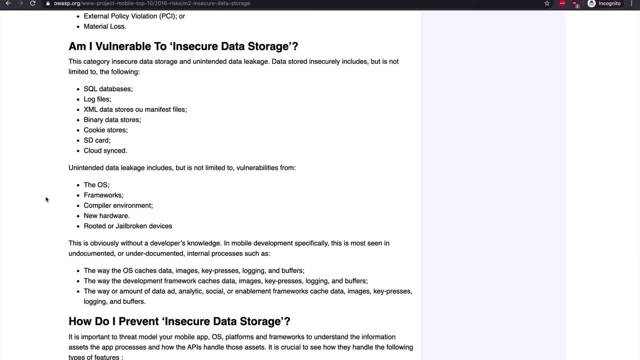 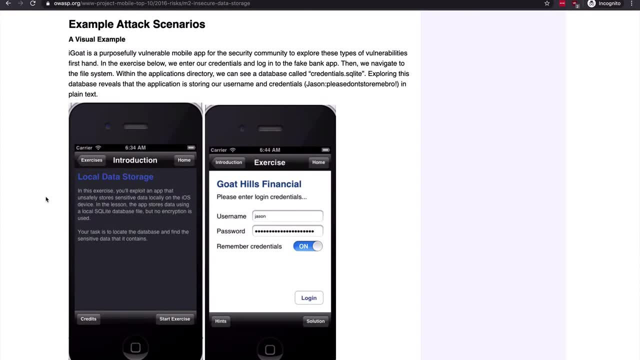 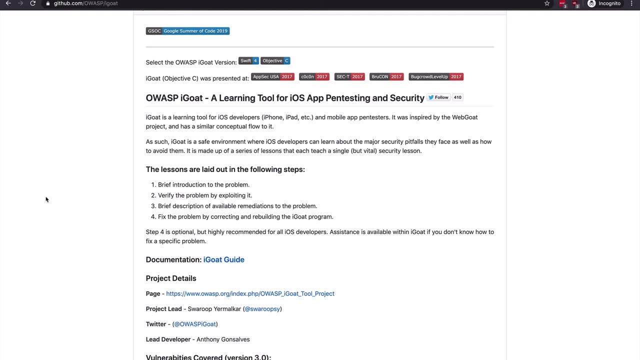 Again, don't make assumptions, instead verify. And again we can see examples of this, The example attack scenarios, And in this case they are including an application called iGoat, which is maintained by OWASP and it provides a learning tool for iOS application pentesting. that illustrates these risks. 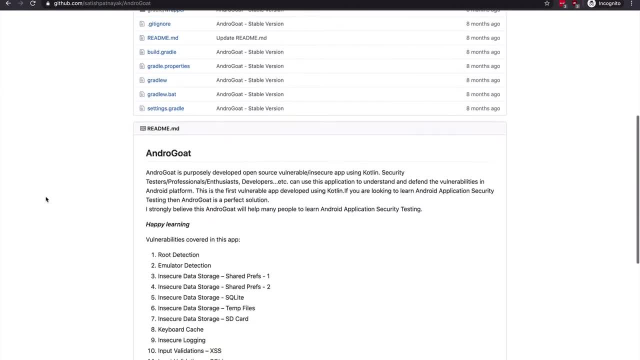 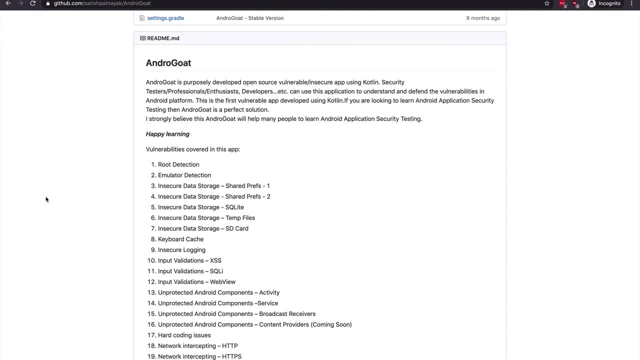 Androgoat is a similar type of application, but this time it's for Android instead of iOS, So feel free to look into these. In a later section we'll talk a little bit more about application testing, for both the web and also for mobile, so we'll probably see these tools again. 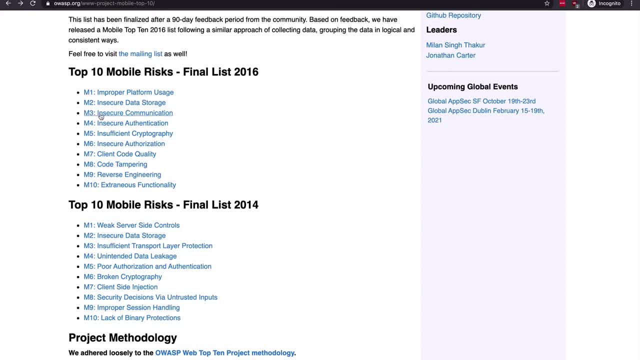 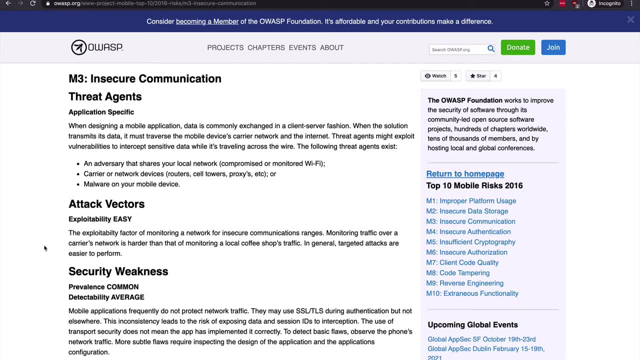 Alright. the third and last one that we'll look at in this lesson is about insecure communication. This was the third highest violation in that report that we saw earlier, And insecure communication has to do with how data is transferred and the fact that attackers can intercept that data while it's traveling. 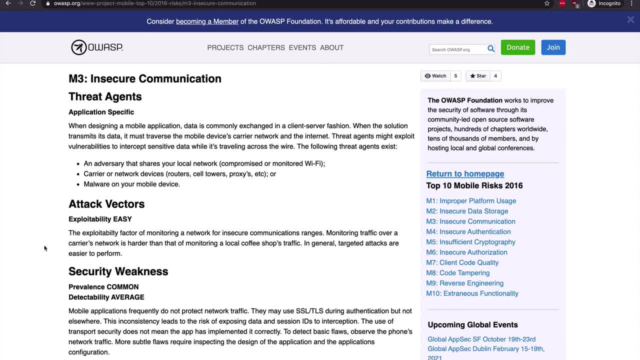 And this can happen if you're sharing a local network, such as a compromised or open WiFi that's being monitored- so think of coffee shops, hotels and so on- Or It could be carriers or network devices like routers, cell towers, etc. that are compromised. 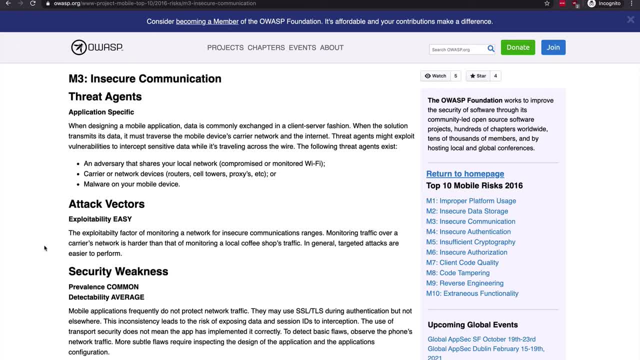 Or it could be that you have malware on your mobile device, So making sure that communication is encrypted when it travels is critical, especially if it is sensitive data. The problem is, you could implement secure protocols, but that doesn't ensure that the application is using it correctly. 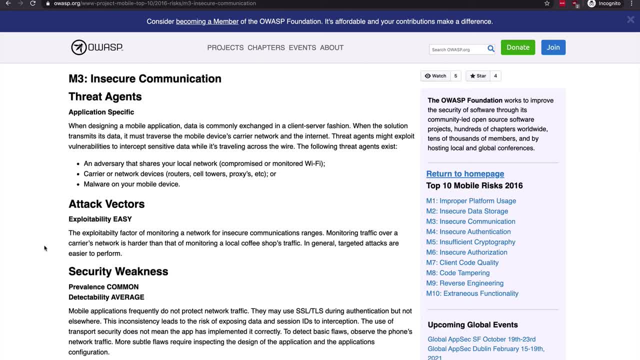 Perhaps the encryption setup was poorly done and so attackers can do what's called a man-in-the-middle attack. Be sure to look that up if you're not familiar with secure protocols. If you're not familiar with secure protocols, be sure to look that up if you're not familiar. 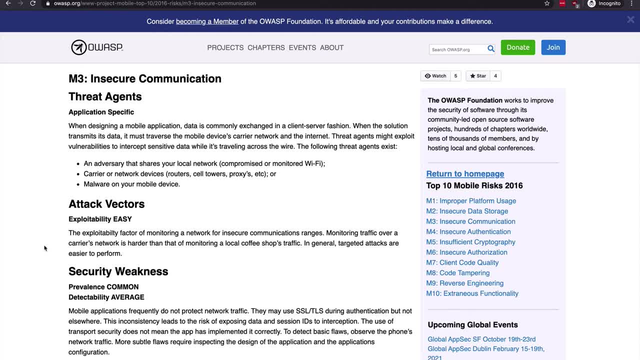 with what a man-in-the-middle attack is. Or perhaps the encryption is properly configured, but the application uses a call that does not go through that encryption. There's a number of different scenarios that we have to be cautious of and test for when we're building mobile apps. 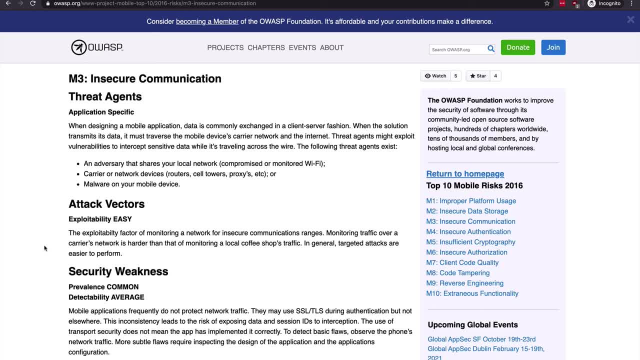 And, by the way, this is not just for WiFi connections. it's important for Bluetooth, NFC, 3G, audio and really any other type of communication technology that a mobile phone might use. So go ahead and review this page, Just like we've been doing for the other two risks. 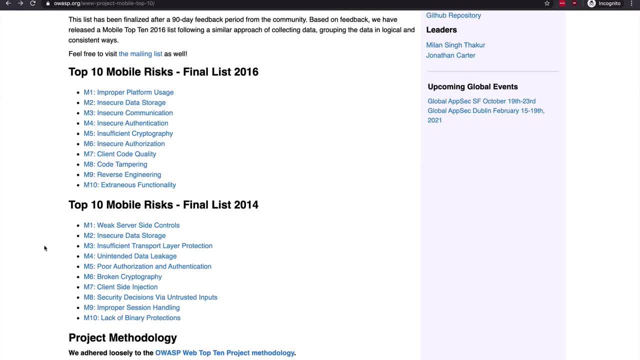 And then be sure to review the other seven risks as well. The other seven risks have to do with insecure authentication, insufficient cryptography, insecure authorization, client code quality code tampering, reverse engineering and extraneous functionality. Especially look at the extraneous functionality one because it was the third highest violation. 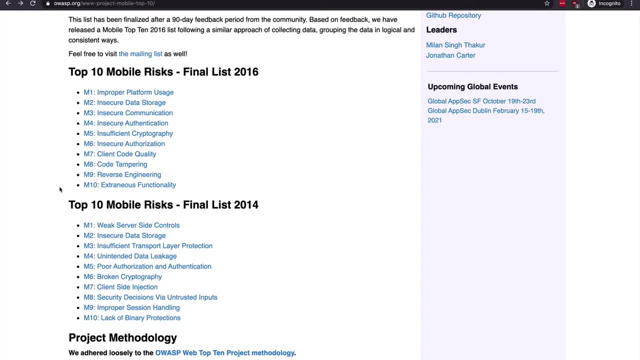 in the report that we saw earlier. But, as I say that, Do keep in mind that that doesn't necessarily make it the most important risk. The other risks are also just as important And as you go through these, think about how you could apply them to your current or future. 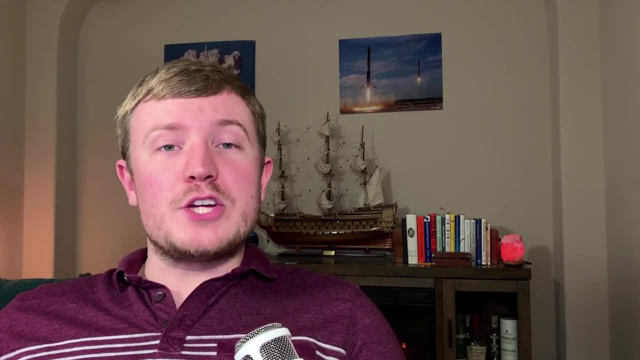 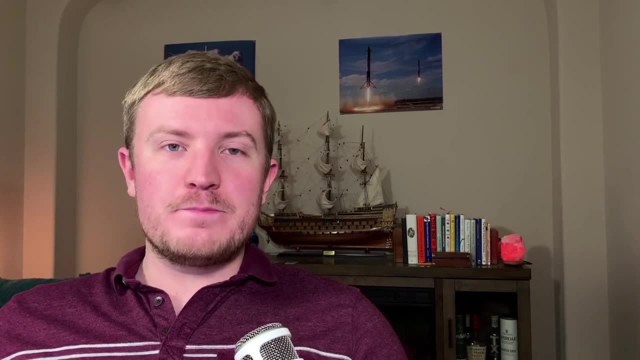 mobile applications. You can even think back to some of the older applications that you've worked on, where maybe they had some of these vulnerabilities, but you weren't aware of the risks And so you just didn't realize it. And once you're familiar with these risks, go ahead and mark this lesson as complete. 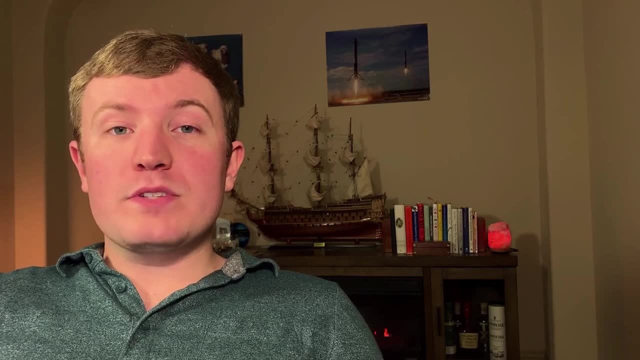 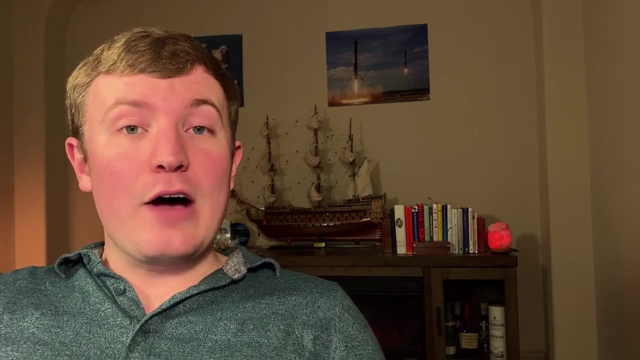 and I'll see you in the next one. Given that the public cloud platforms can be accessed- Can be accessed from the open internet, Identity and access management, also known as IAM, is more important now than ever. Users can connect from almost any location and any device, even if they are not company. 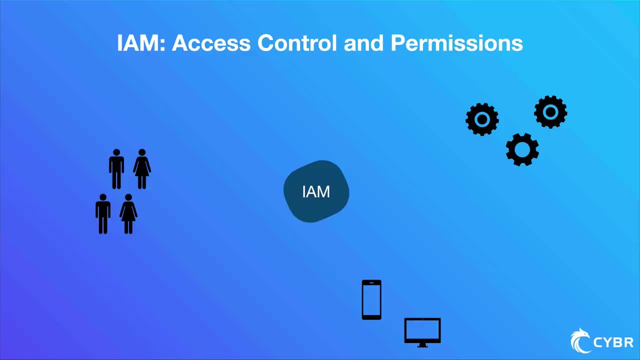 owned, and the same goes for systems. So, to help with this, the major cloud providers being AWS, Azure and Google cloud- bundle IAM with their services. This means that you have a central location where you can manage access, controls and permissions And, as you use, 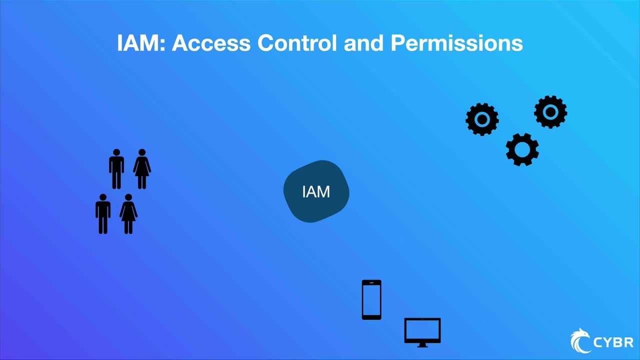 Or deploy more services, you have to define what those access, controls and permissions look like. IAM follows the principle that everything and everyone gets an identity. So if an individual needs access to something, they get an identity, And if an API application or really anything else also needs to interact with another resource. 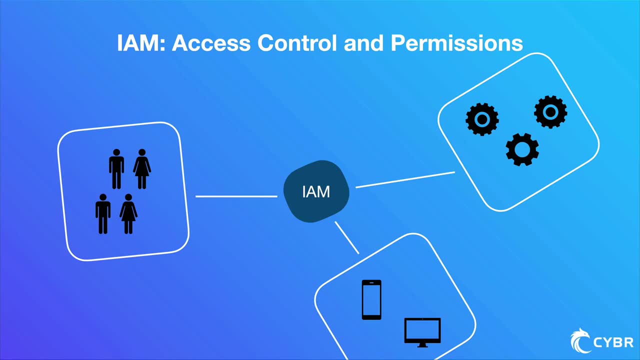 they also get an identity And, as verification occurs, IAM checks policies to identify the limits of that relationship. So let's say, for example, Let's say, for example. Let's say, for example, that you deploy an application to Amazon Web Services on a server. 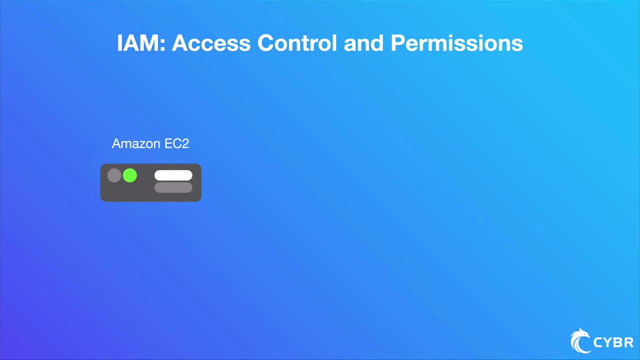 which they call EC2 instances. That application needs to access data that you've also stored on AWS with a service called Amazon S3.. In order to limit access to the data from your application, a best practice would be to create a role for your application to assume. 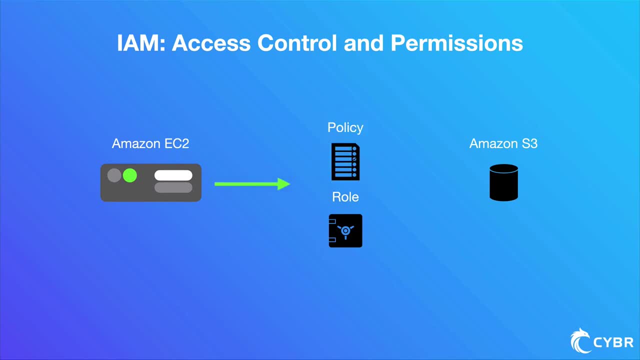 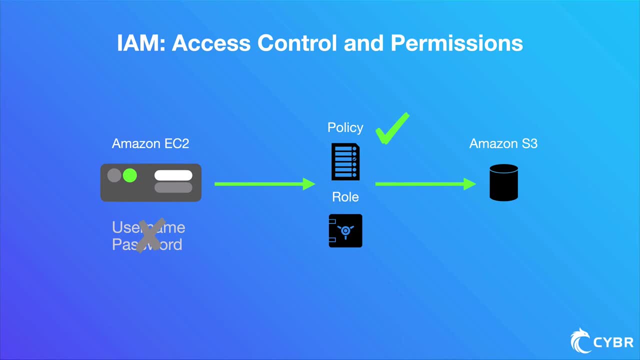 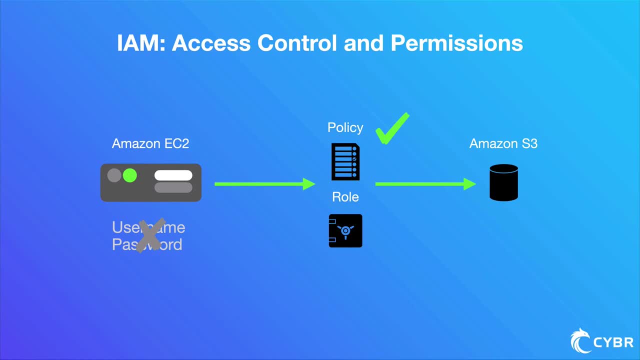 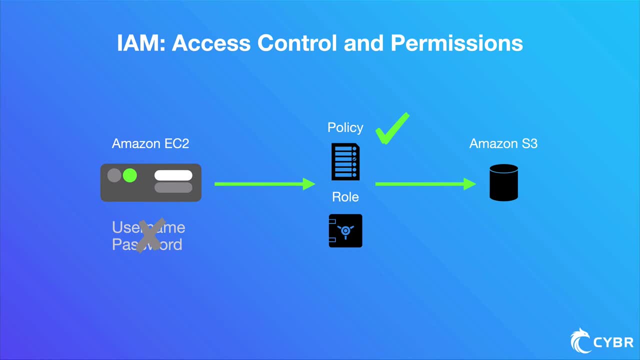 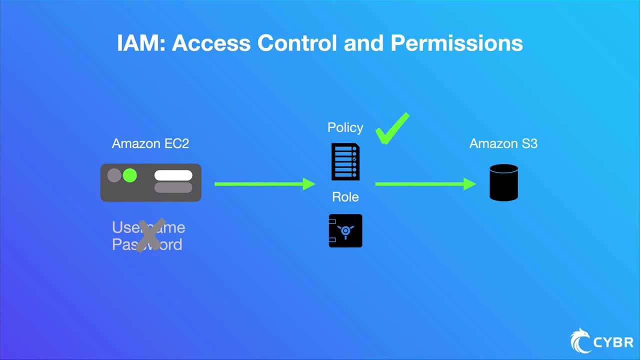 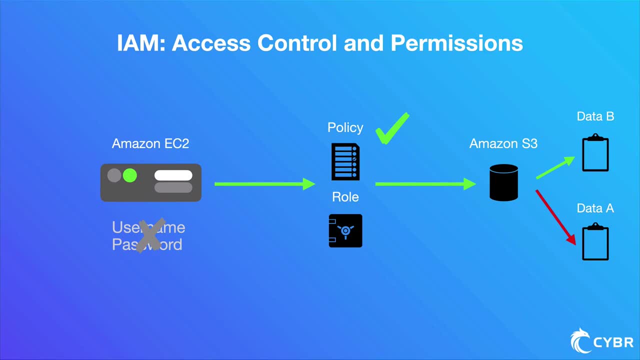 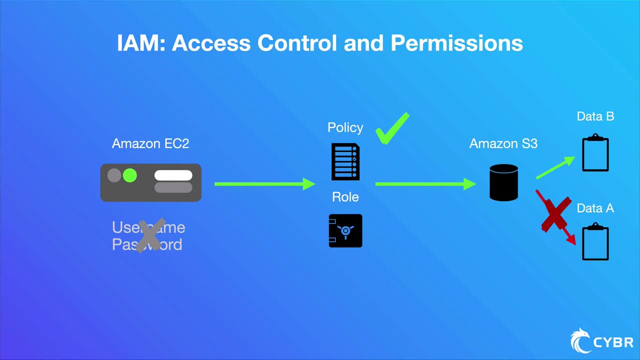 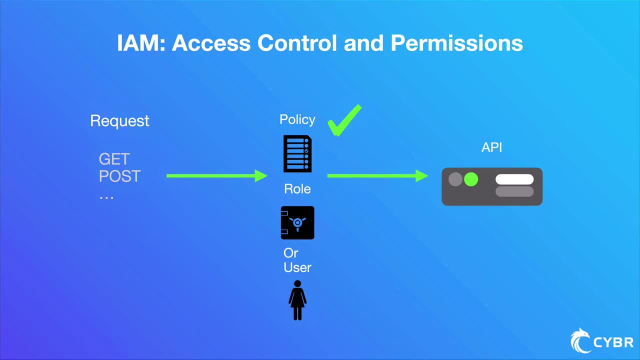 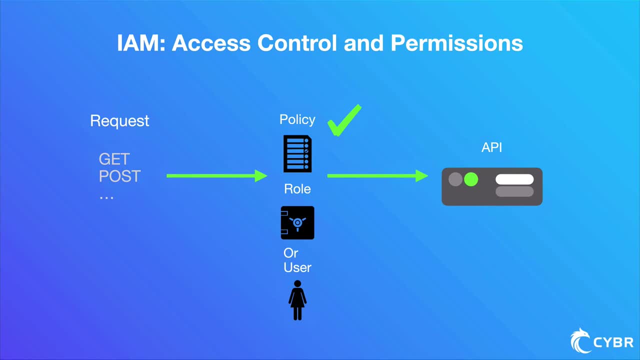 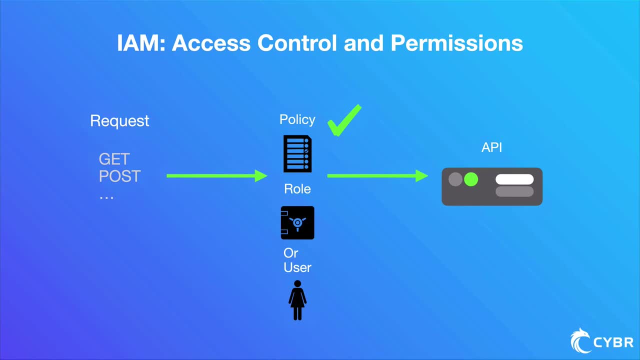 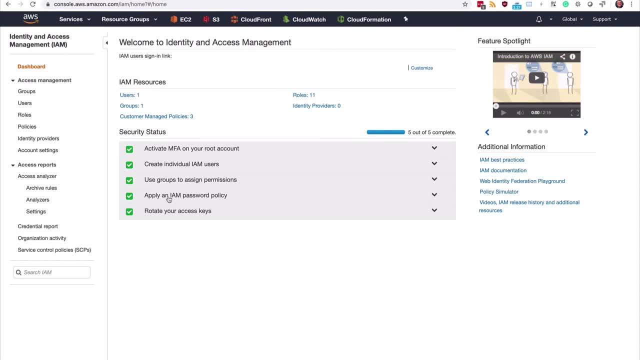 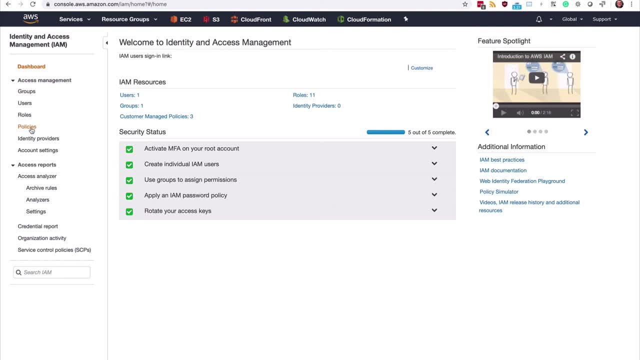 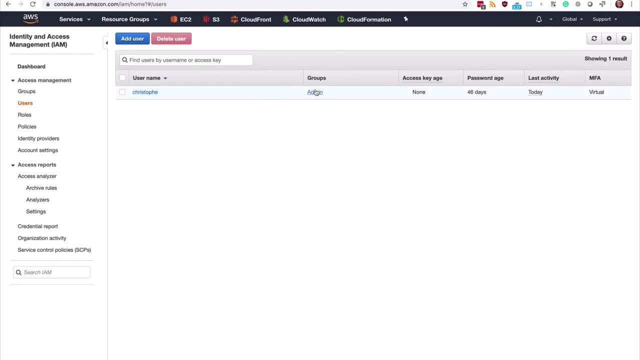 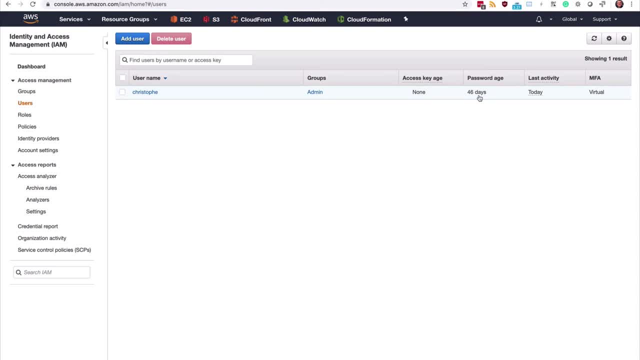 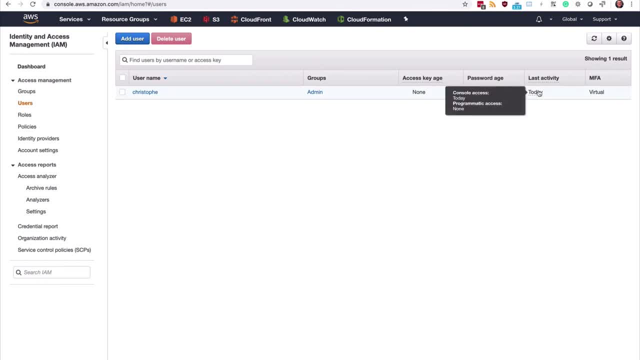 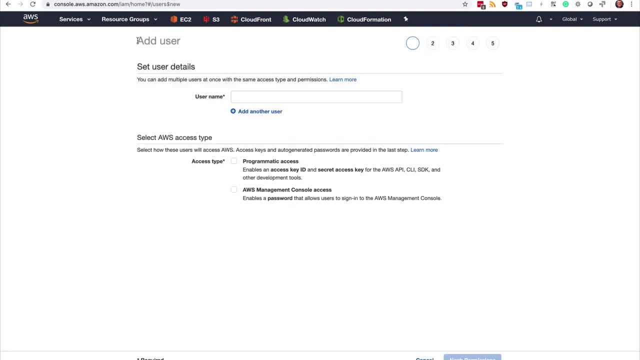 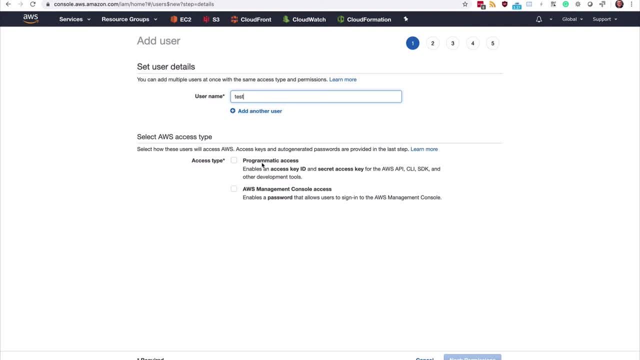 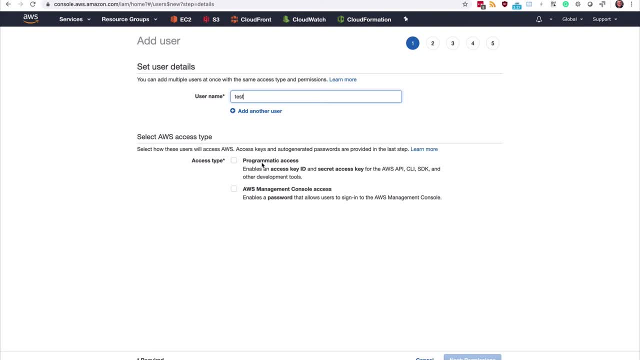 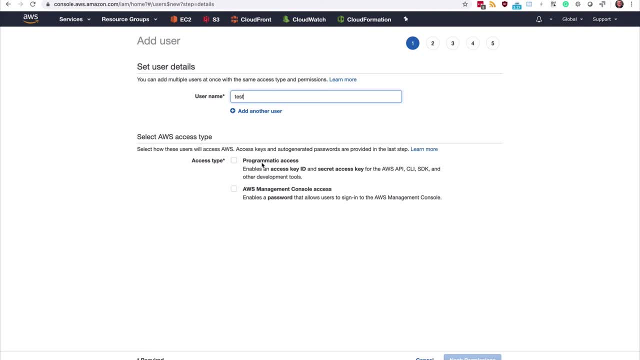 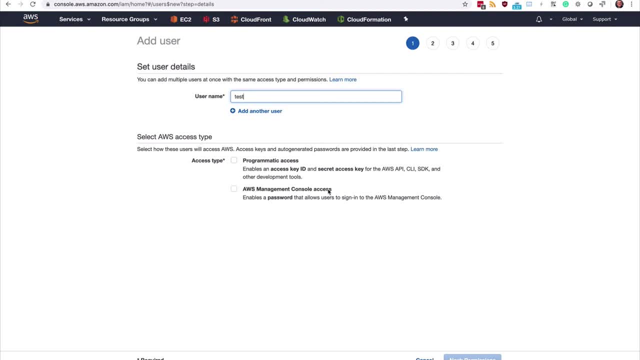 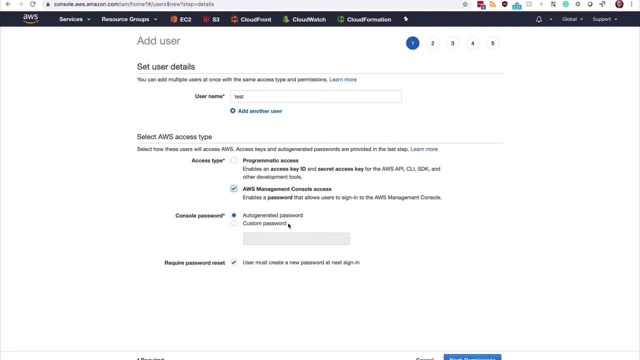 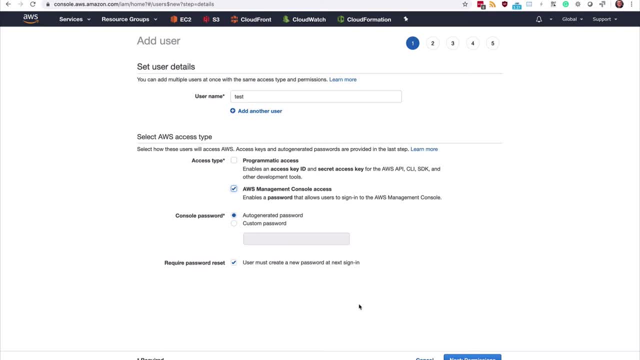 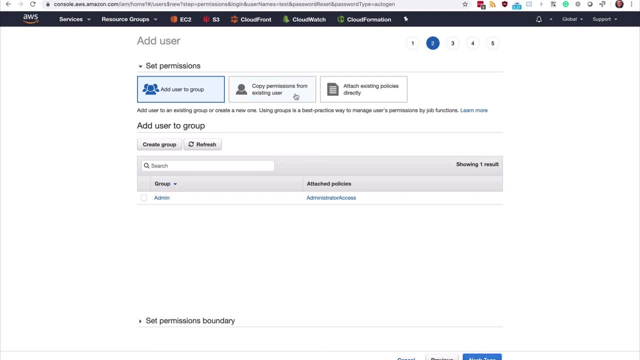 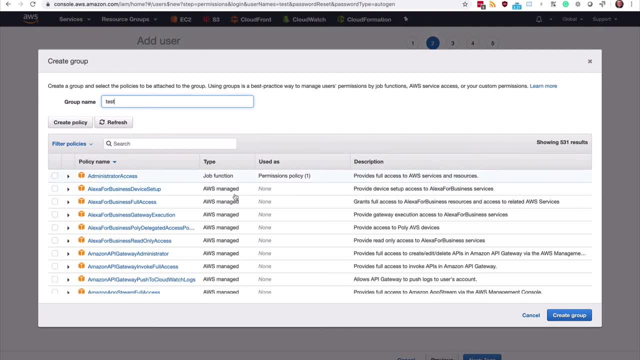 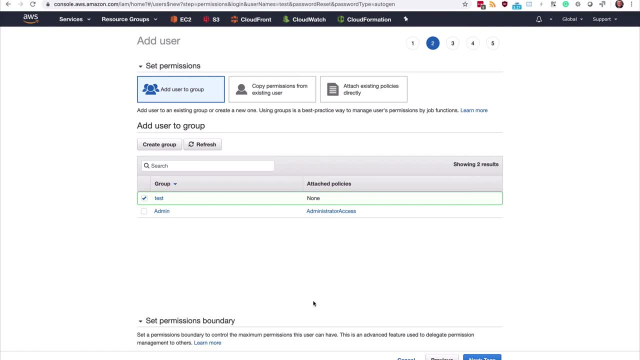 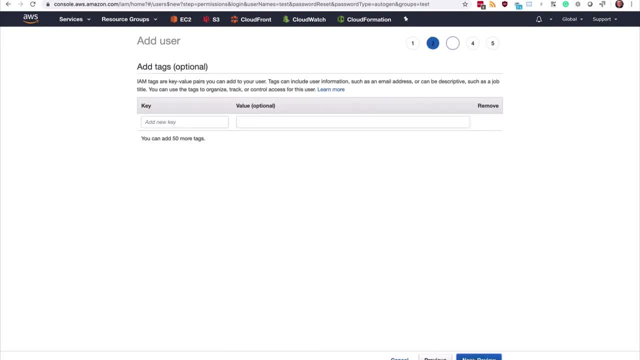 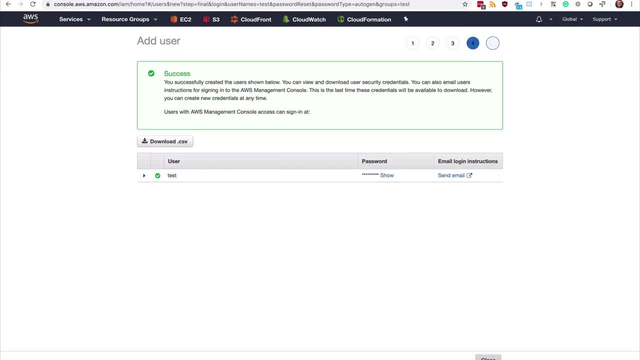 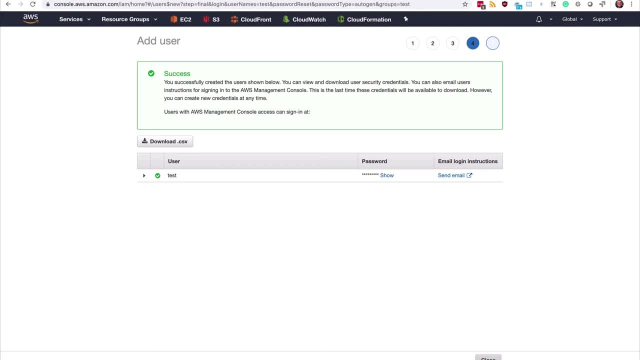 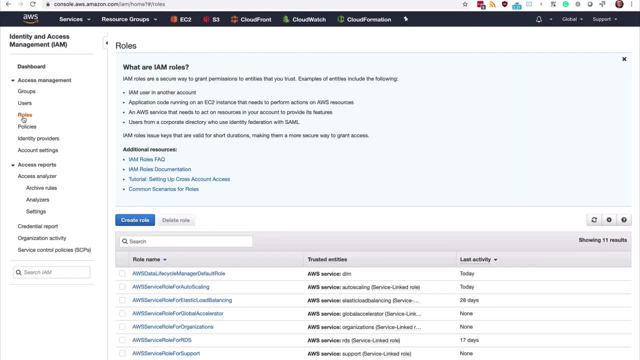 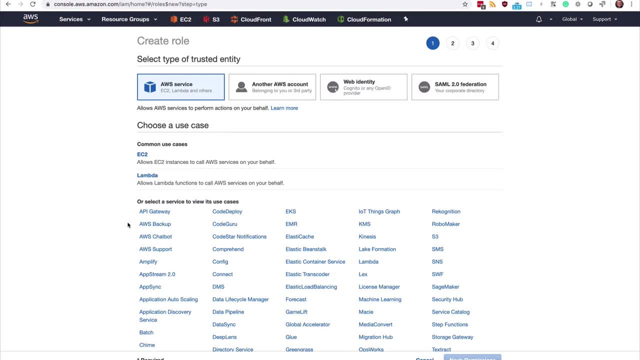 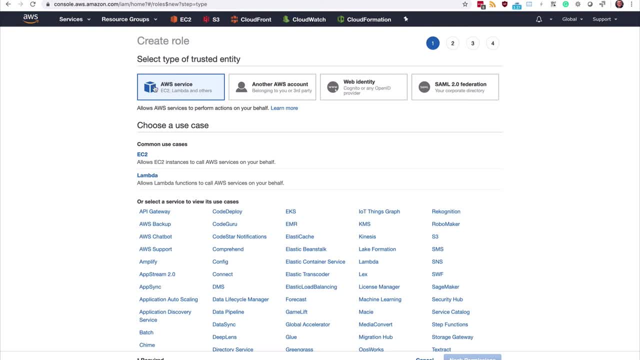 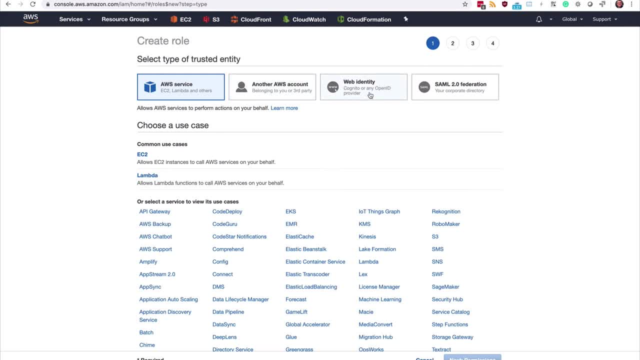 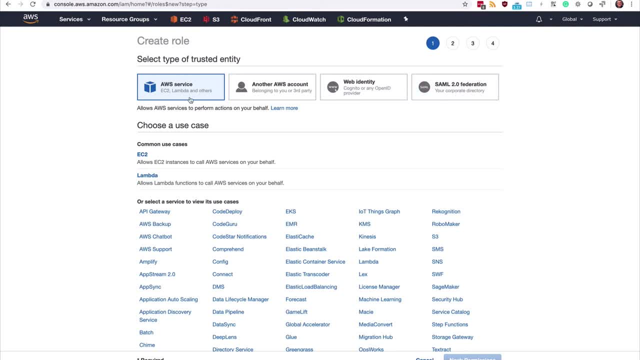 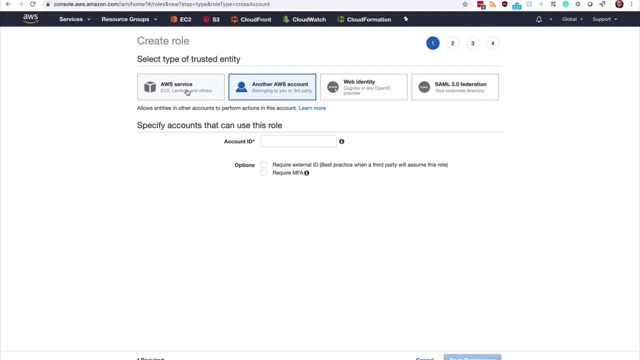 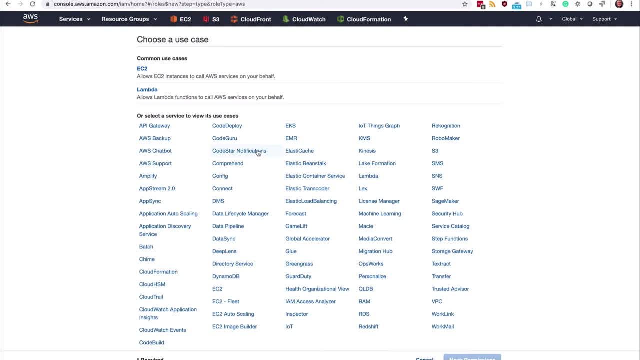 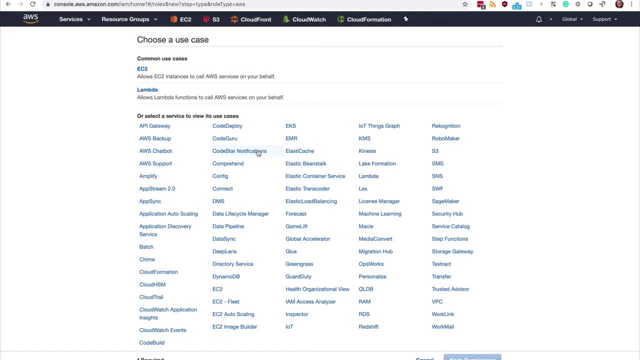 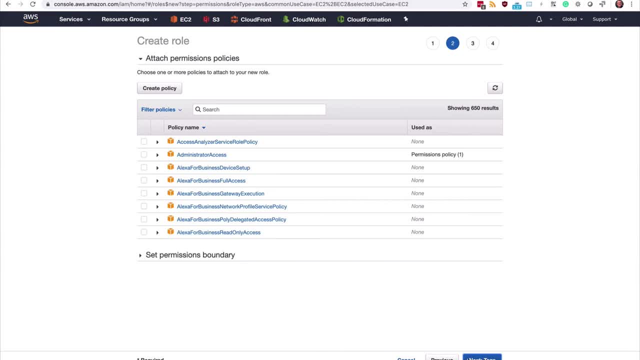 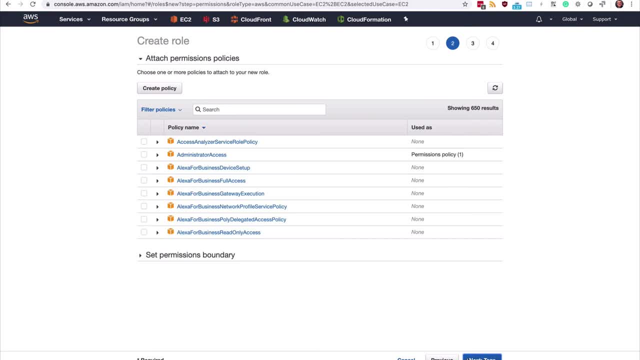 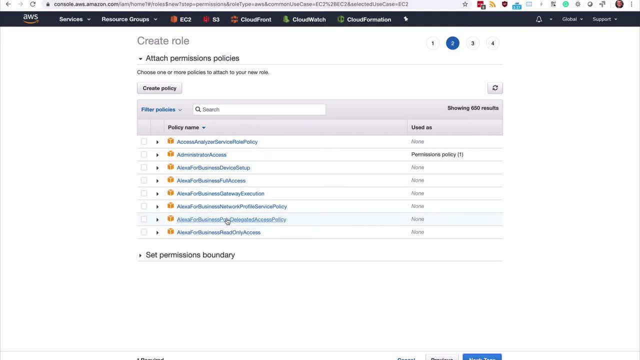 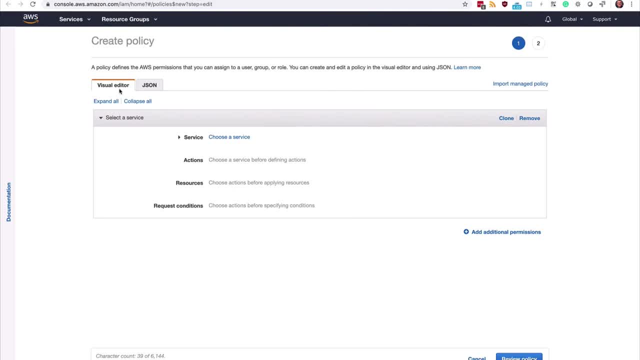 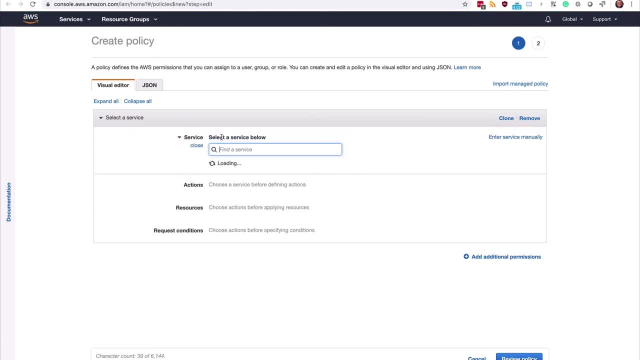 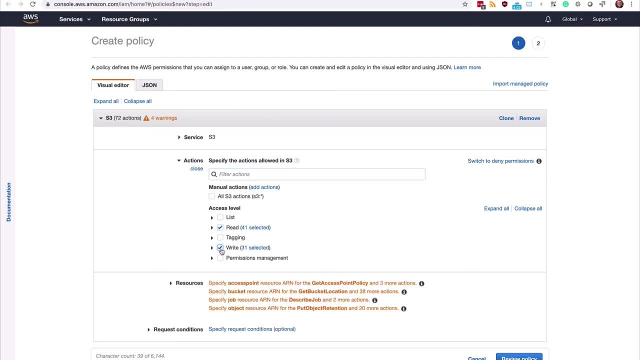 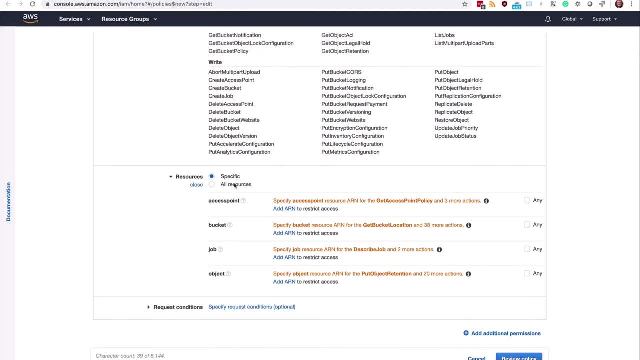 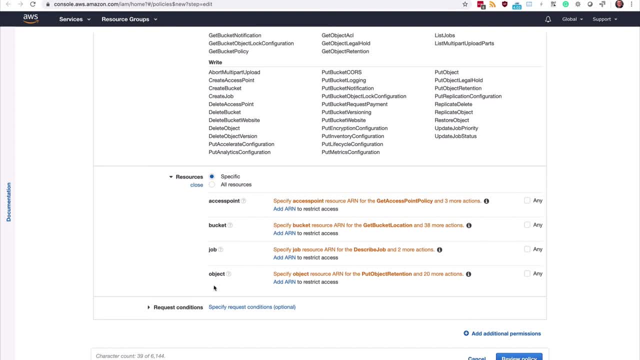 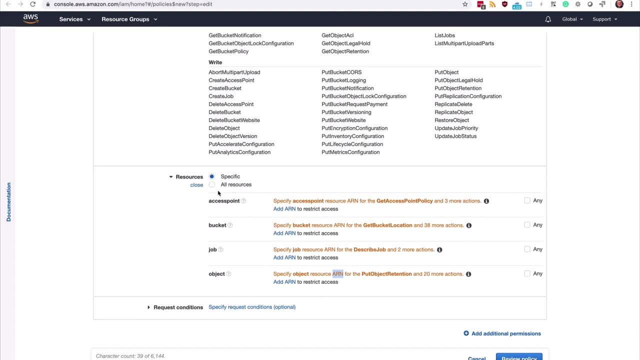 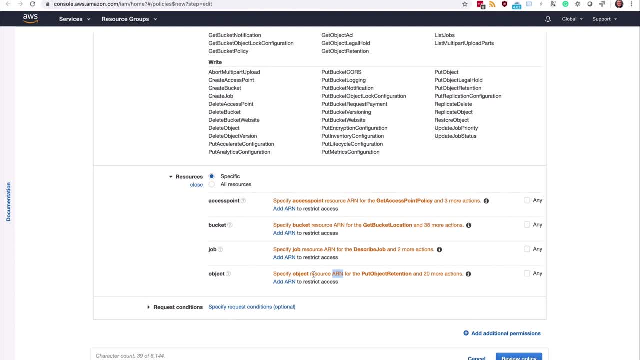 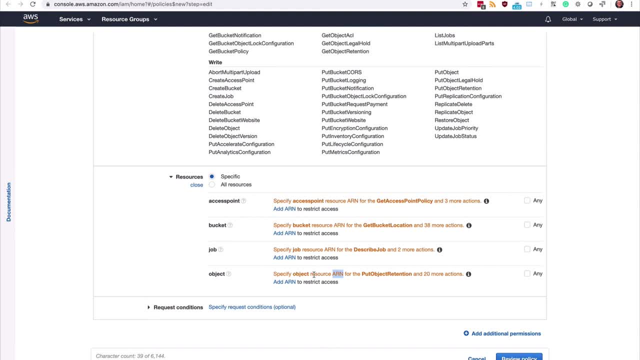 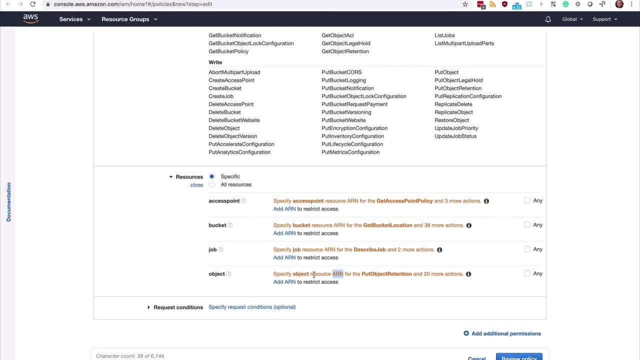 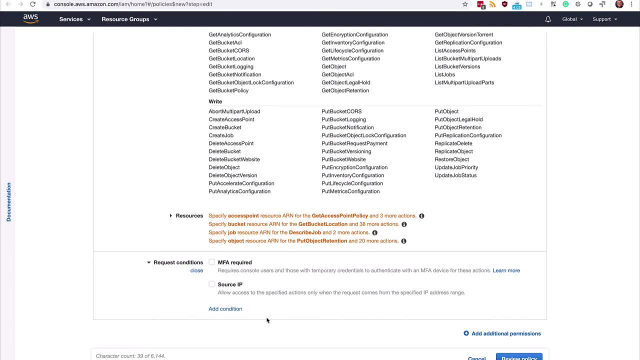 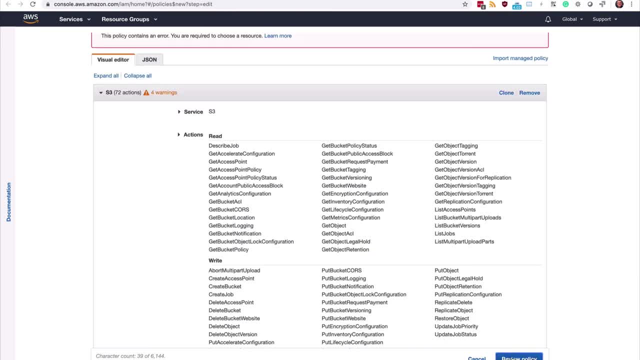 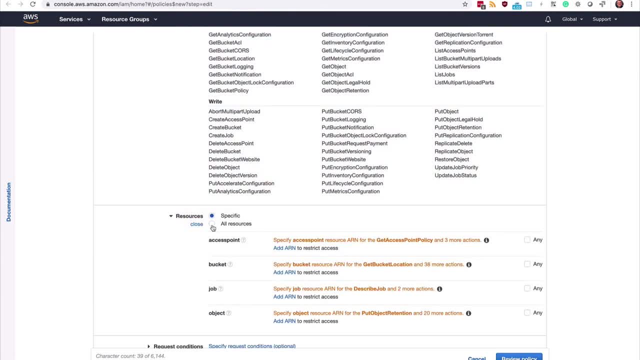 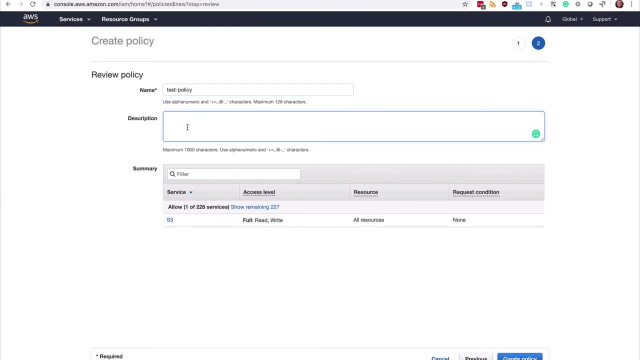 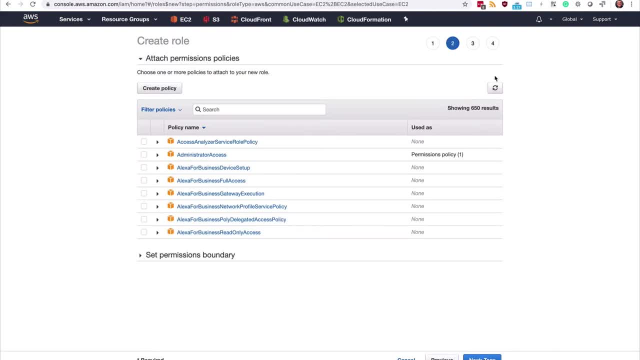 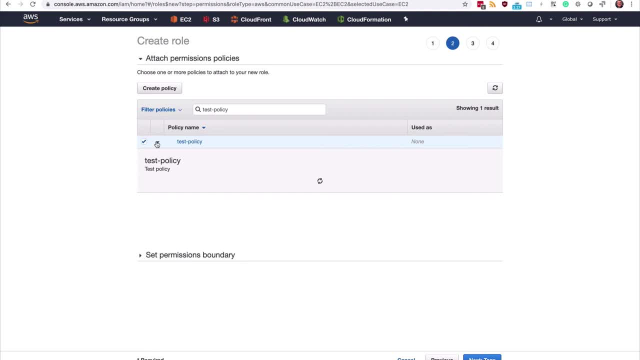 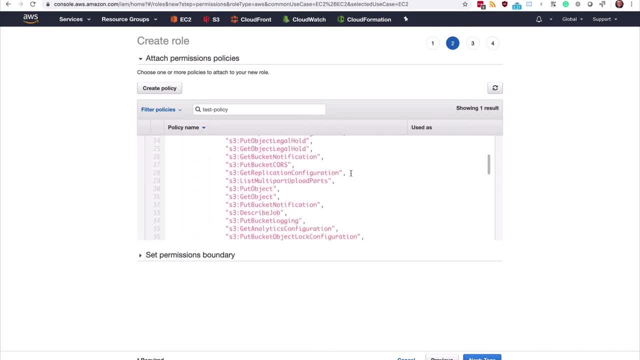 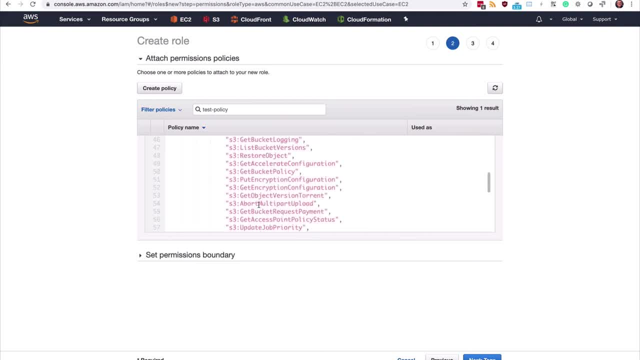 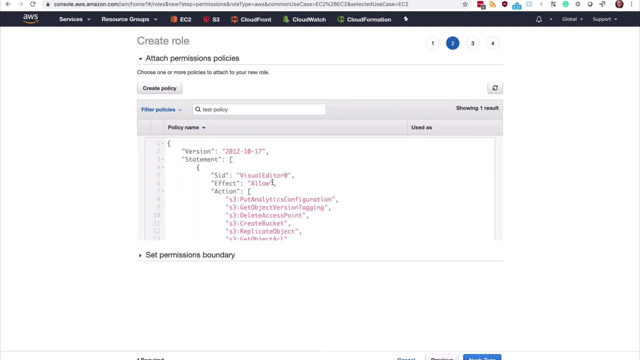 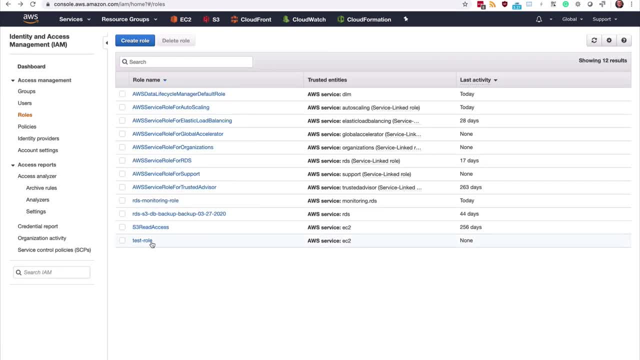 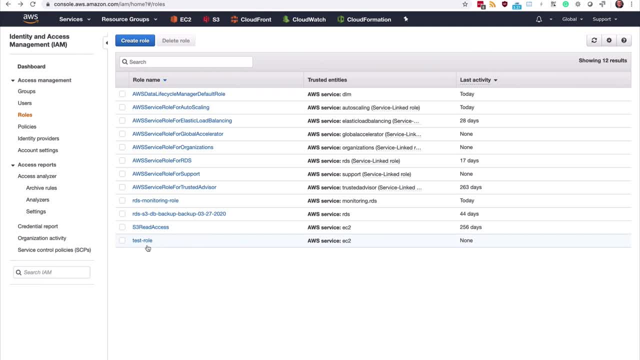 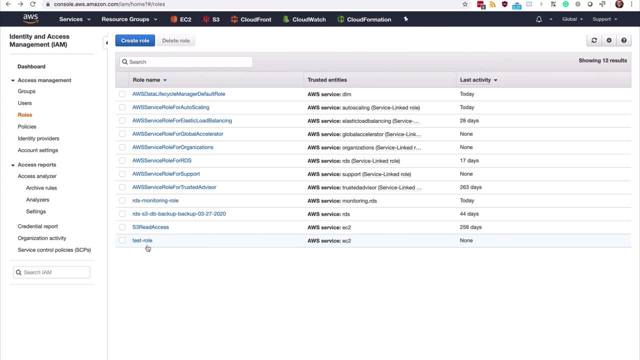 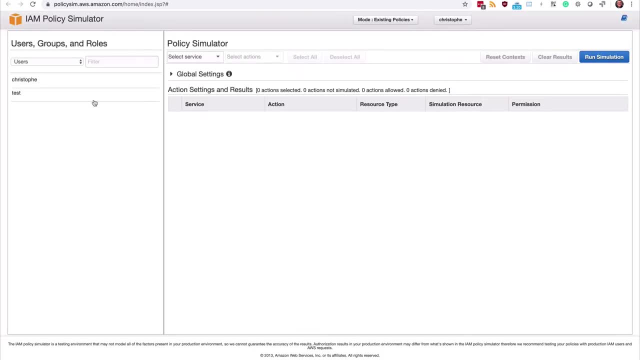 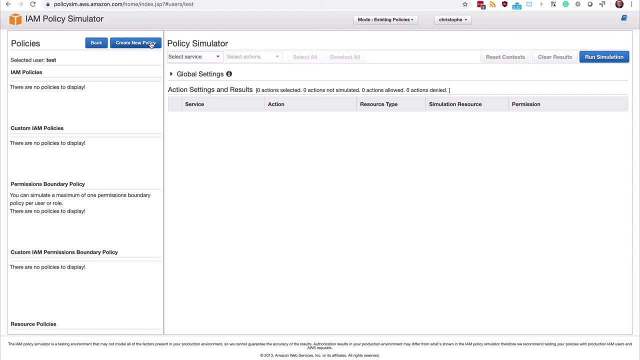 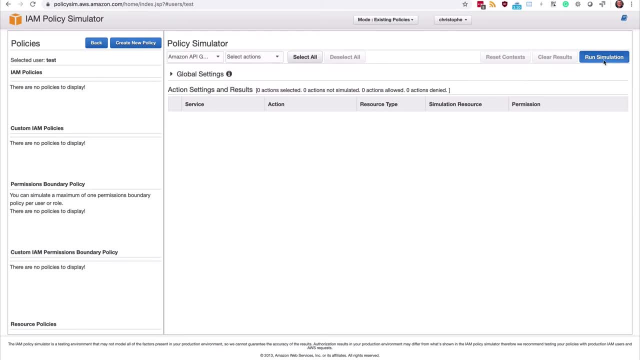 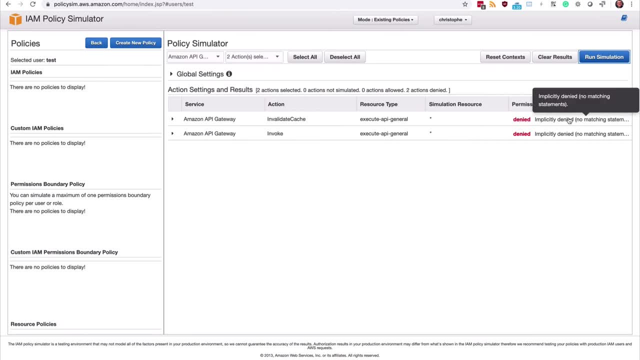 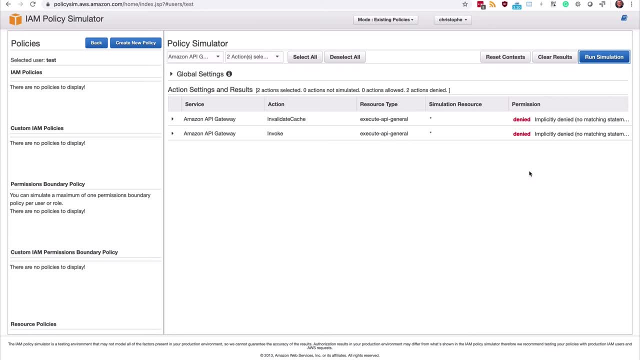 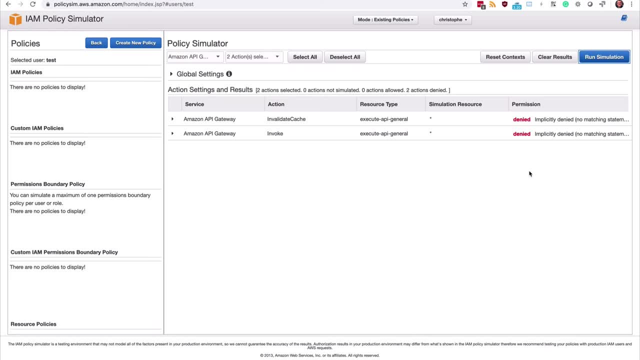 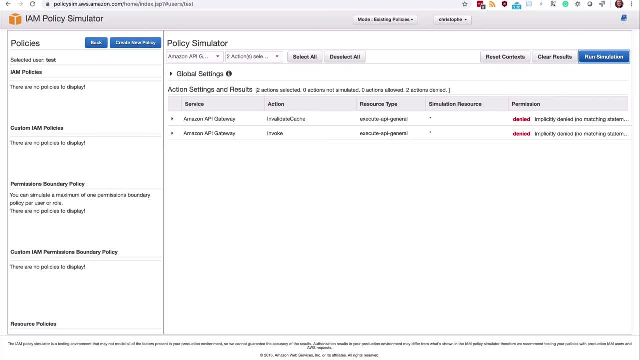 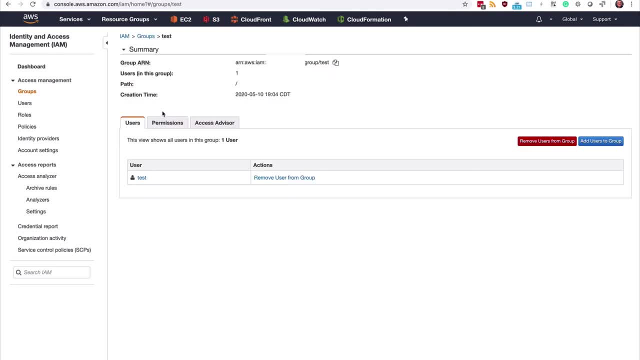 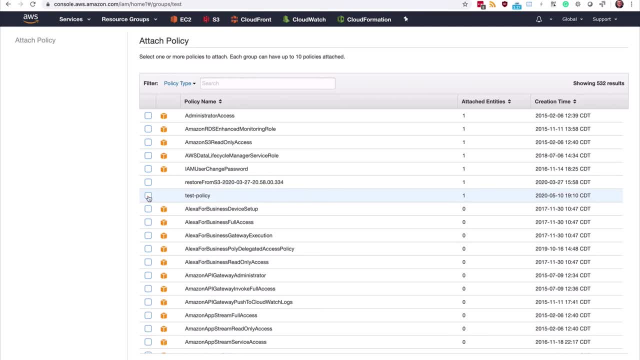 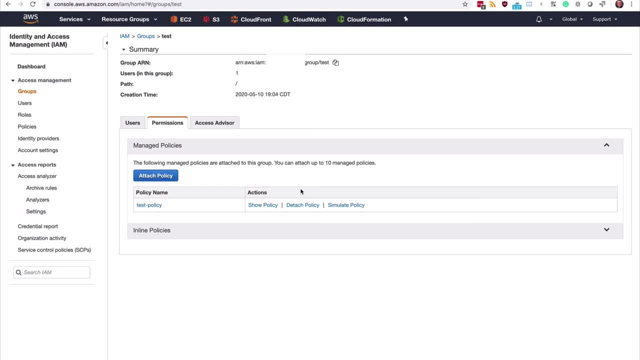 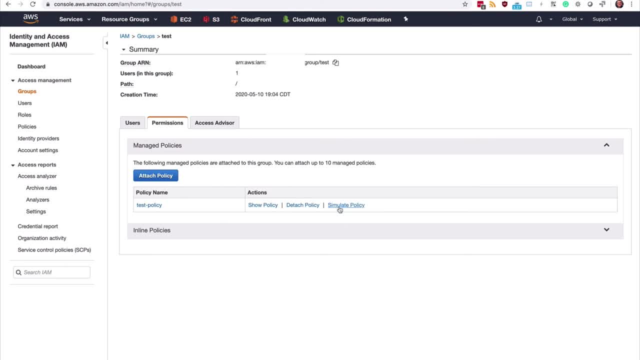 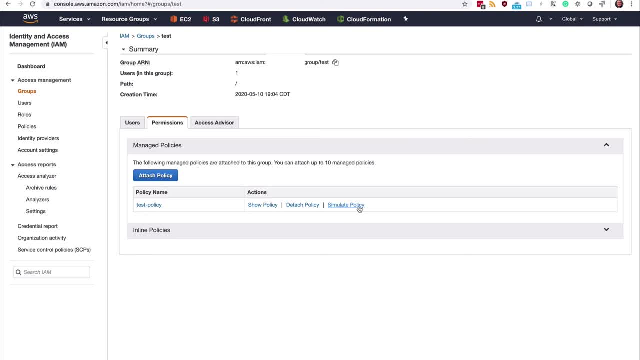 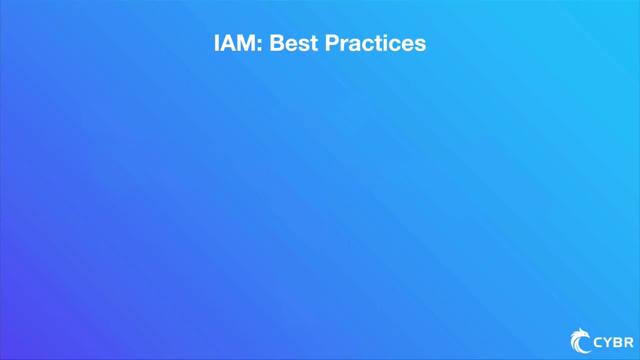 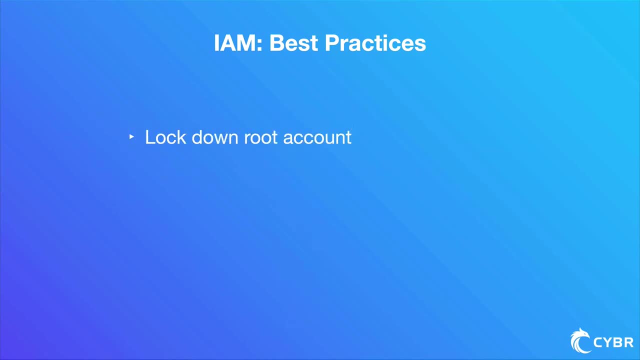 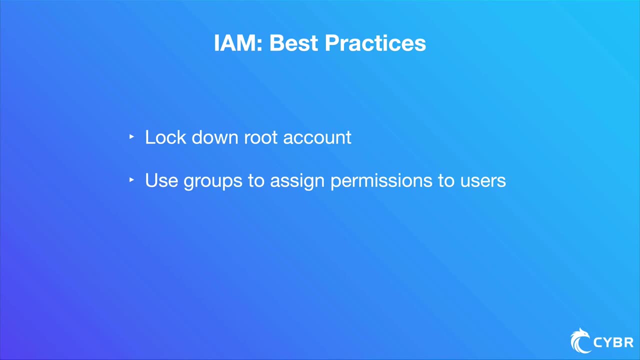 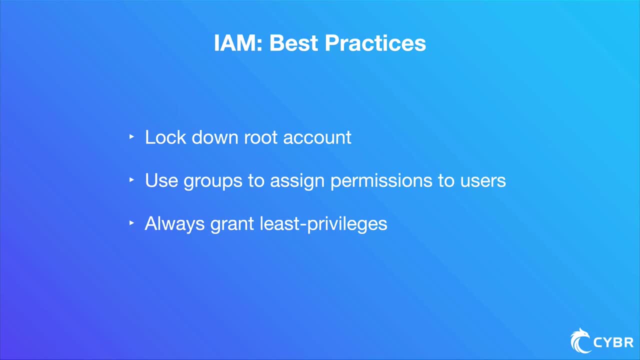 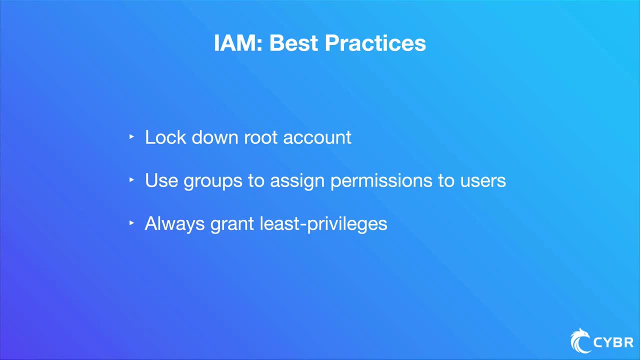 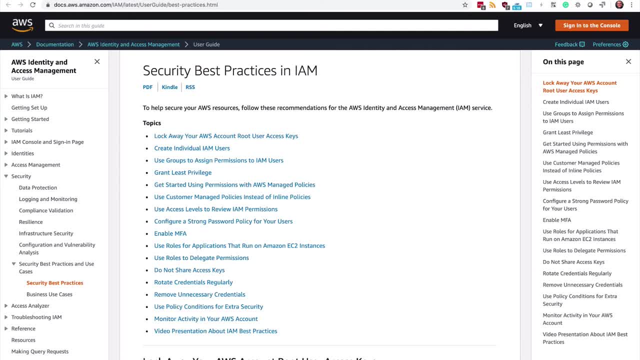 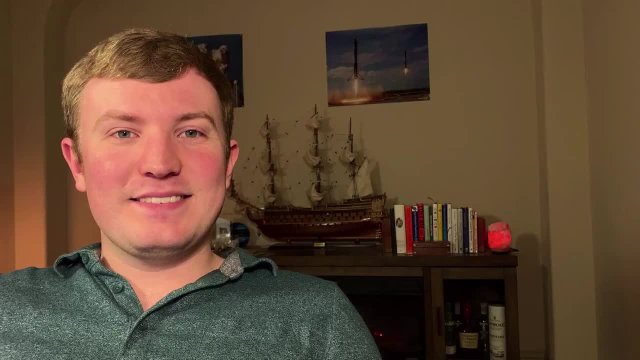 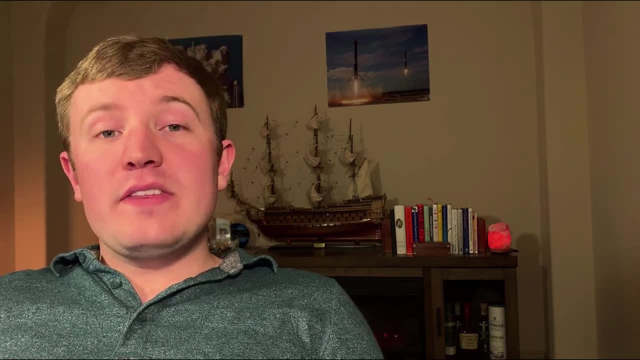 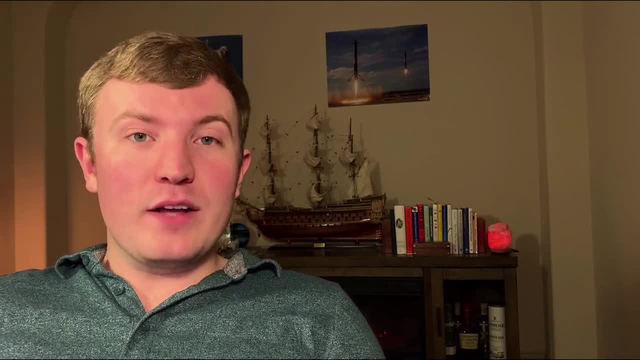 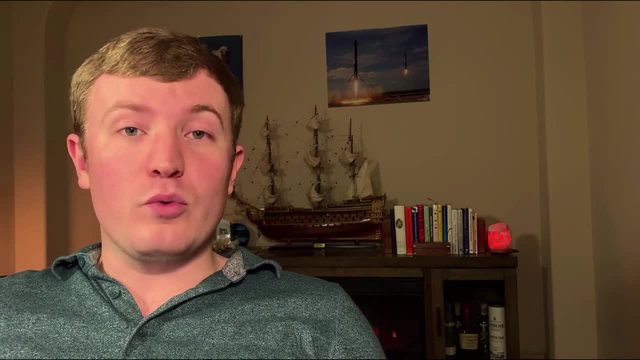 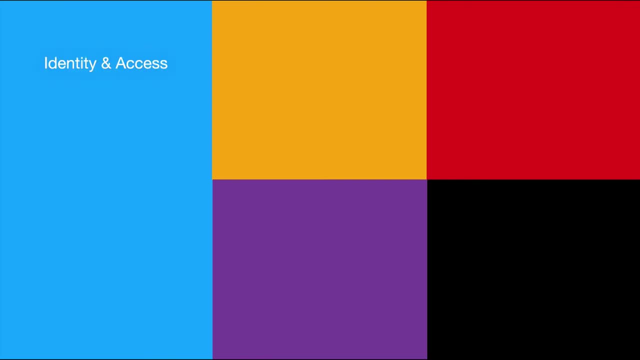 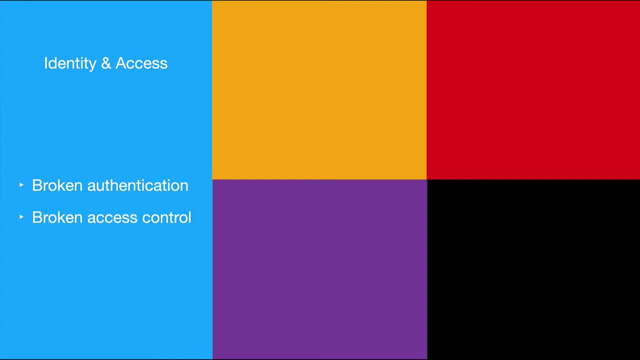 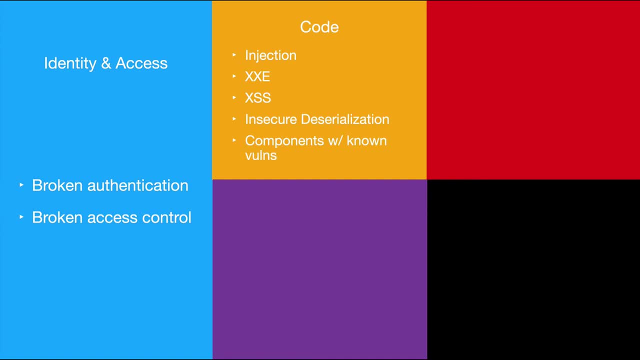 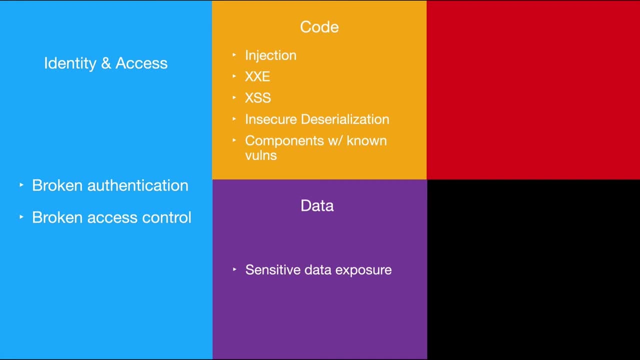 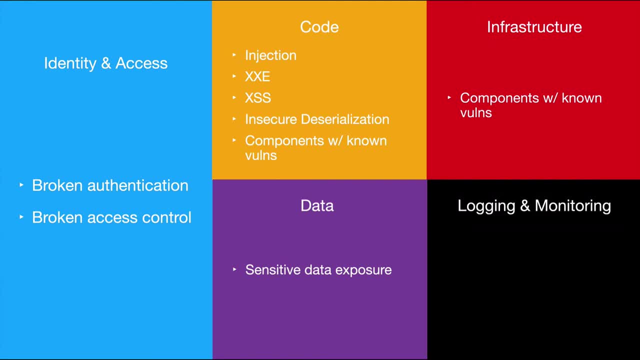 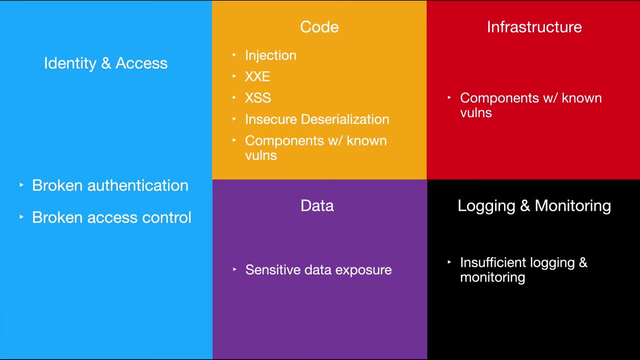 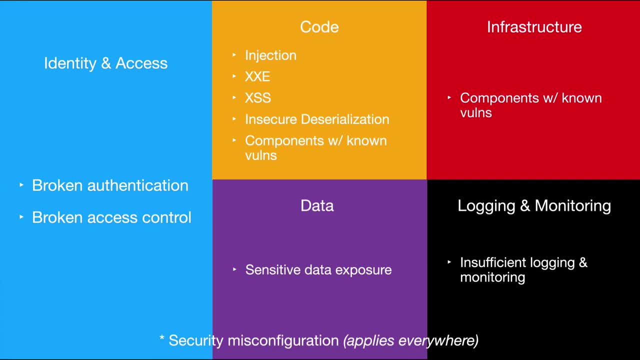 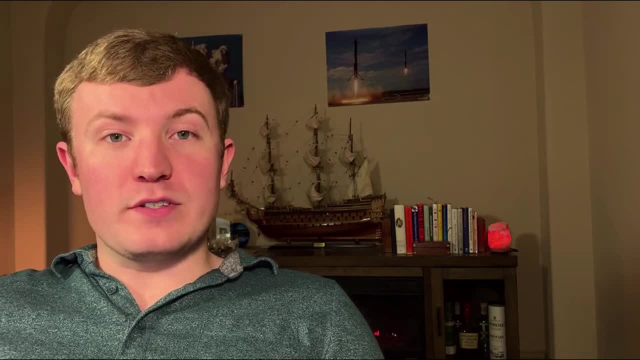 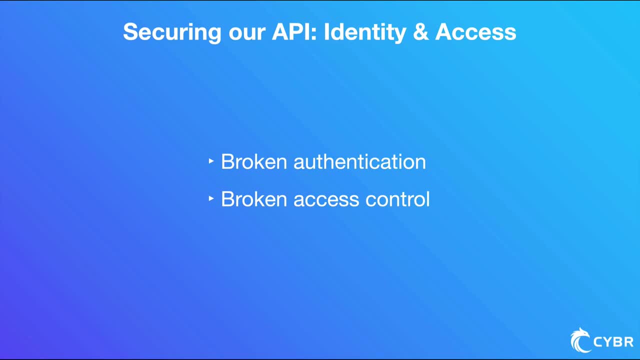 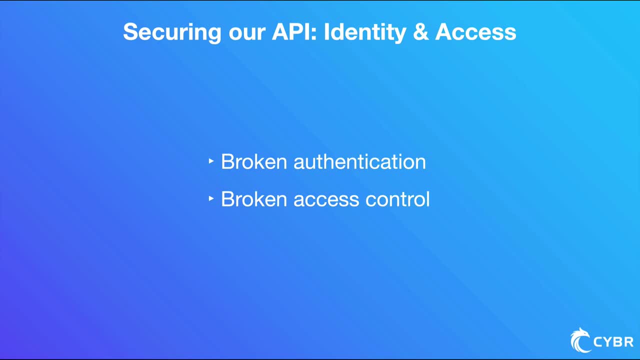 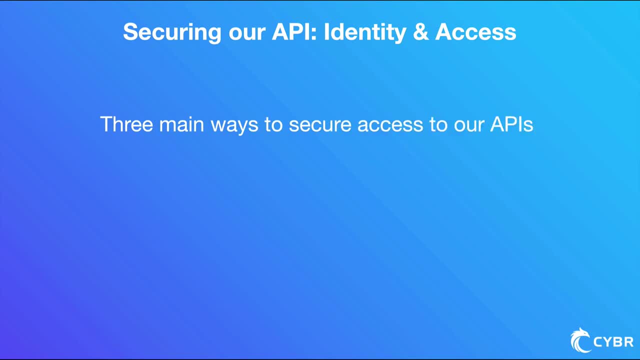 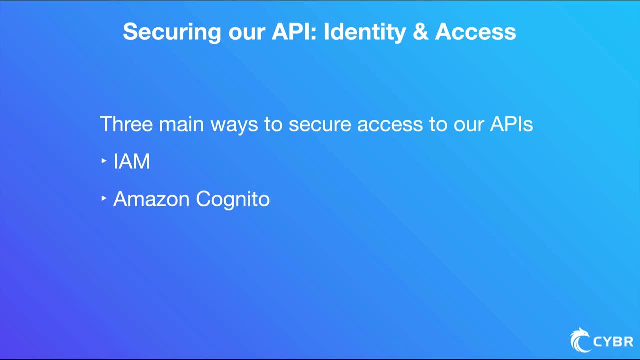 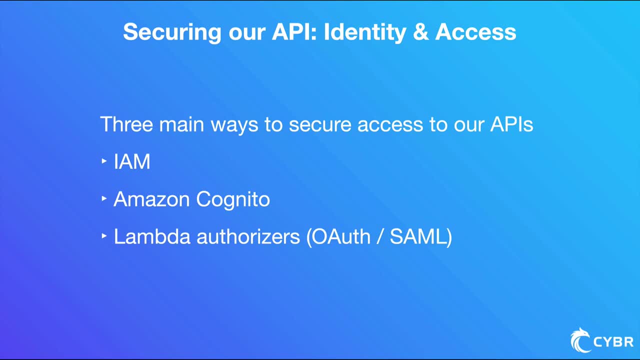 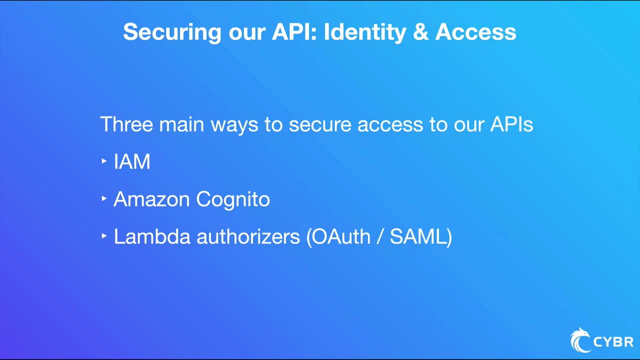 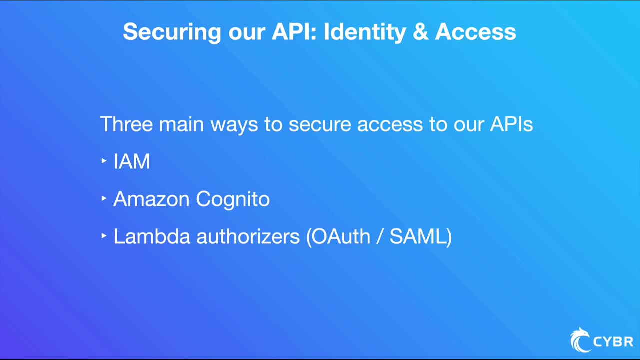 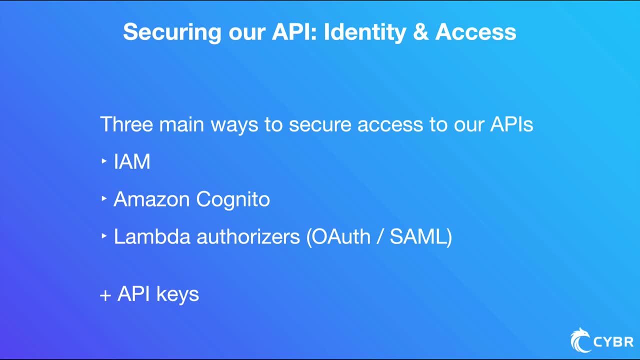 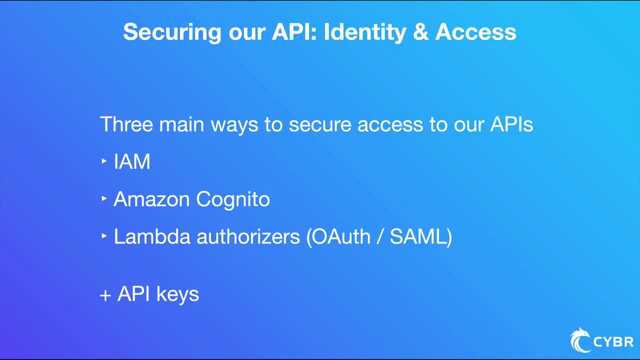 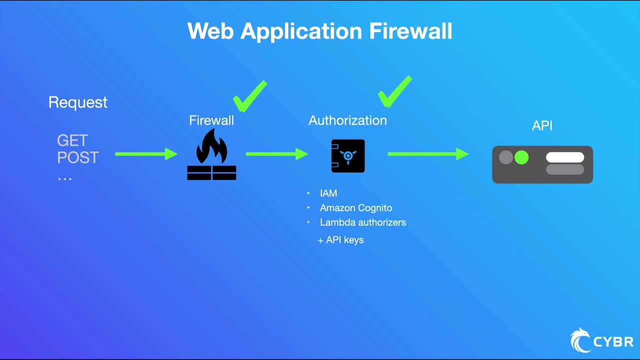 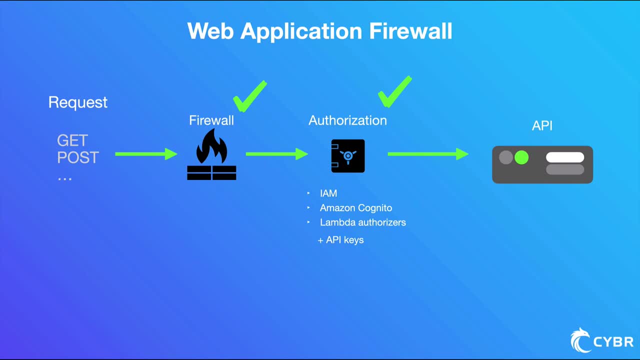 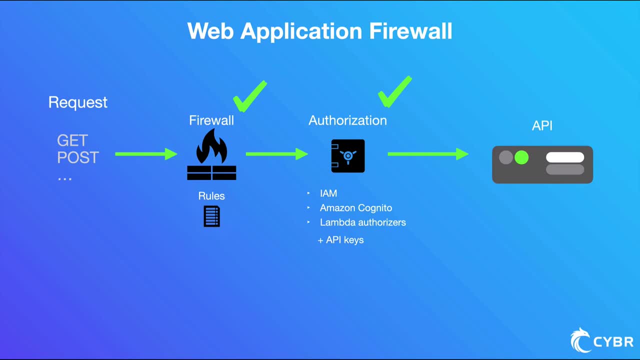 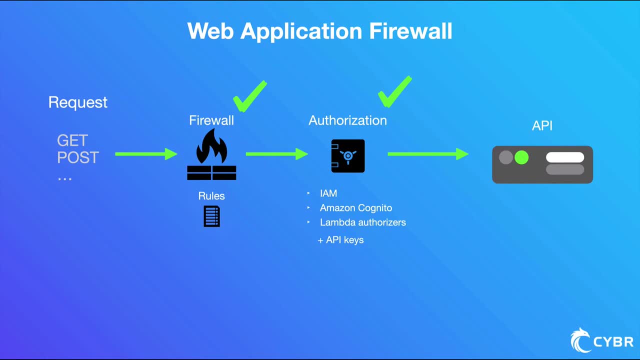 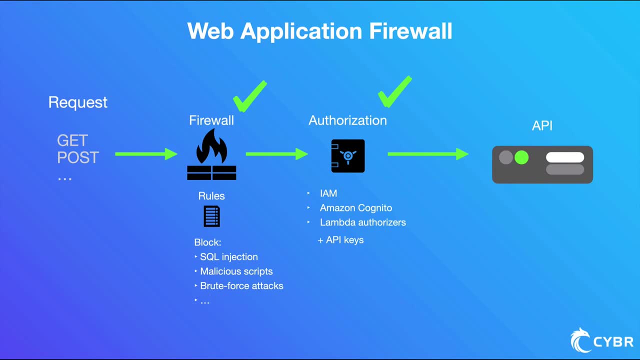 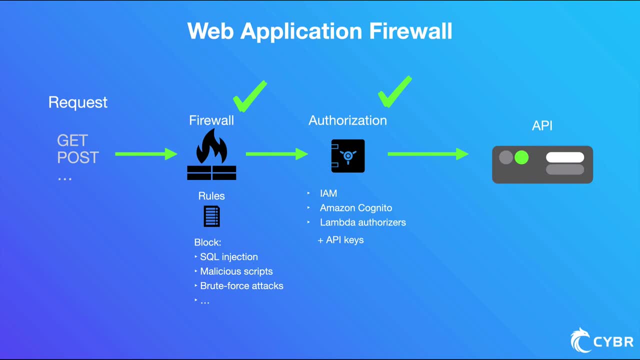 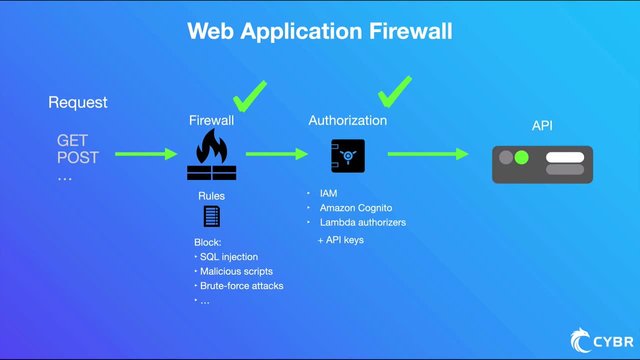 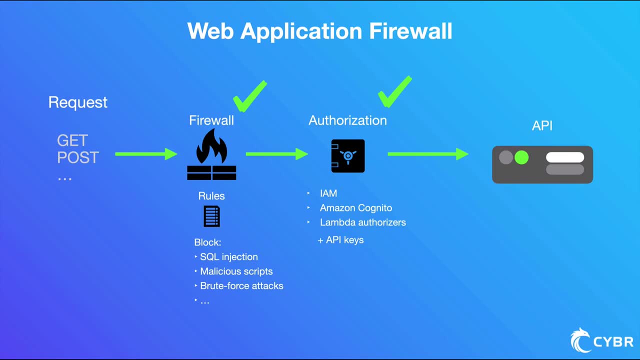 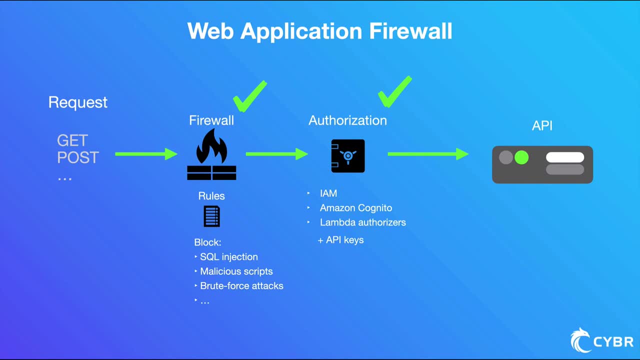 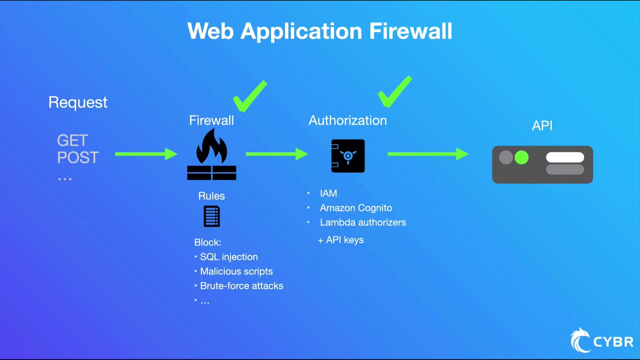 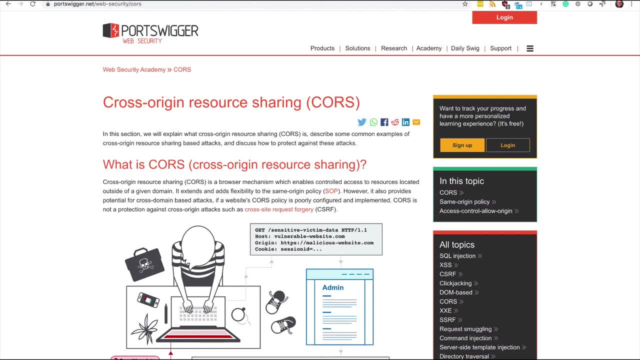 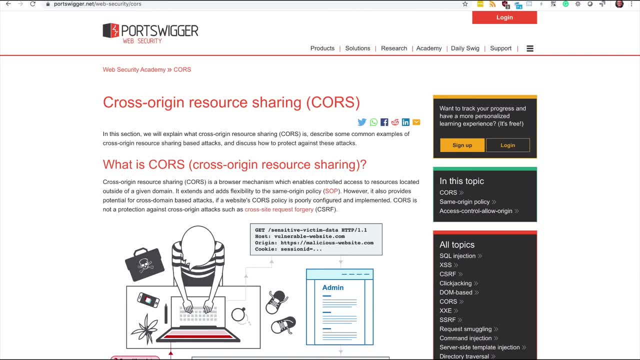 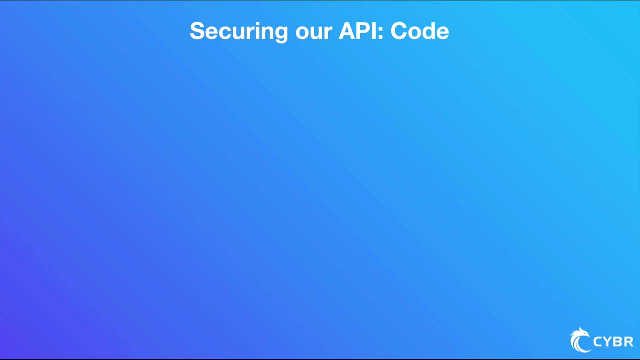 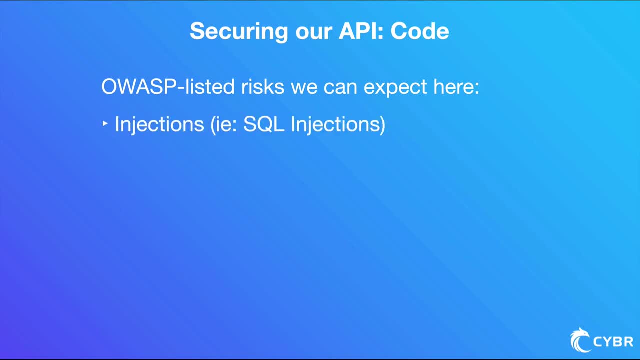 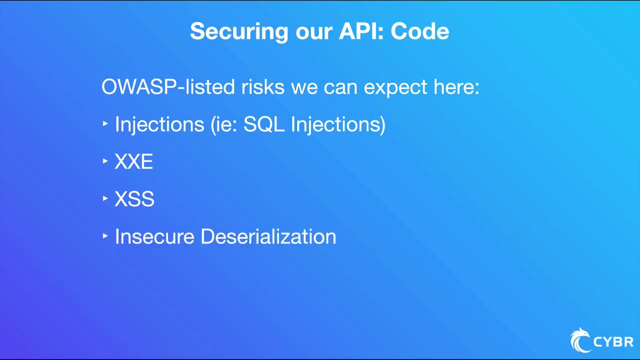 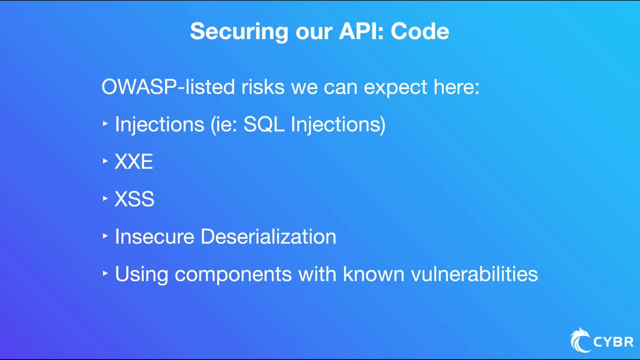 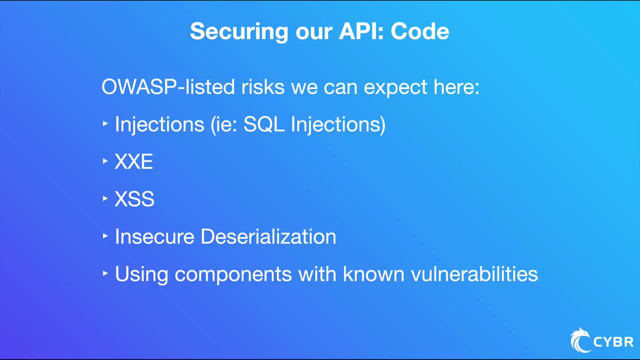 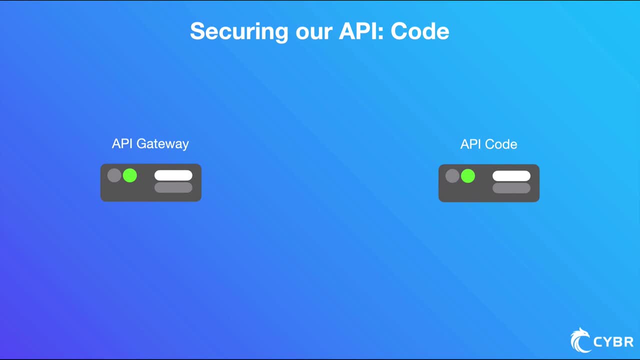 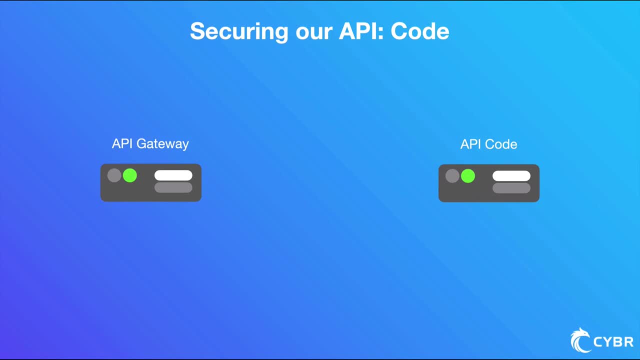 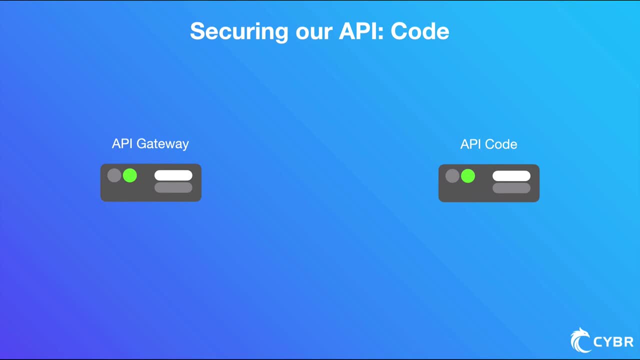 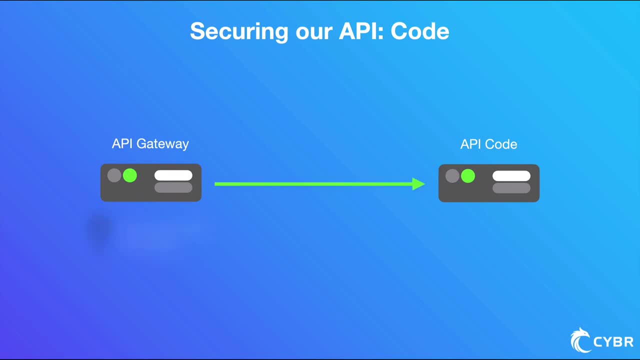 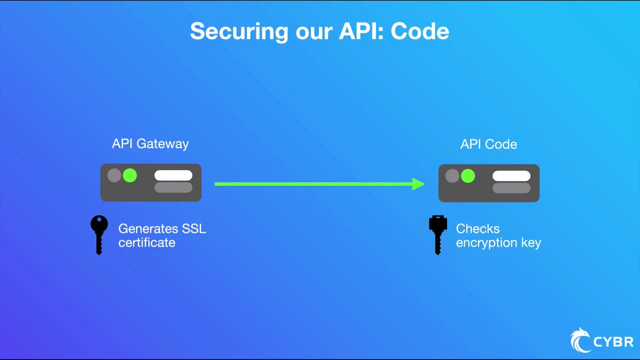 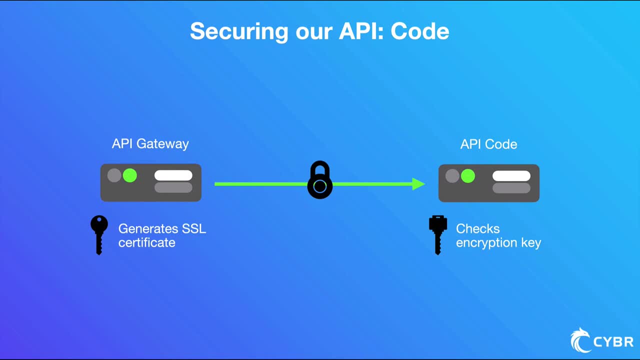 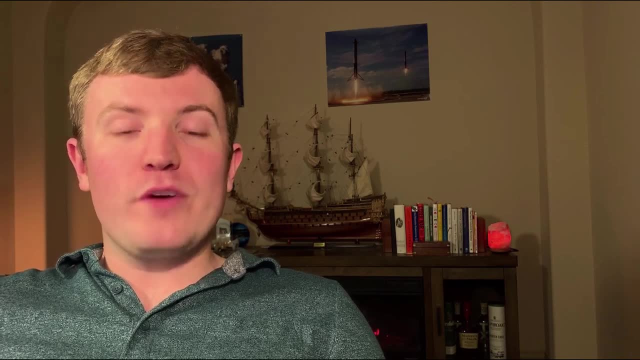 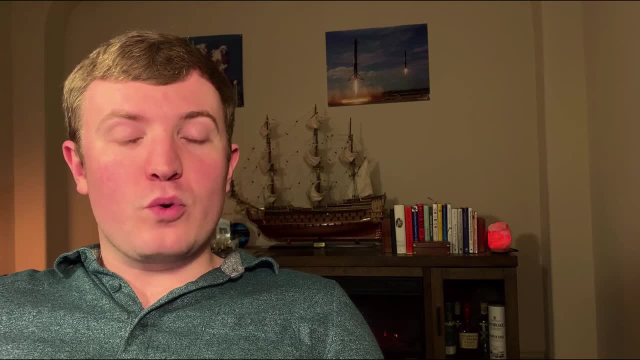 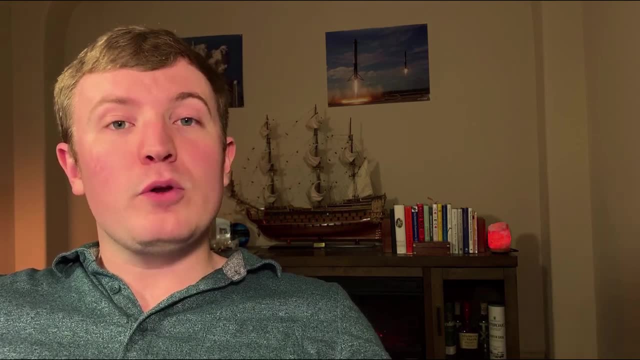 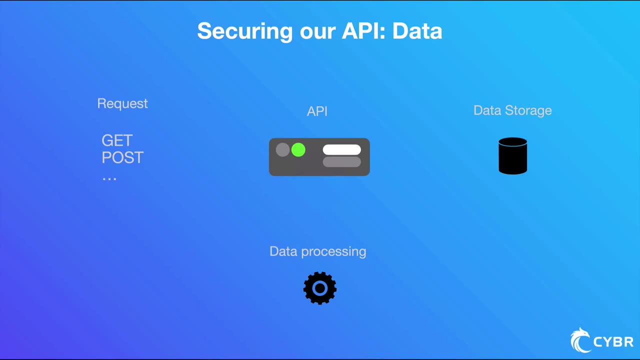 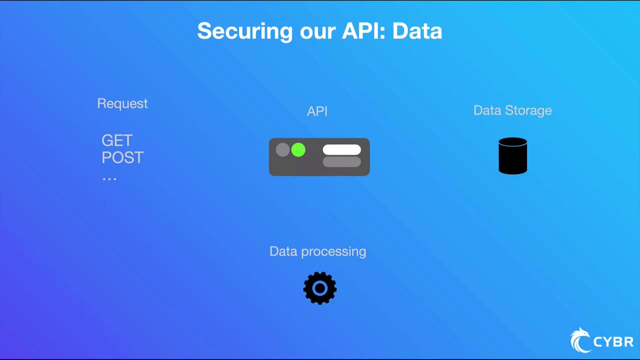 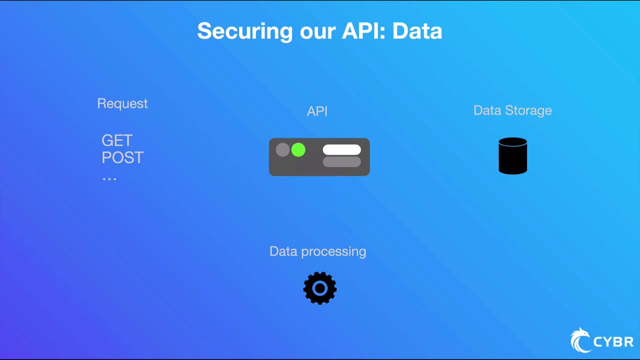 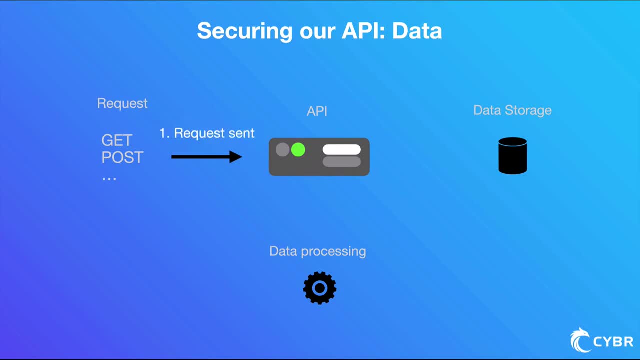 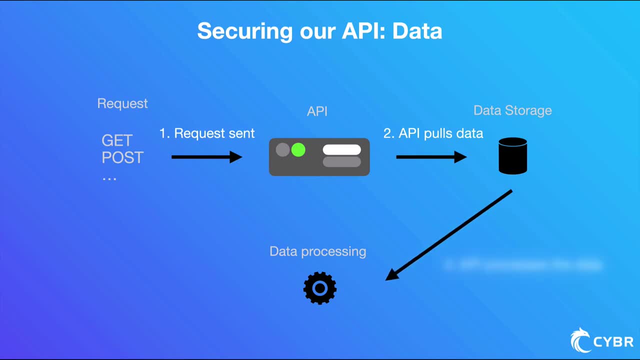 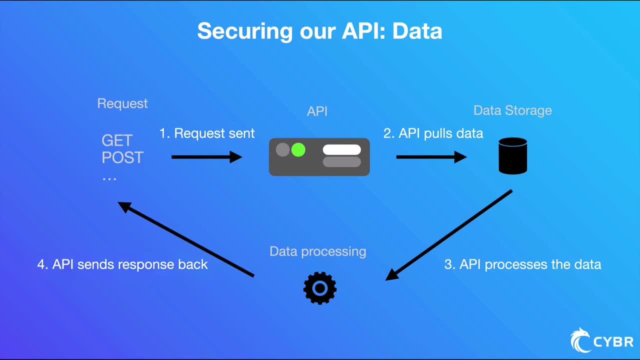 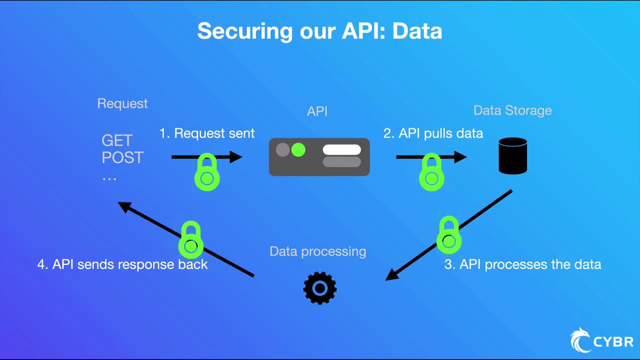 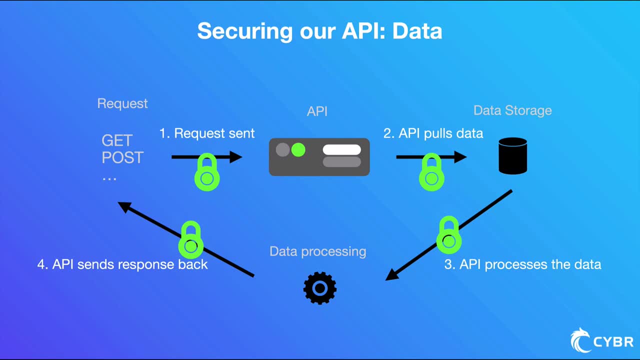 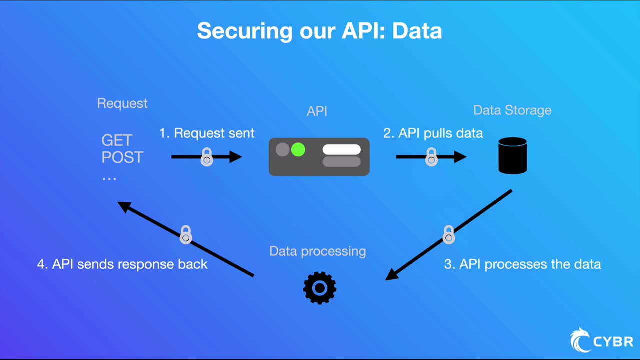 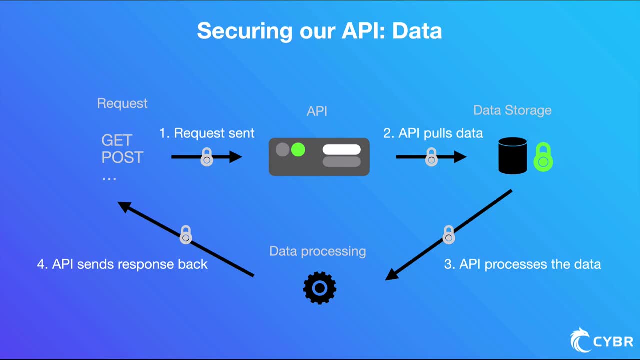 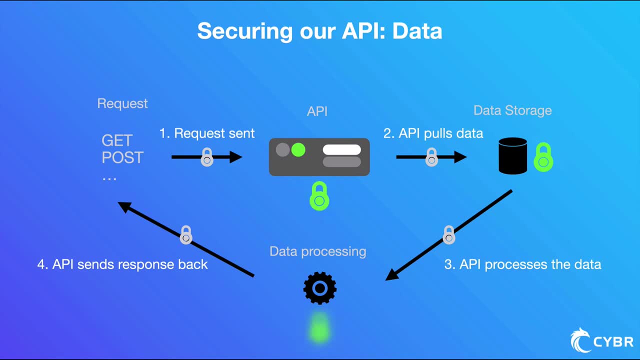 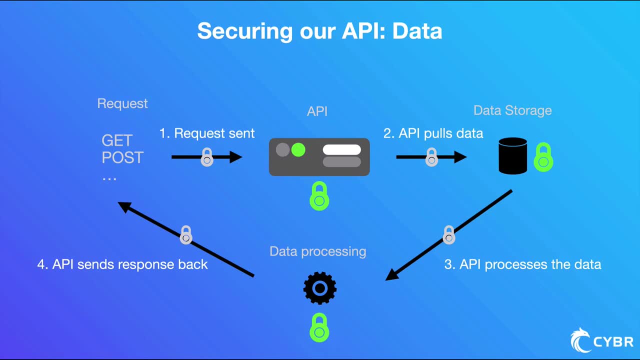 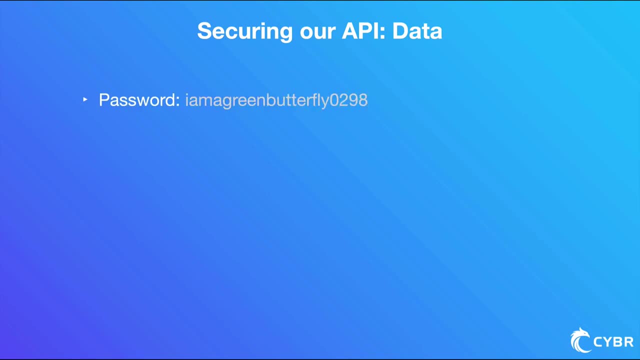 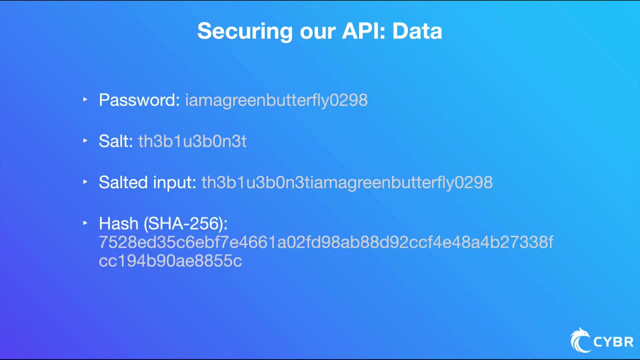 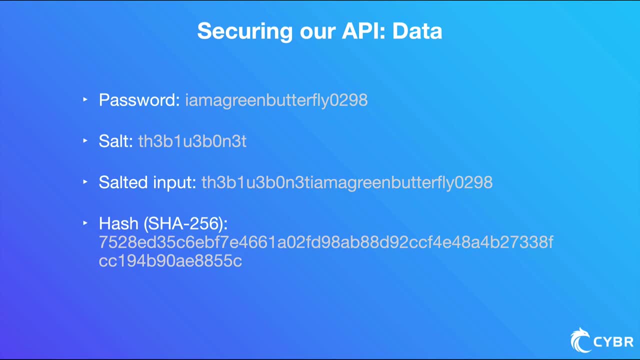 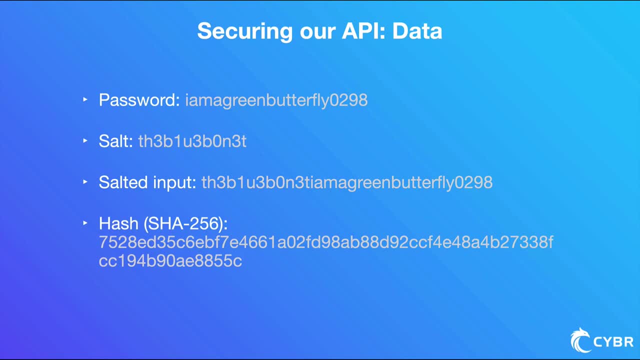 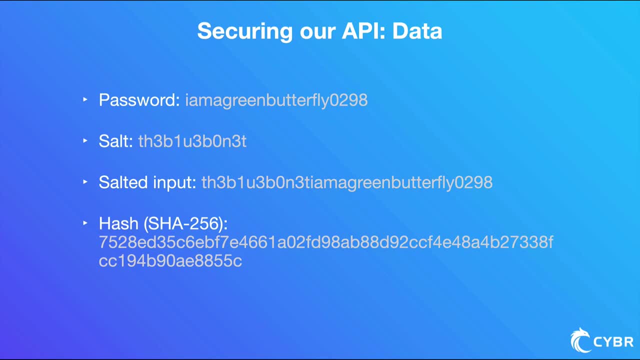 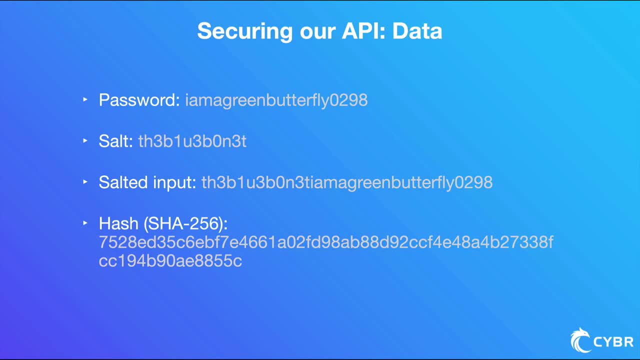 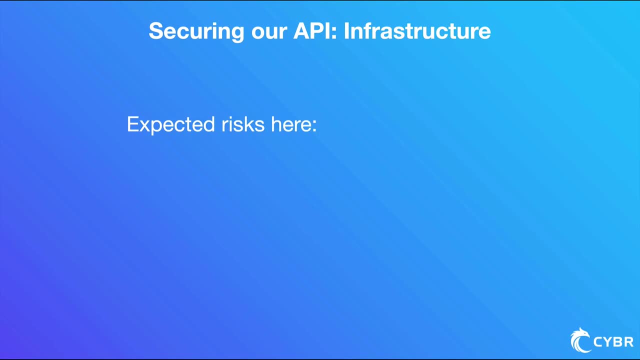 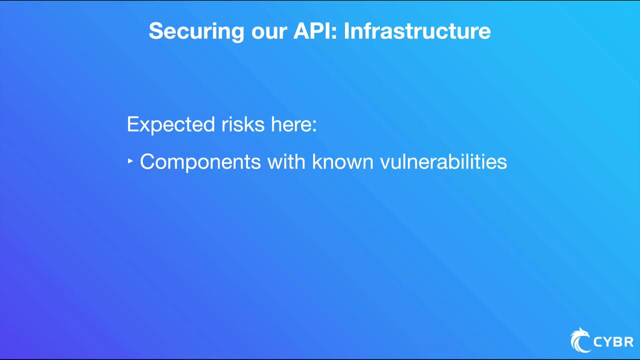 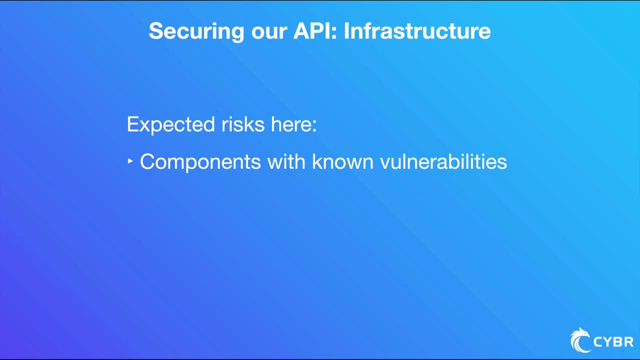 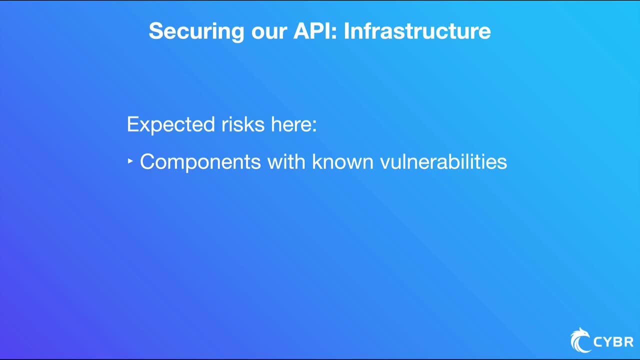 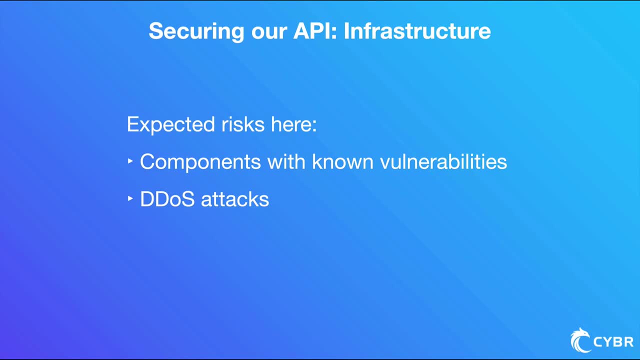 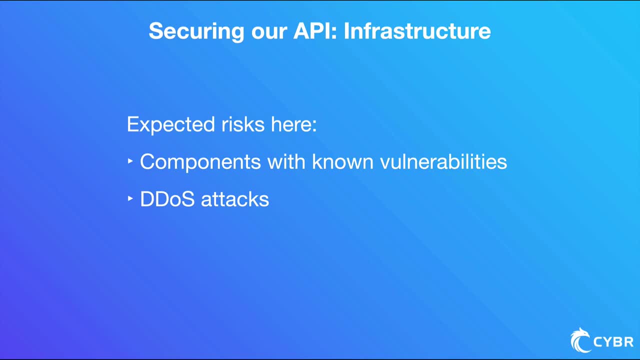 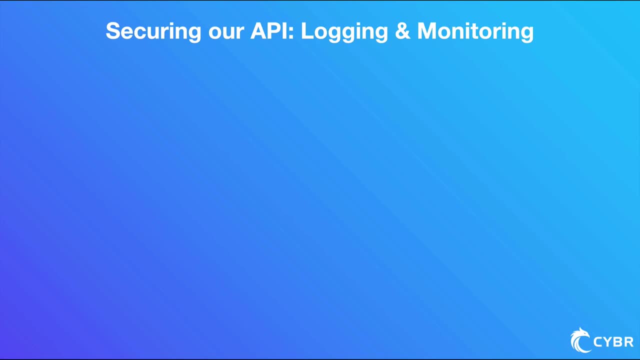 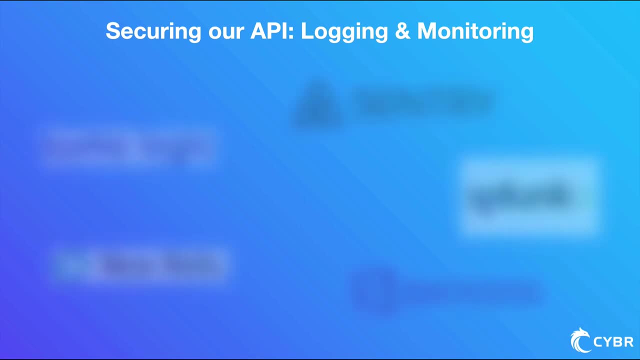 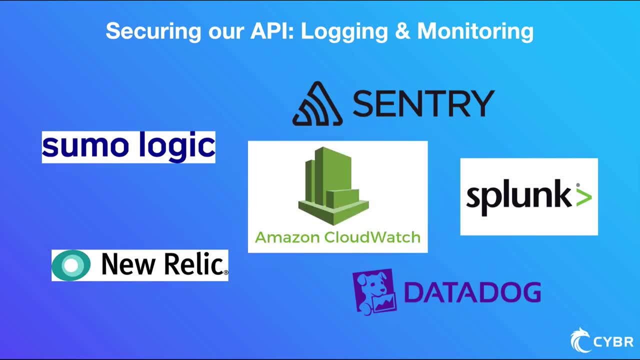 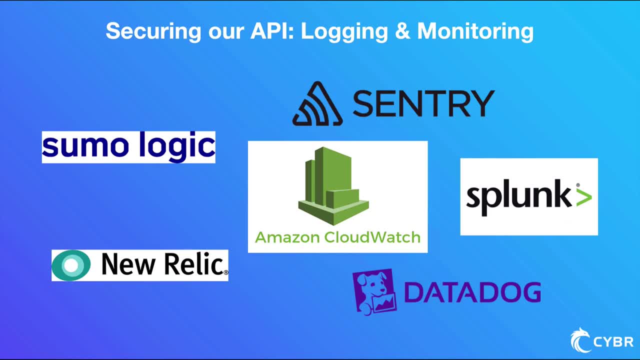 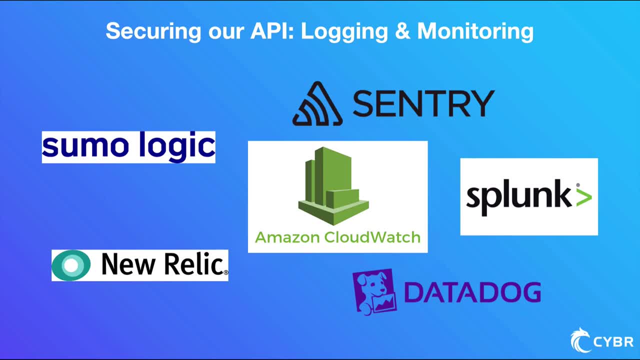 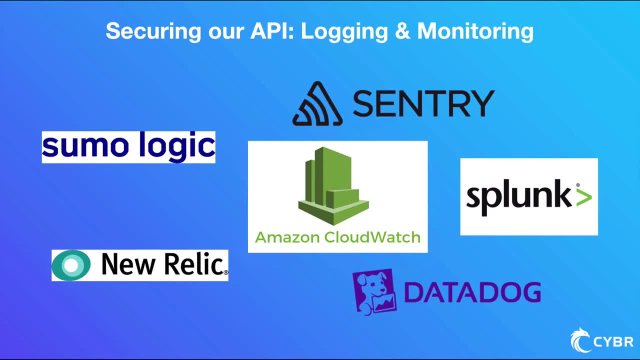 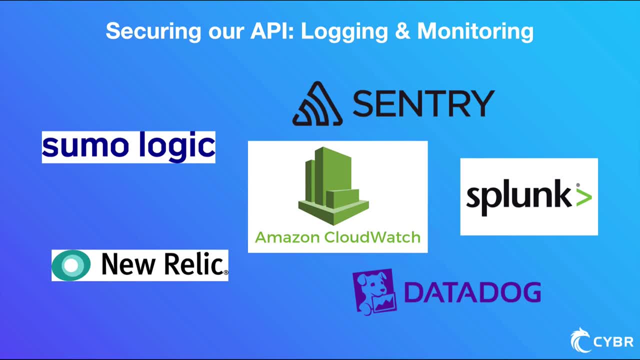 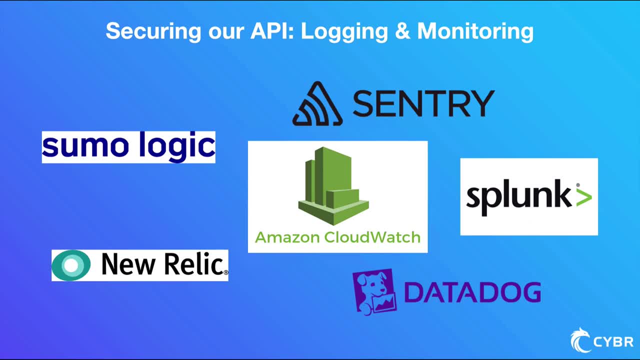 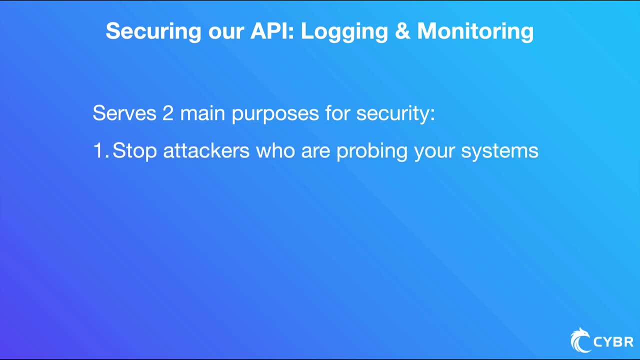 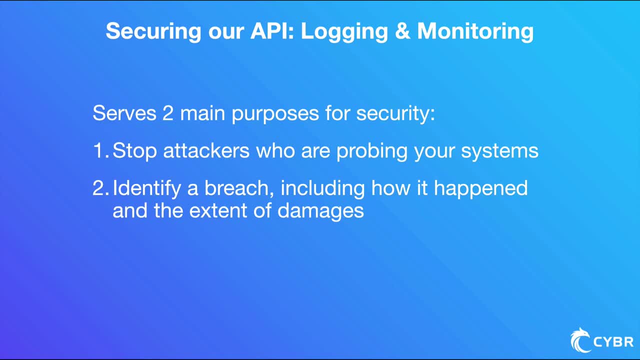 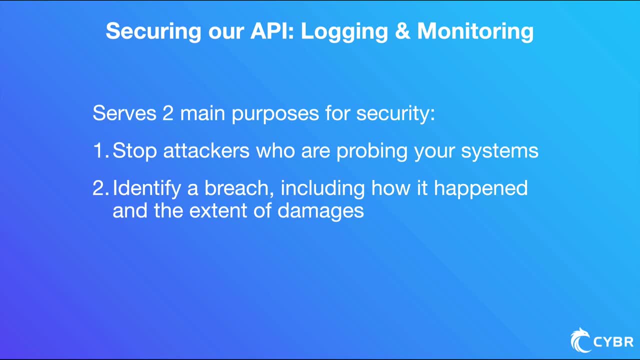 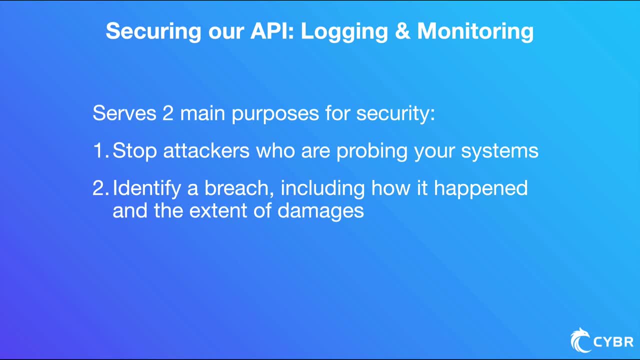 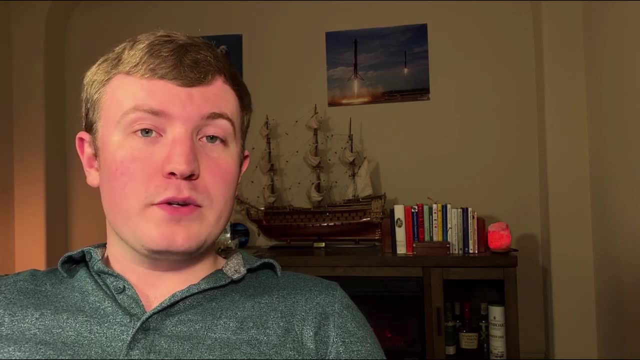